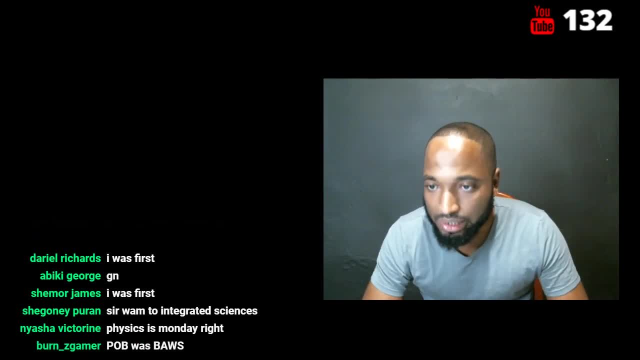 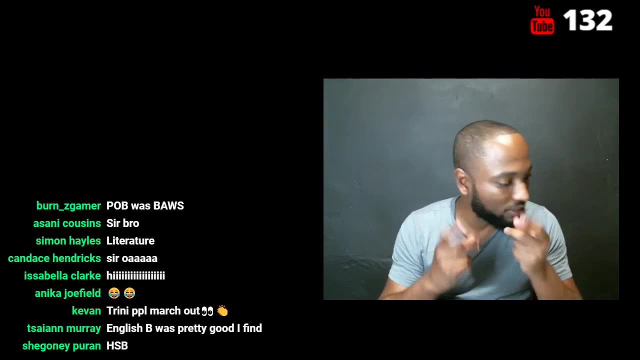 My brother Lessons How much people you have inside. We have 135 people inside already, So you all right now. the life is now warming up, So you can feel free to snap. In fact, everybody here, everybody here, listen to me. 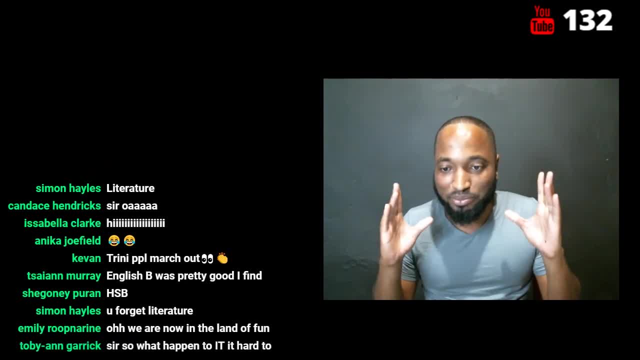 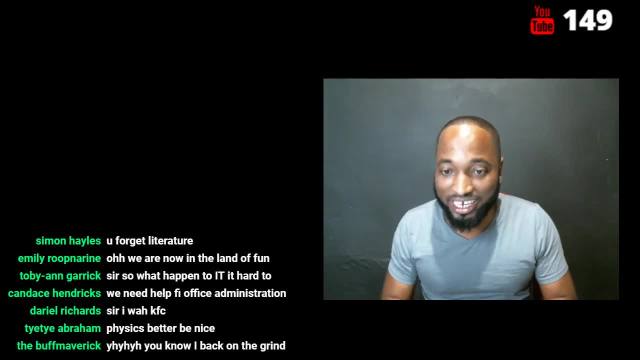 We had to get this live pumped into the max Boy. something with Caribbean people is, when I do a live the night before the exam, everybody there, Everybody there, Everybody and their grandmother and their auntie there, But like if I do a live not before the exam. 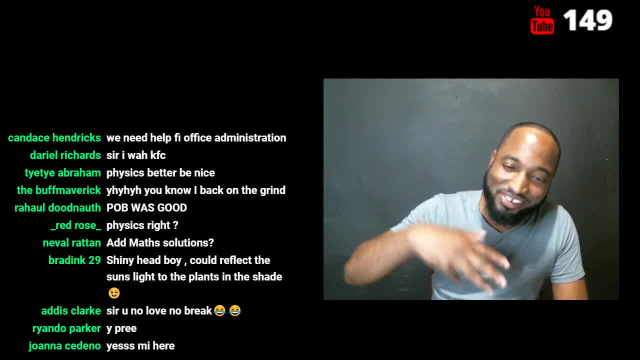 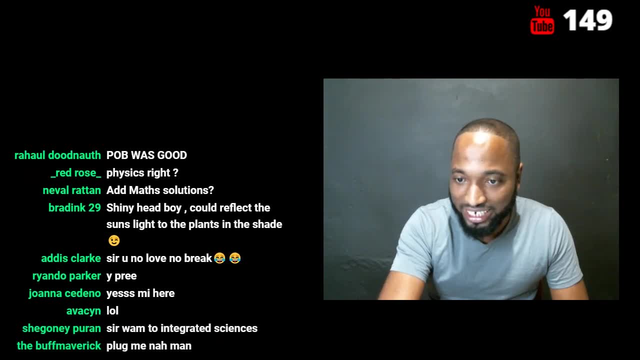 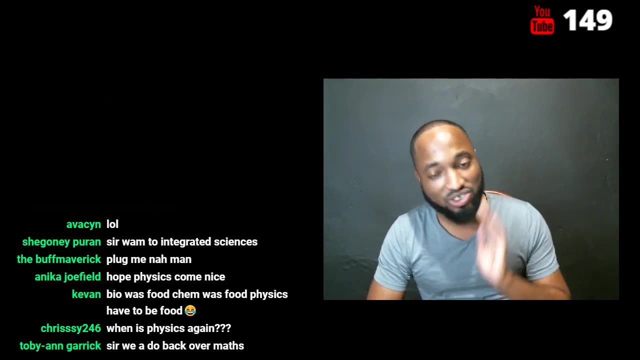 The night before the exam, people there say: we are time, man, We are time, But physics is a scene. So our everybody, Our everybody, just take a snap. If you're on Instagram, take a snap, Close it on your story and let people know we're doing our little physics course here in electricity and magnetism. 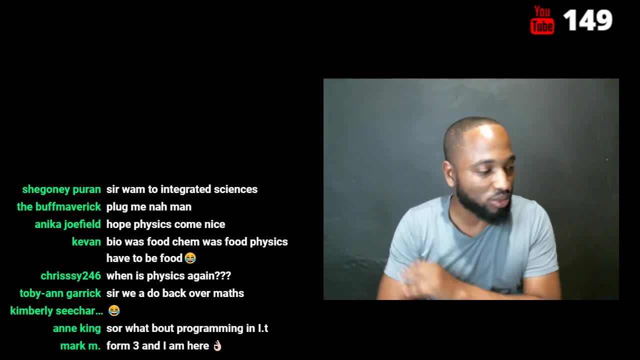 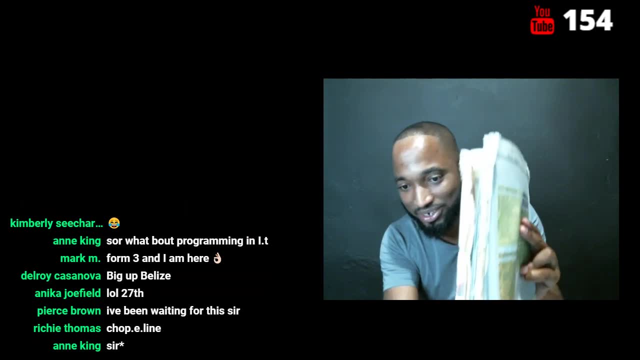 And physics and maths are my mains, Those are my main soldiers. This is the book I learned CXC, CXC, physics. You can even see the front cover, The condition of the book, The condition of the book boy. This is this book have for maybe over 20 years. 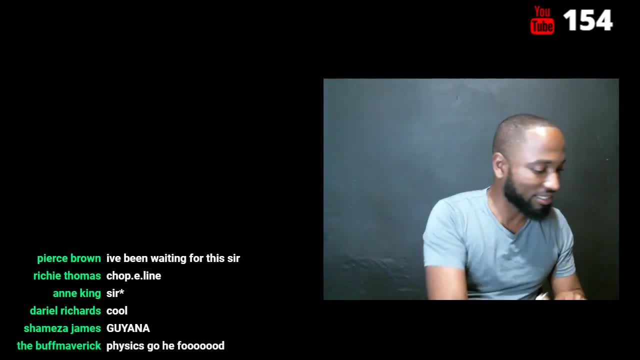 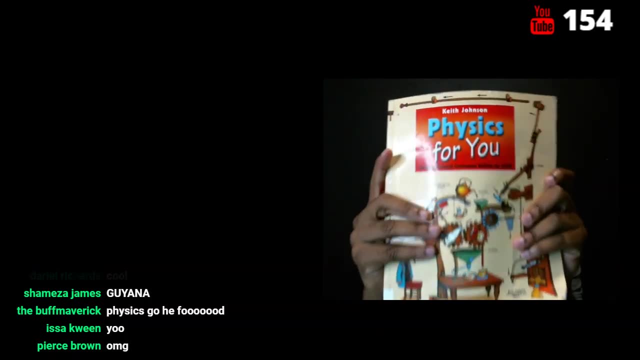 You just see the back of the book, But I have a new one. I have a new one to it. This is the physics for you. Now, this book is not according to the CXC syllabus, But this book is what I can't show you: the contents of the book. 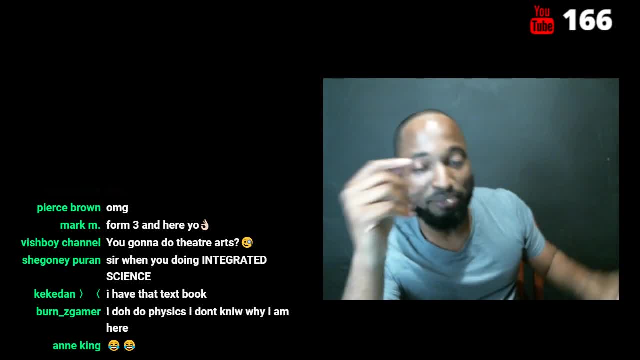 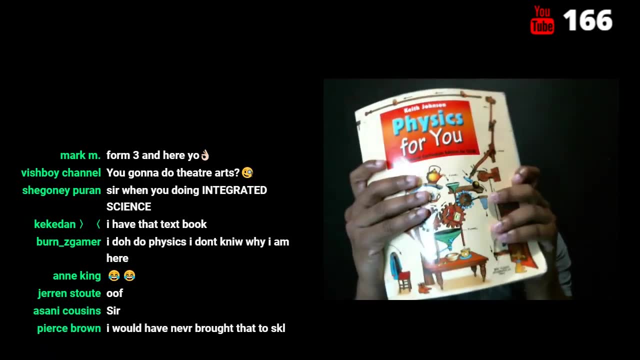 But this book is what really break down physics for me, Like when I got this book in Quamon before I reached the school, Before I reached the school in September, I knew everything in this book Because the book is so friendly to read. 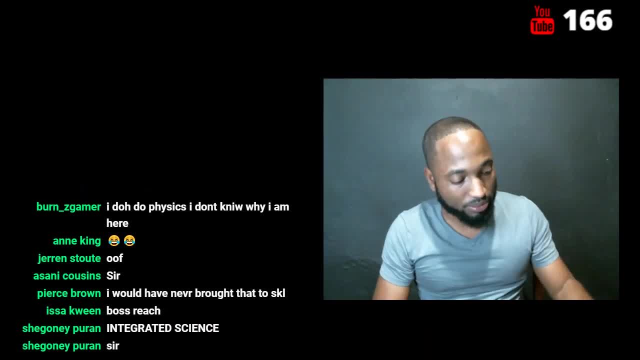 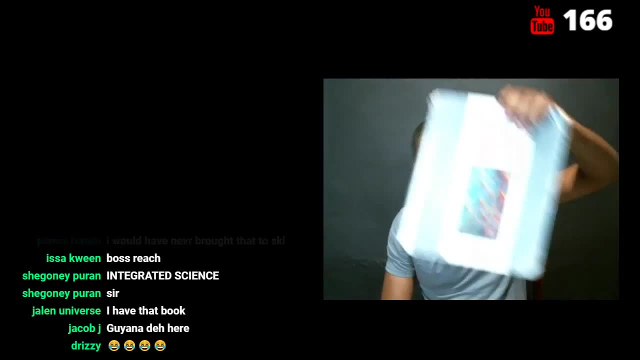 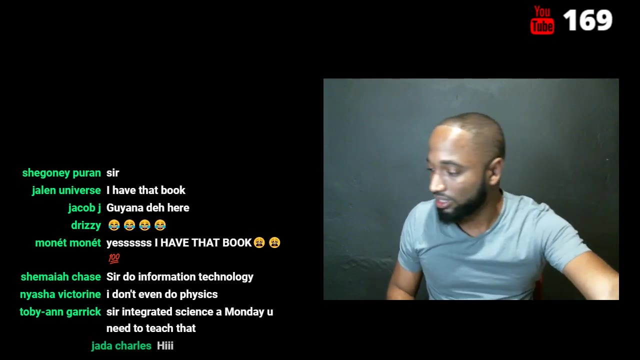 So physics was never, ever, ever, ever a problem for me. The other physics books- we have other physics books, We have this. I have a good bit of other physics books. You know, I just really buy. I just really buy books, textbooks. 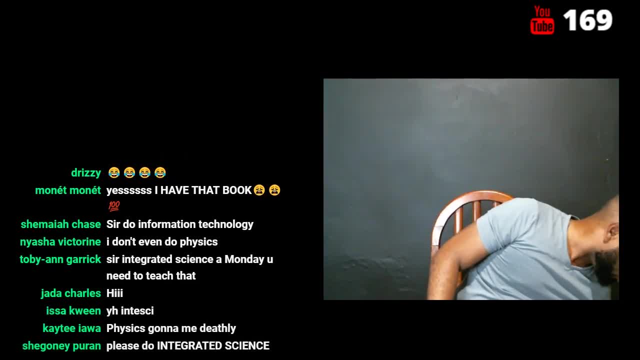 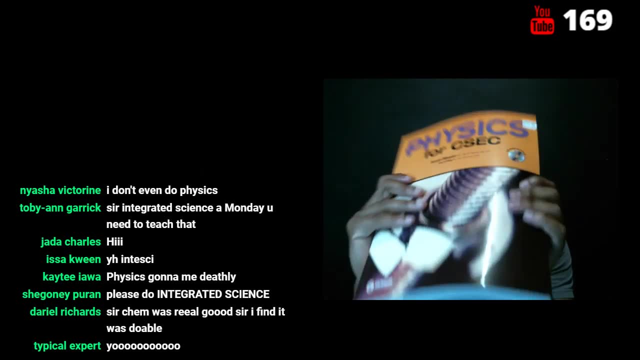 We have a new one here from a lesson teacher who teach me lessons in Cape. This is one of the latest on the market. I like this book because it has everything. This is by Manny- Anybody who's taking lessons by Manny, Sam Lal, Manny. 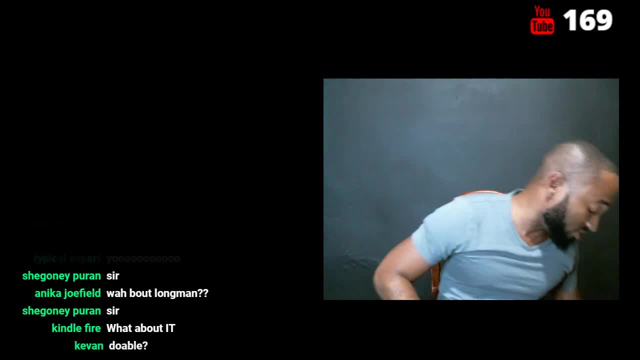 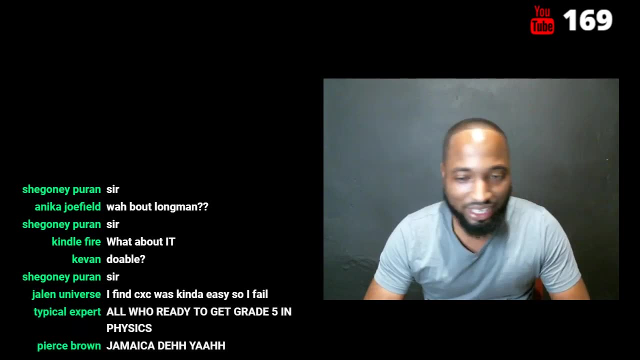 A teacher in Caps, Good, good, good, good physics teacher, Really good physics teacher. I like the book. I just have a few problems I have with the books. You know I don't really recommend textbooks. I buy all the textbooks I want to read. 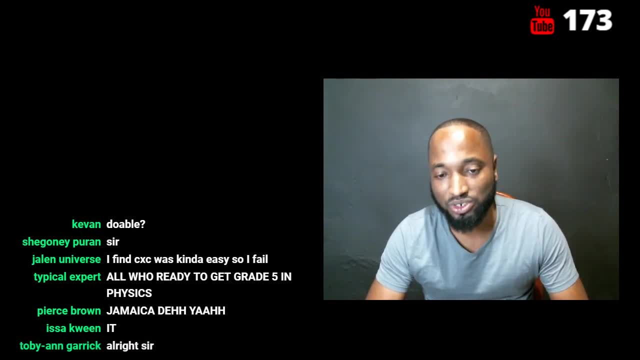 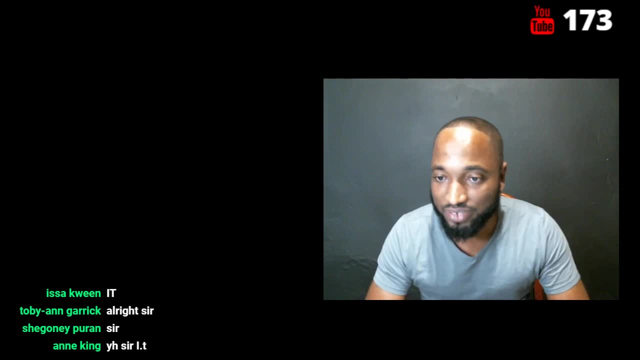 The textbook I really recommend is the Antindale by Chemish, The Chemish person. If anybody want me to recommend the textbook, they can. That'll pass some cash and the textbook better be good too. I wouldn't recommend it if it ain't good. 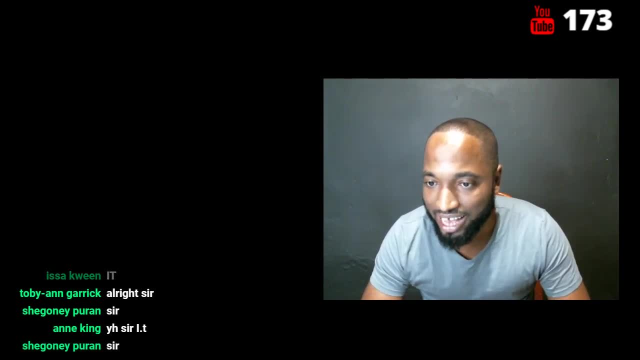 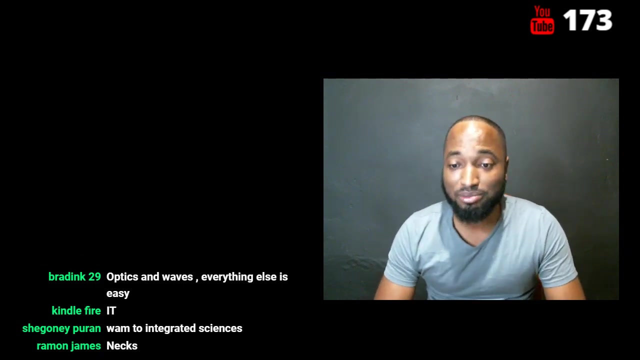 All right, sir, Sir, Yes, sir, IT, Yeah. What about IT, IT, You want to touch down on some IT too? IT requirement: I was reading some IT today. Wow, All the real definitions to learn Real acronyms and things. 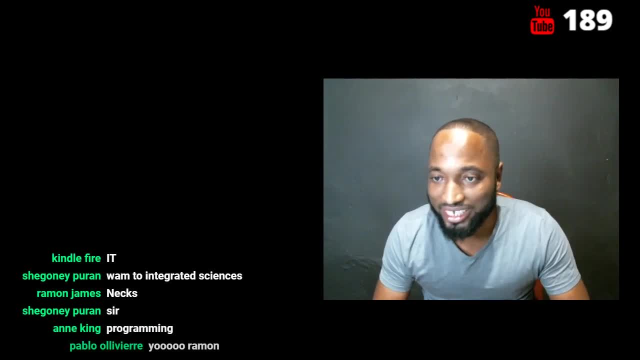 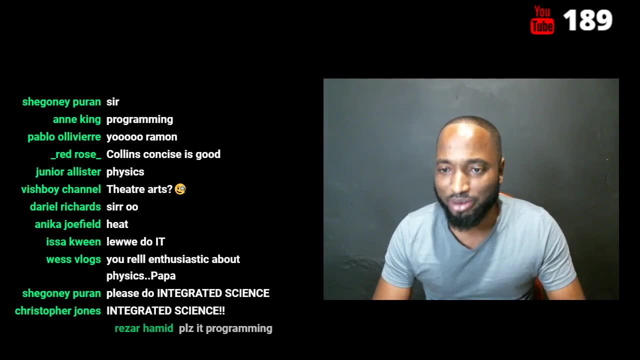 Geez, I need cheese Next. Somebody say next: No, We're starting up in two minutes, We're just taking a little talk here. We're just taking a little five minute talk, Especially when we're on the last day before exam. 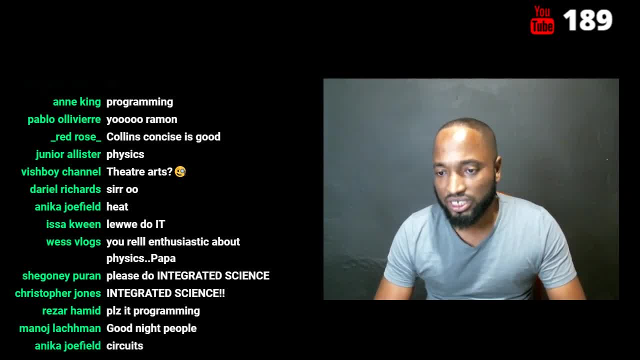 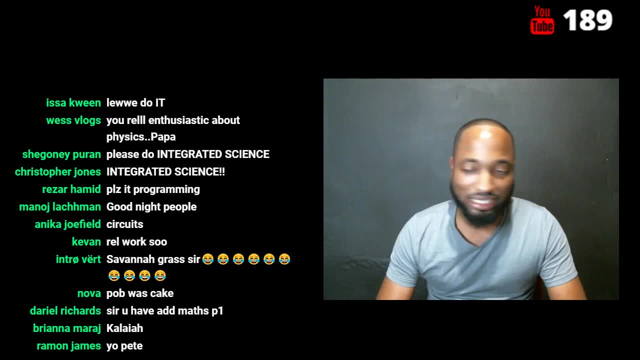 Integrated science is coming. Physics is coming. Theater arts is not coming. What is that? So we're doing? electricity and magnetism That will cover circuits. IT is going to be stressful. I want to try and see how much I can do in IT. 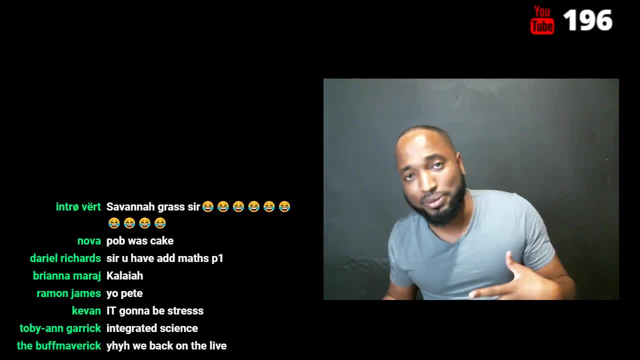 Last year I wanted to do IT. I didn't get to do it. If I could at least do maybe some programming or something in IT, that would be good. But the requirement to go and do some revision because I didn't teach IT in a while. 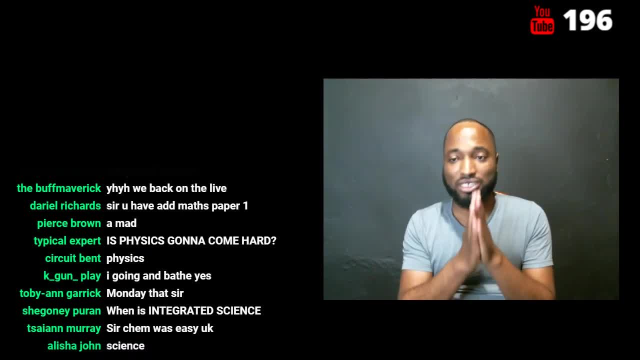 All right. So chem was easy. Yeah, Chem was easy. A whole stack of things was easy. So, yeah, How many likes on the video? Let's give them a little like: How much likes do we have on the video? We're about to start in a little bit. 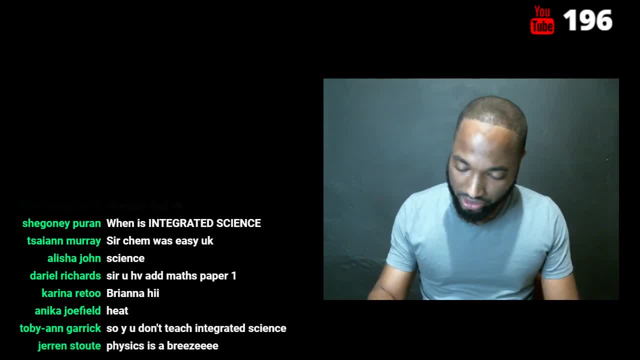 How much likes do we have on the video? Make sure and press like. I want this video to get as many views, reach as many people as possible. All right, If you haven't pressed like, press like. Let the algorithm in YouTube do it. 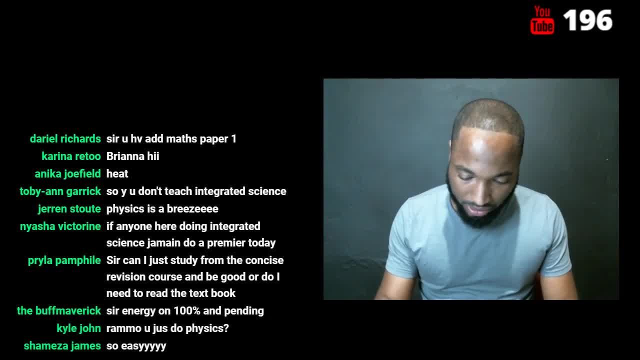 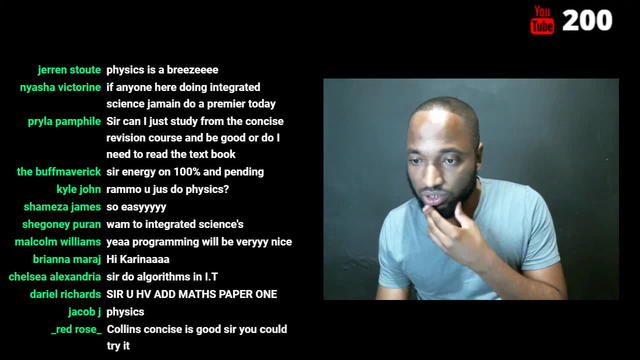 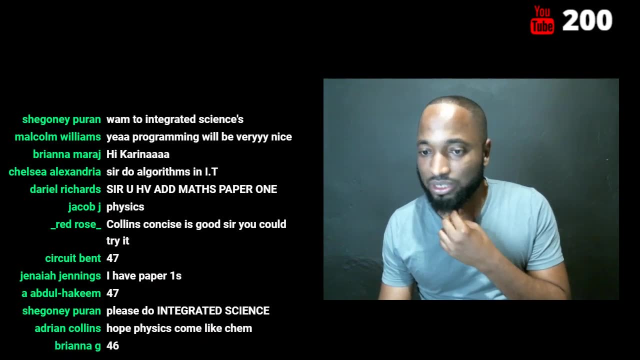 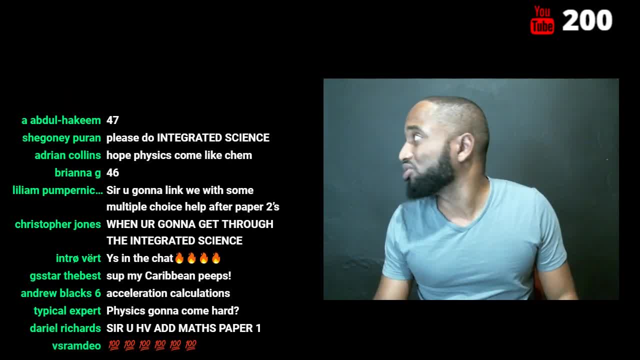 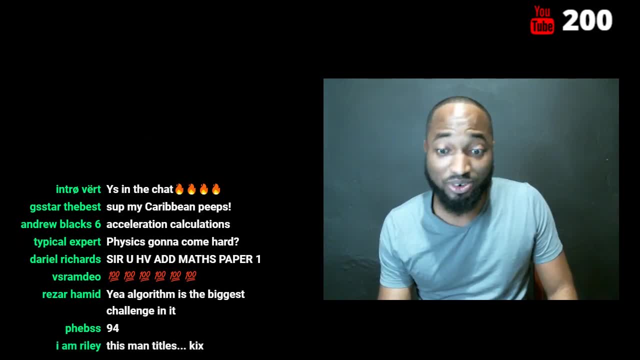 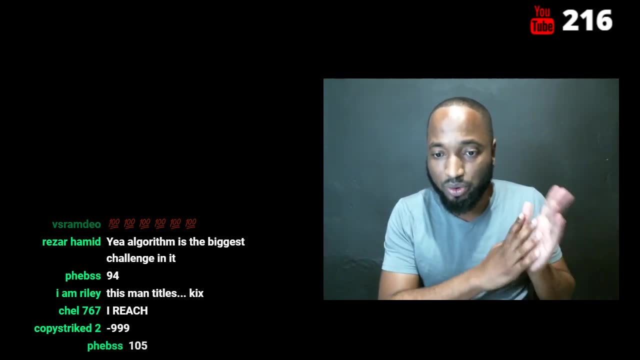 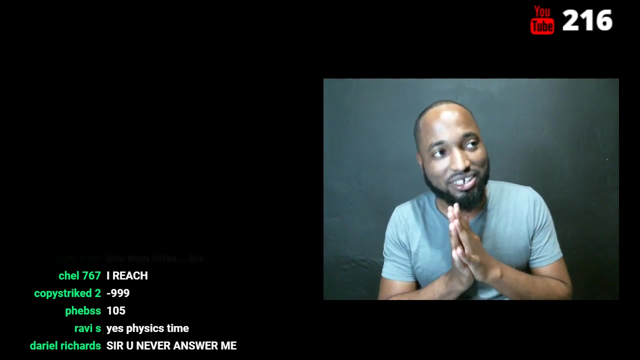 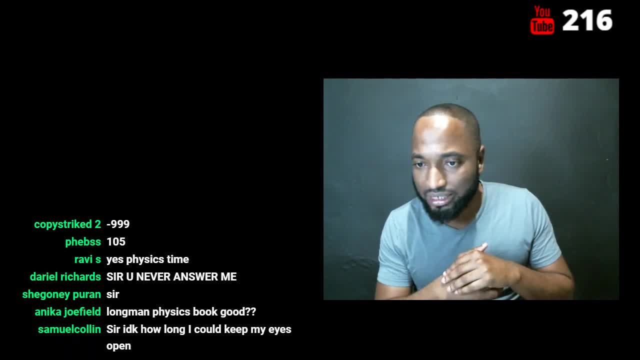 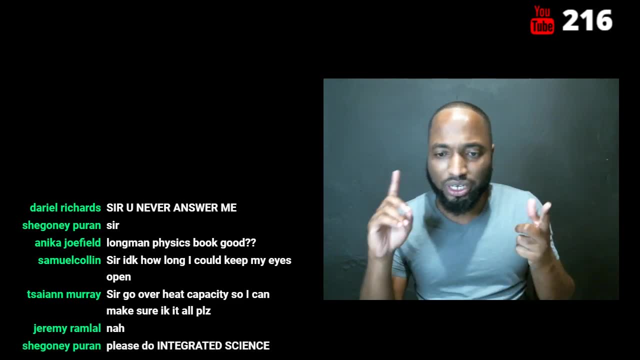 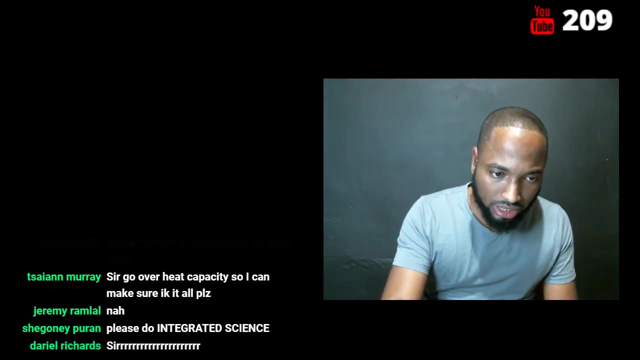 go down, everybody press like when you wanna get on five lights. half half of the two are how the amount of use and try and bring it up to get closer. so we doing electricity and magnetism, maybe we'll do is afterwards, so let's, let's. but I want to do as much physics as possible. maybe if I could cover all of 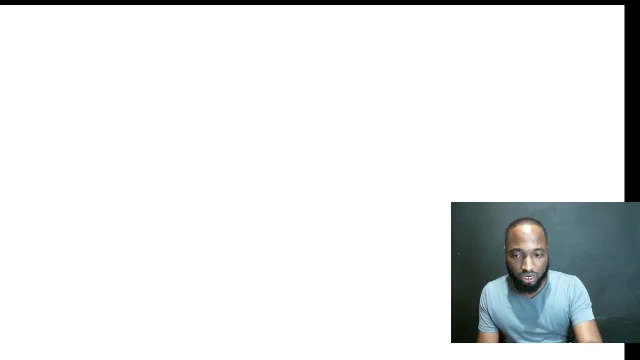 the hard stuff and a little bit of easy stuff too. all right, let's see if this is with you or you or you- this is the syllabus here. let's, let's, really let's, put it back better, feeling, crying and taking back room. you know, you know. 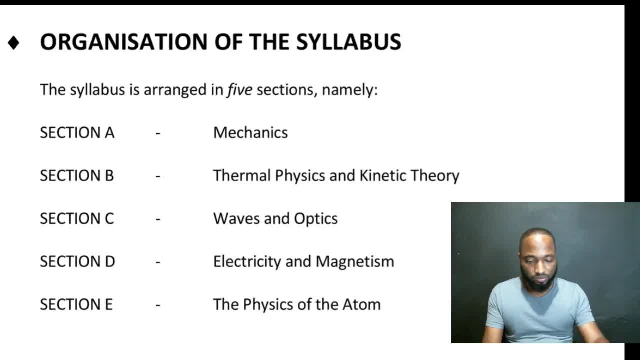 things is gone, so this is the syllabus here, you know, you know things is gone, so this is the syllabus here. so tonight we're gonna lock off where scene is one, two, three, four, five sections. right, tonight we're gonna lock off one fifth. you want to lock it up? 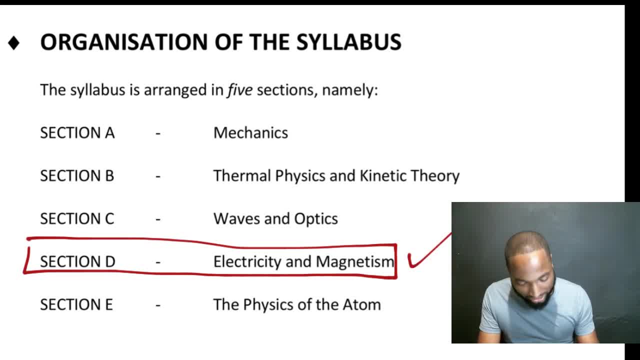 where the security bar, what? completely lock this down, completely right, maybe tonight if we finish early, maybe we can try and completely lock this down too. but I saw me. I don't think it is. you know, I will introduce my body to some sleep yesterday. see you there long lines. whoo, that him life was a signifi. I think we will. 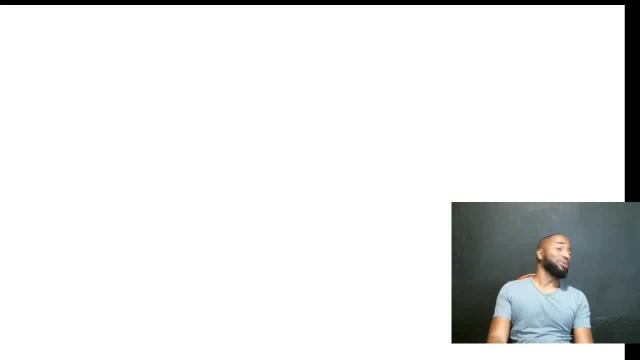 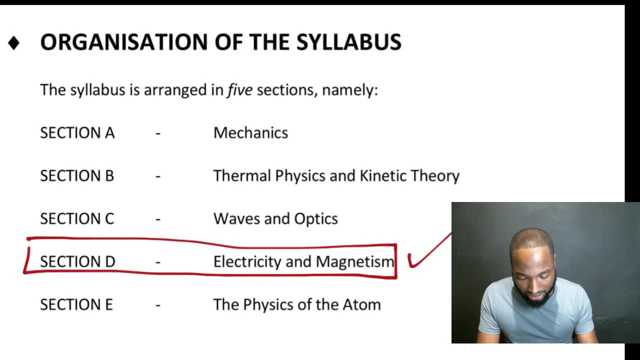 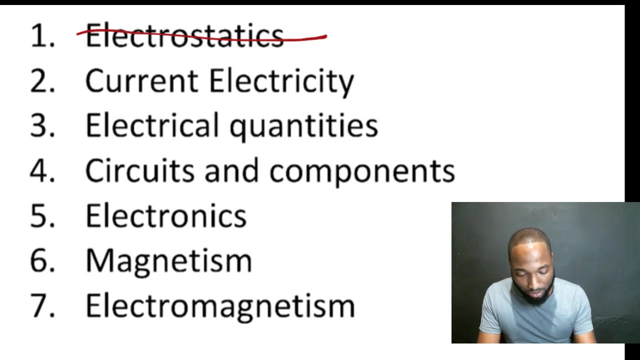 have a baby girl? you are the new hospital? I don't think so. so these are the topics. these are the topics in electricity and magnetism, electrostatics, which I already did a video on all of electrostatics. well, I'll talk about it tonight. current electricity: electricity- electrical. 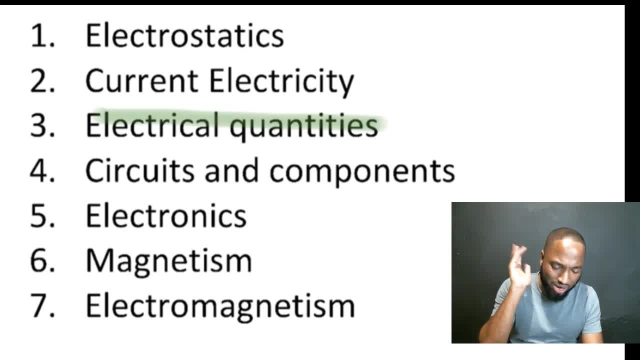 quantities, power equal I, T, e, formula, e, circuits and components. knowing your circuits, know how to do the second diagram and everything. right then, electronics, magnetism, electromagnetism. when you post an Instagram, it can't admin. tag me any post as well at Cohen Springer. so if you're not following man Instagram, yeah. 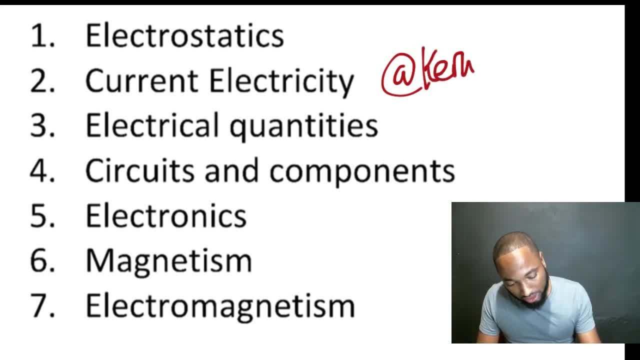 I don't know you need yourself at Cohen Springer, especially if you plan on doing stuff in a levels. I'll be continuing a levels keep. I'll be continuing with keep right to keep students all right. so three of yourself. remember we have yourself all right. so let me get, let me get, let. 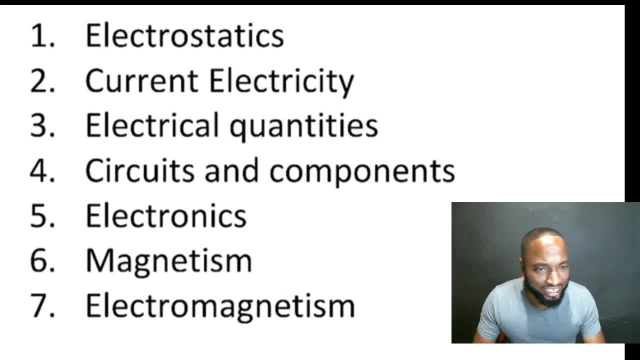 you guess that any questions before we start, let's get this bread. everything need to do here. you want some? who wants a Jamaican wish? we were prepared to do nothing. yes, like the single definition, hi ID doesn't allow me to follow anyone else. you are following people. that possible free up yourself thing. but again, this I can. 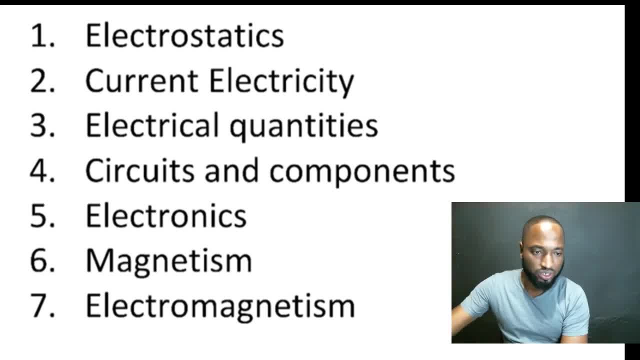 follow exactly what you need to know and not give a little much extra stuff. no, the technique for revisal can was being concise book the technical revise in physics I always say theory vices. you want to try and understand as much as possible. you can revive it's concisely. I've just diplod vacant in now in that one week it. 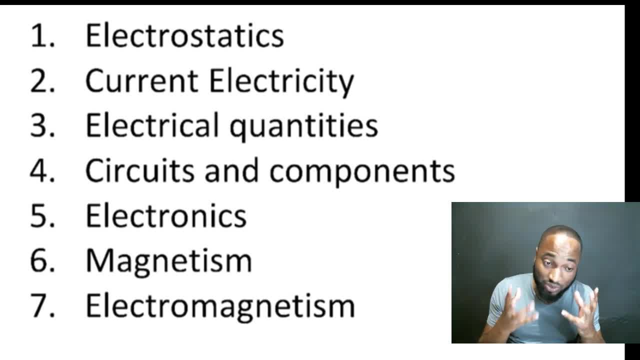 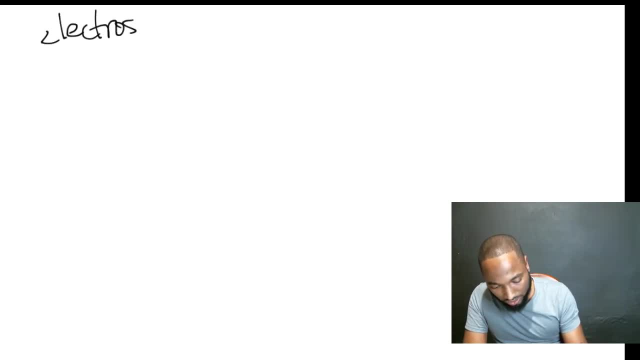 will be hard for you to do that. physics becomes very easy for you when you actually understand what you're doing right. so we started off a church. we started off with electrostatics of my pen. my pen wrote tonight, so you let your statics. I'll be asking your questions here. my next textbook to the habit in: 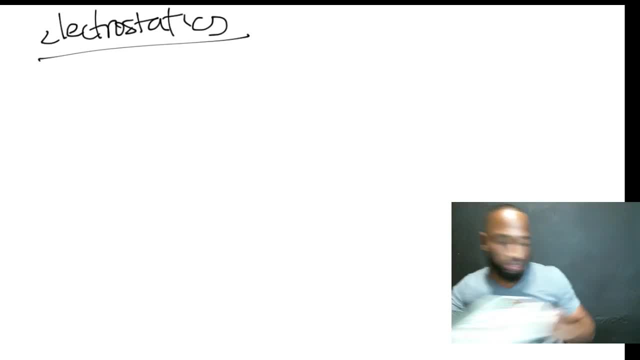 point form. so I'll be on precision. yeah, how we all feel about electrostatics. there's like a little beta question. make it up in the beginning. the big formula: anything I need electrostatics is Q equal I T, Q equal I T. what you stand so. 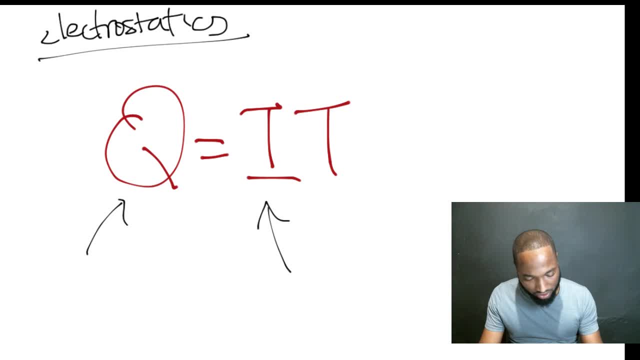 what does Q stand for? what does I stand for? what does T stand for? so there's the first thing you'll get. so enough blood line and get shitty, we in it, we inside, we inside. what does Q stand for? I should know Q stands for charge right, charge, charge. I stand so current right T is. 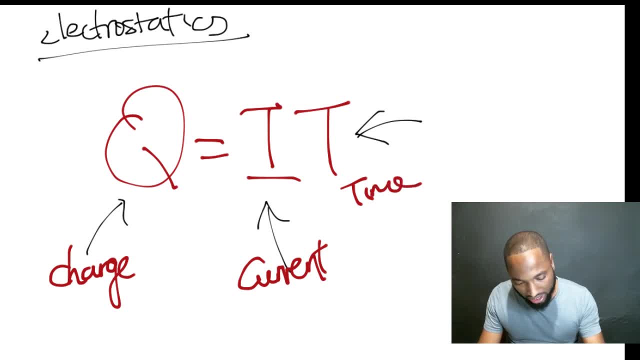 time, obviously, and the units would be in seconds, current amperes. anybody person units Q is in coulombs right, coulombs, coulombs, coulombs, right. so that's the that's. that's that's our SI unit day. you need to know what. 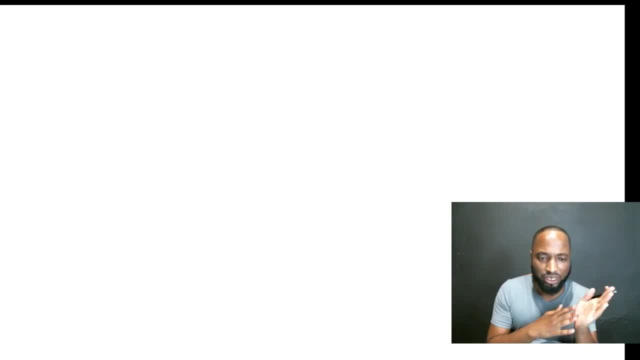 like friction. when you do the friction experiment, some things will be negative, some things will be positive. what I'm talking about is like if I run and you rub it with cloth, remember some of the elections has come off. one is been negative. sometimes when you're a bit, it caught elections going well yeah. 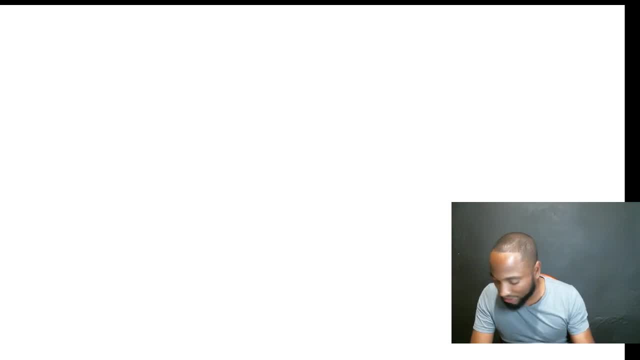 yes, yes, the positive ones, the ones that turn positive was the one that in positive, and when the world is that too negative, what are the ones that turn positive? what are the ones that to negative? I'm at accident office administration, where I I do know a office administration. 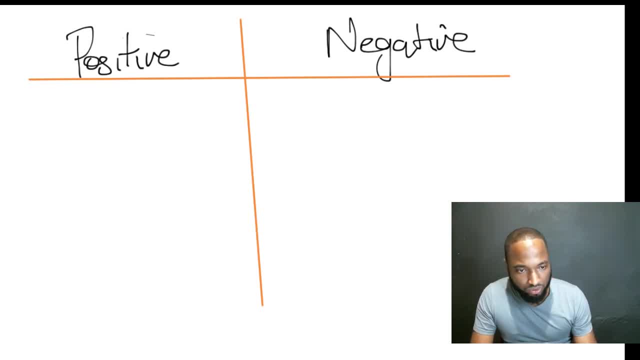 I do that. so the rods, yeah, what which? nobody seen it, okay. well, I'll give you a clue. the one that's in negative, there is quality. you remember that quality, neural experiment and your ability to plot the ones that in positive would be like, which is the cellulose acetate, cellulose, cellulose acetate, oh, and glass. 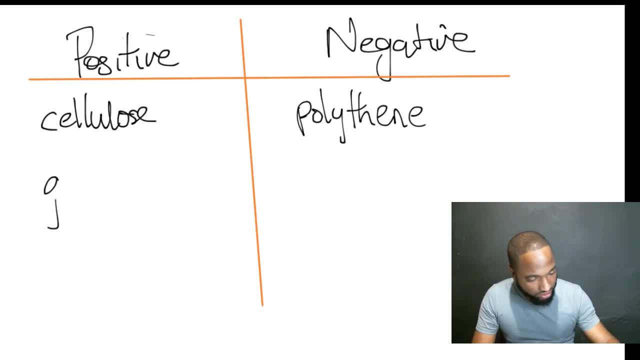 as well. yeah, glass, let's try to make sure open right to certain parts of a screen you know, today comes on, you can ask me tonight, yeah, glass, so some people, some people never see this. we didn't learn this. well, you know, you know. but normally they will tell you which which one it is. well, we come in everything a. 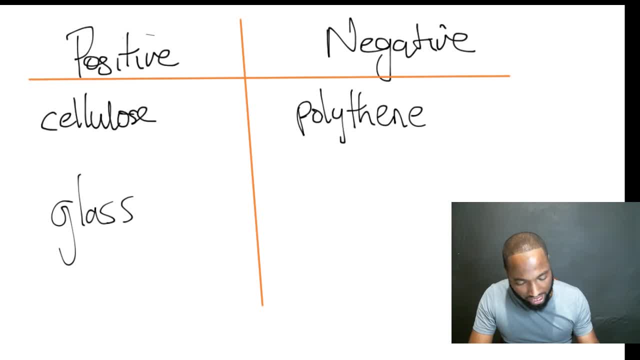 little worried or come in everything glass and an excellent. nothing positive is some people ever night or some kind of thing, so I don't think I ever see that before. right you. this is like, if you have the rod, I run and I do a video and you let your. 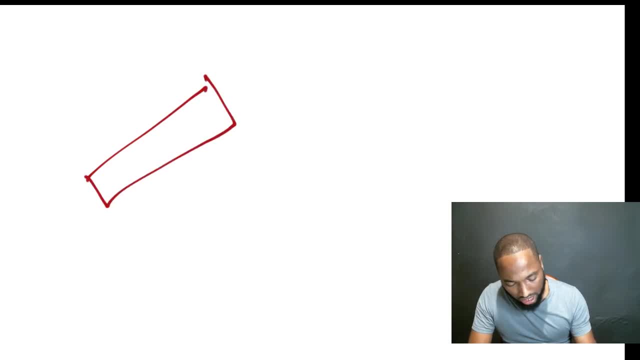 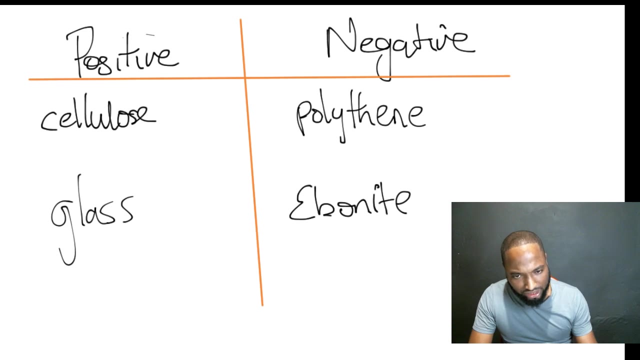 statistics. you can probably take a peek at that when it's like: done, I have a rod. depending on what the material is in Europe. your material you had made out of this back would be positive. what material? you rub it with some kind of cloth- now you was there, I've been to turn negative. is that a rabbit, a cotton? 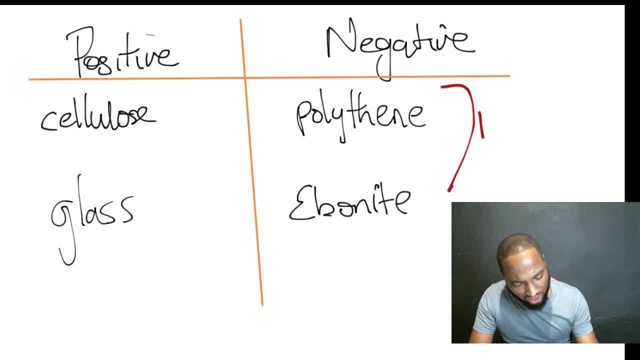 cloth, no food food, food, food, food food cut nothing. and this one I have been to turn to positive. do not use sick. oh, not to forget that, not, we want to will them. by the thing, this one uses it. right, not too important what it's your catchy. 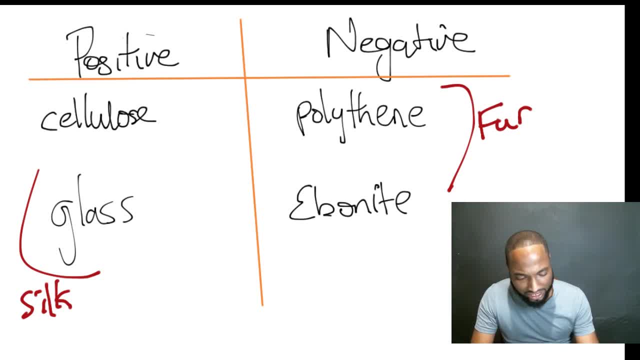 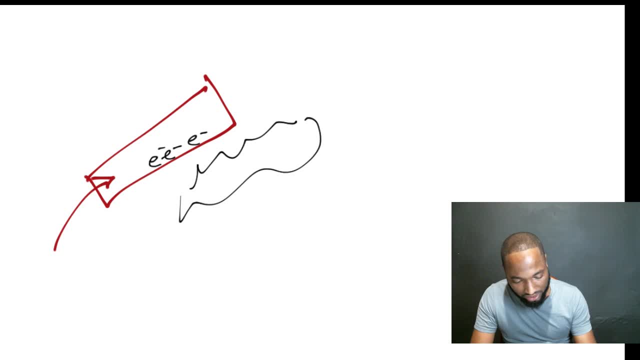 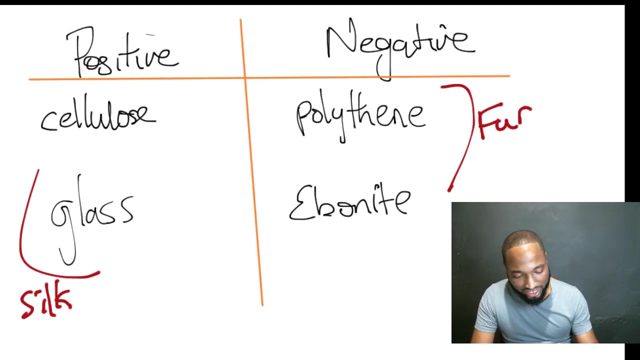 idea, but you need to explain what happens and I did that in the video when you're Robin. it's electrons actually transfer of the electrons can move some electrons on the surface when either go this way- all in the case where it's in negative electricity from the clot actually went that way, so it's obvious. now if you're turning 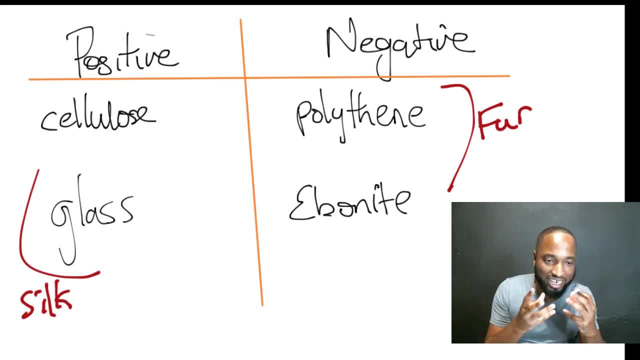 you. if the rod gets more negative, it's because it get free little electrons on the surface. you get a surplus of electrons. if you get positive, it's because it lost electrons. all right, so we'll reach generators and things. we'll reach generators and things. we just we're just chatting along with a full 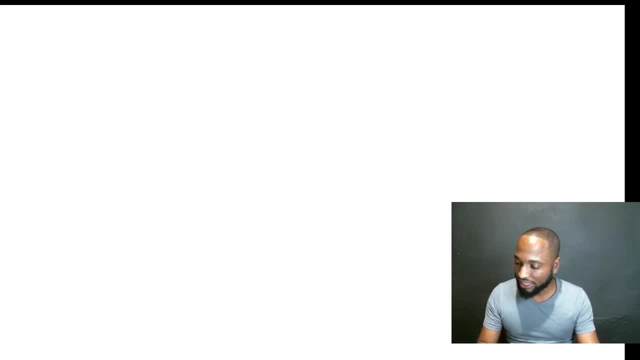 course revision. everybody should know how atom look at skipping that. um, i should mention this charge is also equal to the number of electrons times the char multiply by the charge of one election. right, anybody ever see this formula before? if you ever see wise in the chat, if you ever see this. 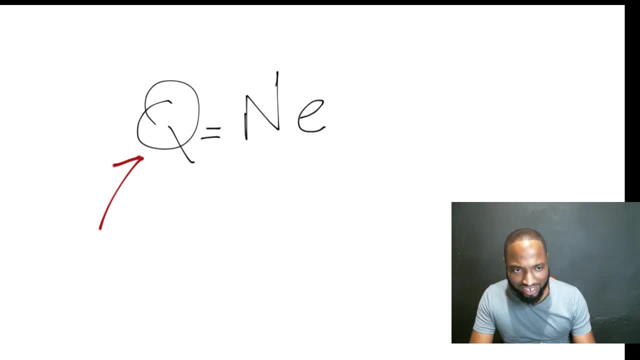 trip. i, i must, i must skip atom. i mean, if you don't know what time is, what going on, what going on with you? right, that's why i say it important: don't, don't take all the little basics. no, don't skip the basics and wait for the 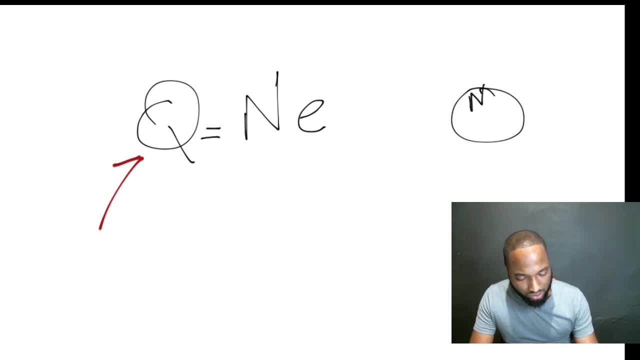 hard stuff alone, taking the basics. so you have your nutrients, you have your proteins, things, the nutrients and the outside we don't need to talk about. if you don't know about that, going to study better, you start back for a month, right? so you must know your. 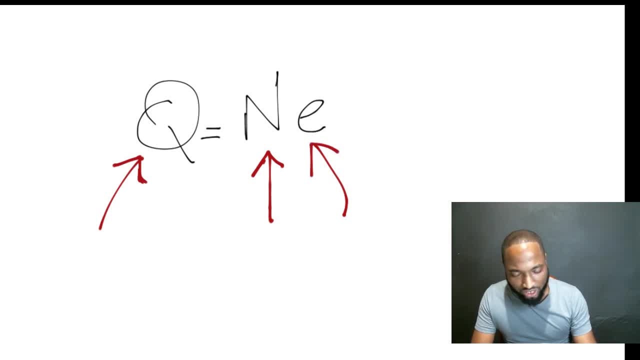 anery electronsхez parrot chu60 ai. given The charge on one electron- anybody know it offhand- It's 1.6 times. it's very small: 10 to the minus 19 coulombs. It's a negative charge. so I can put negative in front here. 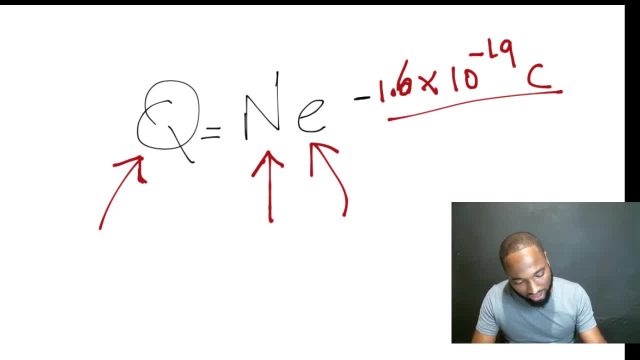 That's the charge on one electron. So one electron has a very small charge. One electron has a very small charge. That's the charge on one electron. So if I want the total charge, I need to multiply the number of electrons by the total charge, right? 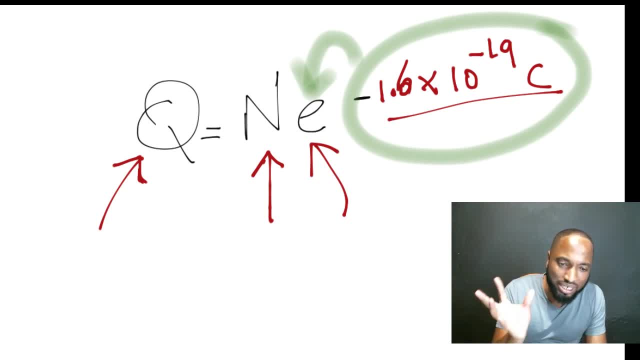 So for everybody who's saying: why is this? It's just a simple little thing. A simple little thing, trust me, And if it comes you might be just glad I mentioned it. It's just a simple little thing. they might guide you if they try to bring something like this. 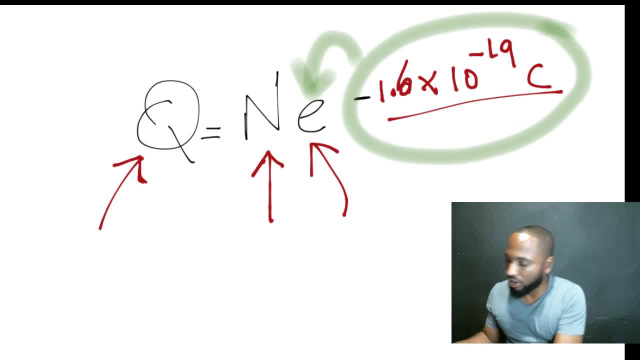 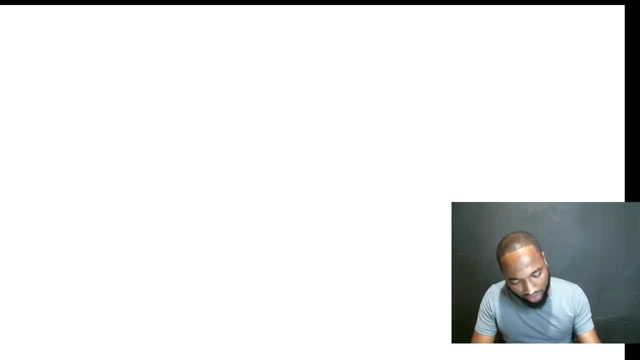 You'll more see this in. keep right. What would happen? what would happen if I have an experiment and I have two types of rods? I'm going to make this a different colour And I have two types of rods and one rod is positively. 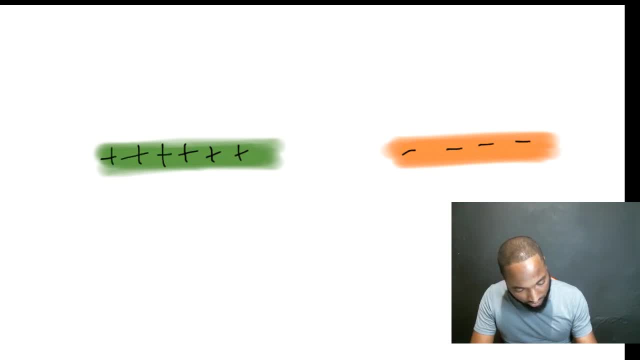 so where's the positive one? One rod is negative. So this would be like the acetate, the cellulose rod, And this would be like the pulley. you know, Right now we just went to right there for the pulley. 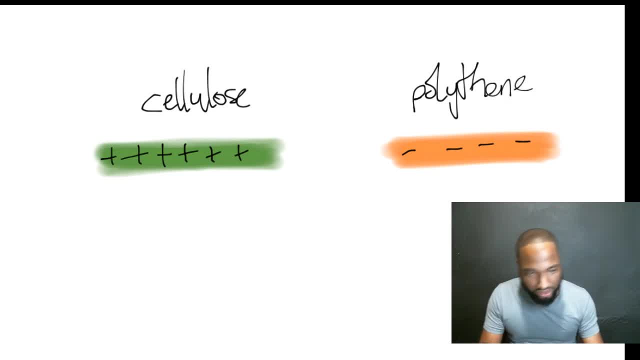 Let's start zooming in and out the right, The other at that. So there would be some attraction between here. Now I should put the iris like this: There would be some attraction. there'd be so much action, me and obviously, if we, if this run, if it was. 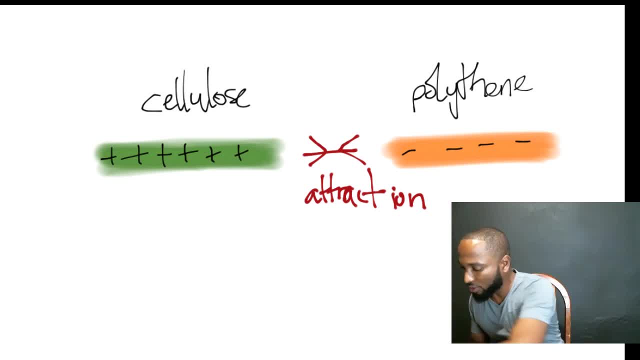 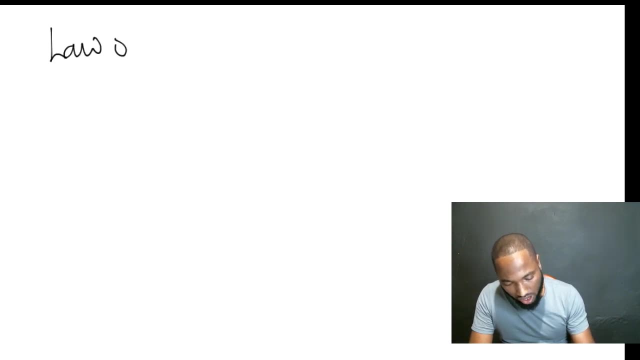 two of the same rats. it was two of the same rats, they would repair. right, it was two of the same rats, they would repair. now, can anybody write out the law of conservation of charge? anybody know the law for the conservation of charge? anybody know the law for the conservation of charge? 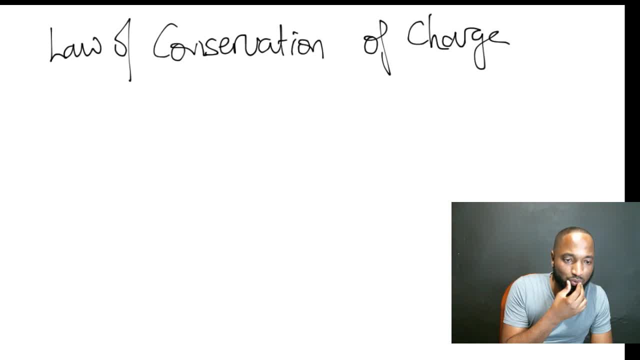 now can anybody write out the law for the conservation of charge? nope, what? what energy? that probably not. energy cannot be complete as the law of conservation of energy. so people gave me the law of conservation of energy, but the law of conservation of charge. yeah, Antonia, see you coming there, bless up. 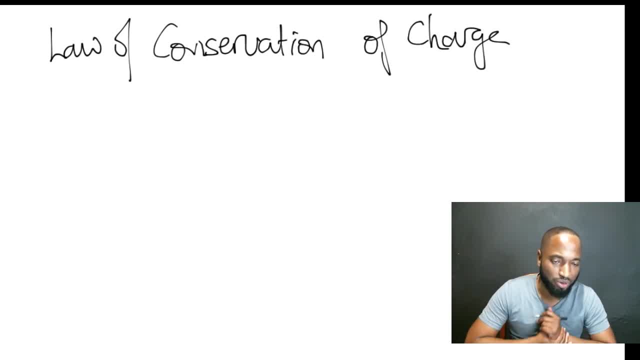 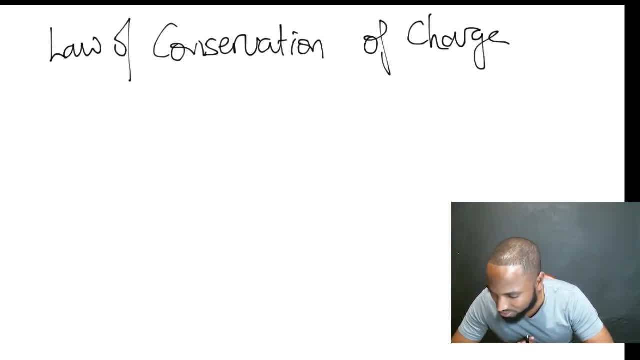 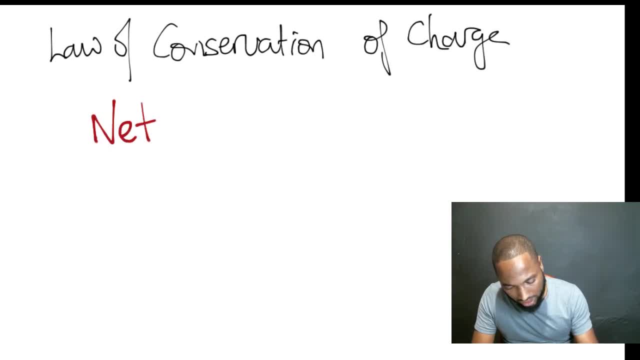 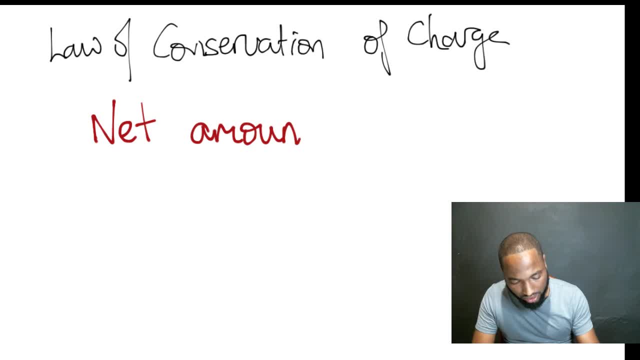 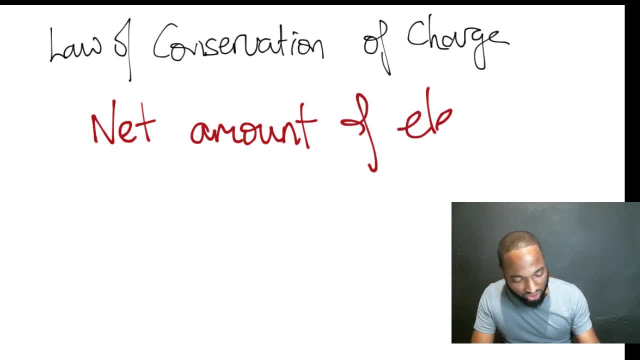 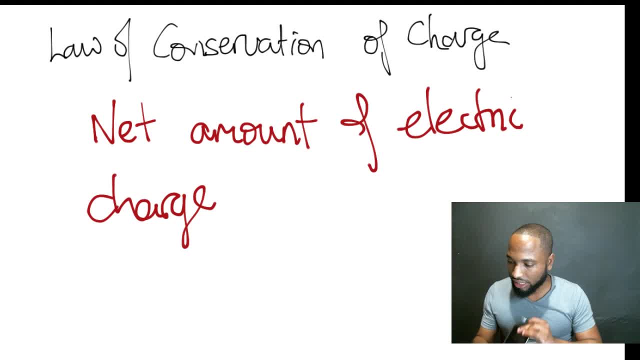 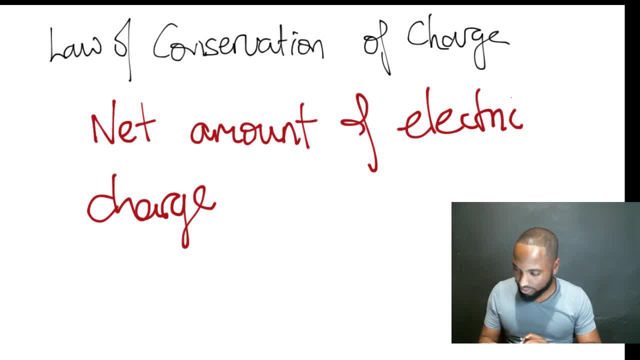 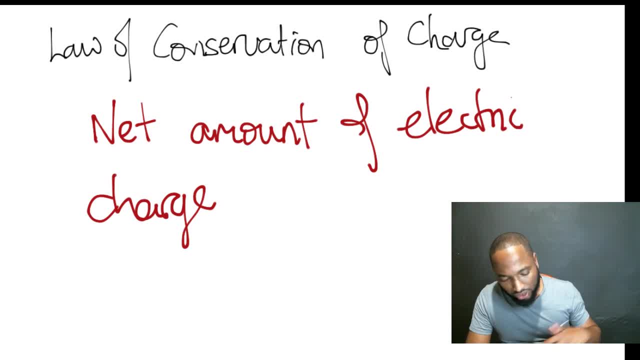 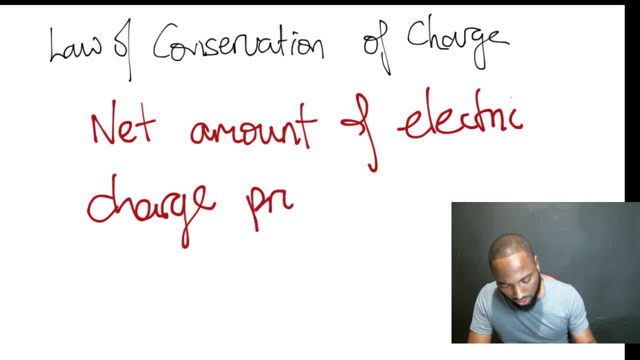 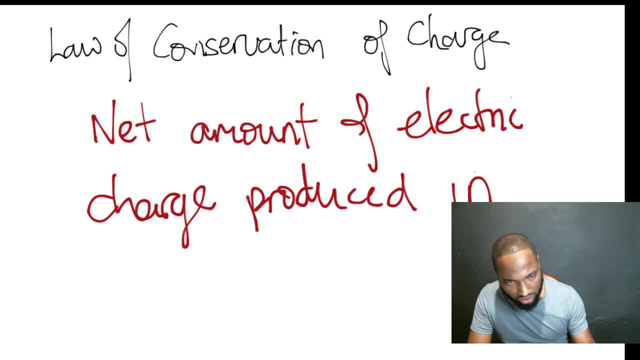 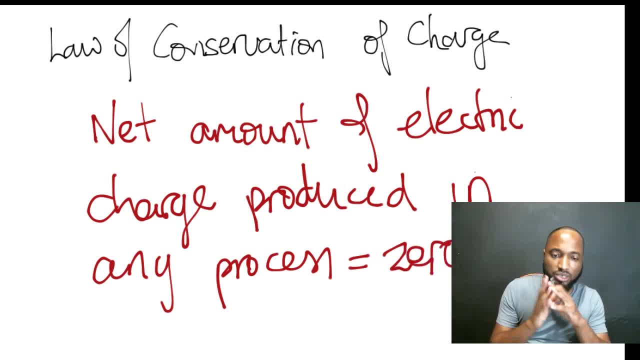 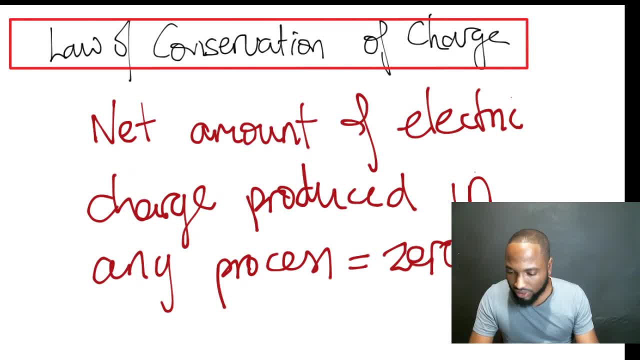 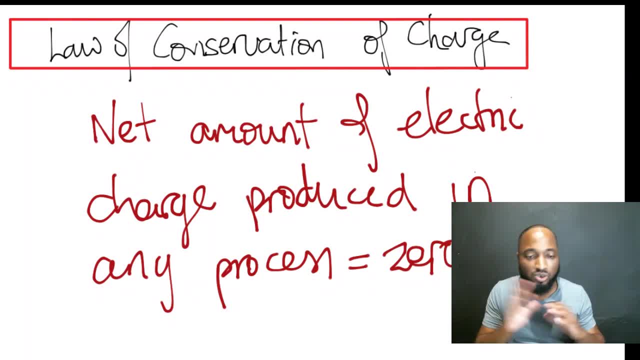 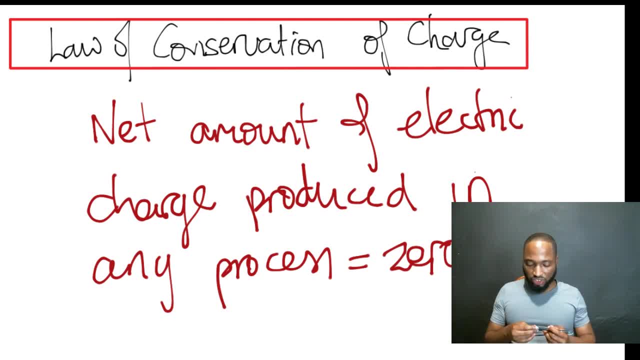 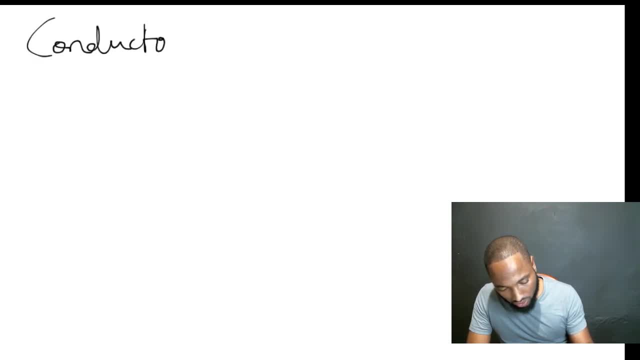 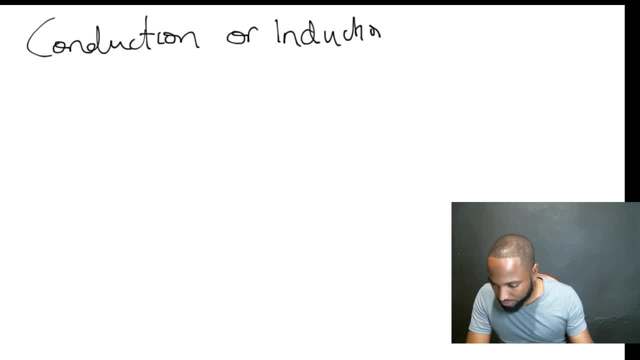 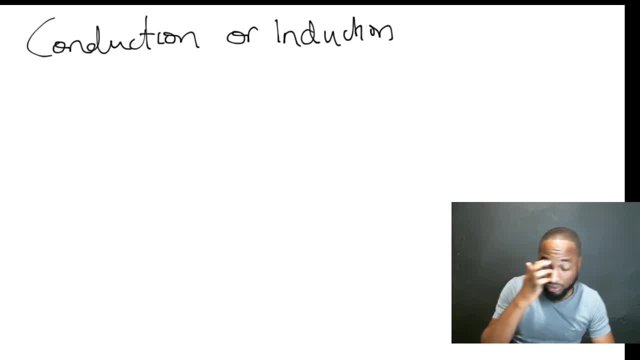 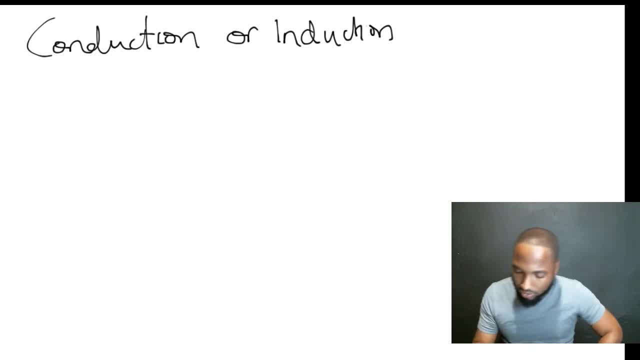 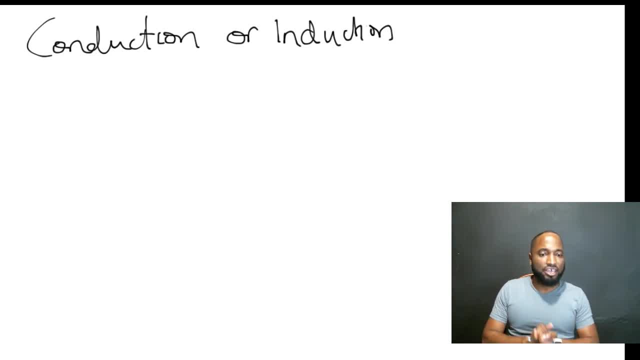 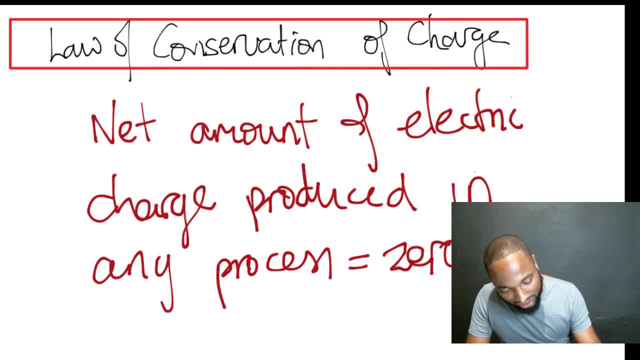 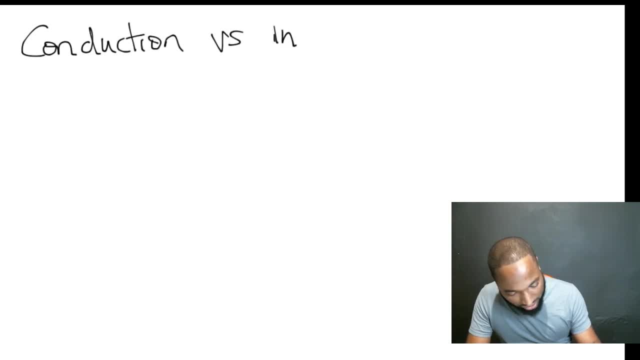 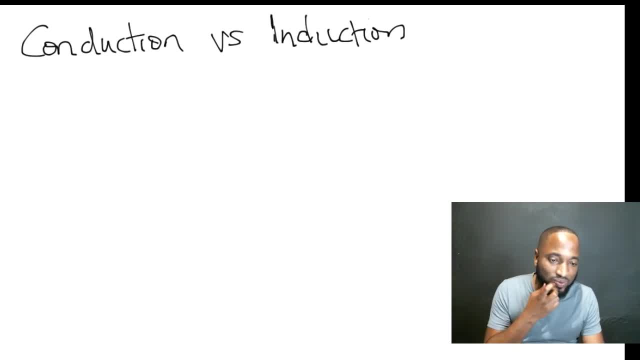 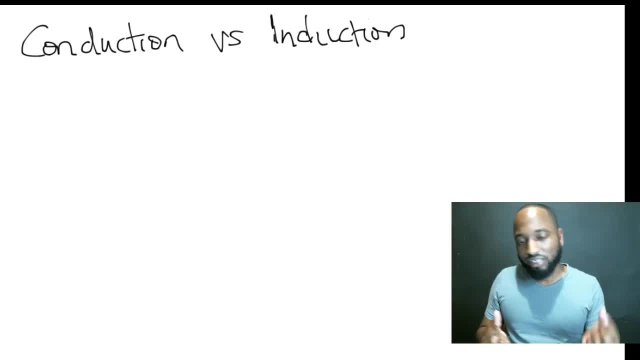 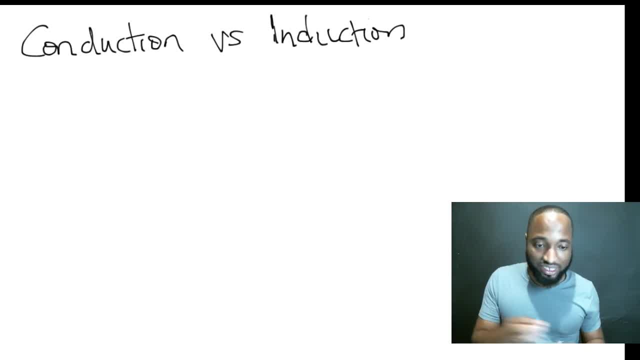 intake as it conducting it. conducting has to do it. conduction, yeah, but we talk about in terms of charge. we're not talking about in terms of heat. remember we any electricity, magnetism here? so the technology induction is when you put a child up. yes, induction happens when you pay any charge of the techniques and 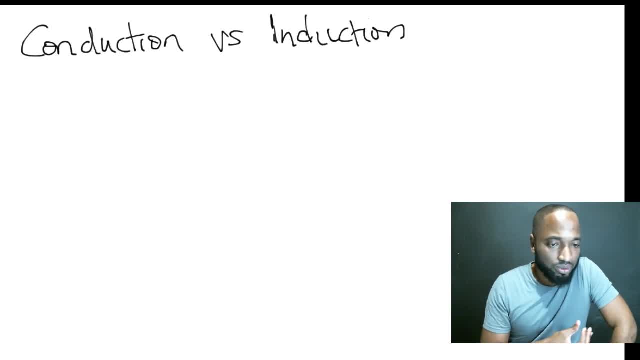 neutral object or something and it induces the charge without touching right. induction means without touching. now I just seen some, I just reading through some answer. one is not like fictional or some, so where induction is, then each other could: yeah, conduction is the transporters charge. yeah, introduction is when Charlie said true. 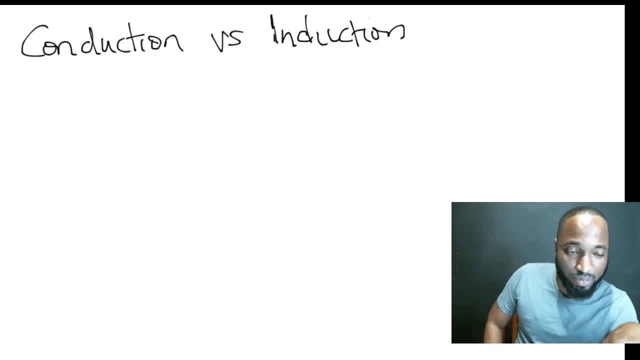 electronic feel from one return. and that's nice, be junking gaming, we are not. we are to something me right. so the conduction has to do it. well, it's touched, so you have to remember it with touching. so touching is happening in the center of the screen. 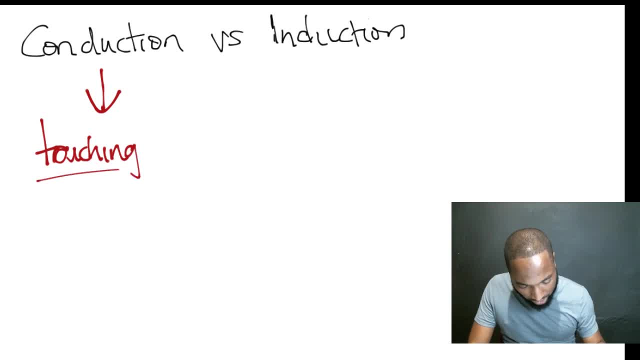 right better, so we actually have touching happening here. that's this means like if you have a charger and I said you are, doesn't negative and you bring it next time, and he can't do it because it's not working, because it's not working right, so the conduction has to do it. well, it's touched, so you have to remember. 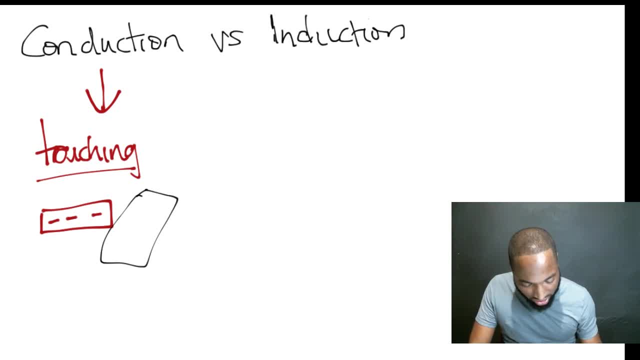 it through the electric field. this is the charge that comes out of the conductor. if we find a conductor, even if this conductor is neutral electrons, the actions are going to be like we and run off into into the object. until it's balanced mundo. there's a balance, remedy charges, turns are considered great. that's conduction, no. 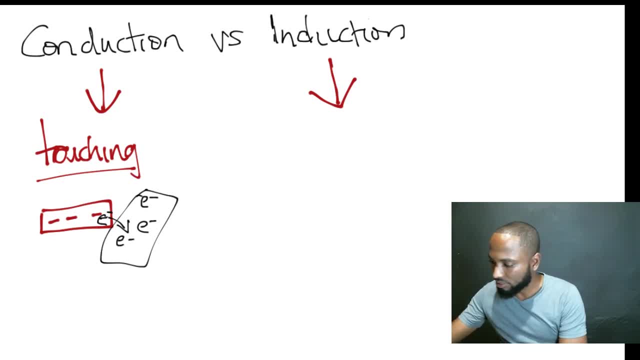 induction. there are a little more trickier to explain. induction happens due magnetic field. right, let's say we have- and I explain this very clearly in the video that I did very clearly in the video that I did before. let's say we have a net amount of negative charge here, so that is like a poly polyteen. 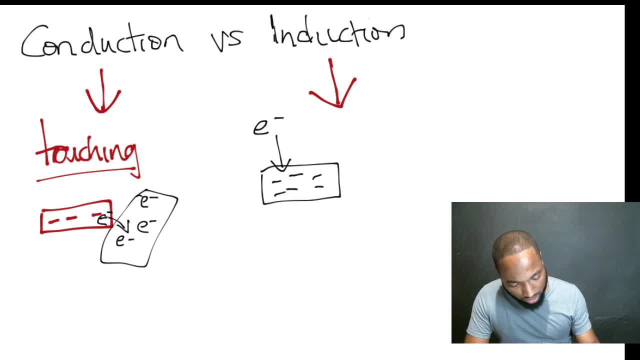 again and we bring that next, a neutral object. let's make a neutral object a rectangle. what happens is all this negative charge here. if we have some negative charges in here, this has to be a conductor. we have some negative charges hearing a lot extra, extra, this, just extra, this negatively charged all. 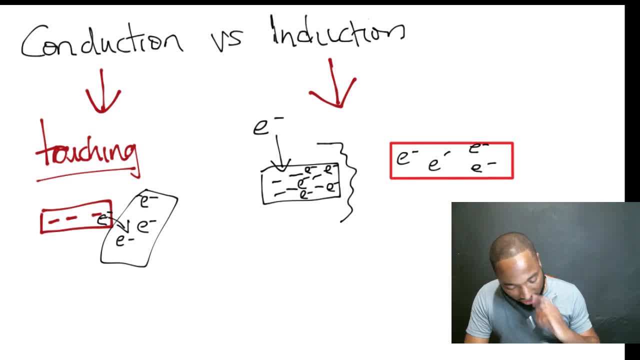 this negativity here is going to cause repulsion of the electrons here you. so all of a sudden these electrons don't want to be on the edge here anymore. it just had too much electrons on the side like, like charges repel, so all these electrons are going to try and pack down here. what will that do? that would make. 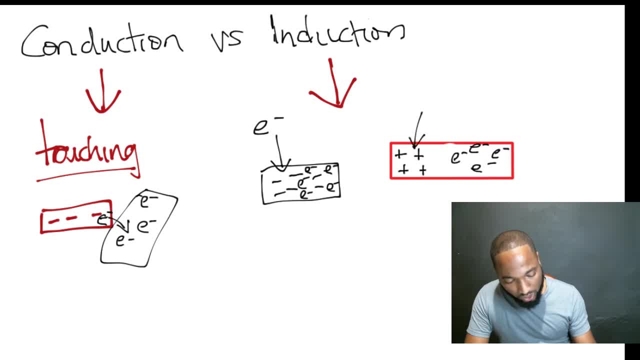 this. that would expose, that would expose the nucleus there, that expose the protons. so there'll be a net negative charge here and a net positive charge here. and now remember this- still negative, this is still negative. so if this is still negative and all the negative charges ran away, 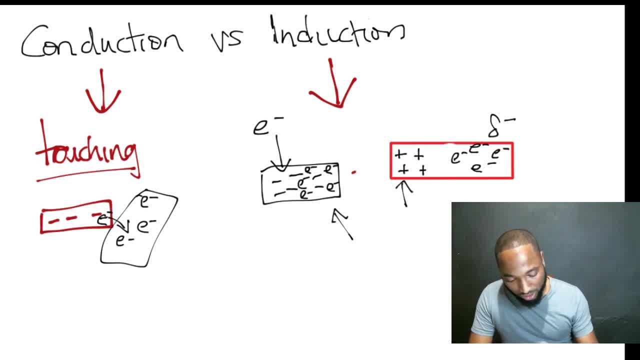 exposing positive charges here. there's going to be attraction and as the whole process of induction and what happens during induction. let me see some wise in the chat, if you could, if you understand conduction and induction, there you wise in the chat. good, good ight, great, great great. now, if this is too smallucktional, be happy too. induction: 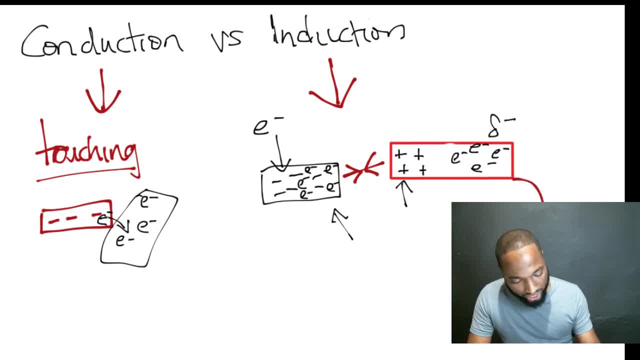 occurs best when the object is grounded. this will mean this will allow the electrons to have space to run away because, remember, just plenty electrons here, they want to runaway. but if the small is too small as to develop an election, but if the small is too small as to have enough space, the like you understand and 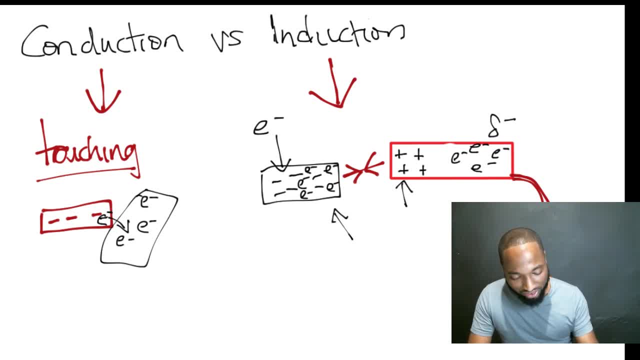 yeah, the runs and Manikin understands parts we can't understand pretty well, because they put intention to think it didn't really know where to run. generally I know where to run, but if it was grounded it would run through the ground and this is the principle of the 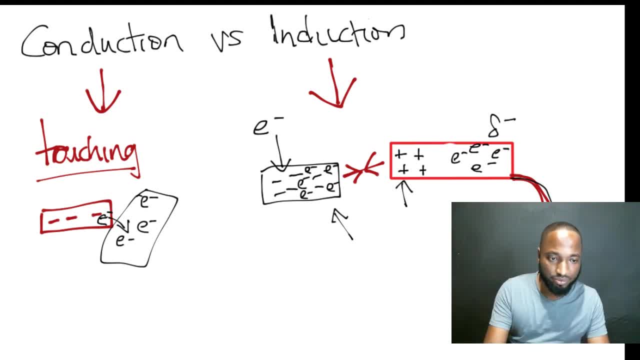 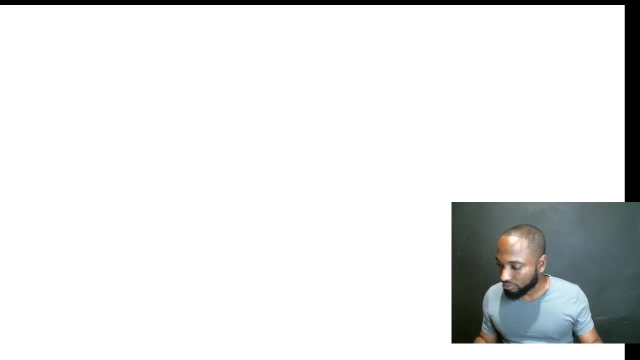 lightning rod right thanks to check your IGBM right in a time. so this brings us to talk about electric fields. so we have to talk about magnetic field sooner or later, but we'll talk about electric fields first. so there's some diagrams to draw. there's the diagram. if you have a positive charge, then there's the diagram. 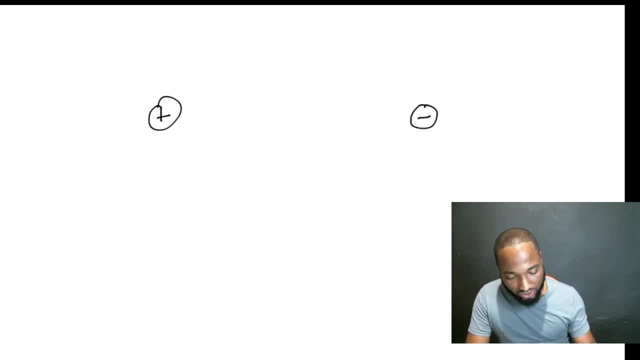 if you have a negative charge. now, these are point charges. let me just draw it back a little better. positive, negative. you draw a little circle around it. it's a point charge. everybody know, everybody know how to draw this diagram. why is in the chat? if you know how to draw this diagram, excuse me. yes, so the positive. 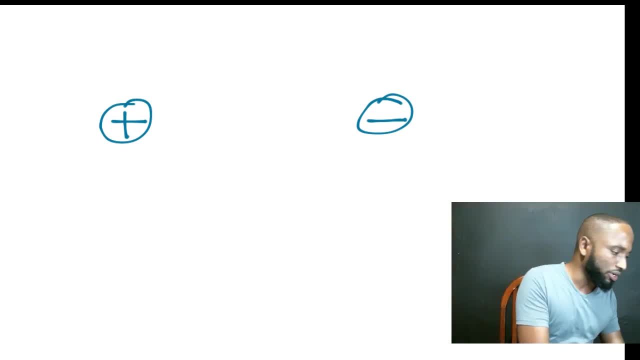 that's not element that's very fine so everybody know how to draw the diagram your home go ahead � Norway we're gonna talk about that s now the positive charge both of them look like this and I were just like one two three four five six seven you know top line in 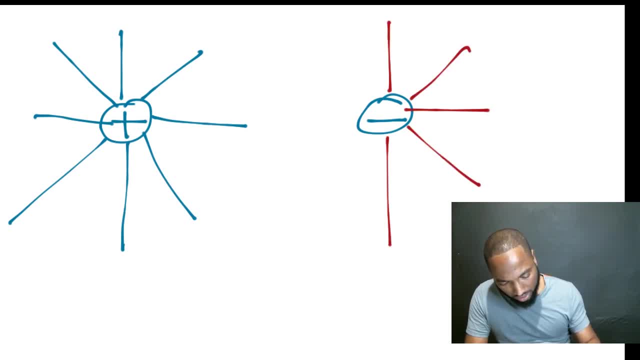 between. yes, alright, this as well, But the direction of the arrows is the key here. If it's a negative charge, we have the electric field going like this. If it's a positive charge, we have the electric field going like this: away from the. 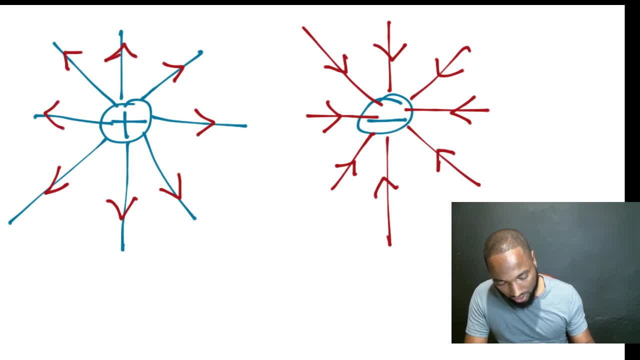 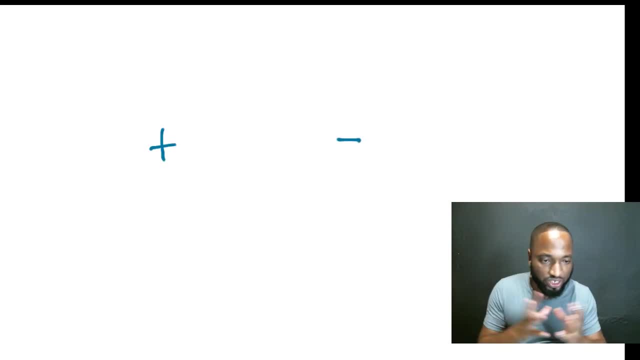 positive charge. That's simple. right Now, if we have a positive charge and a negative charge close to each other, you need to know what happens Before head shining. we move towards the move of opportunity, right, But what happens here? 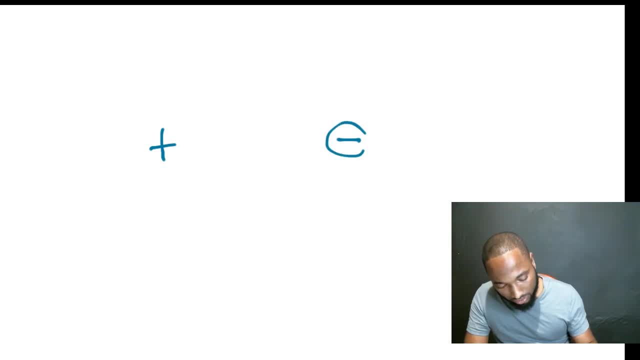 now. Well, draw a little circle around. I will draw one street like this, then the bend, then maybe one like this, one like this. That's what we expect. right, You're getting that through. Everybody catch the idea of this. 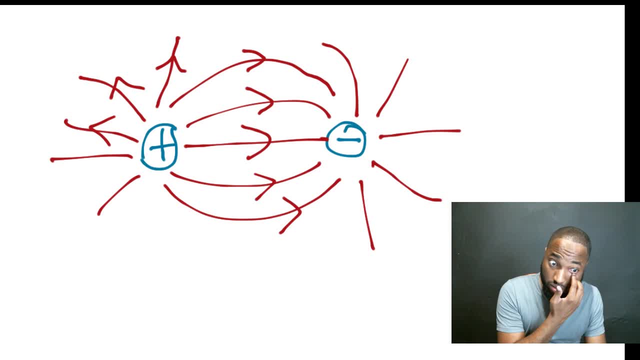 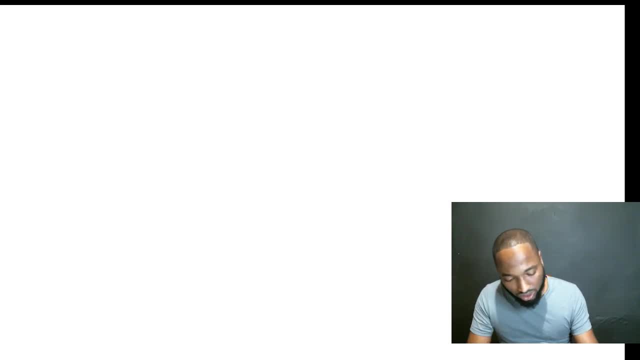 Pick memorization. All you need to know is going from the positive into the negative. Very good, Now the last thing you need to know: Oh, if you have a positive and a positive, what will happen? You're going to get this thing in place, right? 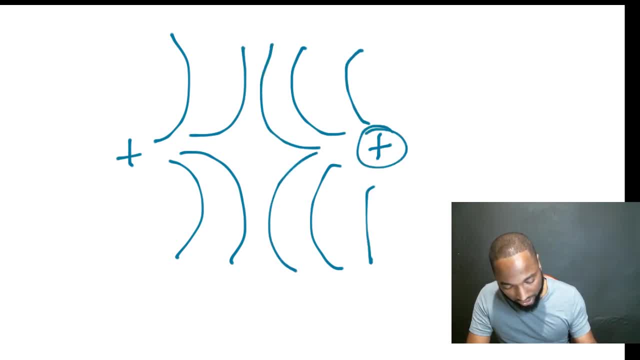 Kind of like this Don't touch me- situation taking place here. It's running away from the positive, but it can't go into that other positive there, so you have that taking place. That's why that diagram is kind of bad. And the last but not least, 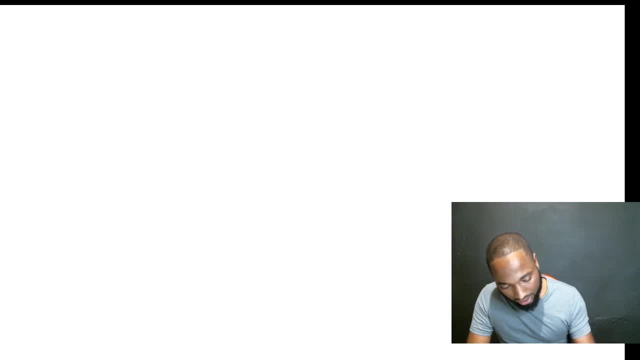 is if you have plates. So the plates are simple. So if you have a plate, you have a positive and negative. positive, positive, something like that. Everybody get taught this right, Everybody get taught this. You draw all in the center street and the ones on the end. you curl it a little bit. 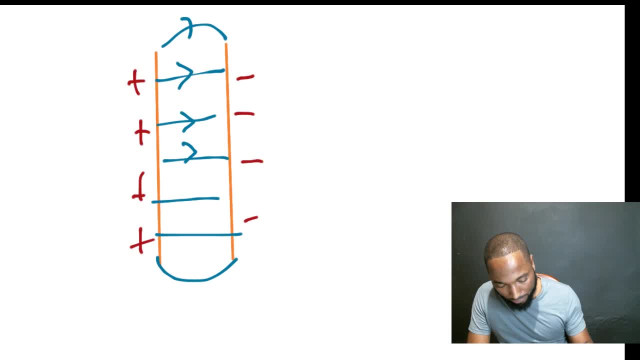 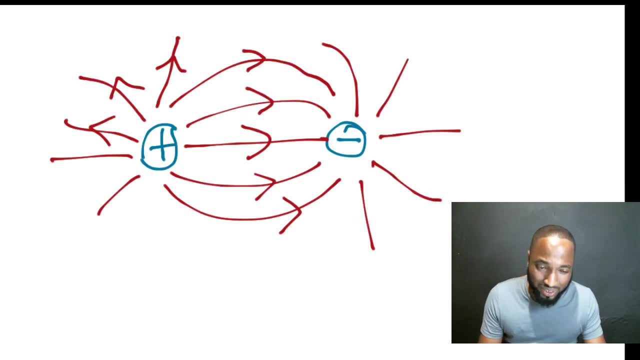 Once again, positive to negative And that's about it for electrostatics. Make sure you know all these diagrams, because they come a lot. They come a lot, As simple and as simple and ridiculously simple they are, They come a lot. 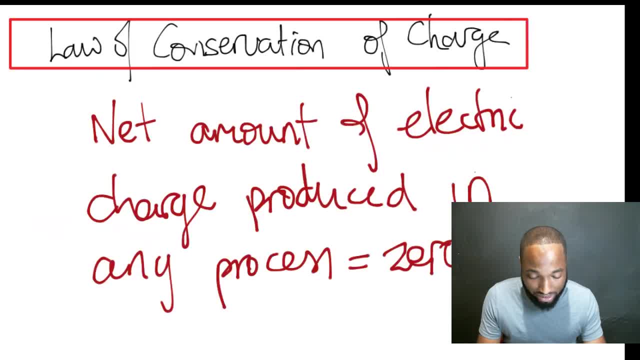 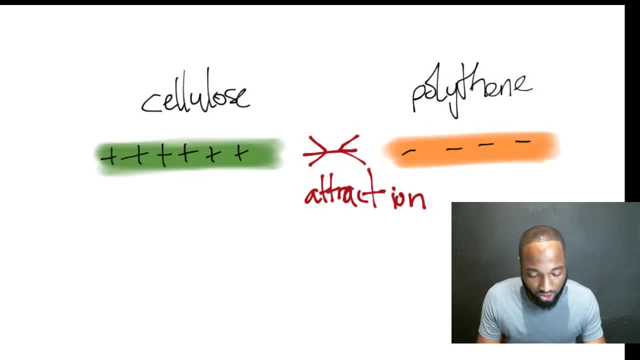 The conduction talking point. Make sure you can explain it. They come a lot. I never see this laws of conservation of charge coming, but who knows, It might drop down on you. Make sure you know about your cellulose and your polythene. 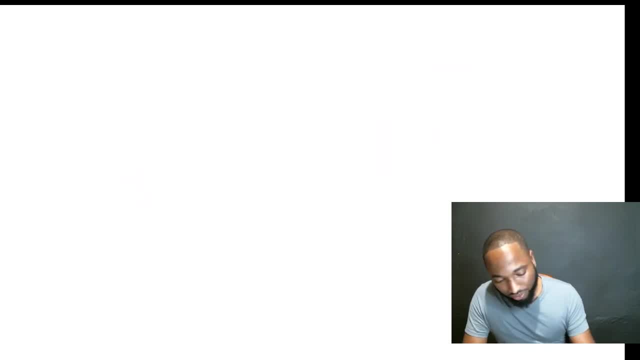 And let's go forward. Next thing you need to know. Next thing you need to know is the hazards. Talk about the hazards. Which part is the sweet part in this pen? Hazards, Hazards of electrostatics. Can somebody tell me the hazards? 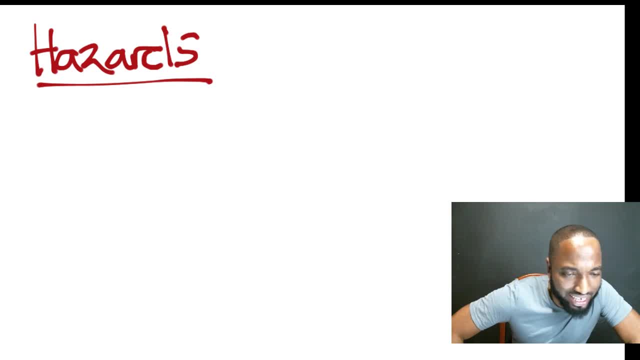 Some people are quarreling in the chat. So that head is, that forehead is a hazard. I see you, bro, I see you, I see you. Right, So we have lightning. Maybe I could put this in another cover. What else people seeing? 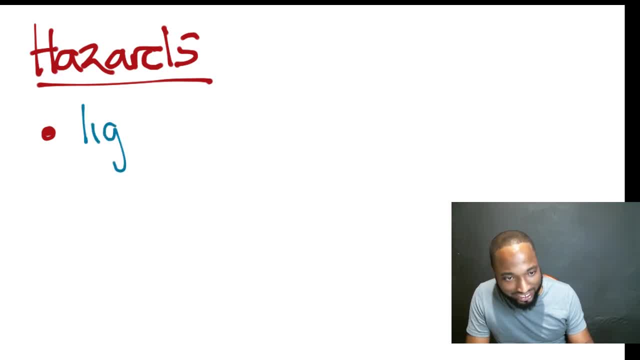 Death lightning. I need you to be specific, Not just death. Be specific with it. Explosions, explosions in flammable environments. So flammable environments- For example, a lot of my jeans, pants- build up static electricity real fast. 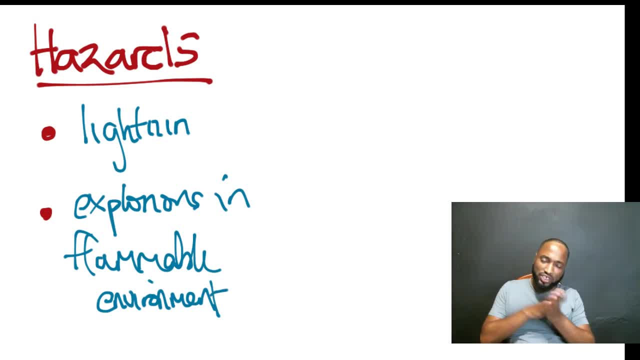 So like if I sit down in a chair and it has cloth, some of the friction on that cloth, when I get up and I touch the door handle, it's like It's an immediate thing. So every time I come out of the car I always make John touch the car before I fall in gas. 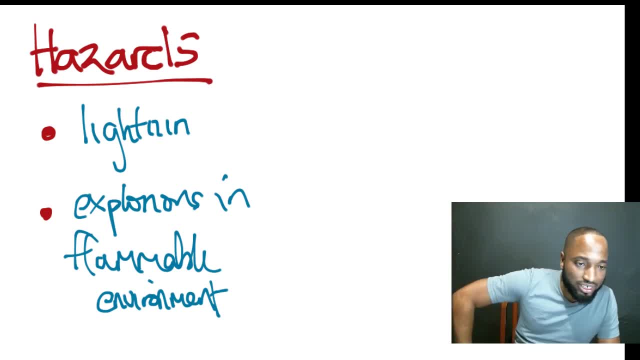 Right, Because then really, what has to happen to me when I fall in gas? Damage to ships, microchips, Sorry, So lightning is the biggest one. I'll give you what you need: Electrocution. We're not talking about problems with electricity. 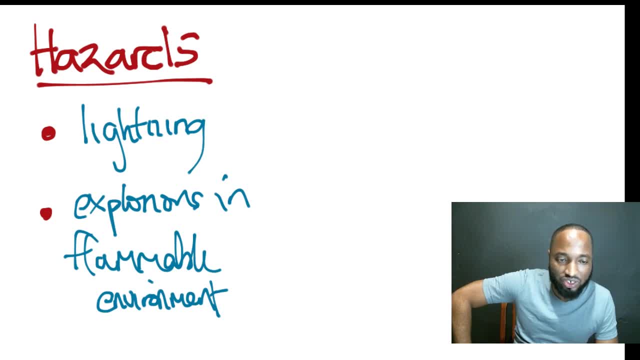 We're talking about problems with static electricity, So you can't really talk about explosions in glass gas stations. Yeah, you can talk about explosions in gas stations, But you can't really talk about electrocuting yourself and them, kind of thing. All right, 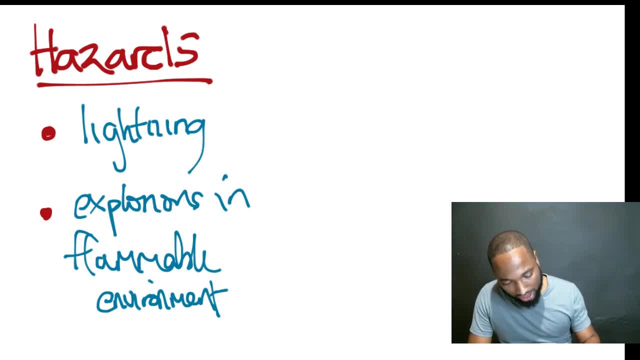 So, and then you need to talk about the applications. So what are the applications? Applications? Okay, So Remember, the lightning strikes, the tallest object. just to talk about lightning. Lightning strikes, the tallest object. It happens when clouds accumulate a large amount of negative charge and they have to discharge it. 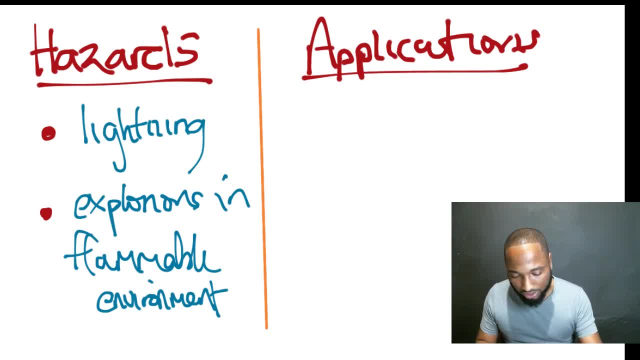 They discharge it in the form of lightning. So a lot of people are mentioning the applications there. You all can have a read at them. We can also talk about static buildup here, which will lead to the same thing. Static buildup: You're going to use that, too when you're explaining this in your exam. 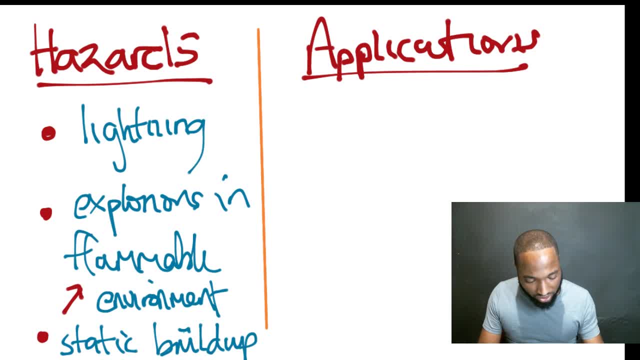 Static buildup of electrons, Maybe in a vehicle, as driving along the highway or on your clothes, Cause a spark in a flammable situation. So applications, So applications. We can say: photocopying, Yes, Photocopying. What else are seeing? 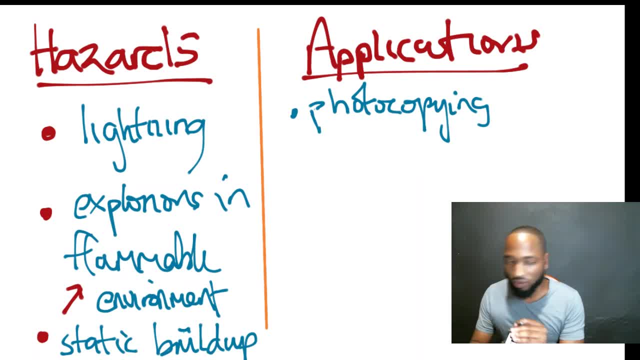 Light lightning rod. Well, you see, lightning rod to avoid. There is something I wanted to see. Where is it? Where is it painted? dust precipitator, right dust precipitator. dust precipitator um crop sparing anything else, yeah, this life gonna be available after lint. 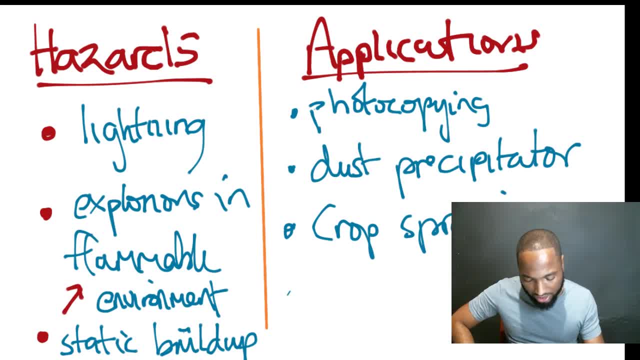 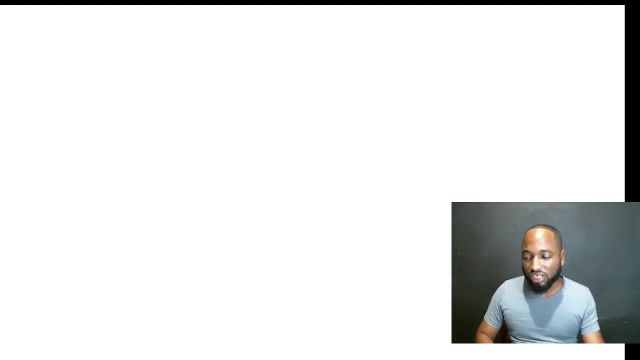 removers, lint removers. I know I'm blocking somebody text they trying to get my pen to lint removers. okay, you're taking that begging painting, right? you taking that so you all know your applications, know how to describe them. to do just know them to see them know how to describe them. y'all please no. 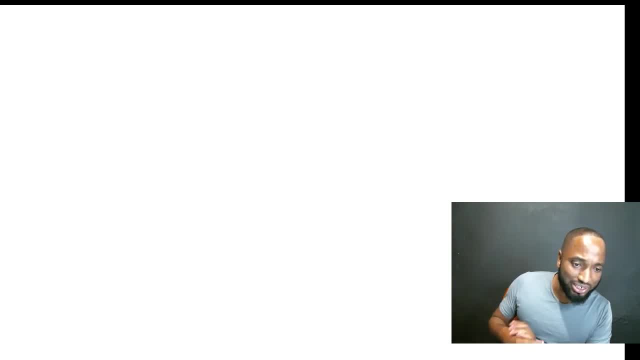 fighting in the chat and I realize I'm watching chat and people calling you. I will do atomic physics sooner or later. so that's the end of electrostatics. let's move on in the current electricity. but before that happens, maybe we can take some questions. could you predict what would happen in 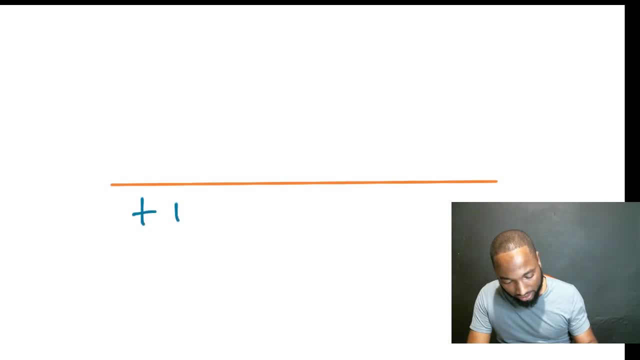 if we have a plate that is positively charged and you have a point negative charge here, can you predict what will happen? write it in the chat. must be able to explain how like lightning works and what are the steps you'll take to remove, reduce the lightning hazard. can you explain lightning? yes, I will explain. 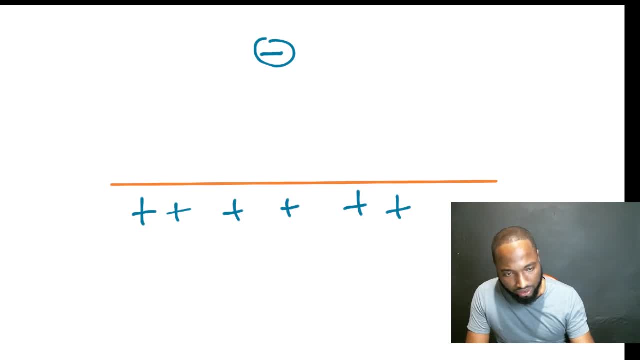 like: No, they would not track. we join the field. we join the field. remember, you can expect something like this: stick in place, which direction is really arable? so the next thing is to explain lightning out. I'll explain lightning and how we get. so the next thing is to explain lightning and how we get. 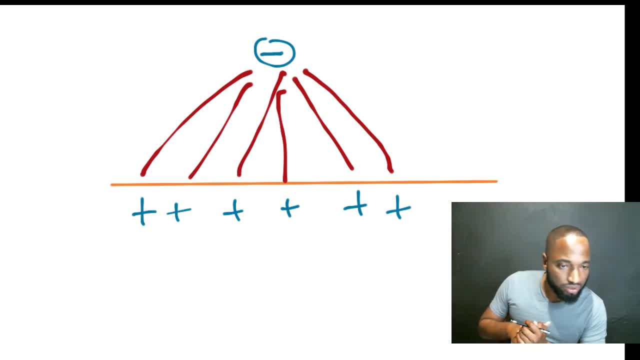 a o right. so this is a person. I just it a way question and nobody. what would happen if so? that is a person. I just it a way question and nobody. what would happen if we have lightning striking a building? we can have fire aim, so to avoid that the 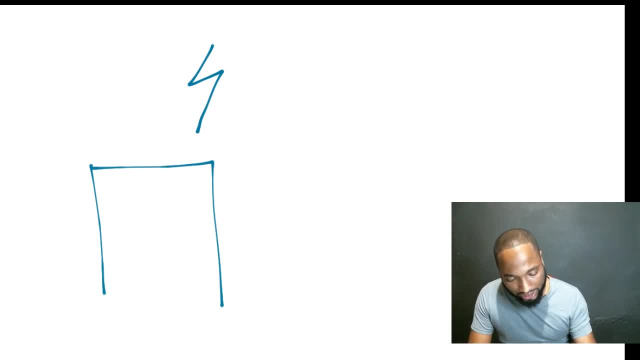 we have lightning striking a building, we can have fire aim. so to avoid that, the is to coloca a, since this would rain a lot of lightning. when it rains, the air in ideal condition is as simple as that. one can catch something right. so to provide the imagination of what forms the smallhop gjort, we had that business state\. 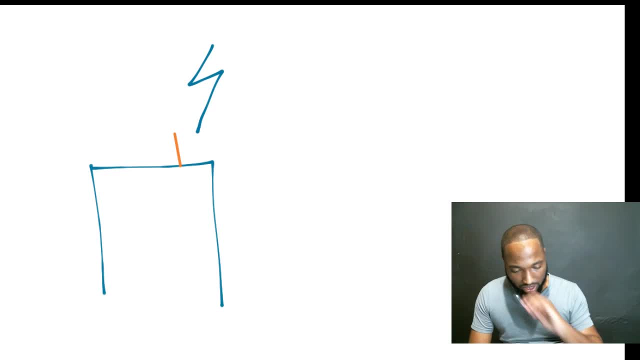 They include a lightning rod. And how does the lightning rod work? The lightning rod works by the principle of induction, Like this: Imagine this is a lightning rod. Let me draw it in orange. This is a lightning rod. As the high negative charge from the lightning comes down right, What's going to happen is going to induce a positive charge here. Now, how is that going to happen? 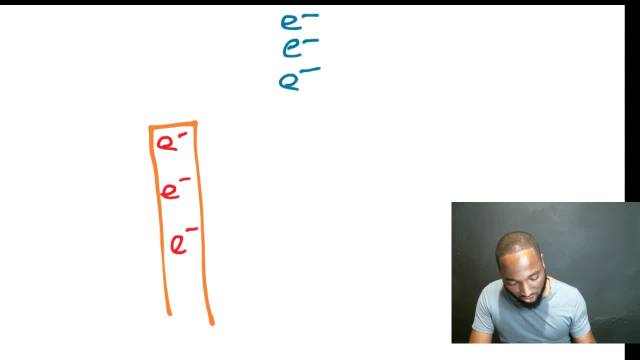 Because this rod was mining. He owned business and had a nice neutral setup. Electrons all over the place. Normal Net density is even with electrons. But as soon as this high presence of negativity come around here in the air, all them electrons go in and dust it And because this runs down to the earth, these electrons will end up hitting here. 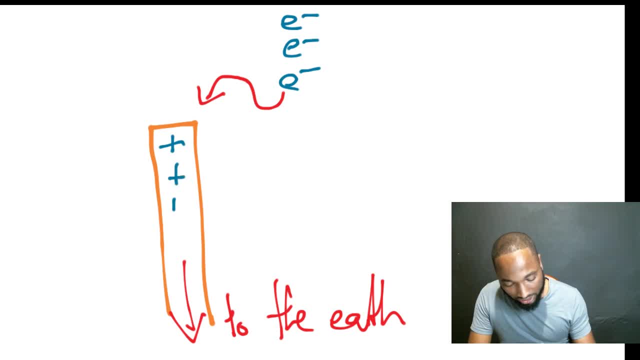 Why will they end up hitting here? Because only positive charges will be here now. Well, not only positive charge, but a high net positive charge, So it's going to actually attract the electrons. So it's like this Induction and explaining all these things work just like this. Listen to this example. 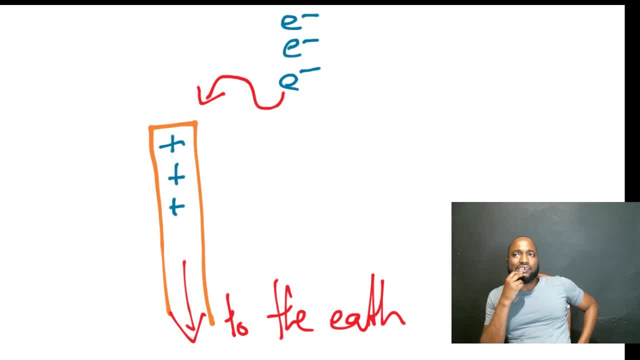 It's like a girl really loves her boy, Really loves him, But he doesn't love her. He doesn't love her, So he kind of okay. Let me not explain it from the girl perspective. Let me just make the girl not liking the boy. 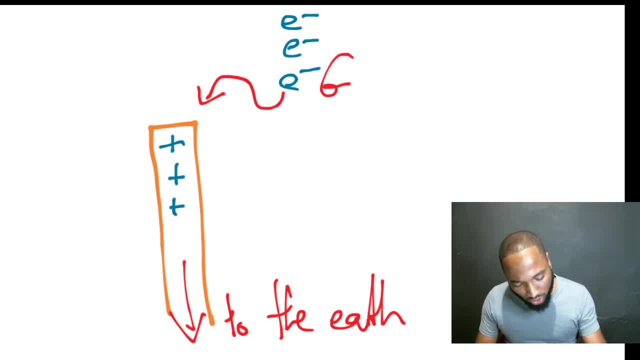 This is the girl here. She doesn't like the boy. She's going along his way, Her way. But because she is not paying the boy any attention, he actually opens up to her. And now that he opens up to her, they get accepted. right, They get accepted. So there's a principle that's going on here, because the negative charges actually cause their own attraction. 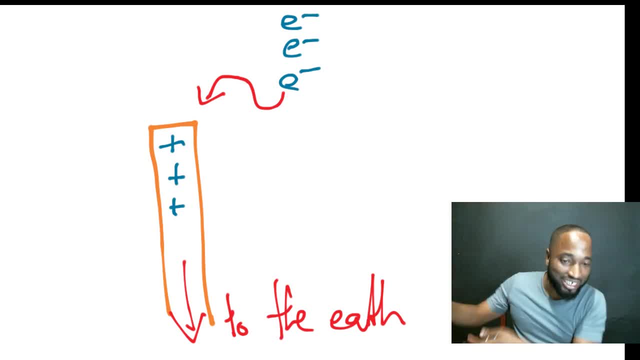 These negative charges are responsible for everything. They chase the electrons away in the lightning rod and all of a sudden there's only positive electrons there, BAM. so they attracted to them. you have a girlfriend. best deal come out. she chased away a girlfriend and are you expected to see something? so something. 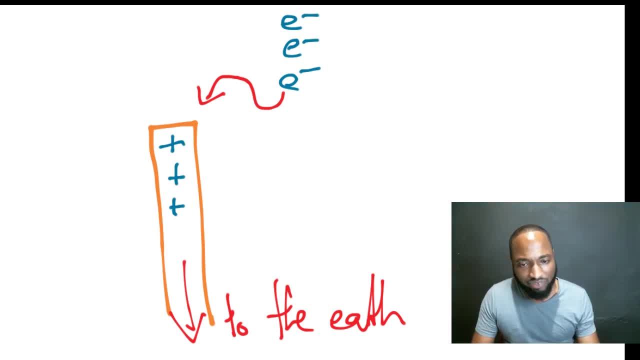 so we know that is induction, induction process. so that is it for explaining lightning and lightning rods. also know how lightning forms like. it has got a research on that. you are something similar I today in class here so a lot of teachers makes explained using that that. so that's gone in the current 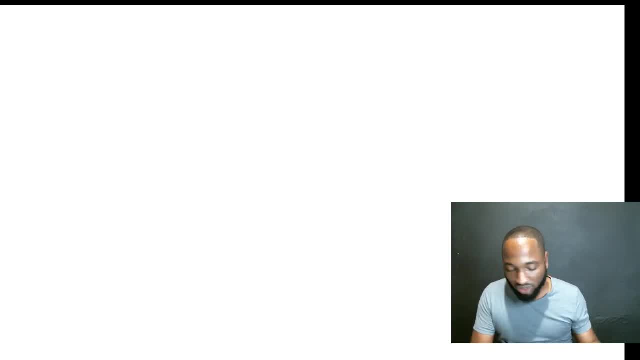 electricity, so current is actual flow in the wire all the time. you're so much static. electricity meaning static means not moving right, but if as soon as you start to talk about flow in a conductor, the net movement of electrons in a conductor, this is something of some ridiculous comments. as soon as we 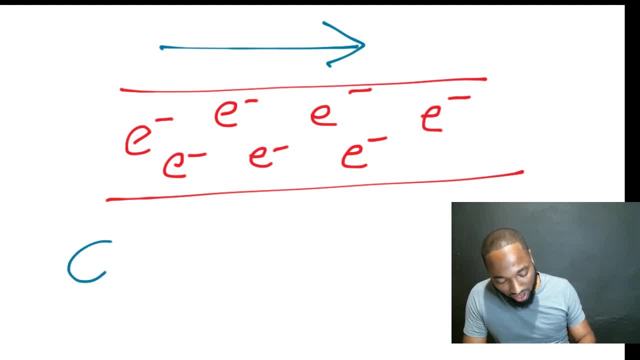 started talk about the flow of elections, you start to talk about current electricity. what unit do we measure current in? what unit do we measure current in? yes, so we measure current in amperes. amps, amperes, I'm for sure right. all right, so a definition for current. 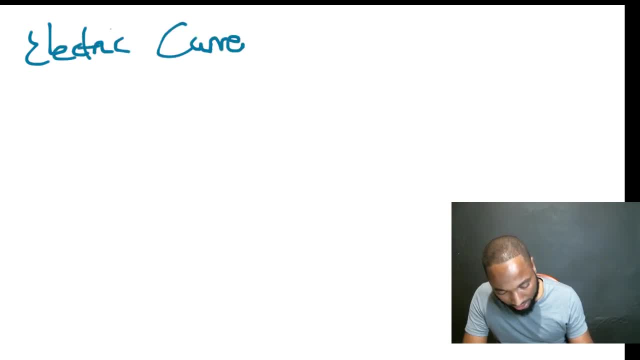 definition few electric current, the masala in your back pocket. are we getting definition for current, please? definition for current in your chat next up we need to talk about the tests for a conductor or in line with the test. hey, in in euro in the implementation matrix. okay, go Gater, we go over and let's start a god, you have word that we can see. let's start a to officer. I talked about some key principles, kind of Loki Indicator here we have to open. I have to stop my browser and stop it there. GATER, you have to stop your browser manual. you are covering some options, not good job. I'm now. 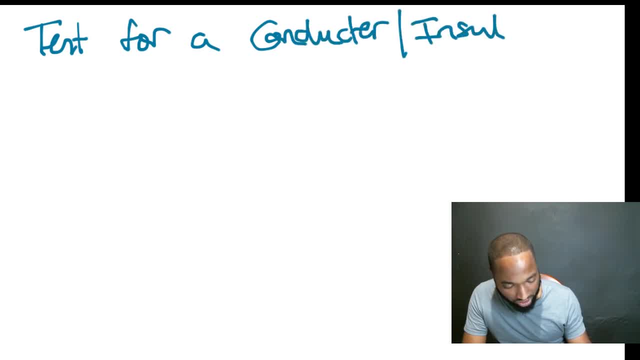 I help you all set up, like: how do you categorize which device and where we have? okay, and the nice thing is they need congress with you. private solution to test to see something in a conductor insulator, a simple circuit. we could set up the flow of electrons here as the moment of electrons in a conductive 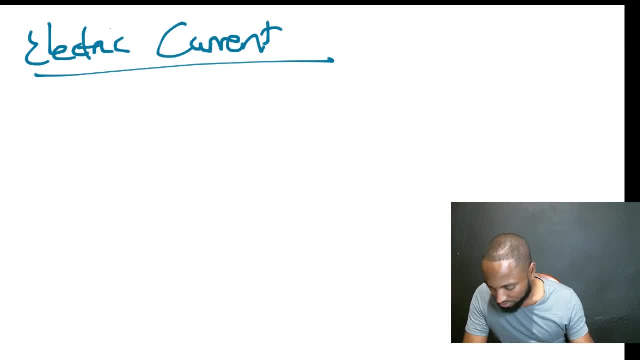 material. that's good, right. so if you want to be a little better about it, you wouldn't use the flow of electrons here, say electric charge, because sometimes current could happen. with all the flow of electrons, right, you could still get current passing through and electrons directly moving, like maybe ions moving. 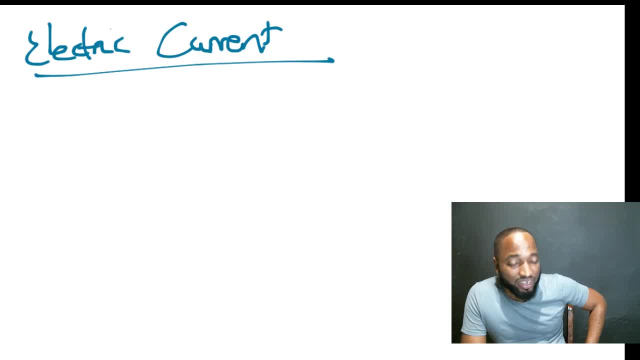 or maybe java diode or something going on there, right, so you let your current net flow and that flow with someone net. now, I made a mistake there, since, since electric current, remember the equation we know from before: Q equal I T and I remember this. I remember this equation. 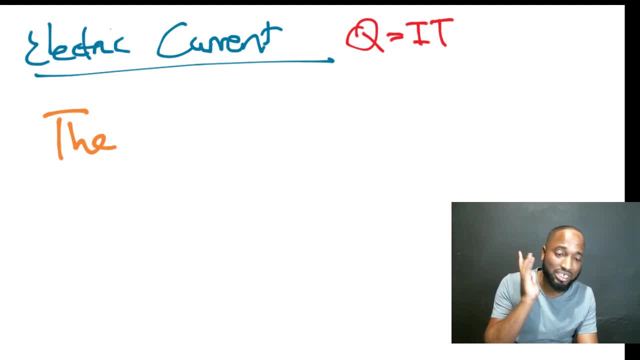 by the word quit or something like that. I don't know, it's just sticking my line: I quit, so I don't know if that'll help anybody. so and Q equal I T. so if I make ID subject of your formula, it's gonna be: I is equal to Q over T, so current is charge over time, right? so 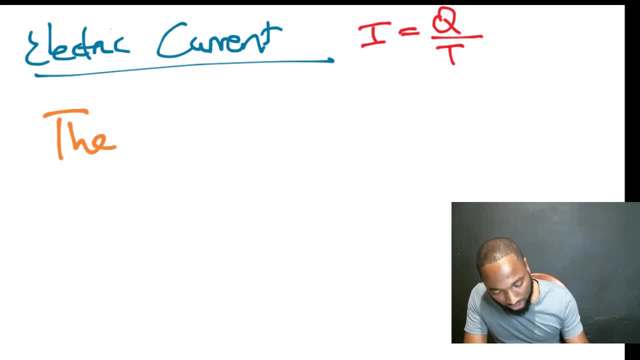 when I use over time. that's rate. so that's this would be. rate of flow is what I should say the rate of flow of electric charge. so rate of flow of electric charge charge flow per second: yes, so you want to use this with rate when you're defining current rate of flow and 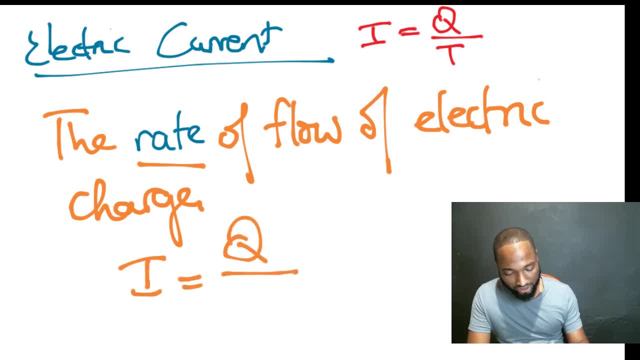 then you put this equation: I equal Q over T, right? so current is V over R. yeah, but we don't. we enrich V over R. so you finally find out what was going on. let's chance, here you can yeah, yeah, yeah, right, so let's keep going, let's keep. 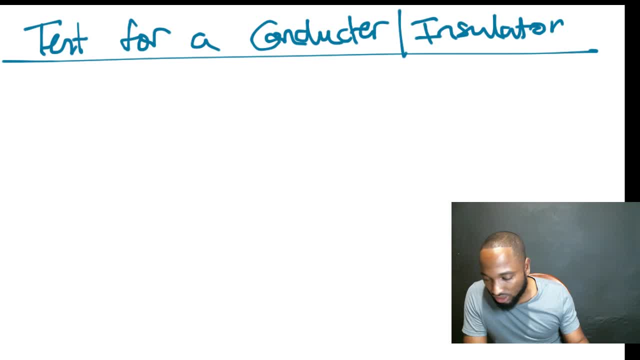 going. we have a lot to cover the test for a conductor or insulator. I want to set up this simple circuit here. you want to set up this circuit. bam bam, bam right. which side of the battery is the positive side? which side of the battery here represents the positive? 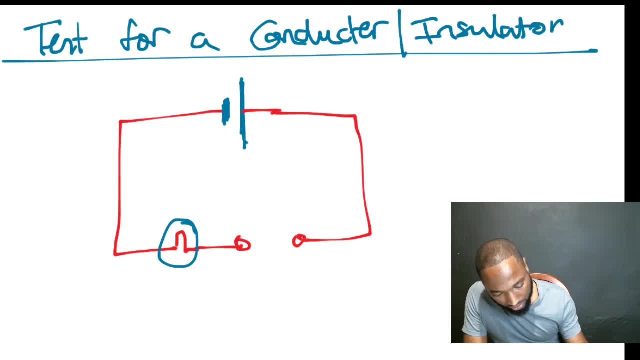 side inside of the battery represents the positive side, the long side right. so the long side is the positive side. so I put positive here, negative here. so you see that green are already. green are pointing you're inserting your object here. when you insert that object there, when I say if it's a conductor, what you 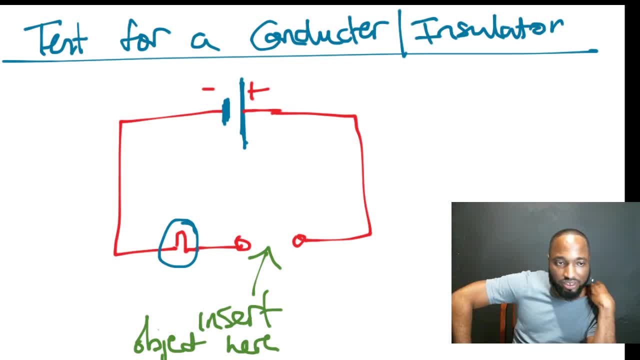 expect to see happening if it's a conductor? if it's a conductor, what do you expect to see happening? and if it's a in insulator, what would you see happening? so this is how you'll test for a conductor or insulator. you set up this circuit, your apparatus. what is this? by the way, this is a bulb, right, so there's a. 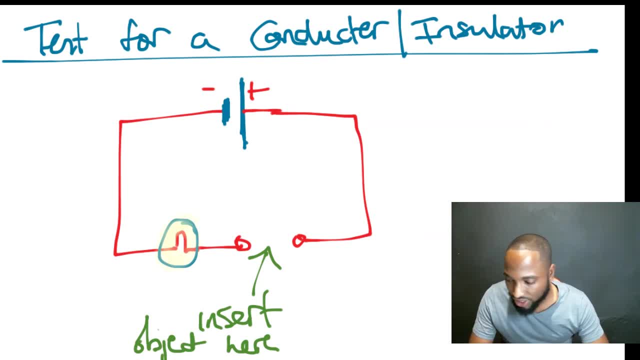 bulb. there you have your battery and you have your connecting wires. so the bulb will light if it's a conductor and the bulb will not light if it's a non-conductor. you need to be able to test it. sometimes test it with a coin, metal, paper clip, a piece of 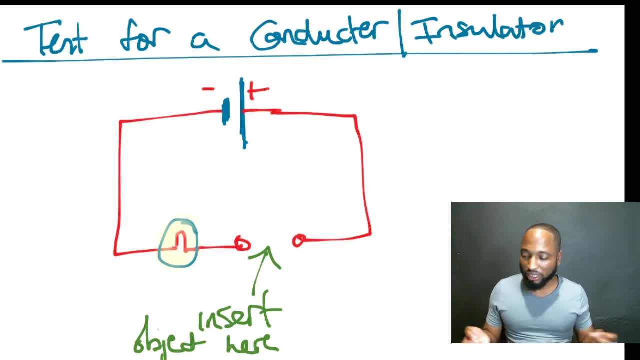 paper, aluminium, foil, and see which metal, which metal conducts, which metal does not conduct, which which object conducts some. some objects may be metallic and not conduct, or may appear For me. I pay Metallica, not conductors, Current in my things. ding ding ding. 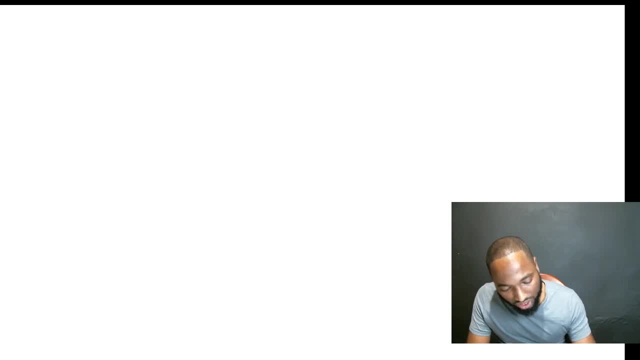 Why are metals such good conductors? Why are metals great conductors? Answers in the chat. Presence of free elections. Somebody, I think we have some tools. we have some tools Because they have free elections right. Presence of free elections. 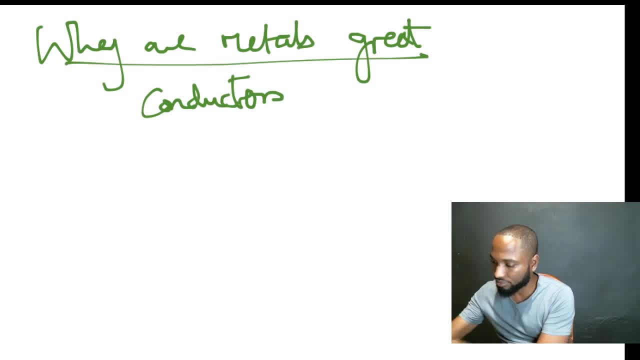 So you understand that. Should I move on to talk about that now, boy? Should I move on to talk about that now, boys? Boys Was the topic current, So we're still talking about current here. Alright, so I'm going to make the big explanation. 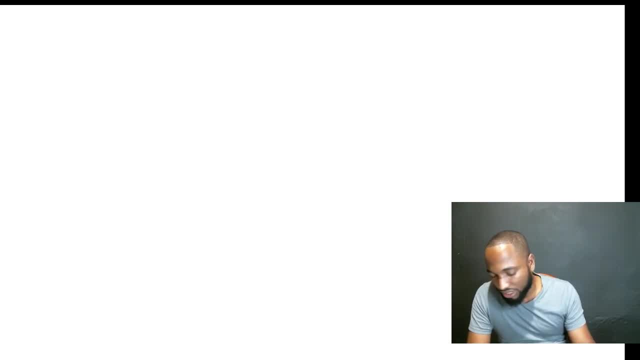 of how current really works. Not yet, not yet, not yet. So current current can flow in a conductor. What else? What are some other ways current can flow? Water inductor, solenoid, air, Electrolyte is what I'm looking for. 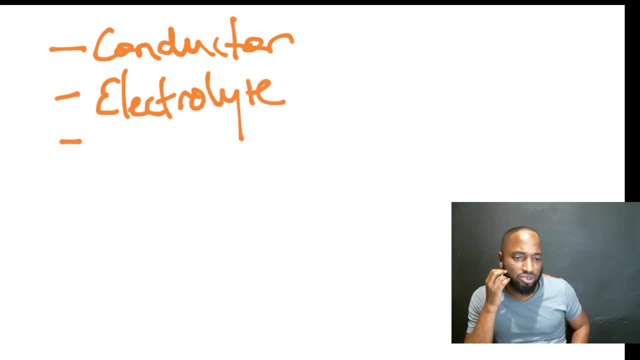 Or so ionic solution, so electrolyte, Or so when you say air or water, Yeah, water, Water is good, but water is a conductor. You know that's already covered here, right? So specifically water will be like a conductor. 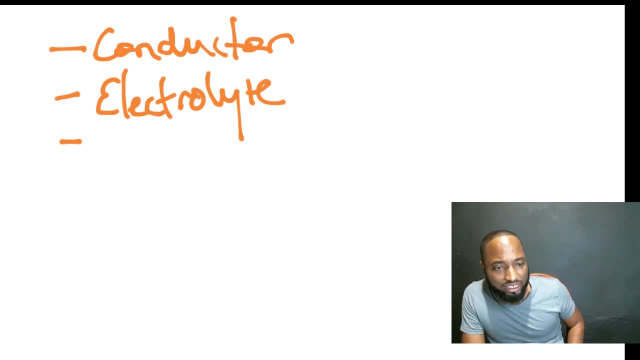 Not convection, Why you talk people only mentioning things for heat. That's heat. We're not dealing with heat. Where's the next? where's the last one? Semiconductor, Semiconductor, Semiconductor, Semiconductor, Semiconductor, Semiconductor, Semiconductor. 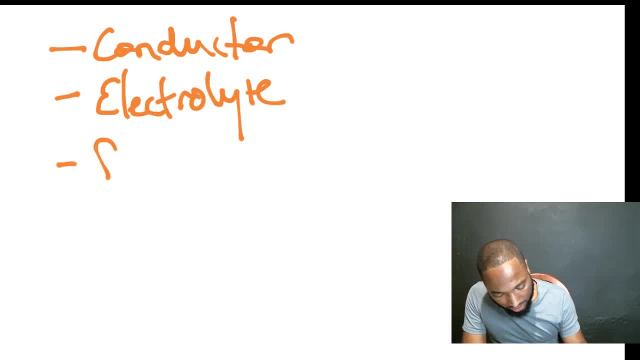 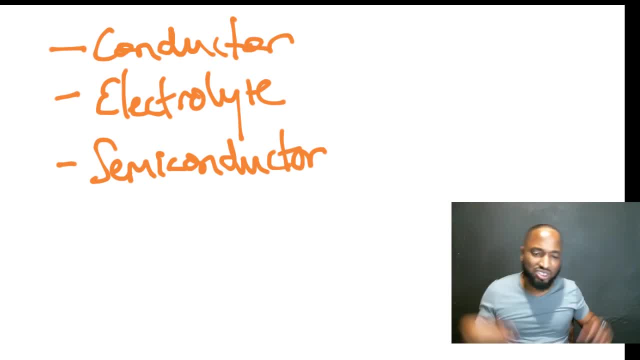 I don't think you need to know about in-depth, in-depth workings of a semiconductor. All you need to know about it is that you have poles. Positive poles are electrons. Positive poles are electrons. see all, I see all, oh my gosh- positive holes and negative electrons and some. 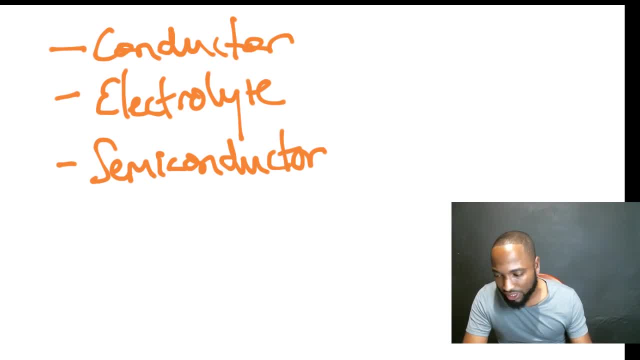 examples of the semiconducting material. give me the examples of the semiconducting material. chat and electrolytes is ionic solution and conductors will be like metals and graphite and stuff like that right- silicon and germanium. one of them will have an extra positive spot. one of them. 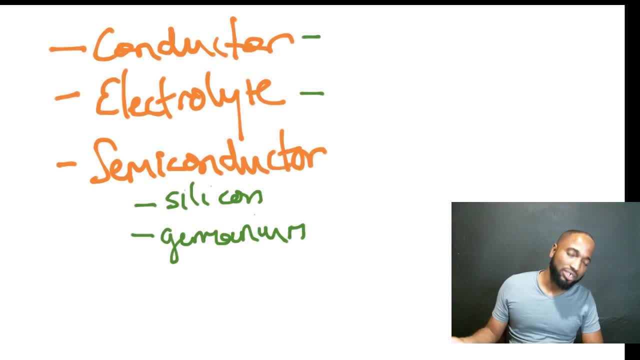 will have an extra. you dope it to have an extra negative and it will kind of hop positive spots kind of hop, all right. so we wouldn't, we wouldn't. I wouldn't wait to the explanation of that. I feel that I see that in your syllabus. so angry into that, right, if he doesn't keep me. 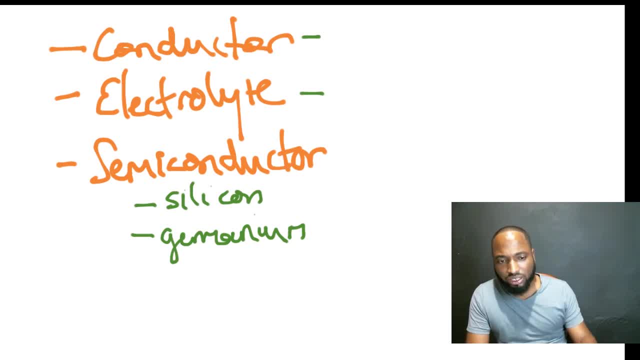 that probably into that. currently in electrolytes you can just take a little watch, maybe on YouTube or as watch a video of the semiconductor a to set two minute video and just watch it. see how it works. nice it's, you have it in your mind. you never did doping. doping is any. 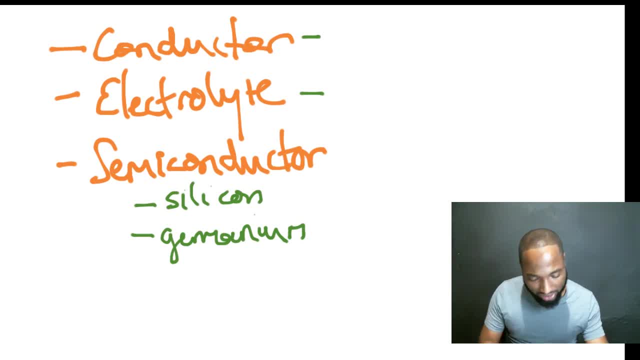 syllabus. you, all of us, never give my little second right, this wasn't up. more doping, all right. so what I mean years? I'm looking for you, the actual magnetism. then I would look to see current and see if you need to know about doping, doping, doping. anybody was taught doping in school, right it is. 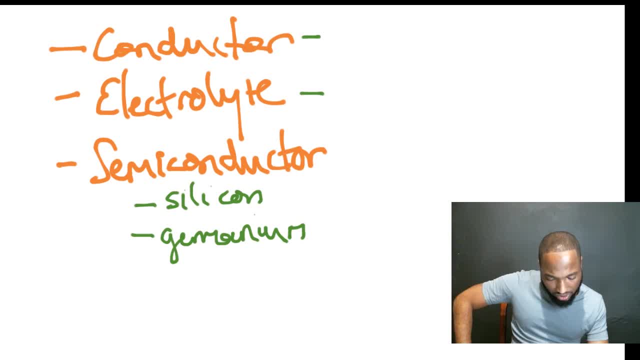 as I saw it, you just need to just need to know about it. you don't need to talk about doping, doping, you know? right, I'm in the syllabus. I'm not seeing anything with doping. the word isn't mentioned. here's what they meant to mention: state that an 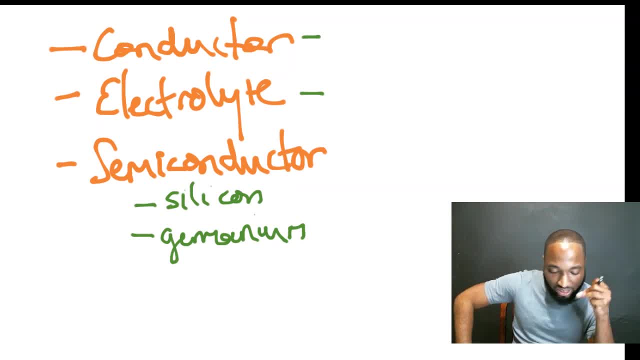 electric current in a metal consists of before elections, and they need to talk about other conducting media, such as electrolytes and such as semiconductors. and you need to know silicon and germanium are semiconductors. right, that's about it. they don't need to. you don't need to know the inner workings of 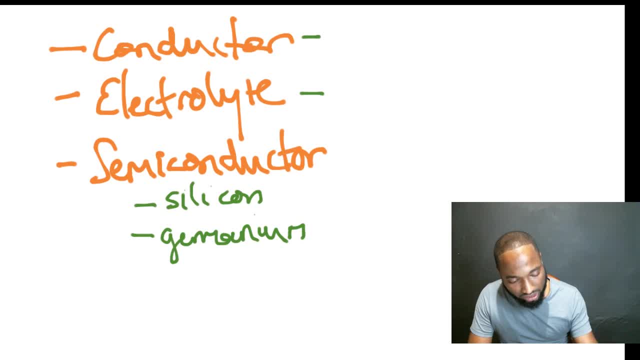 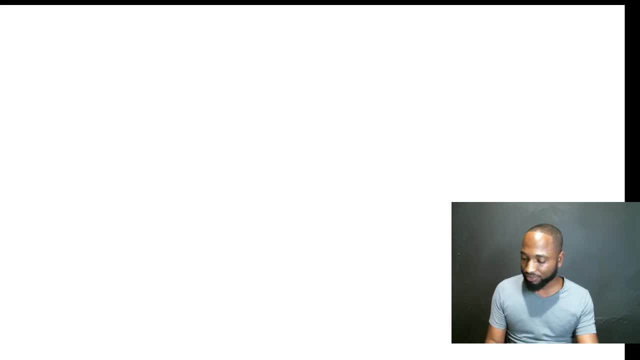 that not yet. but you, physics in, keep we get up water. I can be Kenny next set. so same thing in electrolytes. we know about electrolytes already now. election: I just explained to you that current is the flow of electrons, right. so if the electrons are going this, we've been, the current is flowing that way. but this is in, this is. 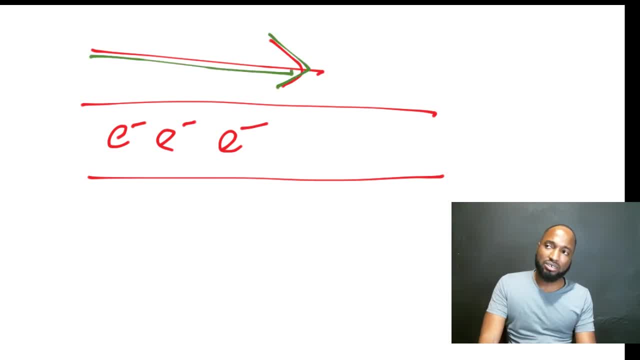 the flow of the negative charge back in the days you know, and they didn't really, you know, they didn't really care about the current flow in that way, but this is in. this is the flow of negative charge back in the days you know. I didn't really, they didn't really. 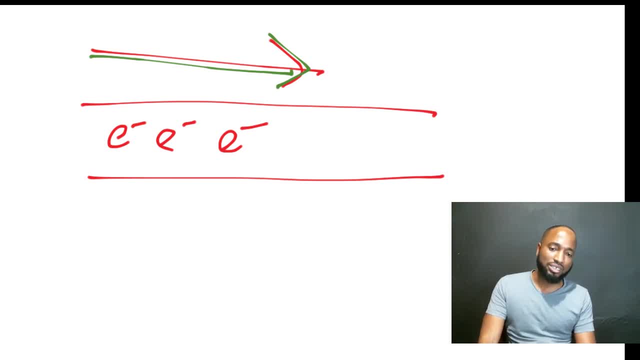 think that the current arose out of positive charges and there was really no way for them to get that yet. So they actually thought the current was flowing this way and that it was positive charges flowing this way, And it now makes sense if there's a net negative movement. 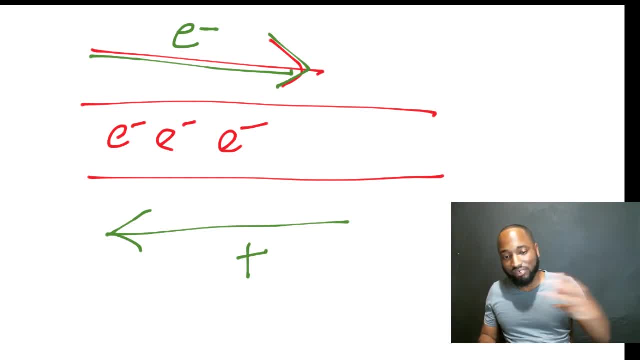 this way, then it means there's a net positive movement this way, so they would be in the galvanometers and everything would be indicating that. So this here is called electron current, and what's the other type of current called The old-fashioned current? What is it called, The one that they use? 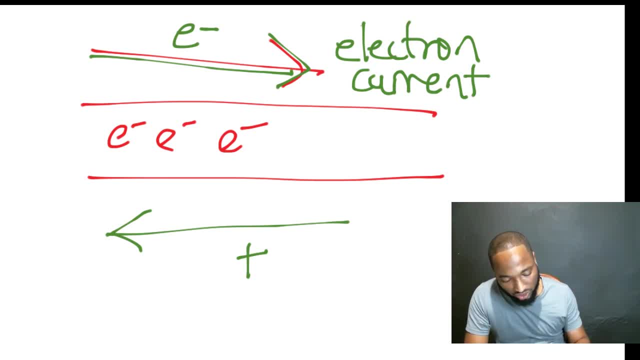 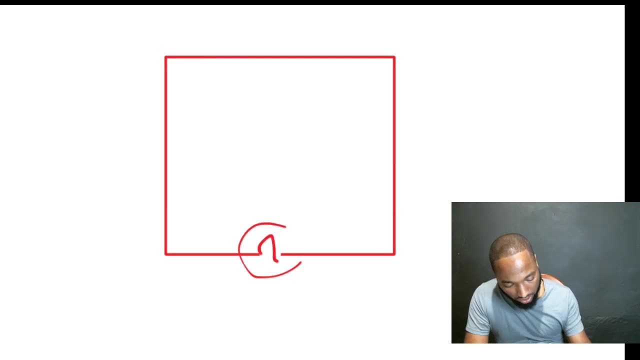 Conventional current is the opposite of electrical, So this is conventional current. So if they act here, if they actually draw a circuit, bam, let's just see, we have a little bulb there, that's all. and let's say, they put in a double battery here, bam, bam, bam, bam. well, you know, that's the positive side, that's the negative side. and they 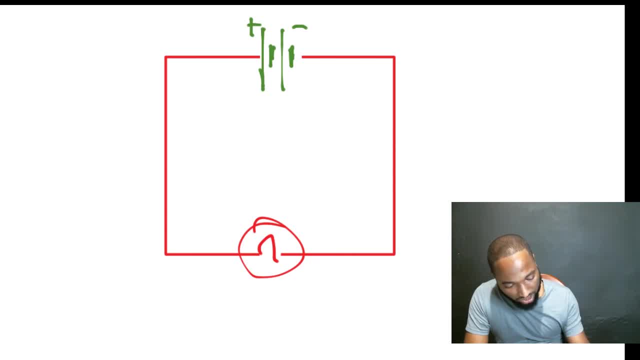 draw two arrows. they draw one arrow- well, they won't put colors, but they draw an iron black and they draw an arrow. so, when they act, which one represents the flow of positive charge, um electron, electron current, and which one represents conventional current, conventional, which one is conventional current, which one is electric electron current? 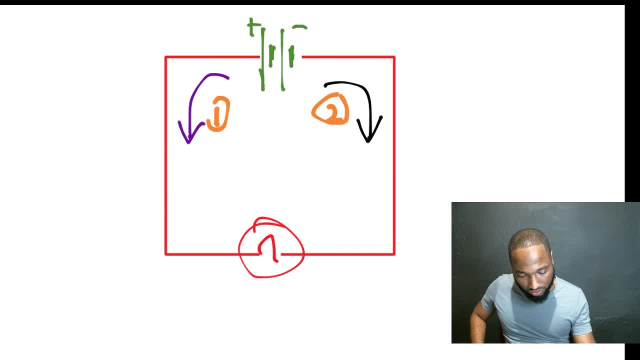 i can put them in numbers if you want one, two, right? so whoa, we're getting different and they'll come to agreement. which one is conventional is is purple and black, right? so one is conventional and two is electric. So the conventional current runs from the positive side because remember the flow of positive charges. 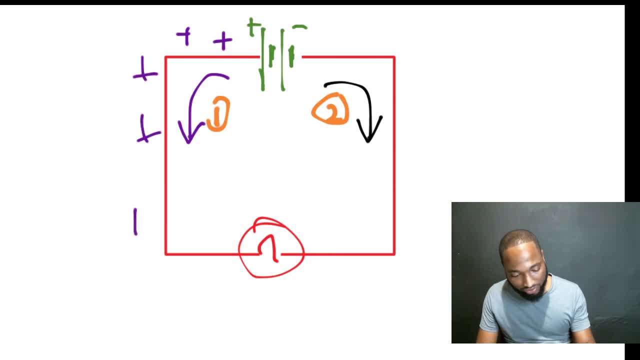 so it didn't go on a b day. you can run away from the positive- this is positive- and run into the negative. that is the conventional current, the electron current or the real way, how current flows. it will run out in negative and run towards the positives. good, so we understand that, right. don't make no mistakes with that. 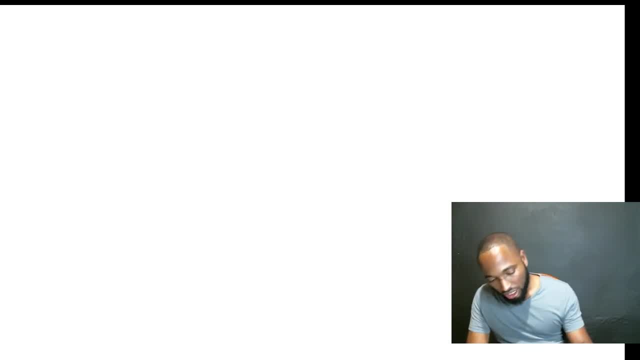 now there are different styles of current. let's just do a little quick current question- what? but there's different types of current in two, with ac and bc. so explaining cndc. why is that right of this question? explain ac and dc in chatwise and write. 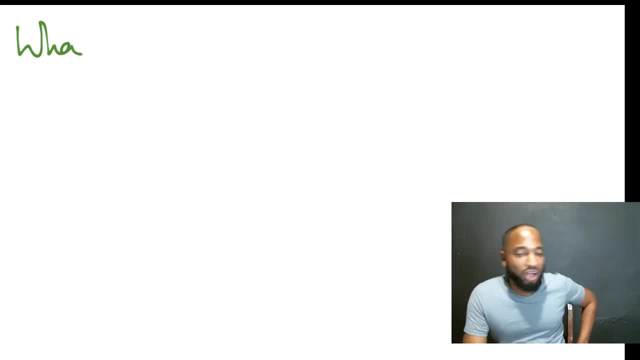 up this question. don't forget to press light in the life now. we don't have a. we have a kind of panic vibes tonight because exams is 90 morning, right, so it's a kind of cool chill back line, but a lot of people will be watching. 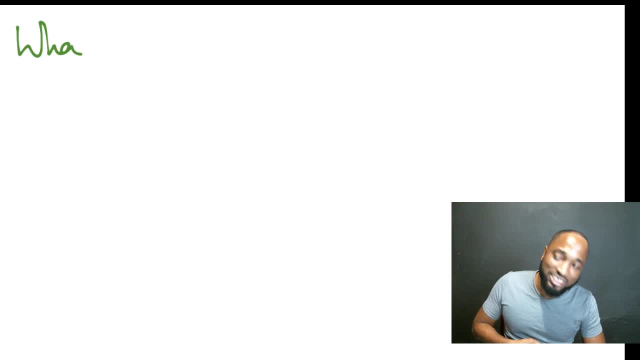 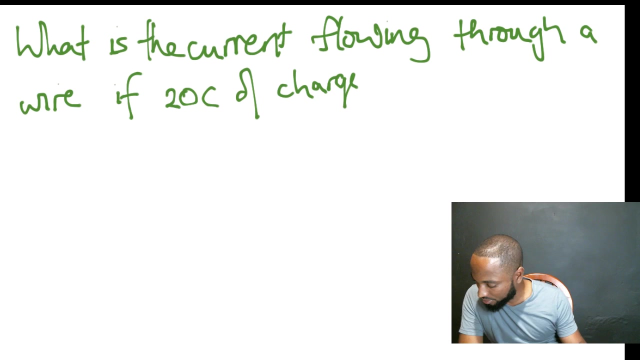 this on the exam, because I'm sure a lot of people probably turn on this live and say, nah, a hot time and start to procrastinate anyhow. so we going request so we explain in alternating and direct currently he why, why? yeah, when two teams are charged as a lot of things, man passes through the past. 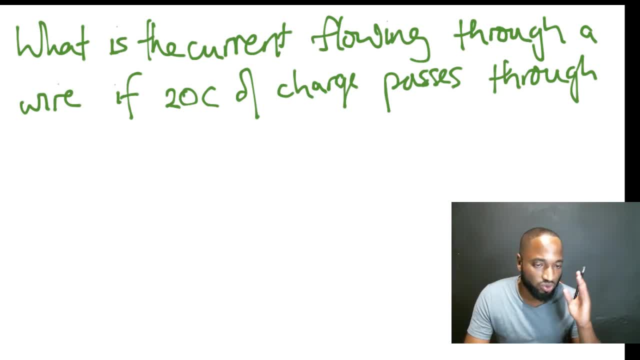 there's something: AC passes a point of passage to the cross-section of the wire every day. hi the answer to that, answer for that in the chat and yes, direct current- one direction, alternate current- different right. so the answer is very easy. now, in physics you always want to start off with your equation. now it's not up with. 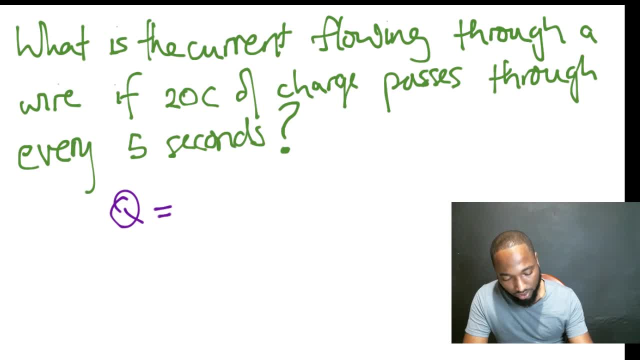 this, because that's really one equation, and then rearrange it into this here and what we learned from our computer alittle. there's a pretty good data. now that I've got this idea to take a little bit of it out. the data sure one, the leading for terms- that it should be right. the value of it is. 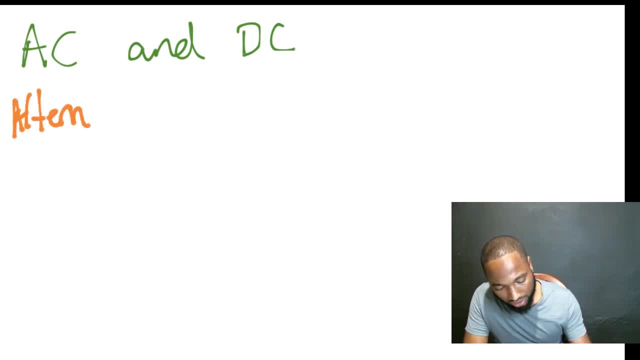 is eight to nine times four, doing number, and eight times three, and then five is And one stands up direct Back in the days Edison and the boys wanted to do direct right through and it's Tesla and the guys wanted to do alternating. 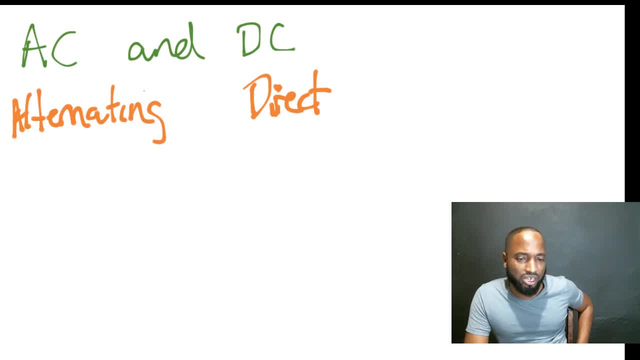 and there's a big quarrel there and Edison tried to discredit the man and thing. Alternating current is the flow of electrons that change its direction randomly- Not randomly really- And direct current is the consistent flow that moves in one direction. by the way, 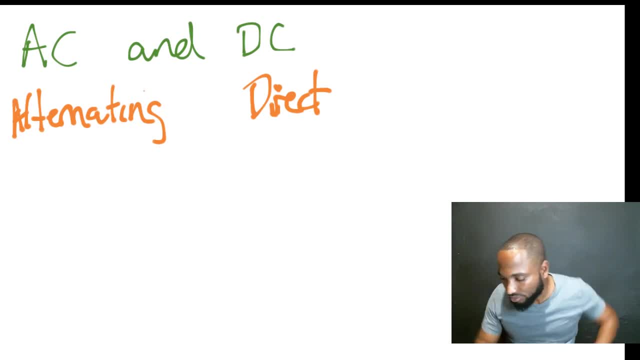 It's not really randomly. So let's see if I can pull out that neat definition for y'all. They see, the flow of current that flows in both positive and negative, but direct is in one direction. Yeah, that's okay. I wouldn't use the word. I wouldn't put the word randomly. 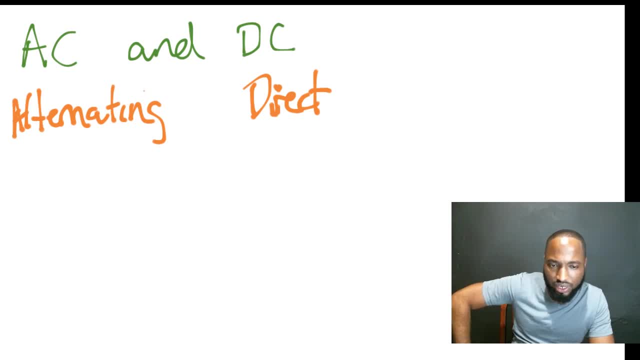 I wouldn't use the word randomly, right? So people, basically that's the definition there. All right, let's see what they're talking about, but I'm not going to tell them anything. I'm going to tell them, basically. 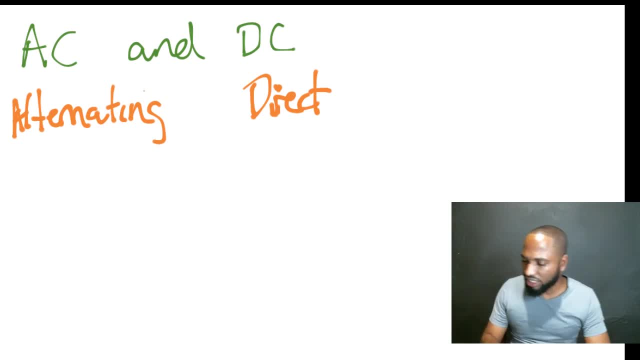 how this shit has to generate. Yes, And I don't think you need to know why. I really don't think you need to know why. Once again, let me just peep this a little bit and see if you need to know why. 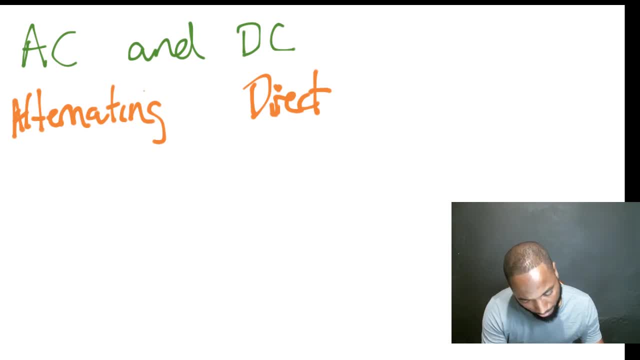 For CXC, All right, so you don't need to know why Alternating current doesn't lose as much heat in the wires. right, Because you're going backward and forward. It's easier to send an electron backward and forward like this. 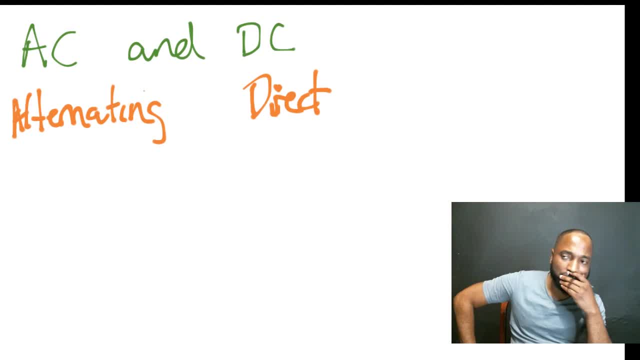 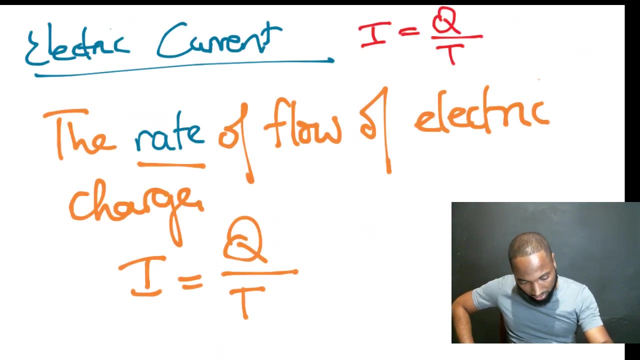 Send the current backward and forward like this, instead of sending it continuously in one direction. So we already some people jump in here and miss some of the definitions. Electric current is the rate of flow of electric charge. Yes, so instead of using it randomly. 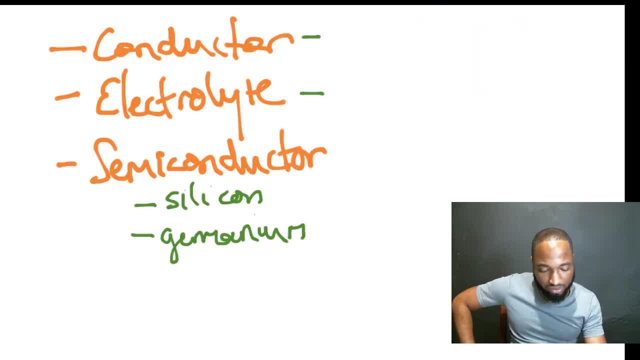 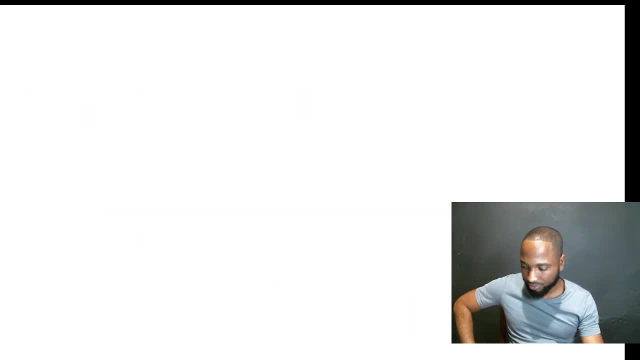 use it with periodicity. So that's the way you want to track, to chop down when you're using alternating current. All right, so let's move forward. Test for alternating. You should just know what happens. Oh, yes, Lord. 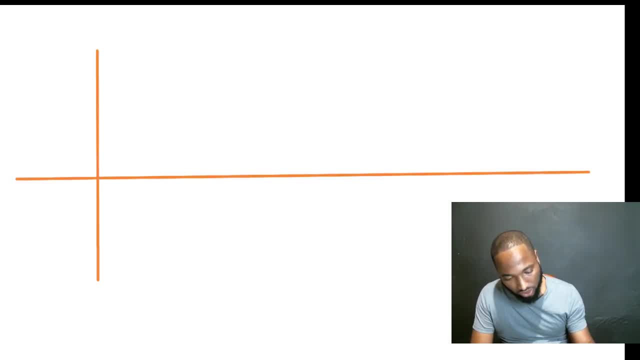 So you want to see alternating, You want to see this in direct And you see this right. So we're going to reach up on them thing. We're going to reach up on them thing in just this. Don't worry, don't worry yourself. You see waveforms, ting, ting, ting. We just want to make sure, we're sure that we're not going to be saying: you know you're going to be in a situation where you're going to be a little bit more, you know. 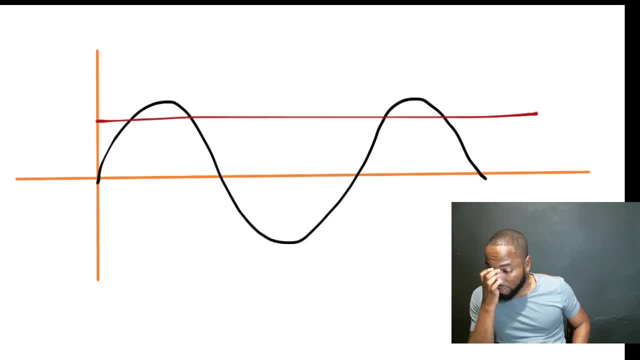 you're going to be in a situation where you're going to be a little bit more. you know, cover all the points listed here. let me make sure I cover all the points as I going up, so once everyone's never see some wise in the chat, if you are. 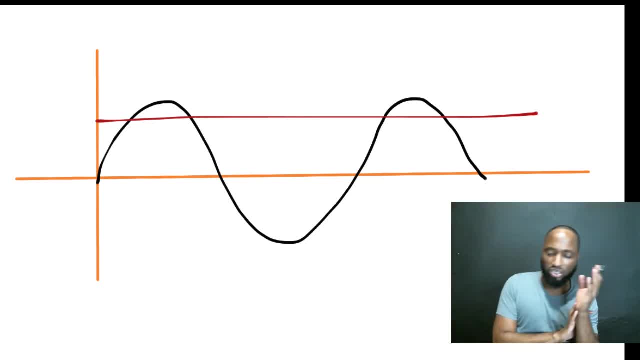 watching, right you? why is in each other, if anybody else here, I trust in 300 people, any life, which is great, right, let's, let's. let's describe this from here to here: is what? what is that thing? what is this term here? what is that to? 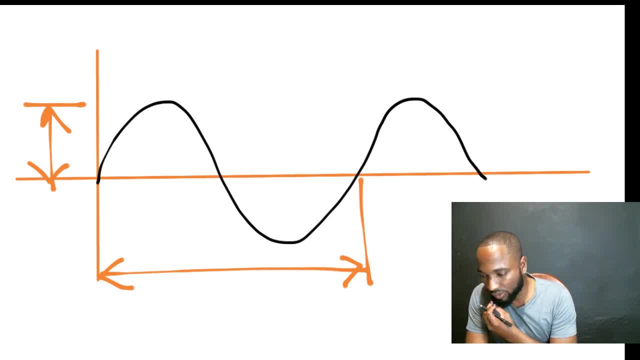 us this year is normally V, this is normally T seconds being votes, so that's one full wavelength. but you better wait, for this is period and this guy over here it's not amps, but I'm tea chewed right. so can we get a definition, pretty amplitude, and can we? 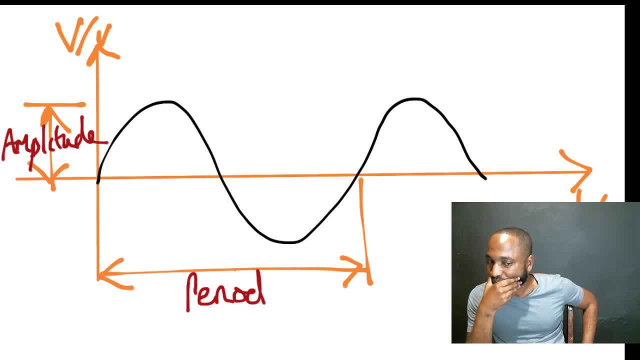 get that definition for the period. can we create one? can we? can you make up one so you like, if you don't find one in textbook, and you might find something if you don't find in txt. if you don't know, oh, you make up one so you might if you don't find one in textbook and you might. 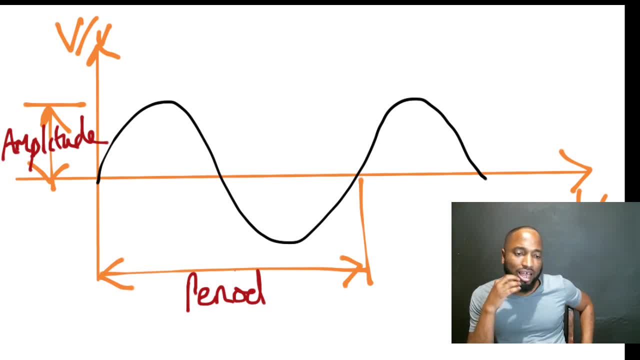 make up one definition for amplitude definition superior. remember period is in capital T. I'm sure I don't worry about. yeah, we get the injustice. come on like, use our forms exceedant, you know, ensure that I'm did you'd maximum. displacement of the waves from equilibrium state that right maximum. 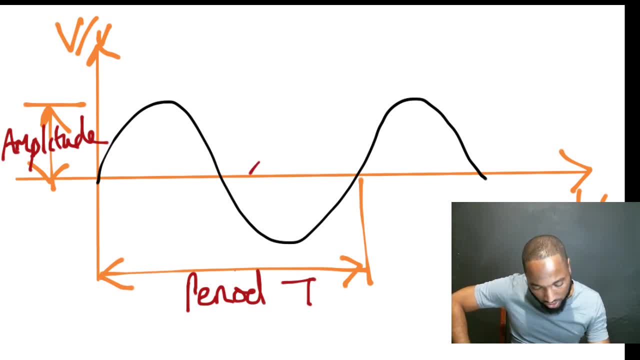 displacement of the wave from equilibrium position. so this is an equilibrium position, symmetrical position there, if you even symmetrical and if you are the time taken for one complete oscillation right. so if you didn't know that, you can look at each other. we have that down there, coke, and 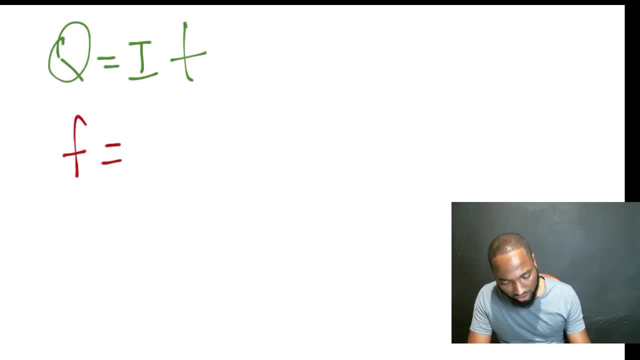 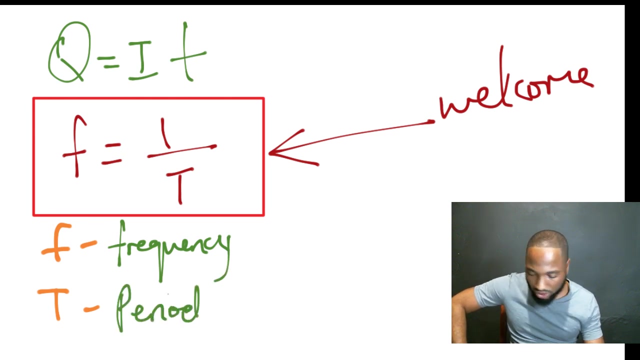 there's one more equation, so so far the only equation, really, one of our team, one of any dance. so everything got a 1 over T, where F is what is F, what is T? well, we know, F is frequency and T is here again. so let's. 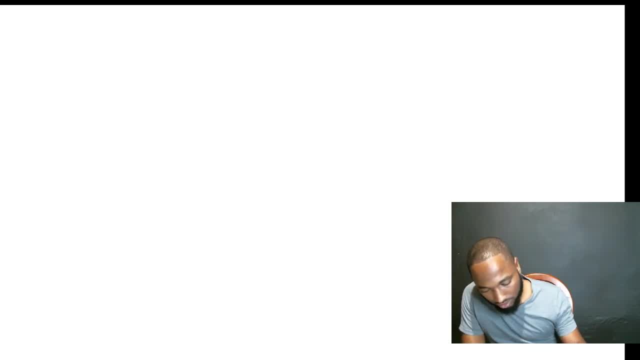 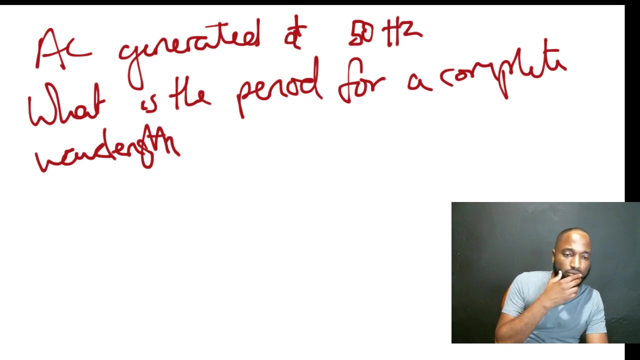 go question. that's the question: if we have AC generating at 50 boots, what is the period for complete with next? so we from more talks about the form, so you can just plug in your formula here. but whoa, that writing sucks, man, so I'll read it easy: generator that 50. 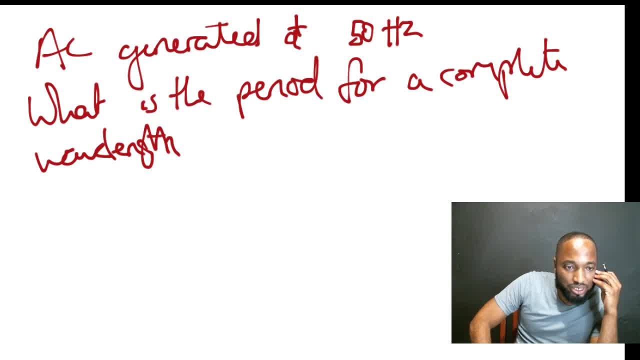 hits was II. what is the pure fire? complete. what does it prefer? a complete wavelength, though. are you gonna do some more complicated question? that's now so the period you can use it interchangeably. you can swap these two, right? the F could go there, the T could go there wherever. so this is 1 over 50. 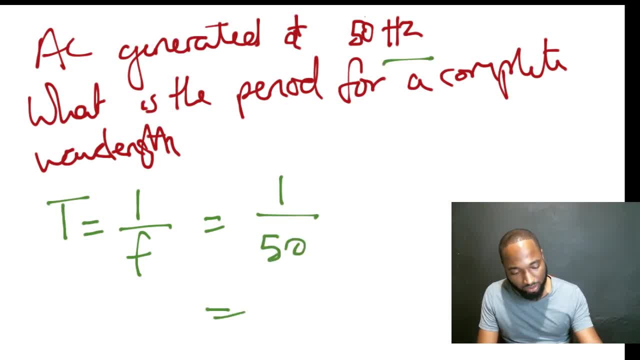 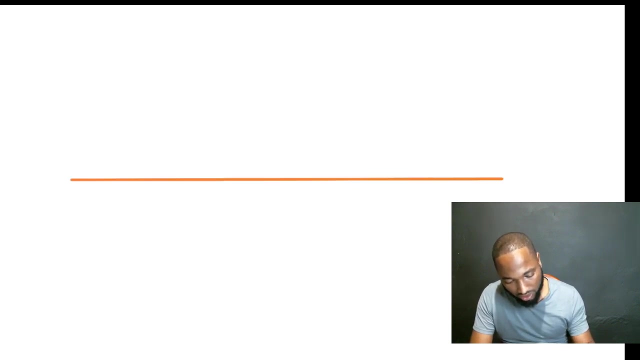 hoods. make sure this in hoods so that the answer could mean seconds and everybody in 0.02 right seconds. let's pull up a little harder question. can I get a harder question? no, man. let's create a person with a diagram then, so I. 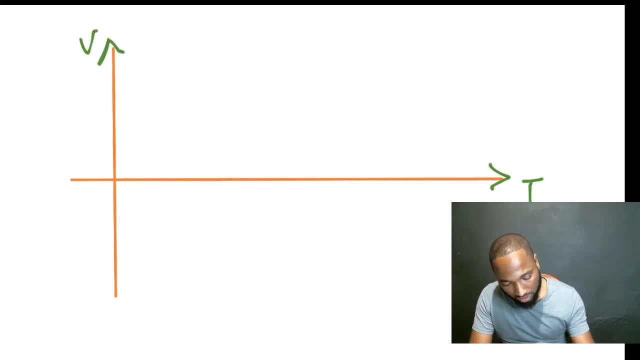 have V here, I have T here, okay, okay, let's draw much more. ya, yeah, if I can get this drawn properly. and let's see: this is, And this is 0.04,, this is 0.08, it's time in seconds. So what is the period and what is the frequency? 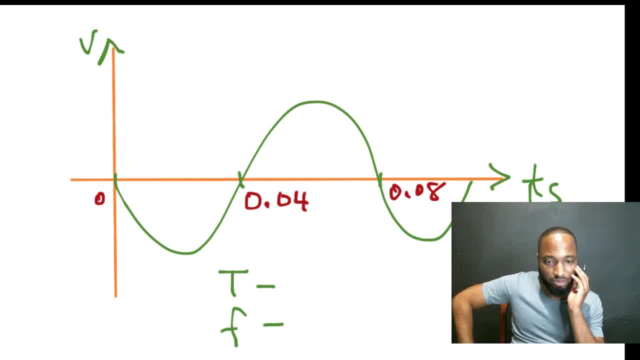 What is the period and what is the frequency? It blurry, It blurry, night It blurry. Turn up the quality. Are you seeing it blurry? Let me check my internet here and see if it's blurry, It's fine. So, period and frequency. 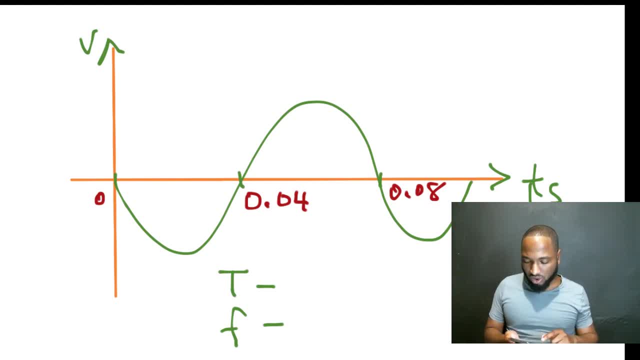 Now I remember doing a pass. I do about three pass papers on YouTube already, So you can search Cohen's. bring up physics and you'll see pass papers. Everything looking nice. Oh it looking real clean. boy, It's like one of the cleanest I see it looking. 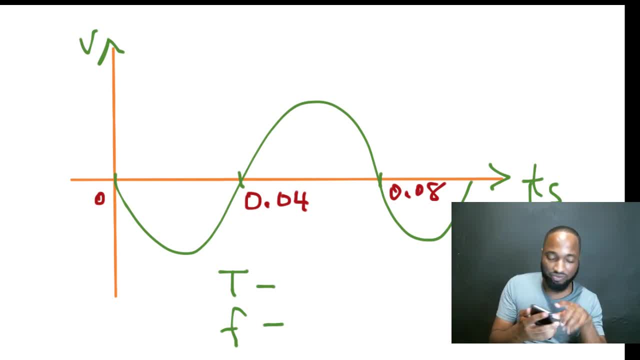 I must use more colors in the lighting: Nice and clean, Fresh and clean, Crisp. So the T. you'll have to use your eyes and pull out the T here, right The T, actually easy. You're looking for one complete wave, like wave four. 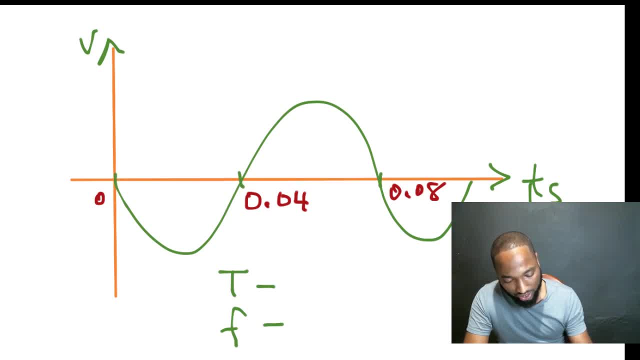 So sometimes they might be a little sneaky with that. however, they do that, Bam. Now, a complete wavelength is from 0.04 to 0.08.. Okay, A complete wavelength could either be from, if they ask for the definition of that and 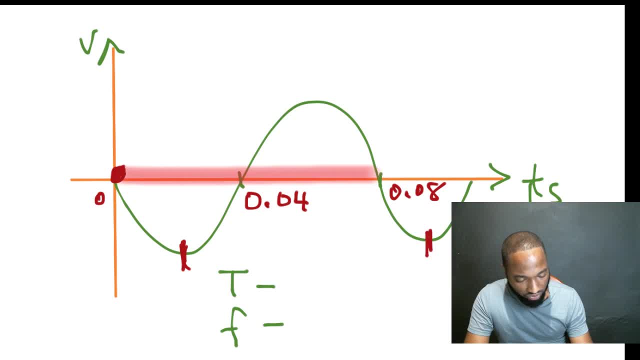 they might ask for that- in waves from trough to trough or from crest to crest. That's the best way to define it, right, That's the length of a complete wave from trough to trough or from crest to crest. So you see now the T here is 0.08, which means frequency will be one over that which. 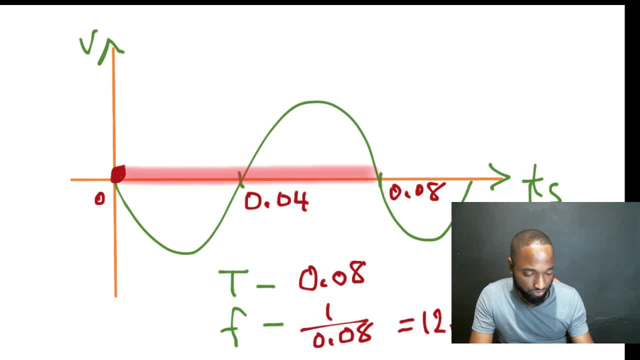 turns out to be 12.5 volts, right, According to the chart there. Now, before I do this here, I'll write: F is equal to one over T, just to make sure you get your formula max there And you'll be good to go. 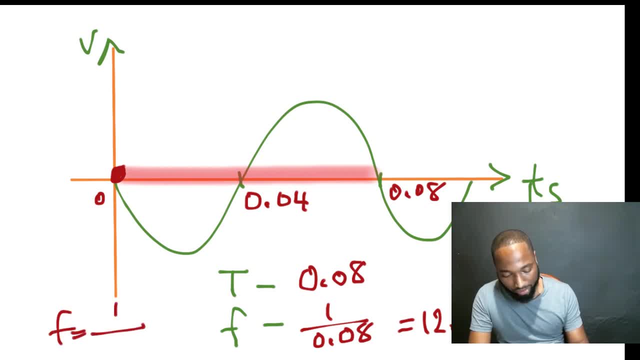 You'll be good to go. All right, Any problems with this? Why is it in the chart? I don't think this will come any more complicated than this. Okay, So let's see. Okay, Okay, Okay Okay. 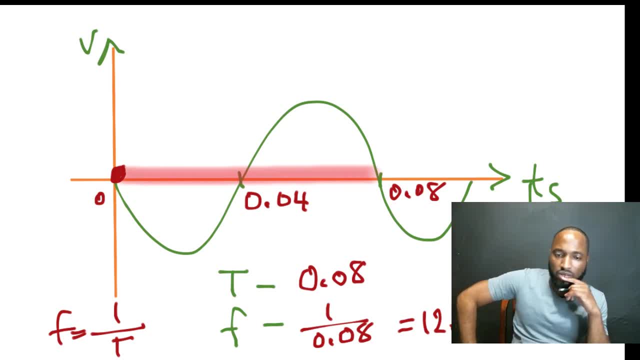 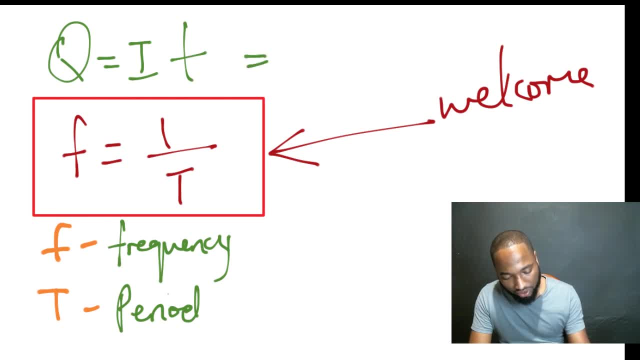 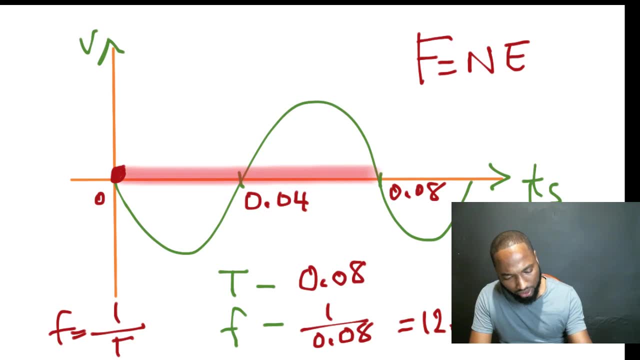 It's not F, Q is equal to NE. No, F is equal to NE. It's not F, Q is equal to NE. Okay, Okay, anyway, I say f1. we end as a number of elections. right, how I guess your point? 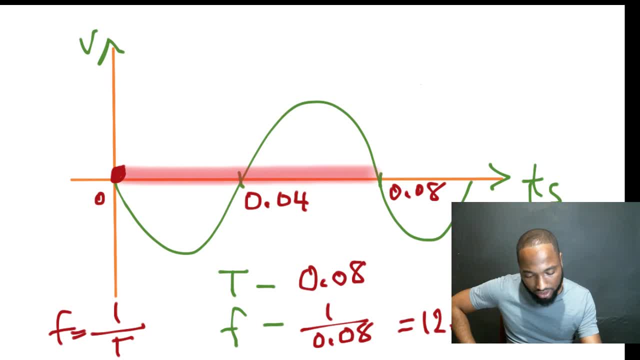 eight zero point zero eight well, is the distance for a complete wave to take place. some of you still don't think it's right. so you get your friends here, eat. understand it now. I understand it now. the next life, I'm gonna do a billion waves so you'll get your optics a light and we use something. yeah, so it's just a. 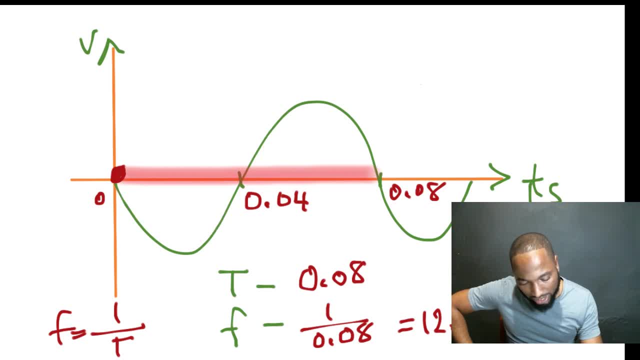 complete wave from zero. sometimes they might start it and not zero, so look for that. you just take away if they don't start to come to you. you just want how much pass here? nothing, 0.08 seconds past there. nine of the car take too long on us. we have a long. we have a long night. 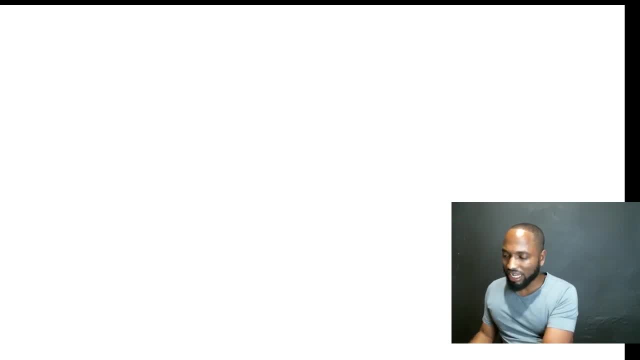 ahead of us. let's look at electrical quantities. no, I don't think. I think we have next, next, next. well then, electrical quantities. electrical quantities. so what are the equations we covered so far? you tell me the equation we covered so far: Q is equal to IT, common T. I keep. 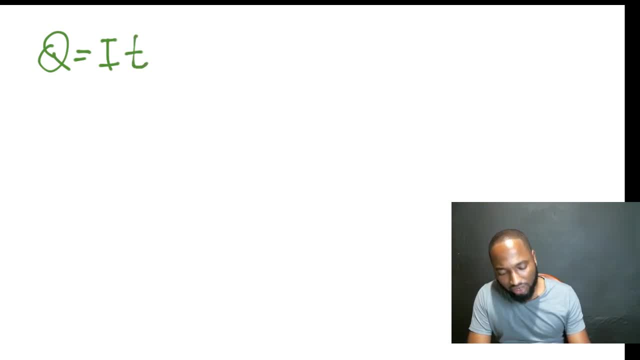 playing capital T, because this book has capital T by a customer, common T for time. we also had a next thing for Q. if they, in case, they give us this weird one- and he, where he here, the child- in one election and n is the number of elections, sometimes written as common Q, sometimes they'll write this as common. 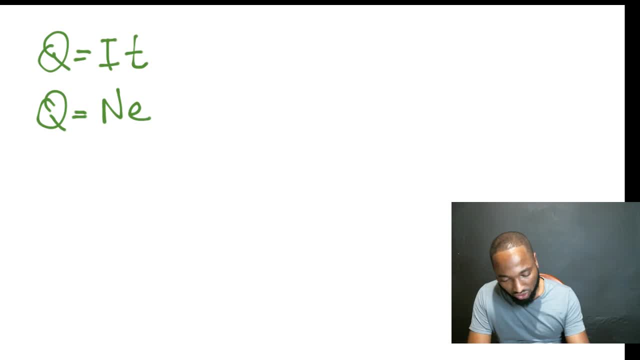 Q: right, and we just introduced this new guy. yeah, we just introduced this new guy, for frequency is actually one over the whole time period, the whole period for the thing. so time to take in some new one, so that he: this is what we have so far time to take in and you bring in a. 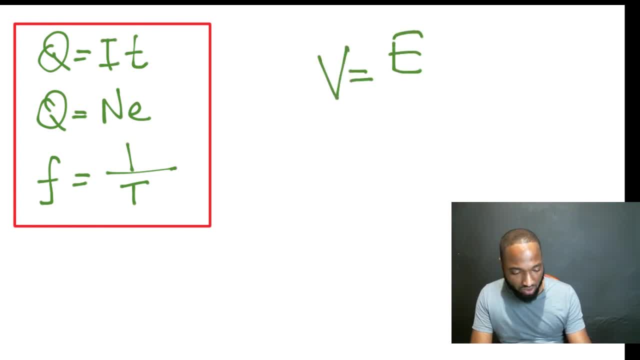 new one into dance. V is equal to E over Q. no, I never learned this equation like this. it's a matter of fact, I never really knew in this equation. I learn this equation like this because I like to start on equations with him, if you that's. 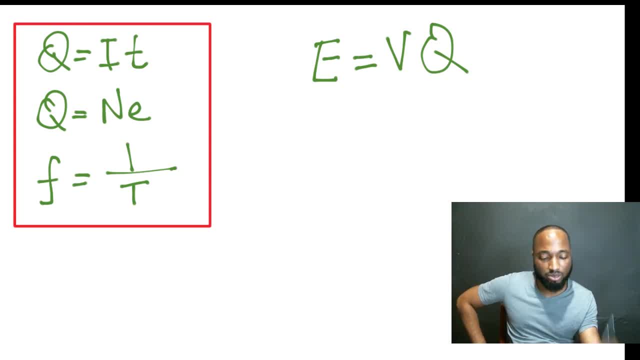 all an equation and I tell with them a thing: right, but we just teach it from: V is equal to E over Q. can you tell me what the E and Q stands for? E and Q? in the chat got the E over Q. he stands for what, Q stands for what? well, we already know Q. 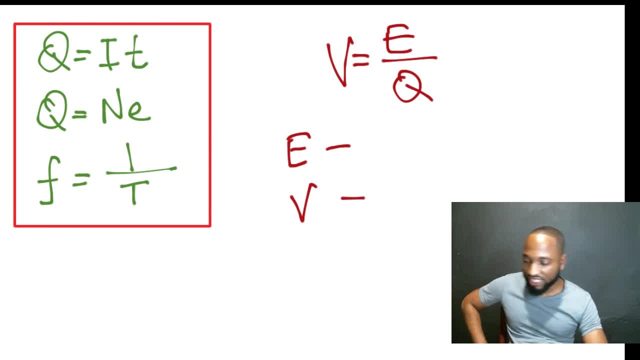 stands for chance. I don't need to see that. what does the E and V stands for right? so the E is energy and the V is voltage. the V is voltage. oh, I missed anything, that's right, he gets to go a little. so this is in, you guys, we introduce and I 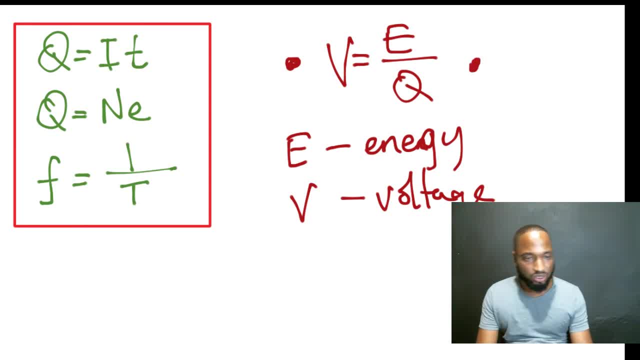 will introduce one more new guide. this is how she should mentor. yes, well, earth, injustice, injustice, but they are final fu is that you come and he do. you come and you go alive with me. why, cuz like, you really think he is equal to now? this exists, this exists to the left by this way, what does this mean? what this means, what does this mean acting, parce dit erre OFFICIIS DE VITAREится perz. I'm not saying anything else now. now, this is the example of non acting harmonizing, or an act of the creation of IAPC. 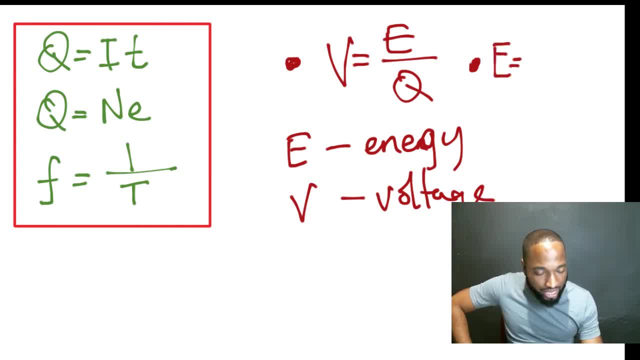 your thing. he is equal to. I squared R, T. no, I didn't learn this like this. I learned it like with H, because most of the time they use any this equation, you're finding energy lost in as heat or something like that. so H here represent the energy for me and I just learn it. I just telling you what I, what I need to. 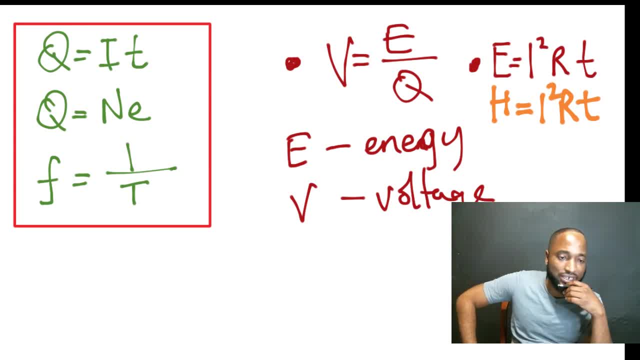 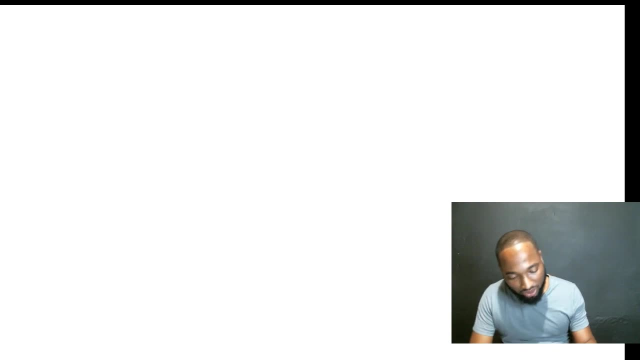 remember this equation and I just remember to square the eye right. so that's the next equation. you want to take him, but learning this equation, not very, very necessary. I might as well tell you the very necessary equations: T is equal to IV, Q is equal to I T, V is equal to I- R and that E is equal to V- Q. 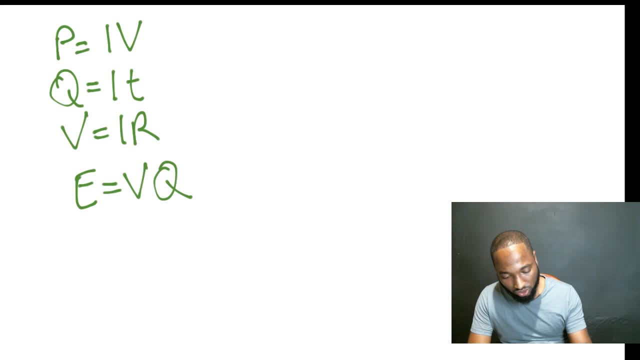 and that E is equal to V Q, and that E is equal to I R and that E is equal to V Q. those are the big boys. learn those right. learn those. so everybody had those equations. don't see if I know what it's symbol. I mean, this is some wise in the chat. 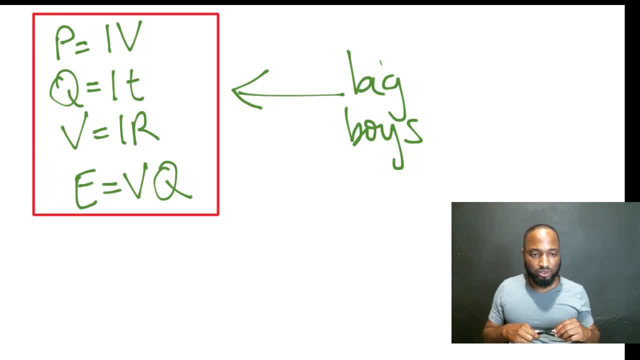 so why so? why? why? why? why? why he has in power, yes, the support I sped out yet, because i sped out yet, yeah, but oh, you don't工 anything else. really, once I was in the chat, these equations, all my Spanish 150, it's just a combination at these two versions. 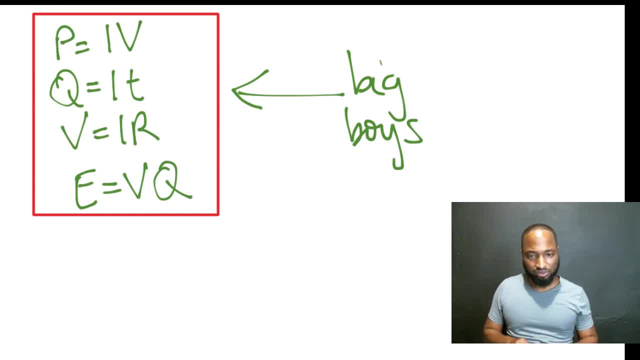 of. as I said, they really should have done anything else in the time frame when it's. If I want to get rid of the V, let me just show you what I mean. For example, if I want P in terms of I and R, if I don't want no V, I'm in there. 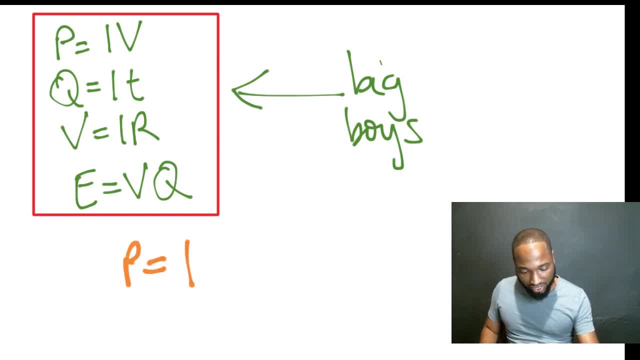 Well, all I'll say is: P is equal to I, and instead of V I will write what V is I, R. So P is equal to I, squared R. So all of those kind of derived, Some of these derived too, but I'm telling you, these are the equations I just want to make. 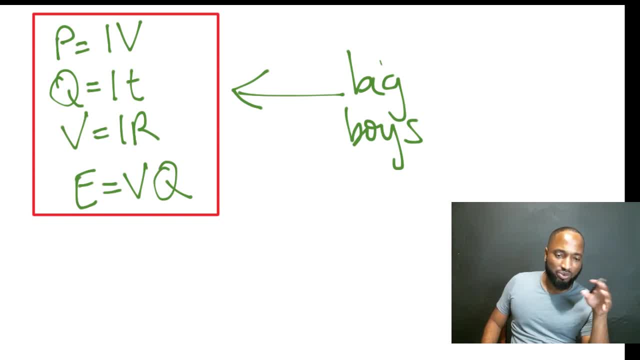 Just these guys. You have a few more equations to do, like the equations for resistance in parallel, resistance in series and maybe something else slipping me or something, But this is the key here, The key to setting people free, Right? So just take a good look at that and you're good to go. 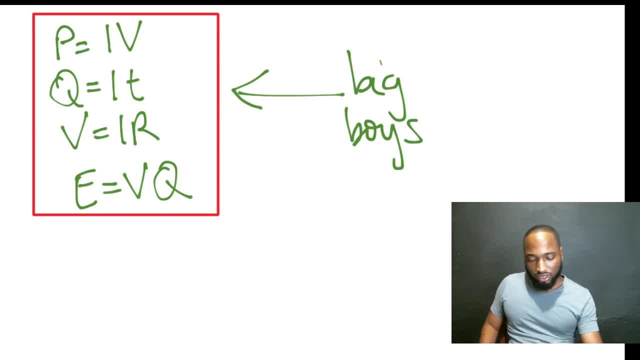 And actually in a question and a concept you must be sure about. a concept you must be really sure about is that power is energy over time. But the answer comes straight from the first part in physics. First fact: Power is the rate of change, of doing work. 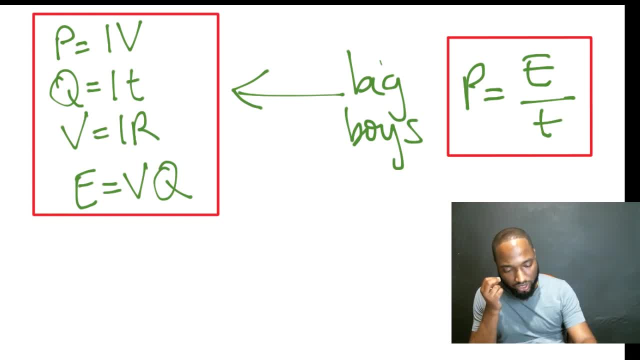 Work done over time is equal. So, with this concept, With this concept, you can mash up. Once you have this and the big boys, you're mashing up an equation, An equation they might ask you, you might find out the electricity, the energy, sorry, and 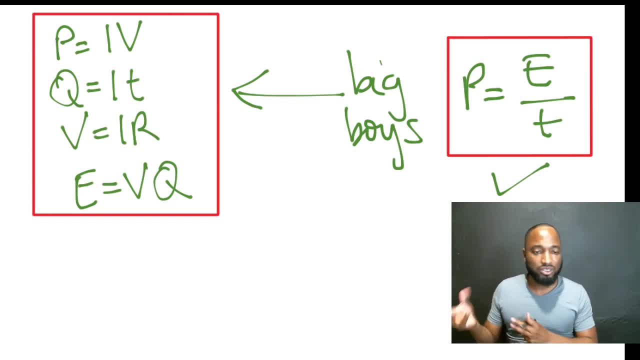 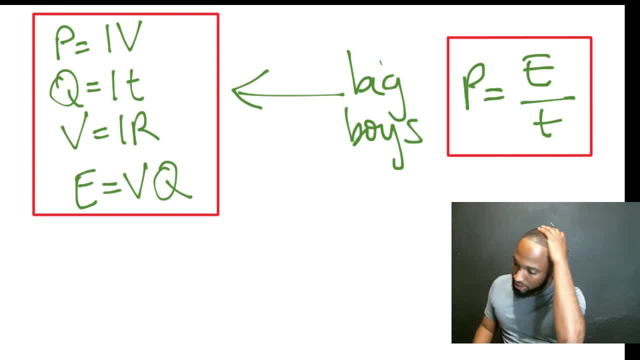 you know you need to know energy conversions of different appliances, like electrical stove, in that you can heater the light bulb and the motor. in the motor, electricity start with the kinetic energy and motors like a fan, electric energy converted to kinetic energy obviously in your light bulb, electric energy. 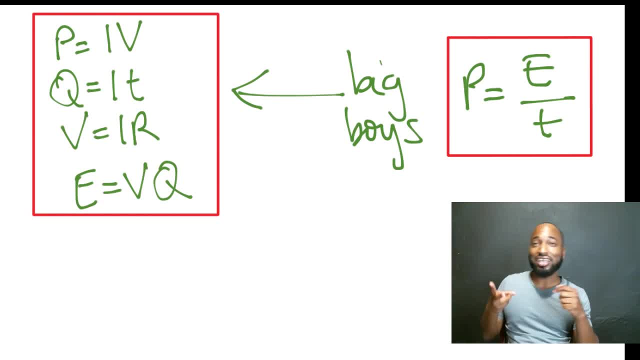 converted to light energy and your heater electric energy converted to heat and your stove electric stove electric energy converted to heat. so you know a little basic conversions, that easy thing. that is annex not a mono engineer fireman that lead to the first time. so they just know what they call a mono engineer fireman in a Dennis. 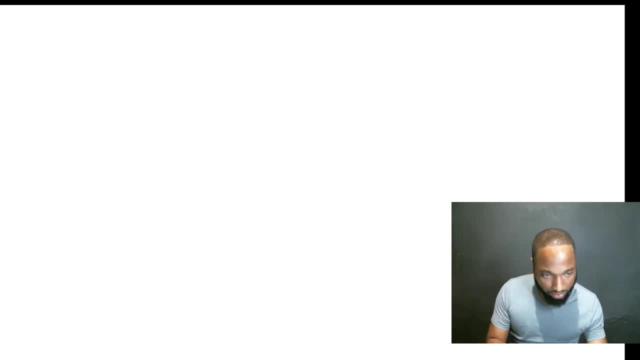 in that they call them as敢. you know you can mean, oh yeah, they can have a little bit of energy. so that's the big thing about the big boy. you know you can waterfall, water and images, right, okay. so, as I said, the technique for learning chemistry when we chemistry exam pass. 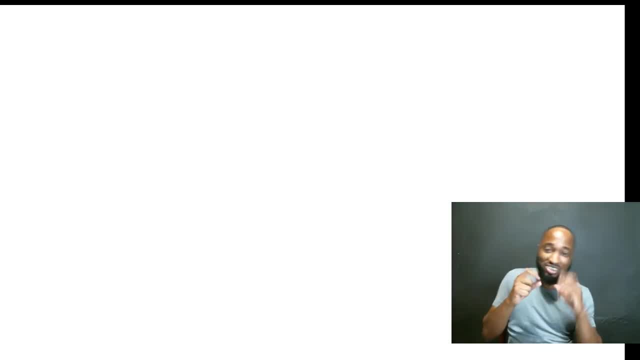 was what we did in that life and I really condensed everything into a nutshell and just kind of cram it in your mind. you know a few exceptions, the rules, you, they see that equation, boom, boom, bam, bam bam. you have it. the technique for learning physics is to try and understand each topic to the best of. 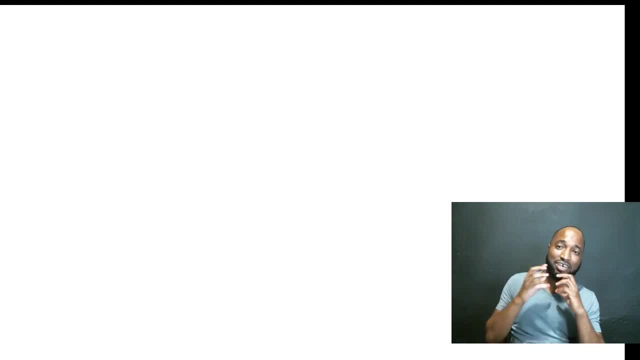 your ability. more you understand the topic, the easier physics become, so physics is not really a something you want to approach from a cram off perspective. same thing with maths. you had to do real plenty questions with maths, physics and maths, kind of. you had to do real plenty questions with maths, physics and maths, kind of. 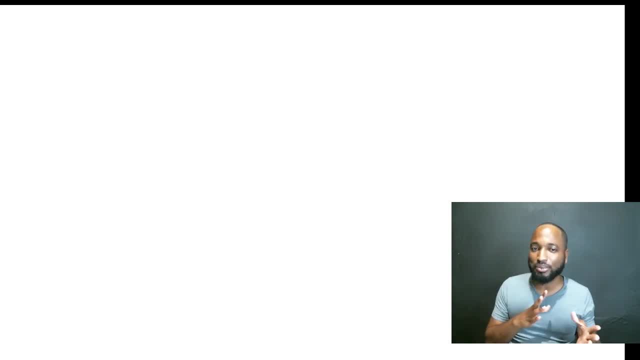 like each other, like that you don't want to approach it too much from a camera perspective and approach it from a try and understand everything perspective and then learn some questions perspective, right? so let's, let's try and understand what is happening here with potential difference that some people see, potential difference and current and they 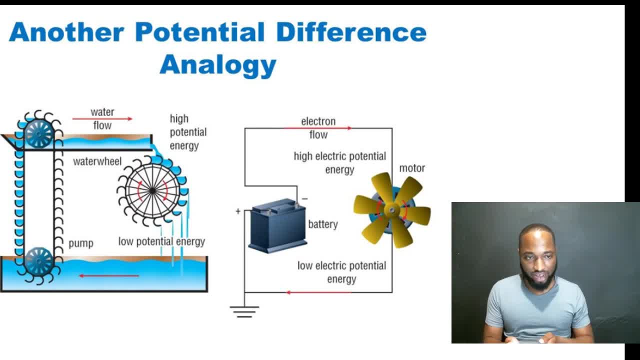 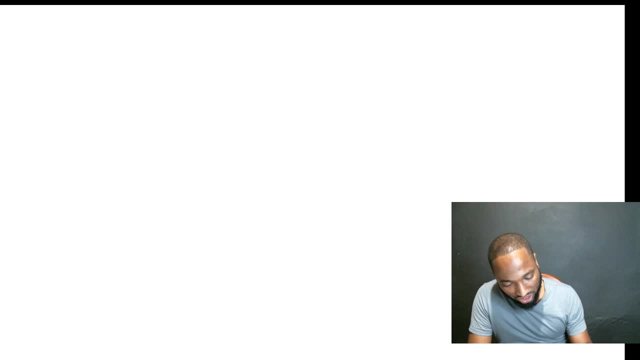 struggle to understand the difference. let me just see if you all see in this diagram properly. yeah, man, see that properly. now this is: this is an analogy. this is an analogy here of what is happening in an electrical circuit. it's an analogy of what is happening in: 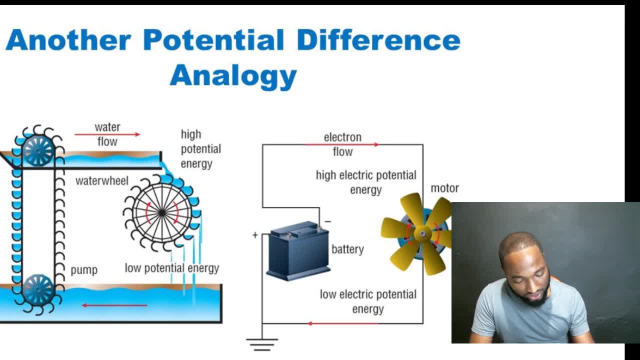 an electrical circuit. well, let's look at the circuit. first, we have the battery. they went and draw the whole battery long side, long side, short side, right. because this is the positive side, this is negative side. it's like, you know you, the battery is giving the electrons a push. it's actually pushing the 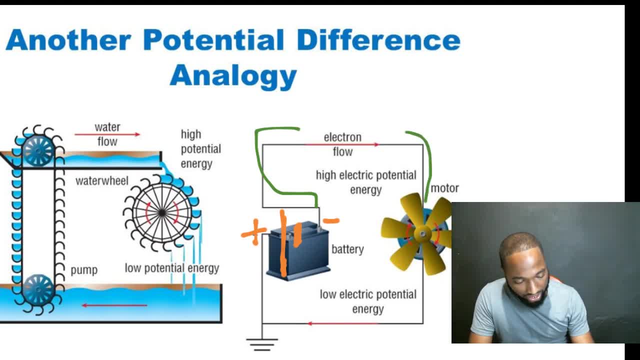 electrons out run. soon it's going to come here and use up in something, some device. now the electrons are going to use up and burn away and disappear. the electron just going to lose. it's just going to lose some electromotive force. it's going to lose its potential difference, the energy you sent it out. 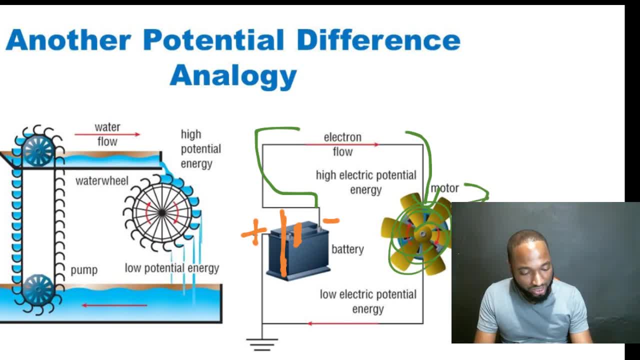 with is being lost and and being used to spin the motor, to light the bulb, to heat up the heater, and then it's coming, okay, all right. so let's see how this analogy helps us the understandings. this pump here works like a battery. the pump no notice, the water will never run the system, but never lose water in our 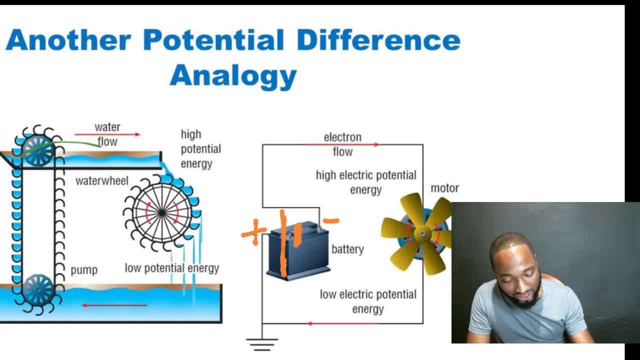 evaporating. but assuming no evaporation, he says no one ever lose water. water, yeah, the water is the current. he waters the electrons, the maturity electrons, in the they don't go anywhere. but these electrons here don't have the same potential difference as these electrons over here. how do these electrons have a? 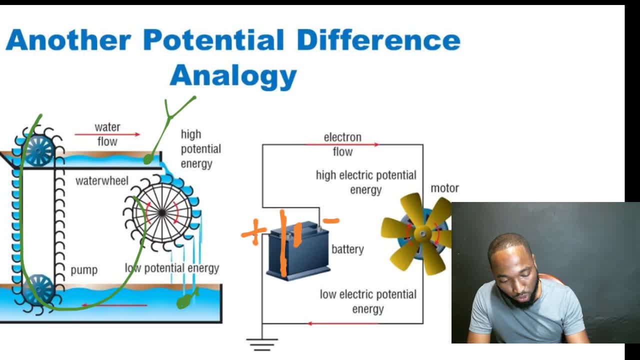 higher potential difference because they pass through the battery and they get boost up. they get boost up and as they fall they get used up in the motor, the light whatever, and they get a low potential energy potential difference now. so they need to come and come back into the battery, be tough and wary all. 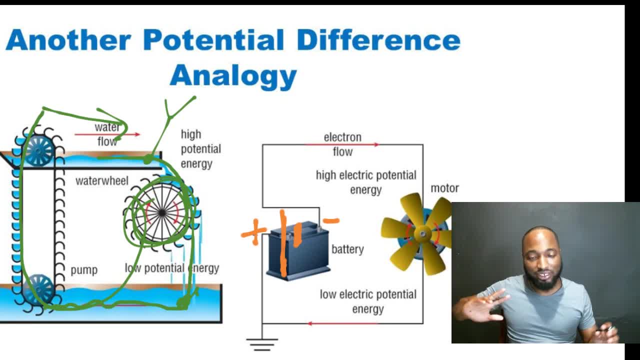 right, which back from each back, reach back, reach back, fellas. what did they say in current? because the same amount of electricity in consumer old electrons, but they have less potential difference. sir the, I won a city. we within the diagram. so in fact, in a parallel thing, you didn't don't write this like a. 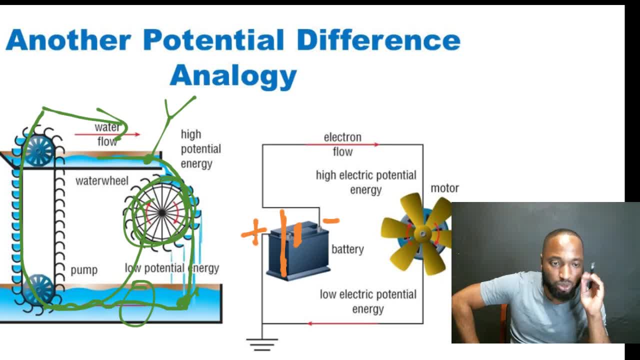 supercharger- no, this is important. and a tricky man, this one. this is important to understand. this. it was important to understand- is it makes it makes it makes getting it real blurry. let me check again. my people seen it. blurry boy, I seen all you, I seen everything I seen. 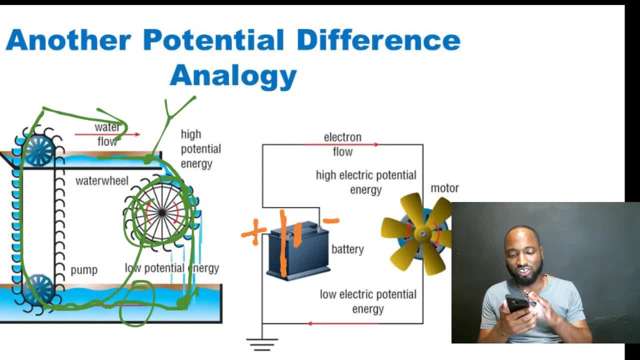 all the words, everything. so going settings and change it from 480p to 720p. I think I streaming actually 720 or 1080, not blurry. all right, so that's the analogy here. we'll start to see this play out in different ways. this is: 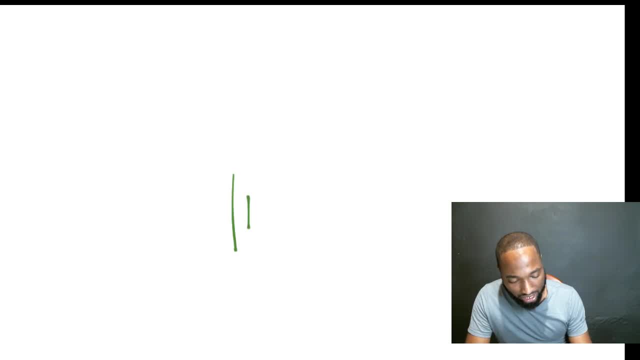 important to understand this figure. one will happen in a circuit, like if we have a battery. why is it that the potential difference here is low and the potential difference here is high, but the current is the same throughout? right, that's important to understand. or why is it in a parallel circuit, if you understand. 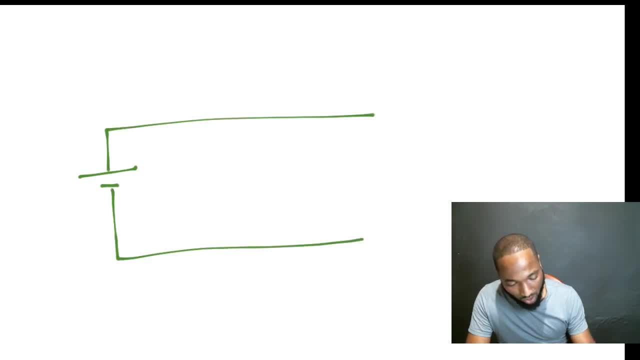 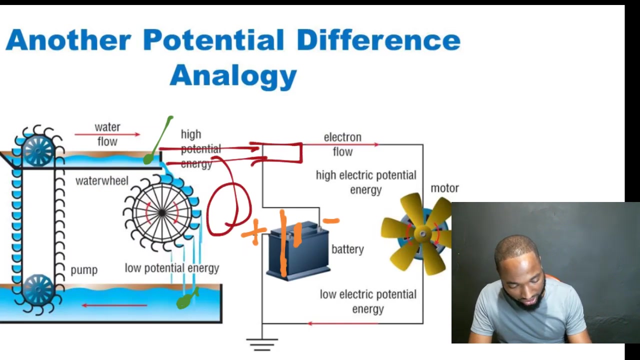 that analogy really good. you'll understand why in a parallel circuit the potential difference from here to here is the same, but the current in each branch is different. the current splits up is because the water is the same amount of water going through. it's almost like if, instead of this, we had more. we had we had more thing more. 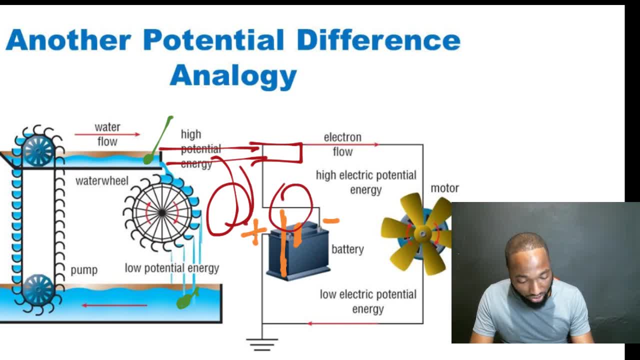 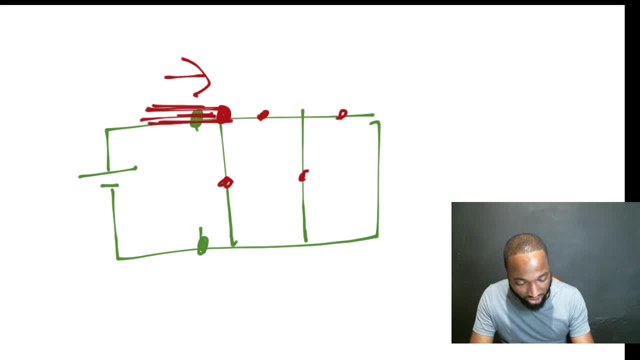 windmills or whatever the hell that is, would be water falling out. here you have the same amount of electricity, electricity here, the same amount of current, but when it reached this junction, some will have to go so and some will have to go so, but from here, from here to here, the same distance and the same like height. it have to fall. 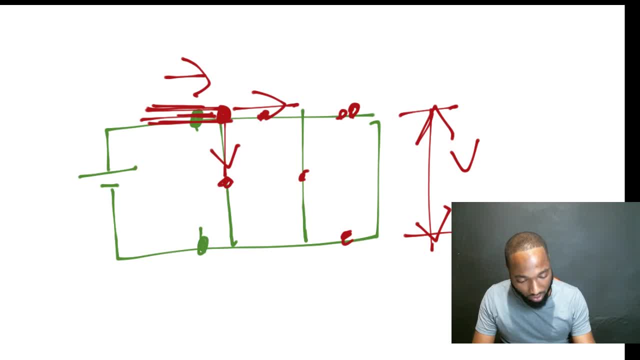 so it will have the same potential difference in all of the branches but it will have different amount of current. so hopefully you kind of see a little clarity there. let's start going to some memorization and understanding of questions. yeah, blah, blah, blah. alright, sure, let's see if I can find a person. so I'm. 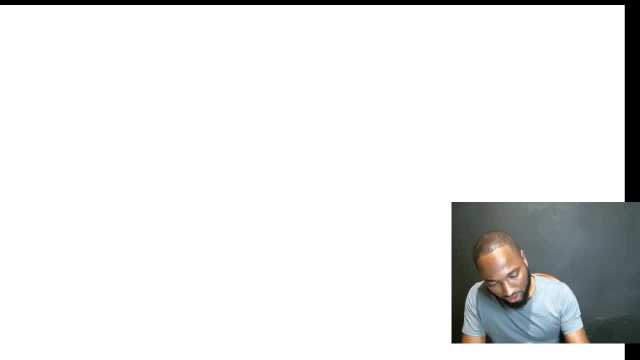 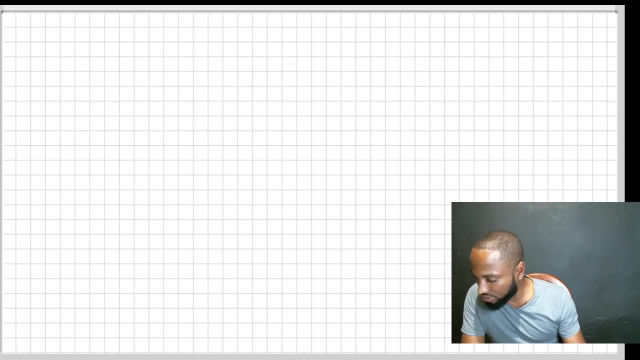 going to write a question here. takes a while to write the question, so you already be watching me writing this question right now. a current. this is not a current. this is not a resistance question, any coming into the resistance questions: красae Zhang current. this is a question involving one equation of three amperes flows through. 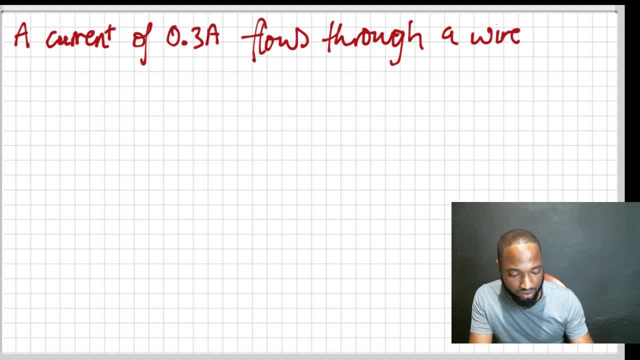 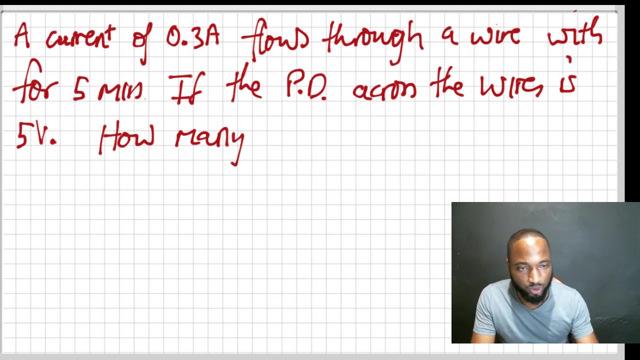 you're reading that- a wire with resistance for five minutes. for five minutes, if the potential difference P across the snowy ever, the the potential difference P across the snowy ever, the potential difference P wire is five volts. how many have seen people talk more things there? Jews, our energy was. 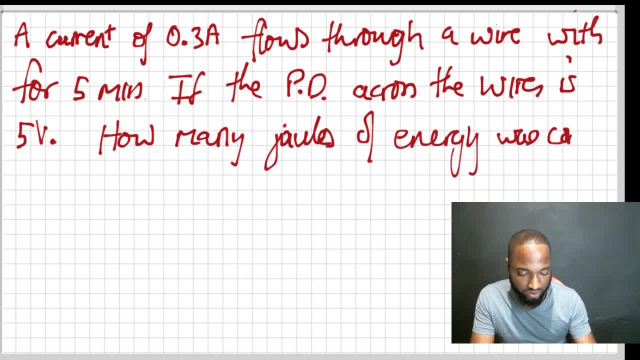 converted from one from another. was converted waiting right? answer this question right. so for 50 Jews to help us at street or the Audi, block somebody. get 500 Jews. second piece: not block injustice. get 450 Jews very neutral in an injustice, running things in this topic right now. 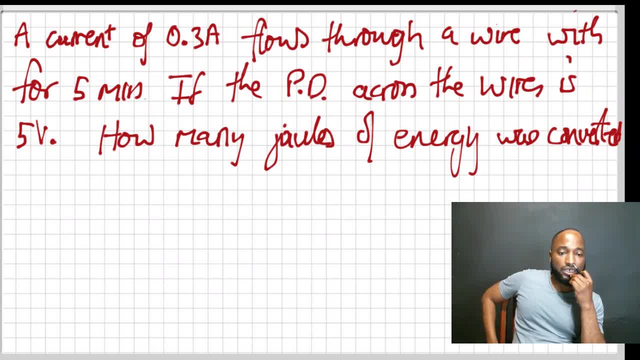 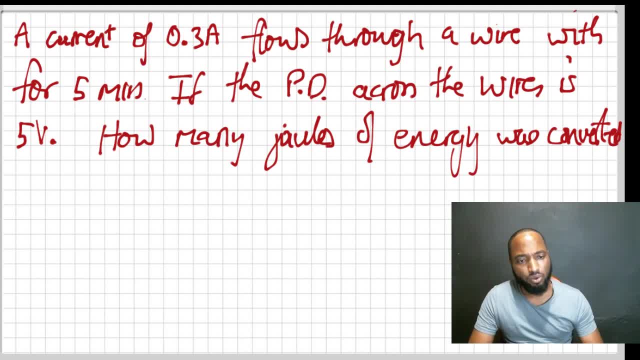 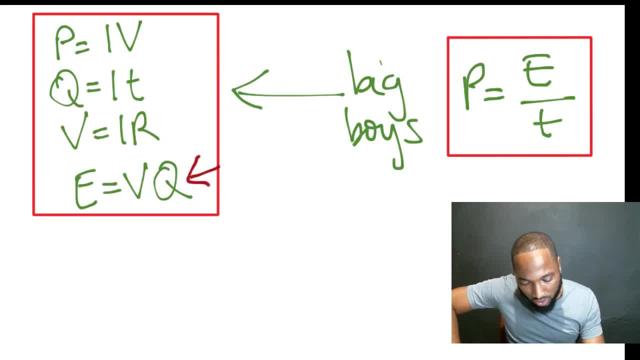 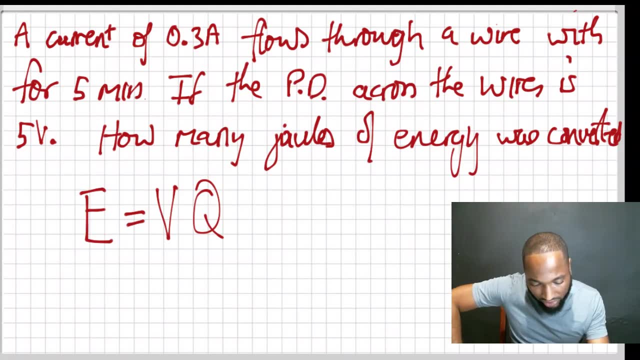 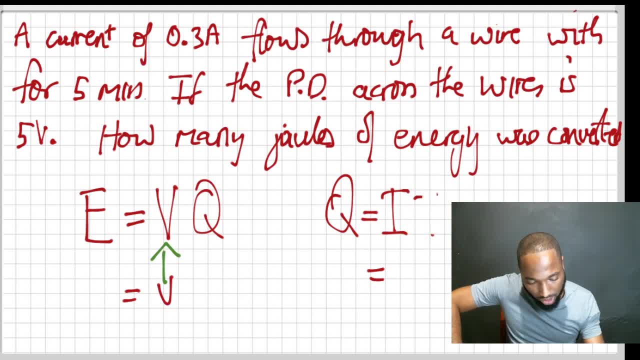 And what about T, Common T? that is, What about T? T? here is time. I have that in 5 minutes, But I need to change that 5 minutes to seconds. So current 3 multiplied by a block in. Well, they catch the idea now. Why is it in the chat? Why is it in the chat? 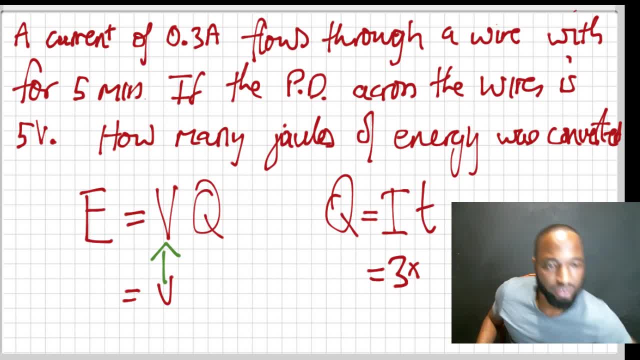 Why is it in the chat, If you understand what to do now Next, So T, here is 5 by. I'm just trying to squeeze it- 5 by 60.. So in the end it's going to be V5.. 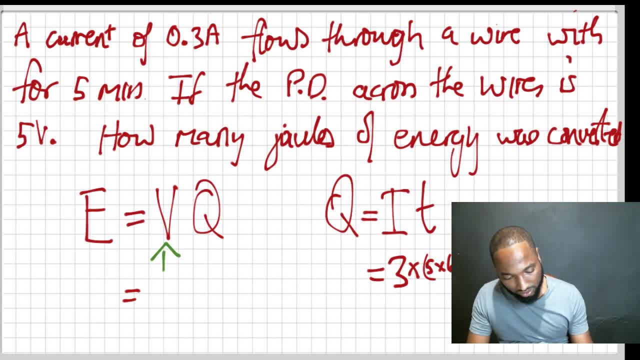 5 by 5, that's hey, the last tree is 0.3.. 5 by 0.3 by 5 by 60.. This is 0.3 from here. Yes, sorry about that 0.3.. 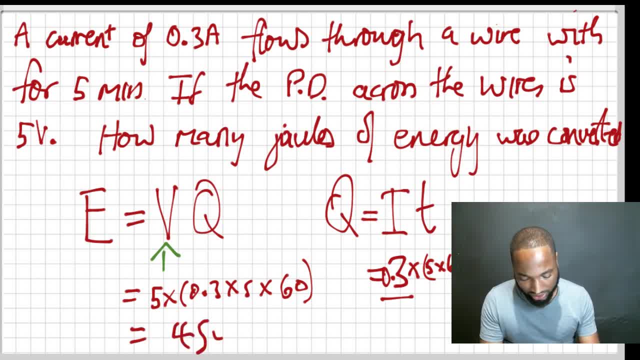 Next And you get whatever they get. I think it's 150. they say they get 5 by 0.3, by 5 by 60, and then you calculate that again: 450.. Don't forget to write J for joules. 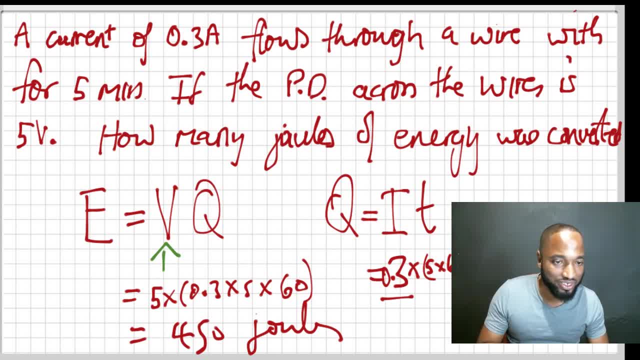 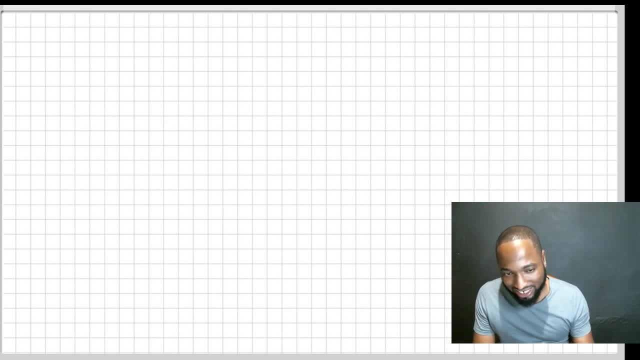 Let's do one more similar to that. I think this is. this is the easy stuff. Do some of Fleming questions, Please come into that. but we had to go in order. Was it time? Was it time 837.. So about 9 o'clock we might be with you, man. Nah, a little after 9.. 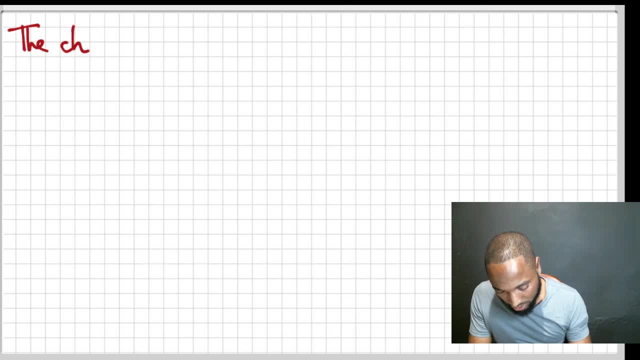 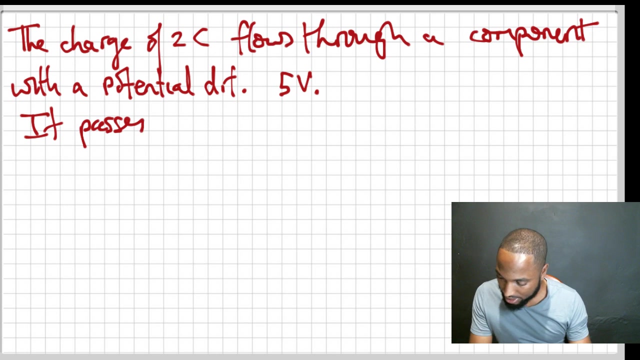 So the charge Of two coulombs, of two coulombs, of two coulombs, a component with a potential difference of five volts, it passes in 200 milliseconds. what so bad is, what is the energy? consumption, and that's what comes on. so, consumption, what is the energy? 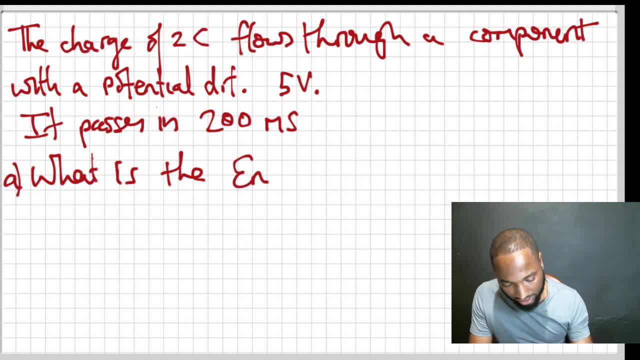 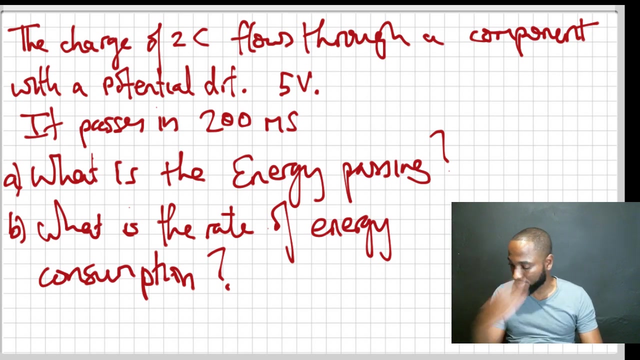 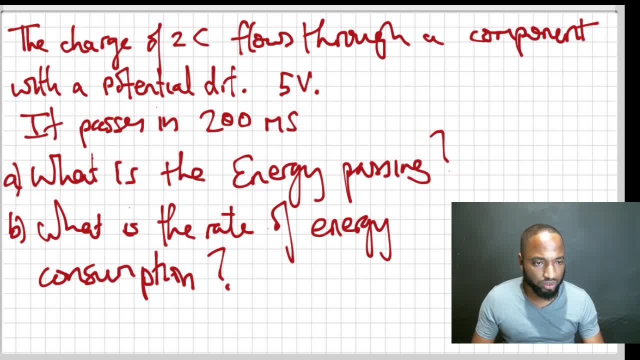 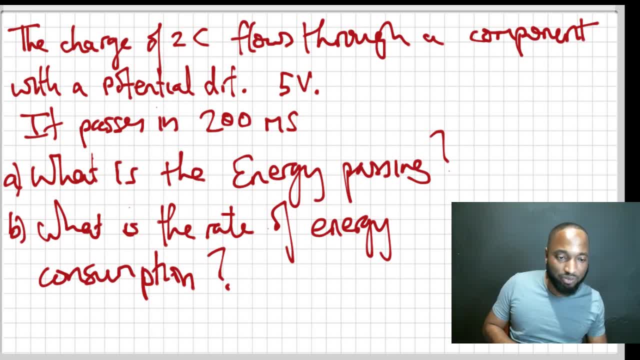 loss here and see loss B is acting for power. yes, so anytime you see, and then you see rate of energy, nice code word for power. rate energy in physics, in any section of physics, rate of energy is code word for power. right, and remember I told you all, you just need to know the big boys, these equations here and keep. 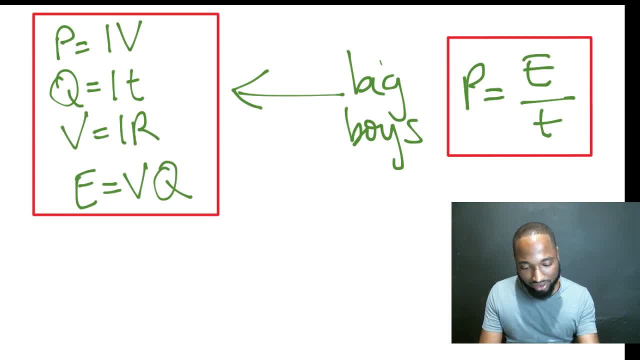 in mind that you need to understand this equation where power is energy over time taken, and normally every time you find energy they might destroy, not a poor talk afterwards. and I read, I read: a poor consumption thing is the straight in, the straight in. so just make sure you understand this equation. so I just come. 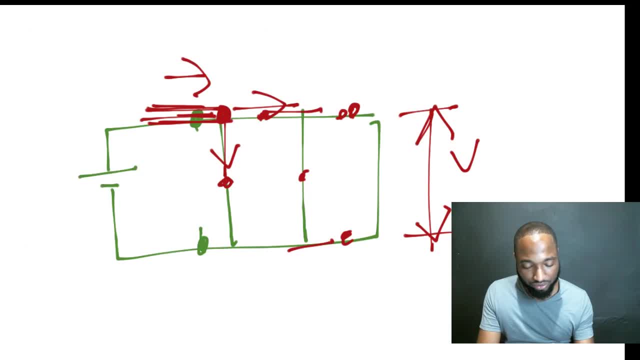 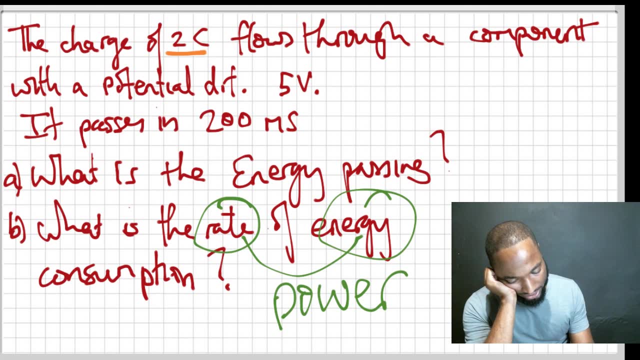 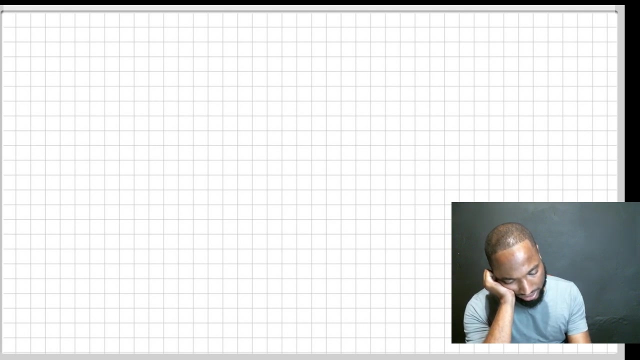 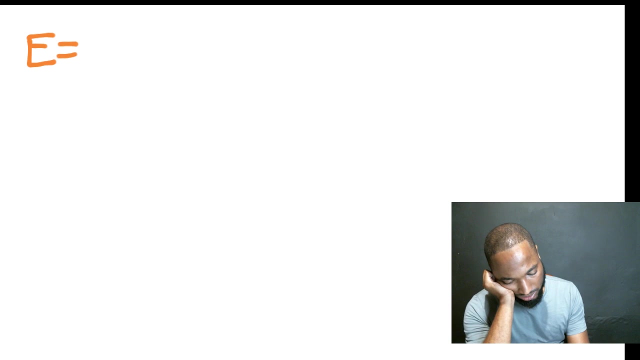 and treat me back here to you. you see, what you could, then we're gonna use very quickly here, finish off this new charge. was this potential difference of that? so the energy, we just use the equation straight up. right, we're writing on this right here. what is the energy? wait, we will just put this on here, let's write. 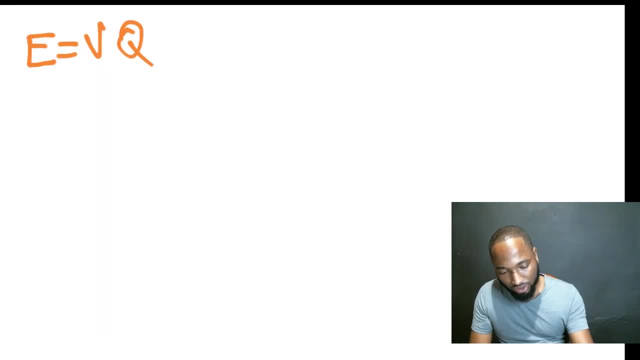 Hart blows two by two by five вопрос to write equal ten than we're going to use this equation. but that's a little minor. guru dia will do do and that you was every time right. but if I was going to be present in my day, this is going to be. 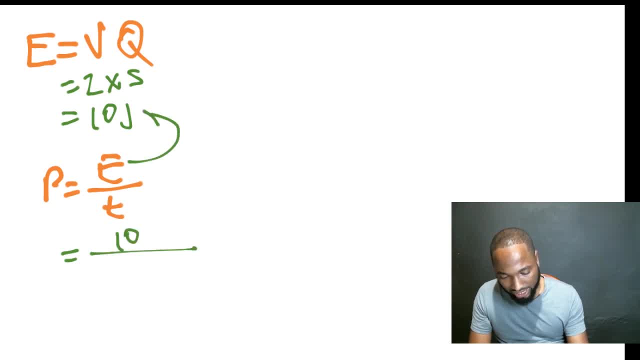 a little mad when I do whatever I'm doing, right, I'm going to break this down, I'm going to get myself, I'm going to work on my, But the time was given as the time was given as 200 milliseconds. so you want to put 200? 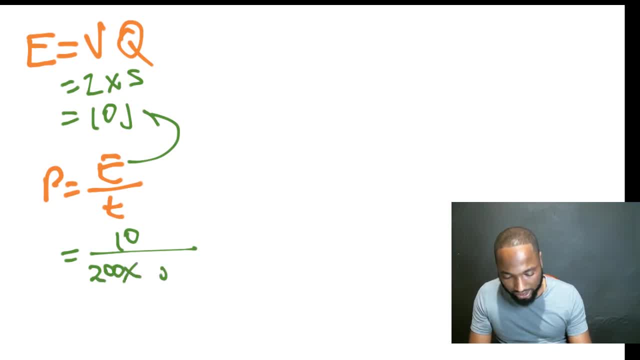 and milli mean thousand, thousand by 10 to the negative 3,. thanks, Shady, thanks, man, thanks. And this is 50 watts. power is measured in watts. Why is it in the chat? So this little part here, this key part here, this was a conversion of milliseconds to seconds. 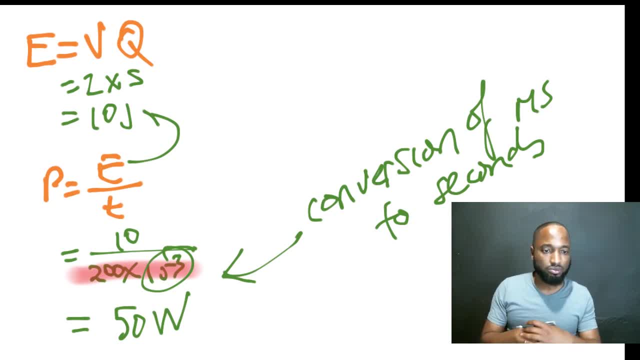 So this, this 10 mic, 10,. yeah, all right, so let's move on, Okay, Okay. So what are some ways we can conserve energy? Conservation of conserving energy. conserving energy: what are some ways we can conserve? 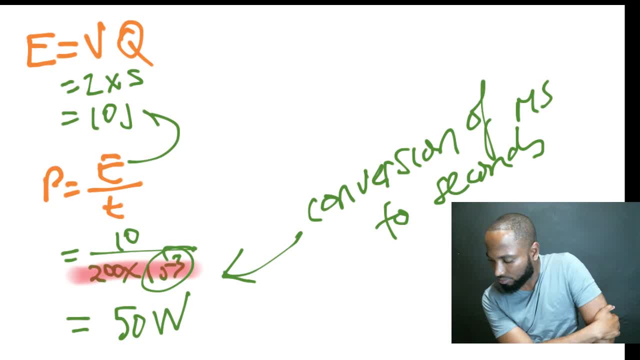 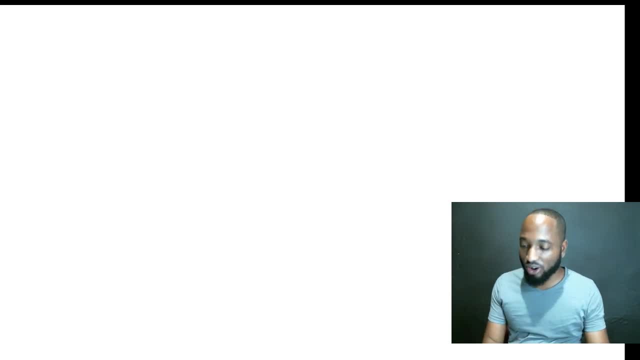 energy. What are some ways we can conserve energy? Somebody say one more. So why? why is he all right? Write while you're all. why it's you're all writing? all right, you know ways to conserve energy and reduce energy loss. 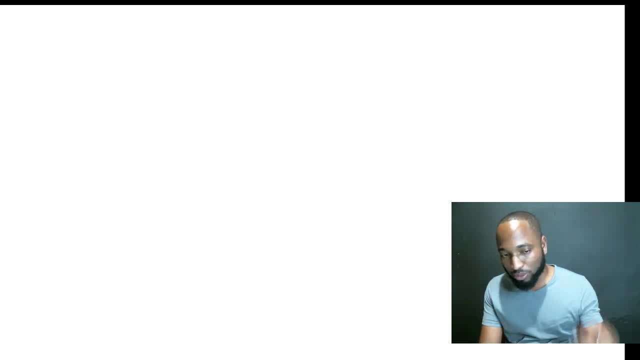 Put this here: loss um, so people can just breathe. good, just reach through that and just write down. one more question: lamp is on for four um 100 watt lamp is on for four hours. what is the cost of this, given one kilowatt hour is. 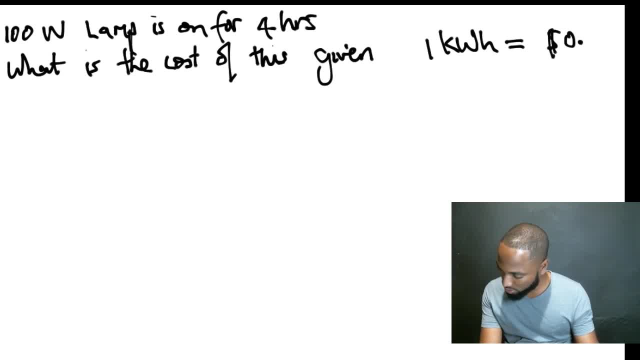 equal to 0.2 dollars. what's the cost of this? now, the key to this kind of question i'm getting- i see one more question because i forget to talk about kilowatt hours- the key to understanding this kilowatt hour question is understanding that this is a unit of 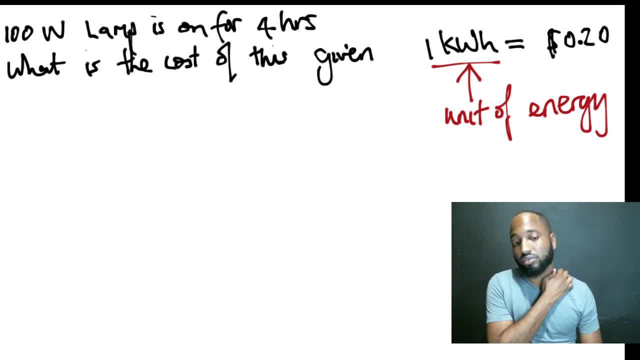 of energy. so i hope you all read all of the steal energy from your neighbors. beg your neighbor for a drive, carpooling right. lock the fridge and stop looking for food if you know it's not there. all that, you taking that solar water heater right, cool, cool. 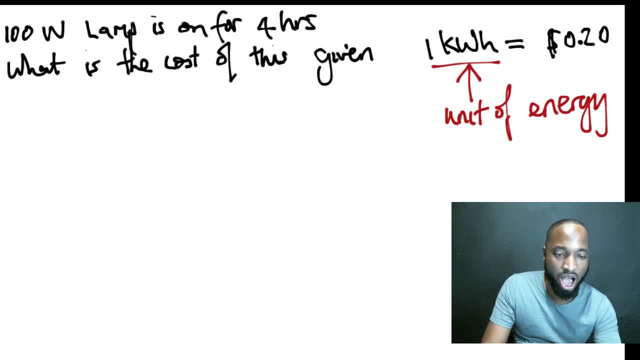 turn off the lights thing, right, good, so somebody get into. well, i'll get this person hang on. um, um, um, um, um. if current family lines 80 cents, so you're going eight cents, you're going eight cents, no, no, no, oh, you're not getting okay cancer. see, i put the wrong question. 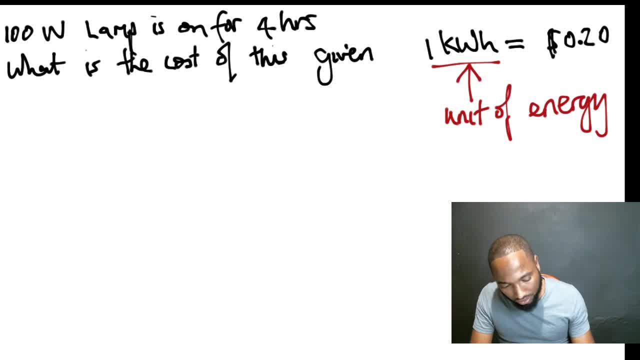 100 watts for four hours. what's the cost if you gain 0.2 cents, 0.2 dollars every kilowatt hour, right? so shania shivani cargani says, yeah, one kilowatt is one thousand watts, but that not. yeah, oh, they forget to make the. 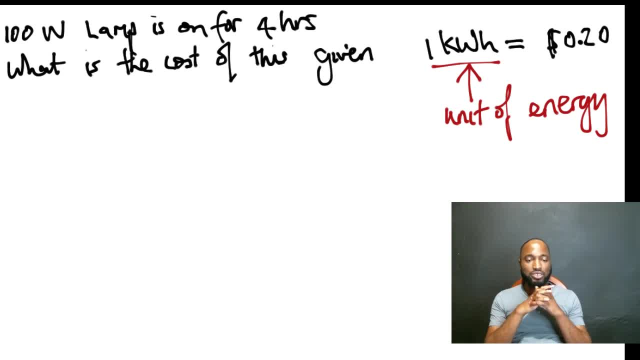 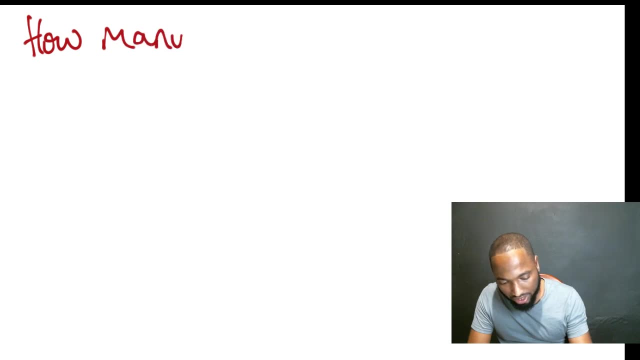 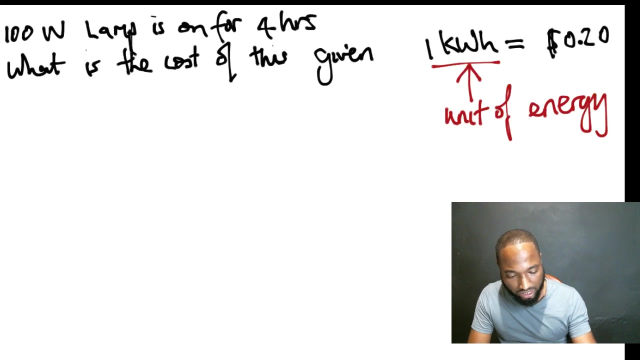 conversation right? yeah, that's 100 watts, so probably some people forget to do the conversion, so i'll do, you know. i'll add in one more novelty question: how many jewels in one kilo watt hour? how many jewels? so people look at 0.08 and don't understand. let's start with this question. 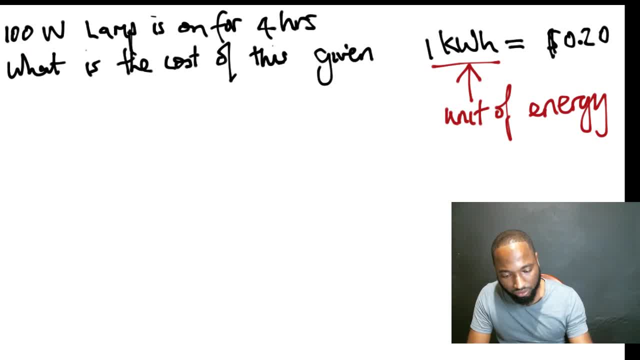 so 100 watt lamp is on for four hours immediately. you want to get energy right. energy is equal to now, we know, we know power, we are given power, this is power and we are given time and i give you the equation. with that, i say power is equal to energy. 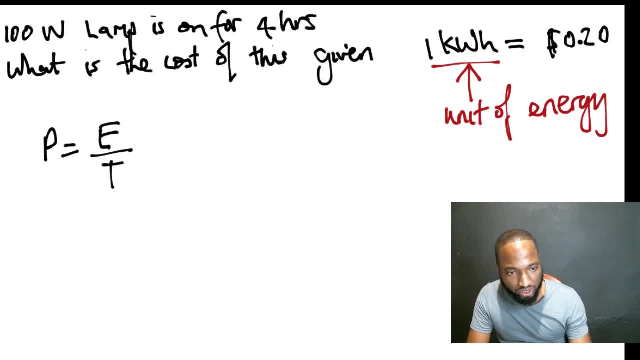 like that rate of change, of doing work, energy over time. so if i i want to find energy now and i want to find the energy in this unit, this is what i do: get rid of that t and bring that t up here. so i have this equation now. e is equal to p by t, where the power is 100 watts. 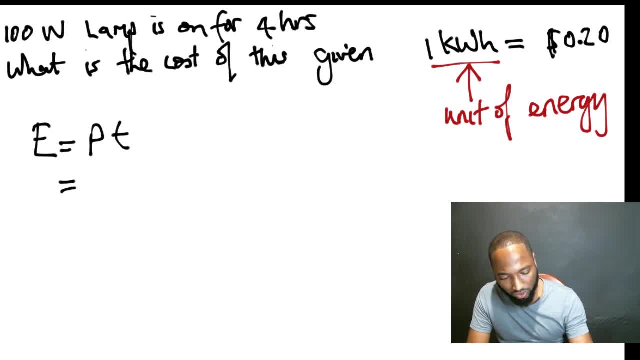 and what watts are kilowatts. so 100 watts is actually 0.1 kilowatt. multiply by the time, which is four watts, and i'll get something here. GIVE me 0.1, Sorry. 1 moyen: 0.2 1. 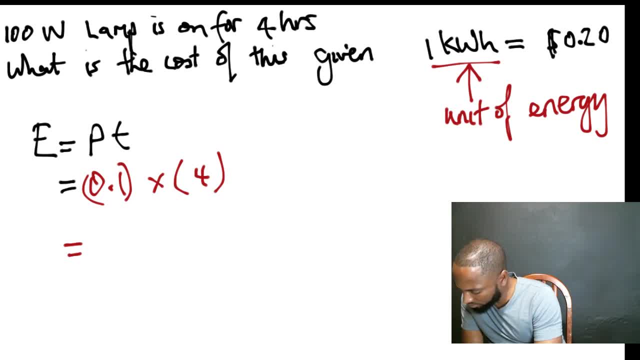 0.1. 1. 1. 1. 1. 1. 1. 3, 2, 3, 4, 16, 5 吃 7, 8, 7, 10, 11, 12, 18, 13, 12, 24, 29. 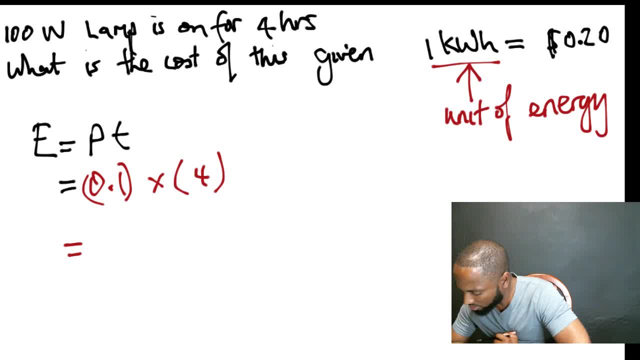 27, 33, 32, 33, 33, 4, 31, 8 05. No, this is correct. This is correct. Yeah, I'm correct And that's right. only wrong thing for the question, So they may have a different weekend. 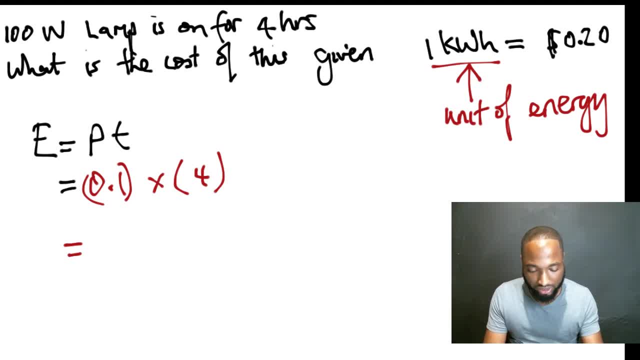 If you're following any book, they have a different weekend, but we'll get our own answer, So what's the answer here? So 0.8.. 0.08.. Yeah, yeah, yeah, My bad, my bad, my bad. 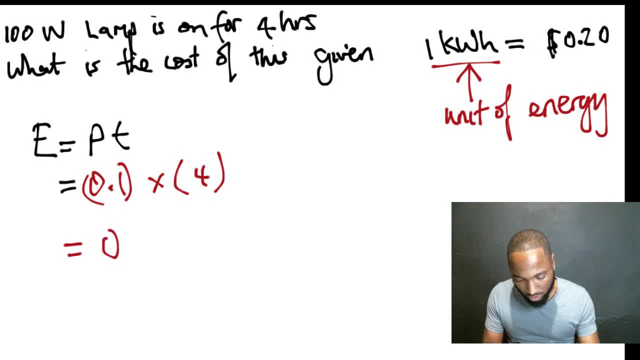 So I was judging all the answers ahead of time. So this is 0.4.. This is 0.4 kilowatt hour And And the cost? Well, the cost will be like All right, so at least we got an experience with this question. 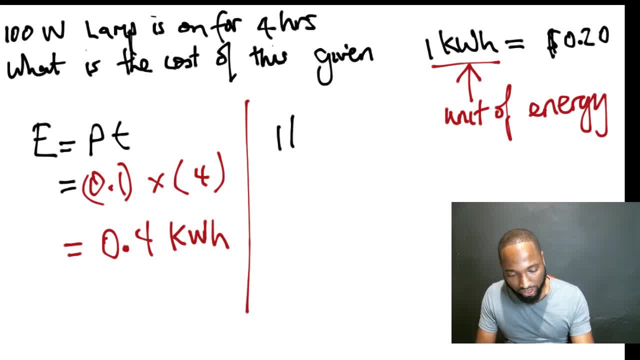 How will the cost be on this side when I finish? right, So I'll start off with: 1 kilowatt hour is equal to 0.2.. Therefore, 0.4 kilowatt hour is going to take this answer from me and pay it. 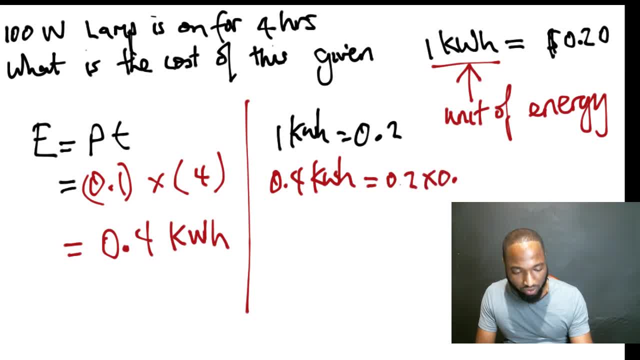 So I'll have to multiply 0.2 times 0.4.. So everybody, So everybody who gets your 0.08 was correct 0.08.. So I'll send to you guys: Yeah, so we're correct, we're correct, we're correct. 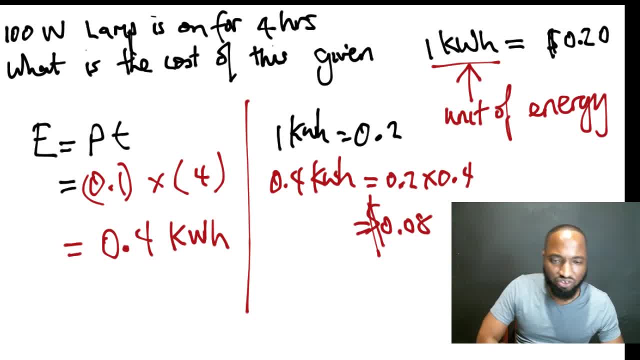 Now in the question, they had three. They had three light bulbs. That's why some people get a different answer, if you was watching the question. So we're good to go. What book is being used? This is a kind of new book. 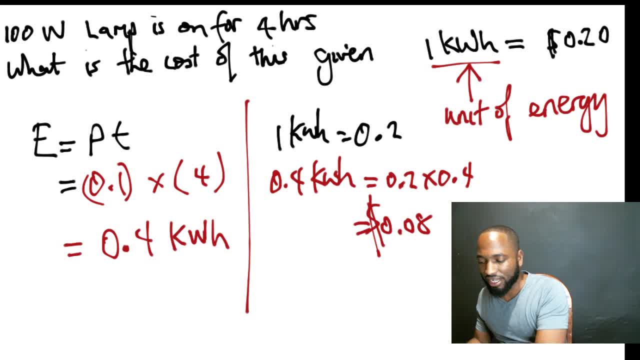 A book: Physics with C-Sec by Samuel Lallamany. Okay, The next book that's being used is this book. haven't I A GC book? And the next book that's being used? a lot of books are being used here. 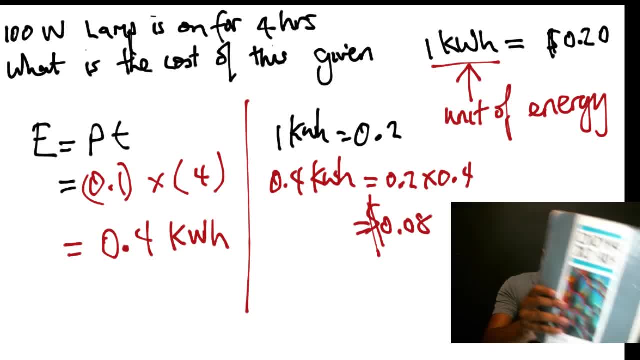 It's this book, But I'm not taking questions from this book. Most of the questions I'm not taking from this book, Right, And apparently I'm changing up some questions, So we're good there. Why is it in the chat? 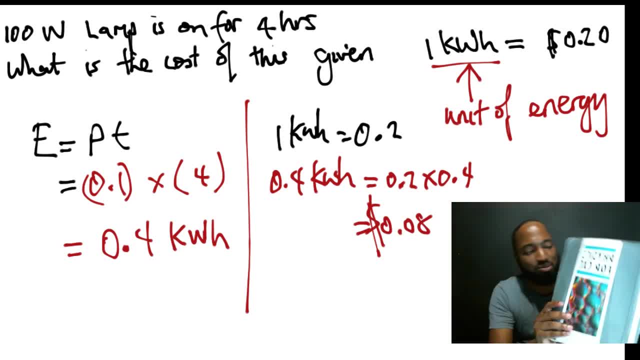 Now I won't say I don't like this book. It's all right, All right, But this is the best book for learning concepts in Physics. But most people wouldn't have this book because it's not. This is not CXC syllabus. 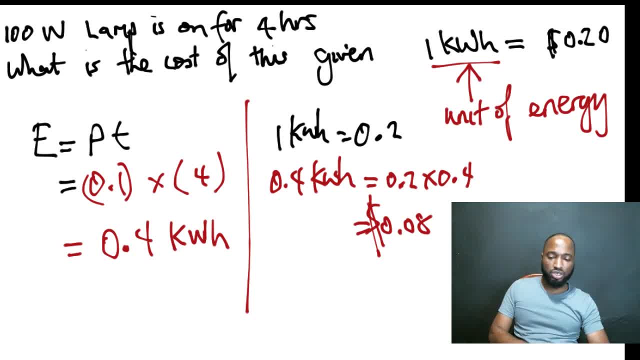 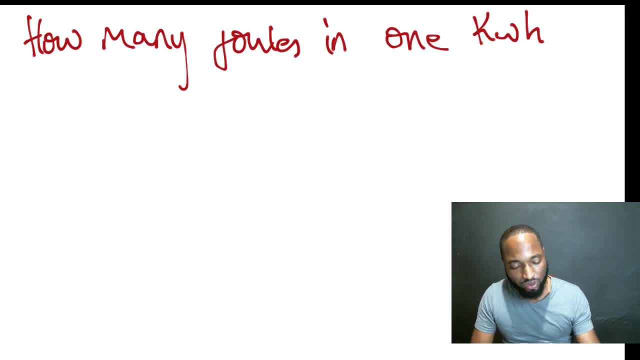 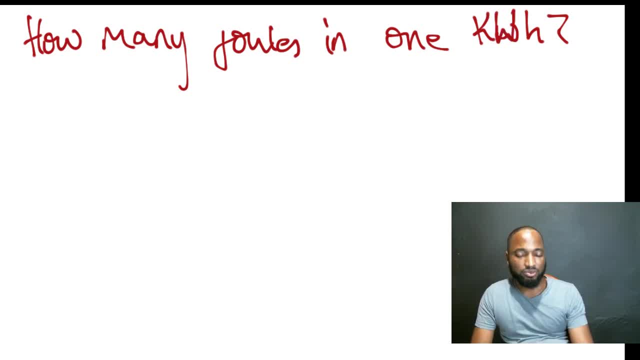 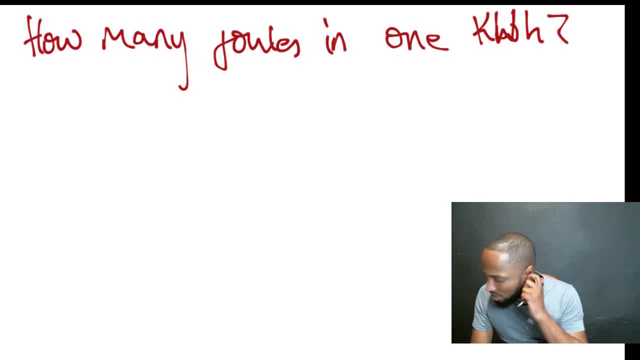 through or something: 3.6 megajoules. well, well done, well done, well done. injustice, injustice. you didn't see xc physics because i find your speeding brother. well, you had that question down. look, somebody say 3.6 j java- yeah, i know you, that's good. 3.6. nobody say a thousand. 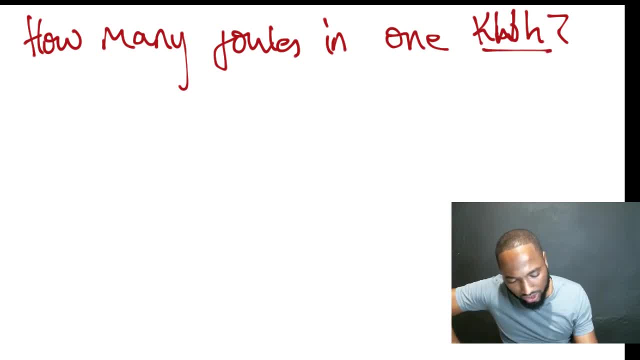 so how are we going to work this out? remember, kilowatt hour is a unit of energy, kilowatt hour. so this is how i would work this out. this stands for one thousand watts in the one hour, and we know that energy is. i always base this equation from this basic, from this power. 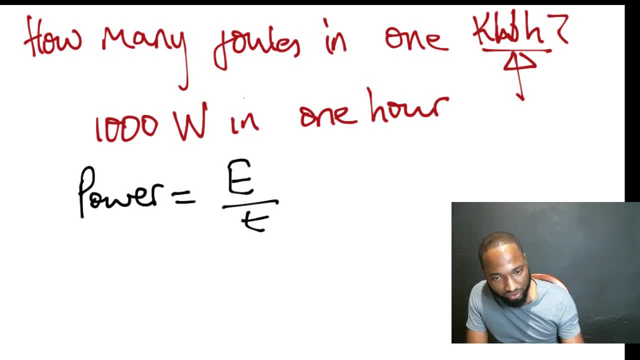 is energy over time right? rate of change of energy: right, right, right, right, right. so rather than you forget good answers there, go deep. what's up with that answer? my friend, you didn't see any mean attacks here. anyway, it's true, because i watched a lot of, and look where i am teaching multiple subjects on. 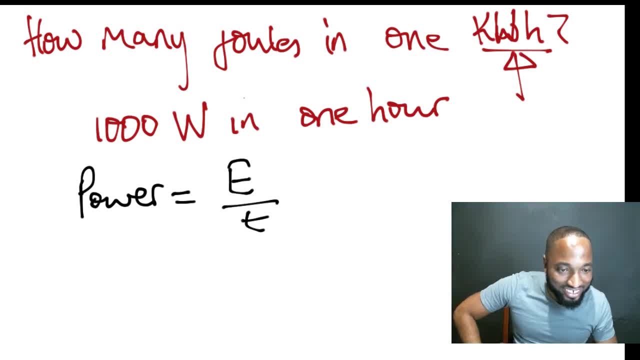 youtube, the keys are new, me, my fellows, all right, so let's just ignore some of those conversations. then i'm just here for nostalgia, all right, the brother gaffing, hold it down, let the nostalgia kick in. all right, so we have e, so let's just substitute in here now, um. 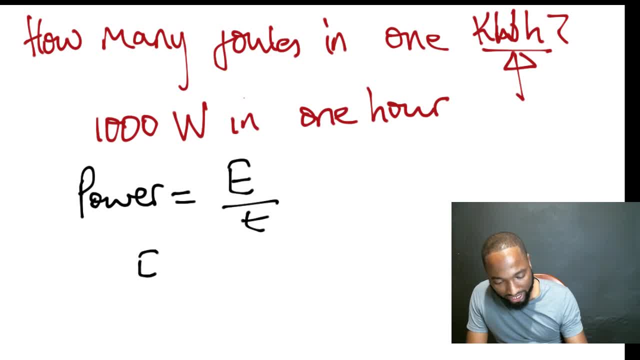 um, i'll put the e here and put the power by time, like this power, so you'll see what happened in here already. one thousand by one hour, we wait in seconds. so 60 by 60, this represents 60, 1 by 60 to get the minutes and then another 60 to get the seconds, and that's how, everybody getting 3.6. 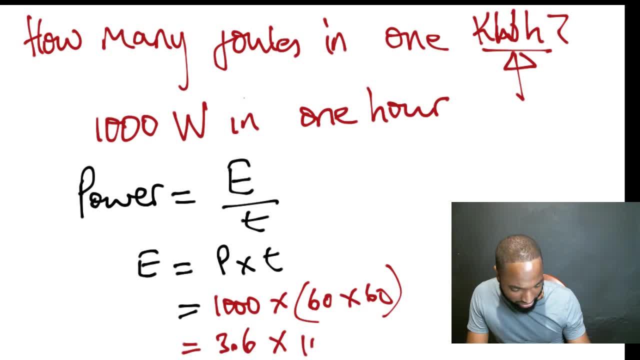 megabits. so that's 3.6 by 10 to the power of one, two, three, four, five and six by six will give me an answer in the 36. so it's six, right? three point six by ten to the power of six. so 36 by ten to the power of five which will turn. 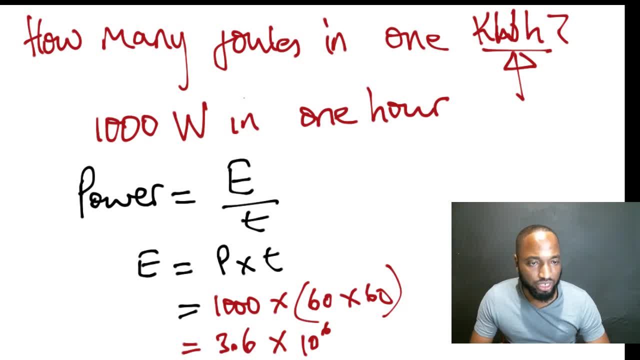 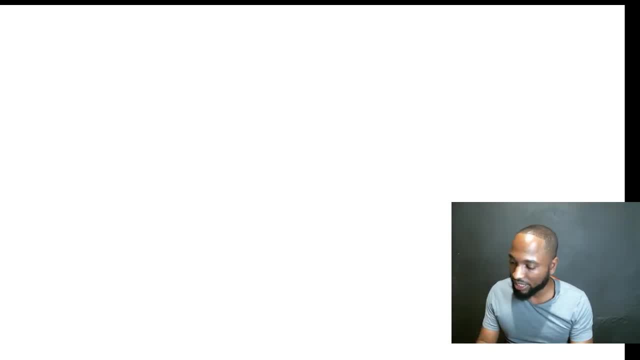 out to be three point six by ten to the power six. we good. all right, why is in the chat? and let's move on. everybody good there. we all talked about conserving energy. we talk about the use of fluorescent lamps instead of incandescent. we talk about using 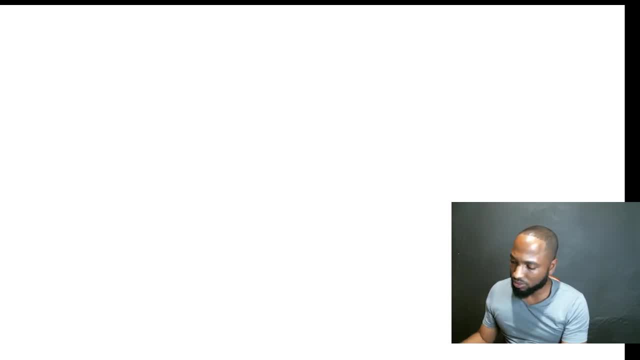 solar water heaters. we talk about turning off lights. we talk about using, instead of using, split units, use large air conditioning systems, right, all right, all right. some earlier- i see earlier all the time here and then always message my instagram and it's get problems to connect your instagram profile to who you. 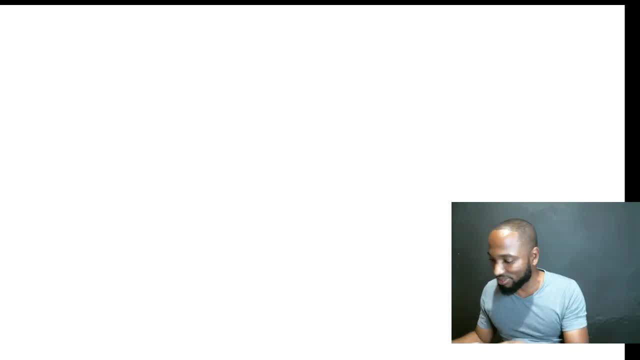 who is on youtube? right, who you are on youtube. let's move on to circuits and circuit components. i think that is it for me. let's move on to circuit and city components. um, i will draw something and you'll tell me what it is. what's this? 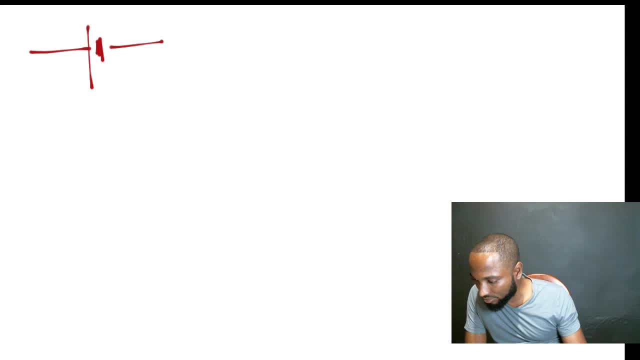 what's that? what does this represent? a man balling relevant. so this is one, two, three, choose yourself. um, what about this one? this is a one, two, three, four, four. two is not a switch. two represents ac supply, ac power supply. well done, pickle. um, okay, so let me train this. then what about this? 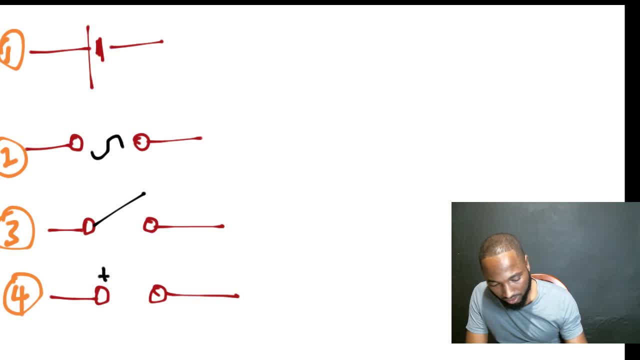 well then pickle? um okay, so let me train this. then what about this? um okay, so let me train this. then what about this? what about that? what is this? so just keep listing out alt as one and you could copy and paste a comment. you could copy and paste a comment and just add on a new one when you 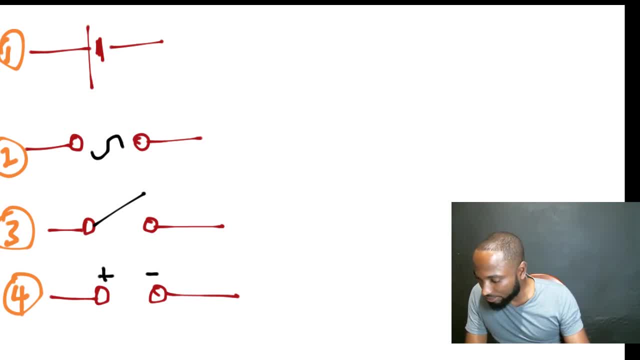 done tough when you get you for very on me on five. what is this? or sometimes it will run as this: what is this the difference? day seven, seven, fifth, is this, what's that? somebody say five, what it's? some people confuse, some people are confused. what is the difference between seven and eight? right? so let's name them off this. 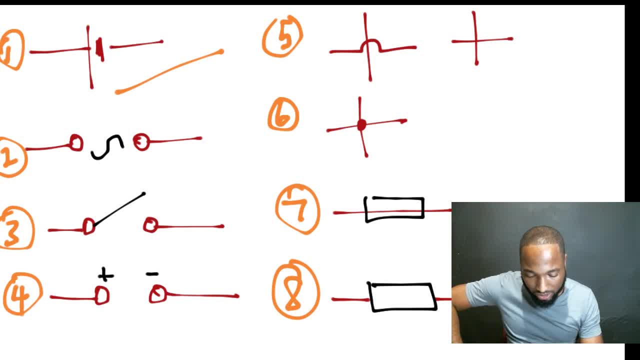 is a cell, right battery cell. this one is AC power supply. okay, AC power supply, this one is a cell cell, AC power supply switch, DC power supply. number four: wires, you know which night, number five, but they're not touching, just crossing over each other. but in the touching number six, these wires cross each other, but 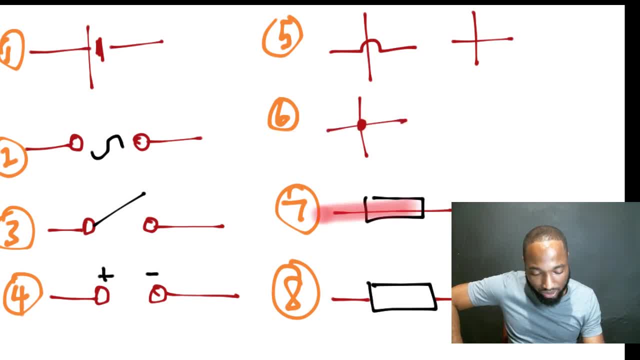 they're touched. an difference between seven. if this one of the fuse, the clearly see the wire going through here, right. so we call out on a fuse, but this one is up. what's this one I want is a resistor, but it's a fixed resistor. fixed resistor. and another, we even draw that. 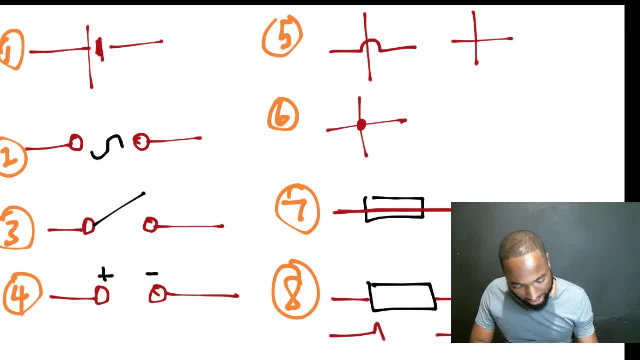 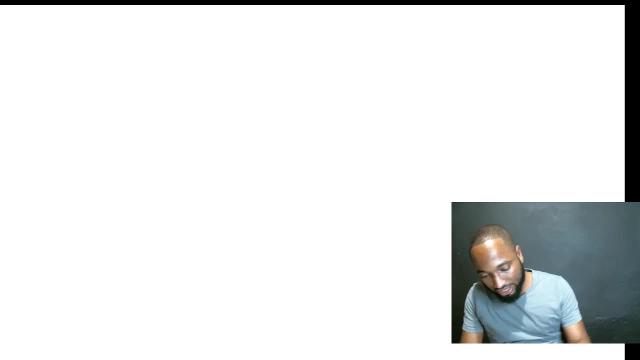 is the Spiegel's like this: yeah, that's the next week, enjoyed. all right, let's, let's do it. let's do our next set. one, two, three, five, six. let's do our next set of them. I'll join it with red. what about if I did this? what is this called? 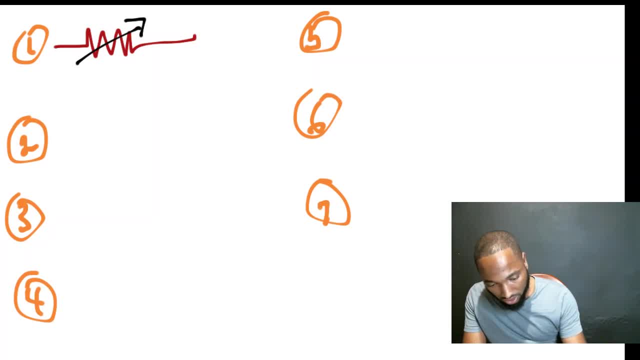 what's that? oh, oh, I could draw them. I can draw it like this in the box again: okay, okay, okay, okay, okay, okay, okay. I put the arrow across the box instead. then everybody knows what this is. if you don't know what this is, room they just. 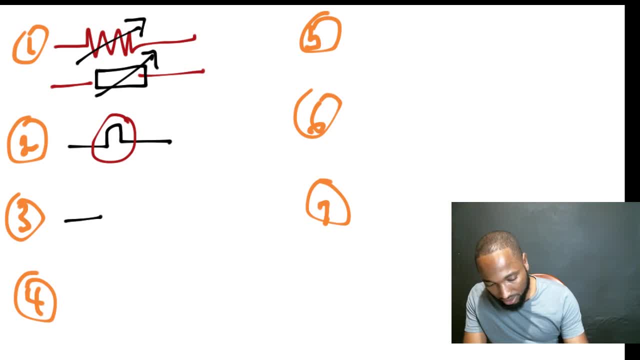 want final bent and beat yourself: what's that? hmm, mm-hmm, right, right. so yeah, Trudy, yeah, Trudy, press, I'll do too much numbers. so variable resistor light, light, filament light, actually filament lamp, filament lamp. it's actually a filament lamp, voltmeter, ammeter and a diode, and it's. 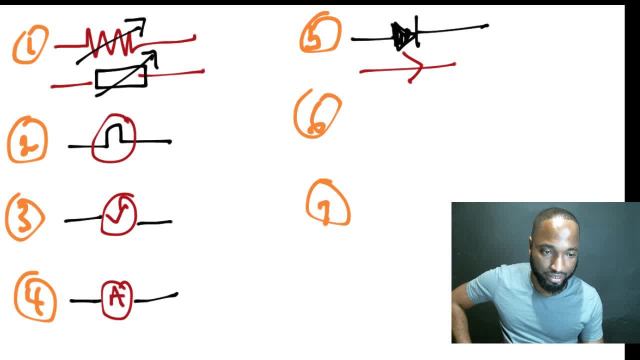 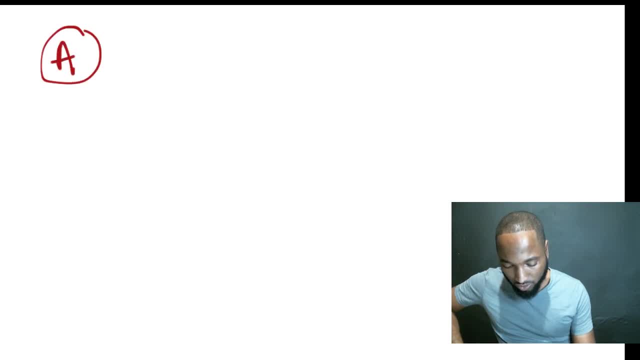 pointing any direction to allow that the current is allowed to pass. okay, all right. it's important to know that one of these is connected in series. I want to be is connected parallel, so which way does it go? which one, which one? which one is it, so which one is? 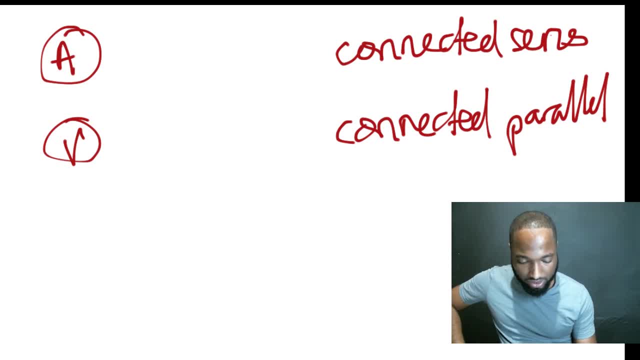 connected in series, I will turn it connected in parallel. so the ammeter is in series and the voltmeter is connected in parallel. but if we'll meet, I have a high resistance in it. right, the voltmeter has a very high resistance and if you connect it in series, 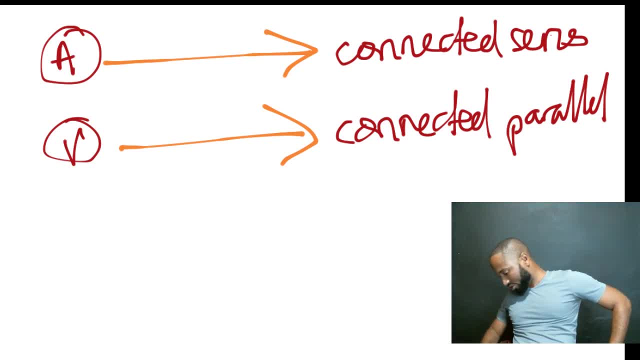 you'll cut your whole circuit, your circuit will be dead right and you want to connect the ammeter in series so that you can measure the entire current, so that it doesn't split the current. if you put the ammeter in parallel, part of the current will go to the ammeter and part will escape somewhere. so the ammeter 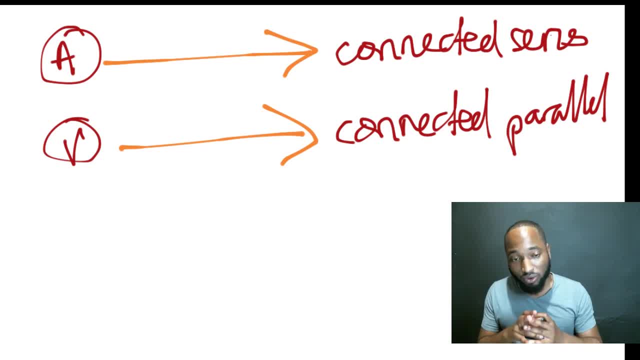 wouldn't give you the real reading for the current for the whole circuit. so wherever you want to get the whole current, you need to put the ammeter on that whole part of the of the- excuse me- circuit. let's draw a cell. and well, I'm not gonna draw a cell. drawing a cell will be kind of hard to do. you see how hard it. 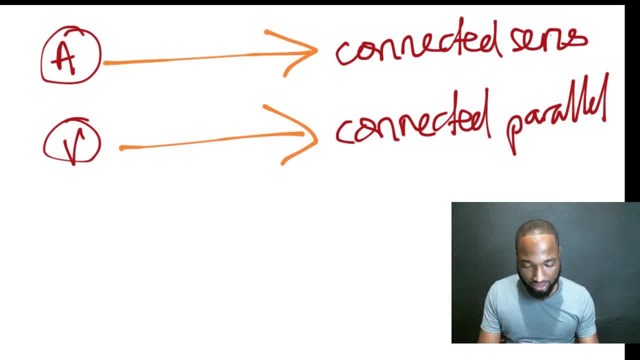 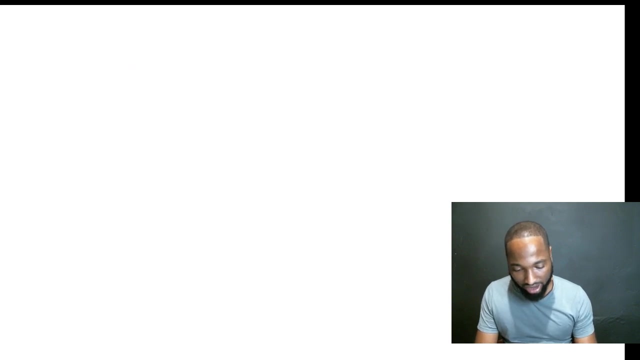 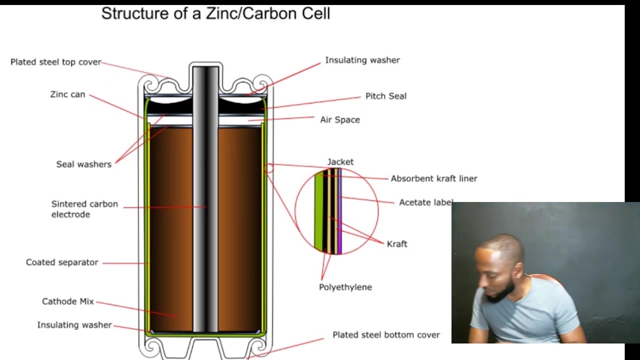 is me to draw these things. so we're gonna pull out a cell, we're gonna talk about it. yes, battery cell. why this man is? why spare me a better, spare me. but so this went into great detail. that we do really need to point too. but I like the diagram. the diagram is very nice, so I'm gonna shade some parts. 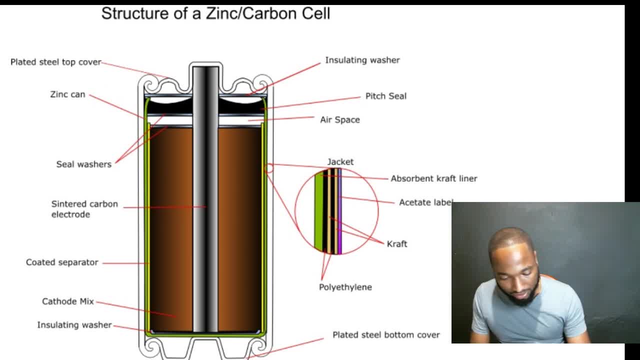 I'm gonna shade some parts that I need to be able to leave them. this is a zinc carbon cell. which side is the negative? which side is the positive? top or bottom, which side is the negative? which side is the positive? we come into all them thing with transform and all kind of thing. don't worry, all this cell, this song in 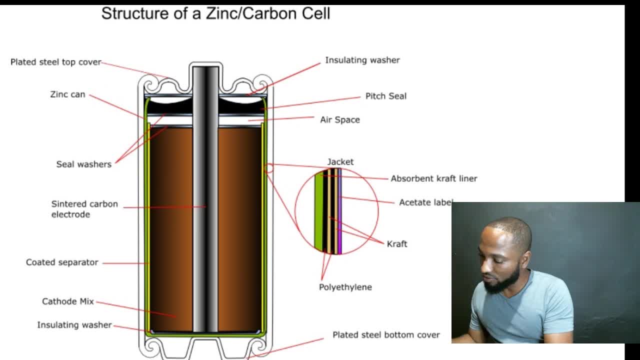 a kind of worried when I reach out. good, good, good, we already have a good, good, good way to go out. I would say: reach about halfway, reach about halfway. so the top is positive, bottom is negative. where is the electrolyte located? where's the electrolyte located? if I was you act like before the exam I had 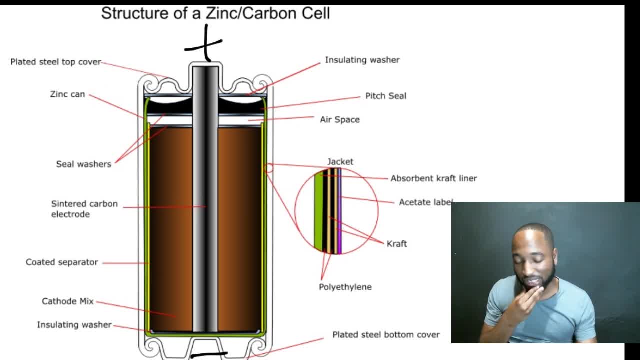 draw one of this, so maybe tomorrow, tomorrow anybody will take a time and just draw this battery cell from a textbook- the one I need to draw- from a textbook so you can label everything, take a time and write. it will only take about 15 minutes to make sure you have this, just in case I'd better talk about. 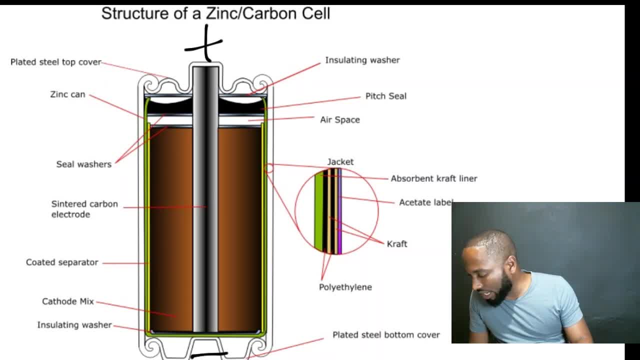 prepared on that. okay, right, so the electrolyte is, it is the brown. very good, we call this. what do we call this? this spot here is the carbon, right, the carbon electrode. and where's the zinc? where is the zinc? the zinc is on the can itself. not any protection, it not on this arm. 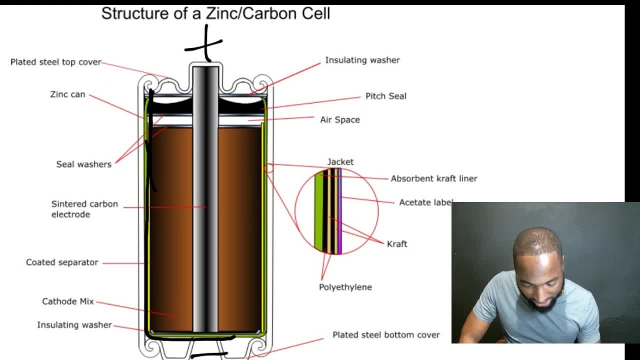 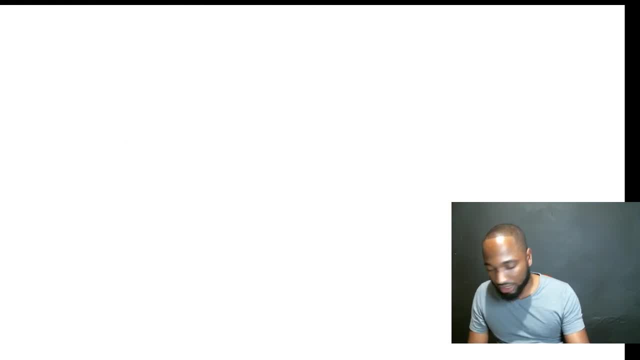 not only set. you think that separate it. here the zinc is on the can itself and it's on the can itself. so let's talk about. let's talk about it, talk about the zinc, talk about the carbon or talk about electrolyte- all these things in to be able to talk about the separator. none of this coming just. 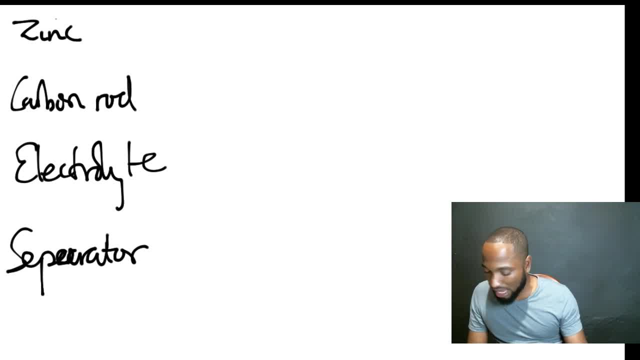 for kicks, the seal, the jacket and the conductor are doing the multiple choice for everything, but it's not multiple choice timing your contacts so is using the positive or the negative electrode, which one is the negative electrode, which negative electrode, which one is the positive electrode? so you can do SHC. 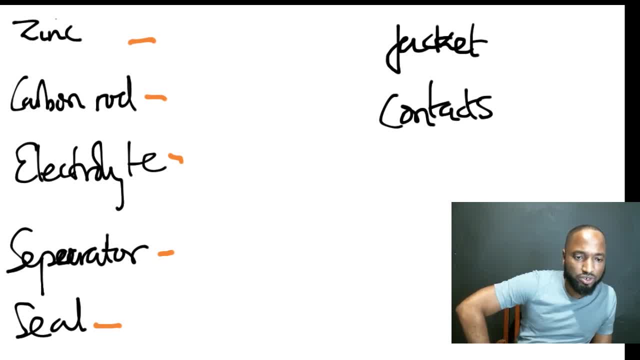 where's SHC? so you didn't have multiple choice. yet some dumb student told you you're a good idea to cheat and see like C math. sure don't blame the whole school. don't blame the whole school. there's one man we call that boss. there's a lot of students actually. 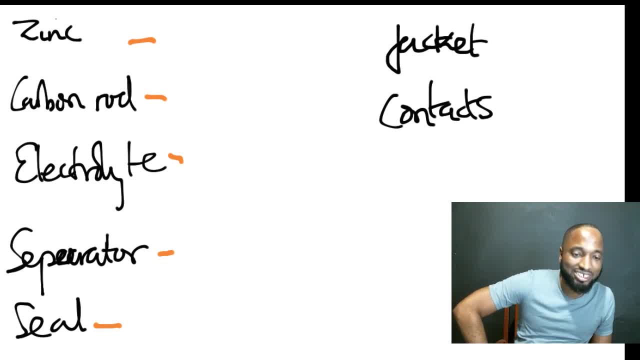 but not like the whole school. some dumb students, not the whole school. don't kill off the whole school. a shiny school had good students, just like you as well. the zinc is the negative, so the zinc is the anode, and you should remember from Kennedy and with is the negative electrode and the carbon would be the 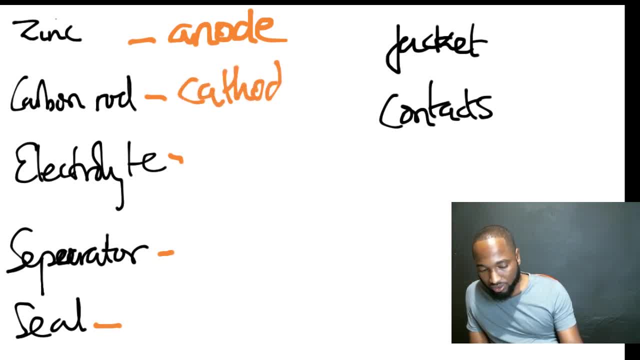 cattle. right, so you know the carbon is the electrode in the center. I'm going straight up. so does it cut to that? the positive side? that's why it goes straight up here, right? what would you lecture like with the electrolytes? just remember this ammonium chloride and you don't need to remember the chemistry of it, just 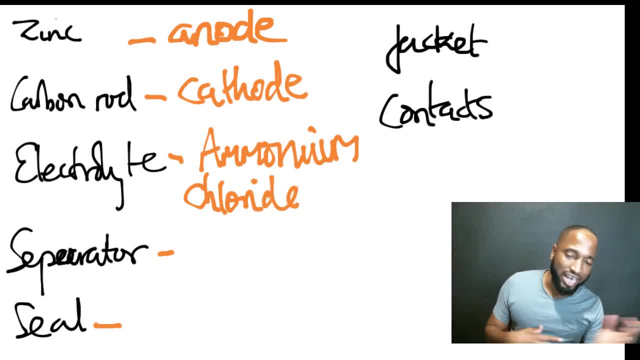 remember that it causes the ions to move again. it promotes a reaction that causes the animal. somebody said, no, cathode is negative and anode is positive. no, that is not correct. what anyway? yeah, take a better response myself, but I am good to be cattled. 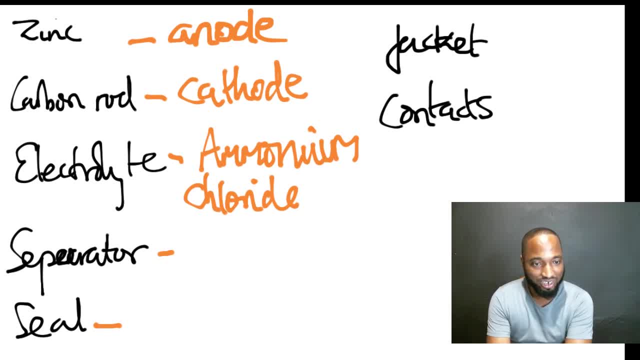 yes, katya, go to the cartoon the jacket and a nasty puppy. right, yes, yes, yes, yes, yes, you will chat jumped on. many are just watching much at explode on top of my she. i will watch my chat explode on top of my. She is a great girl. 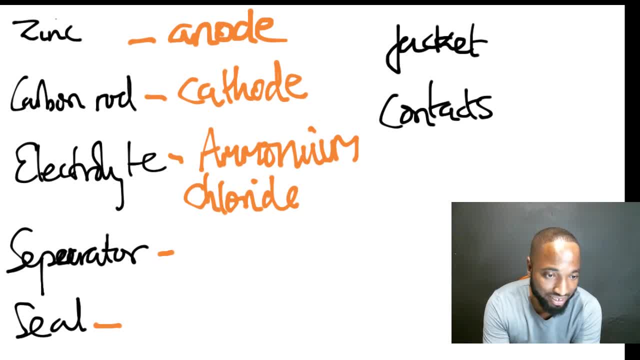 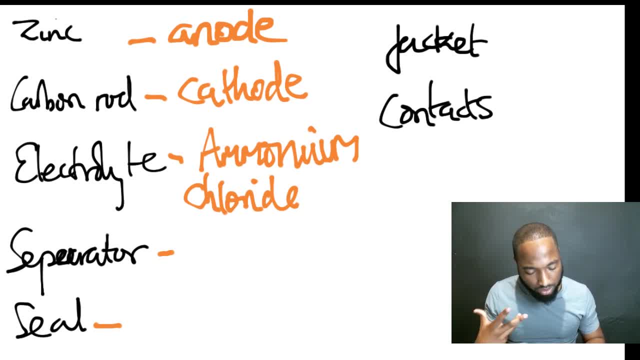 can I get to attractive positive right, yeah, okay, cut, I'll go to the cut out to the capital has to be negative and I am go to the anotomy and it has to be positive, if you like no people. you said the other is negative. I said the other is negative. that's what is negative. we. 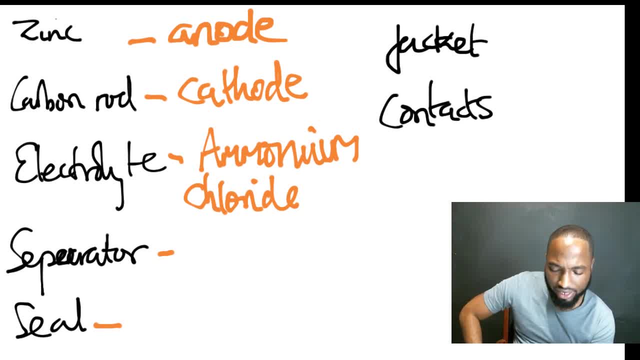 charge and attracts nothing. right, but the other here right. it's not not the anotomy, this is not the another theory, even though the anode here is negative. even though the anode here is negative, sorry, it leads to the negative pool on the battery. you negative spot on the. 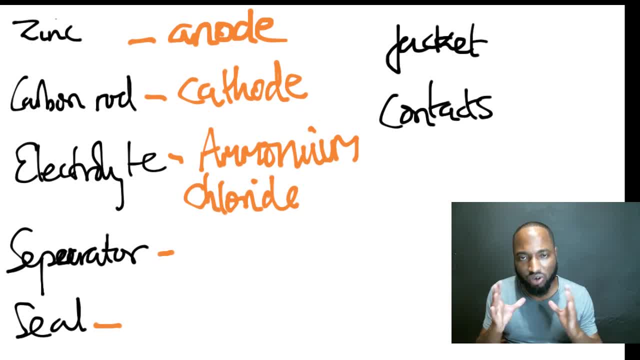 battery. right, so we know the the tinted ground lesson. this in chemistry and physics is that any cuts ions have a negative trial by инструмент. right, so they do. there is no yellow, there is no vertigo means Because this Consumer and� go to the cathode, the anions go to the anode. 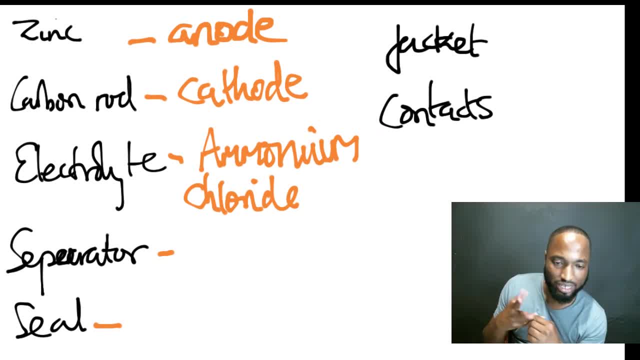 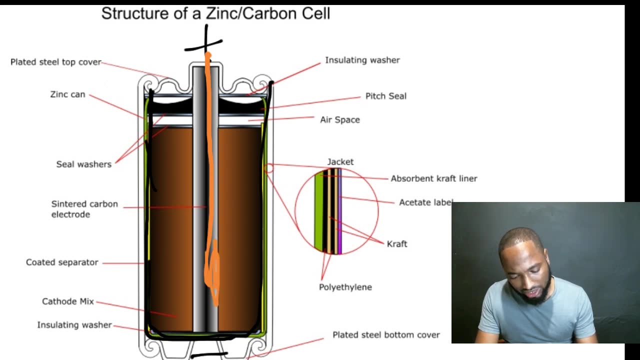 and that will let you know what happened. right, for cations to go to the cathode, the cathode has to be negatively charged. right, that's great. but in this, here, in the battery, the cathode, the what I want to say. 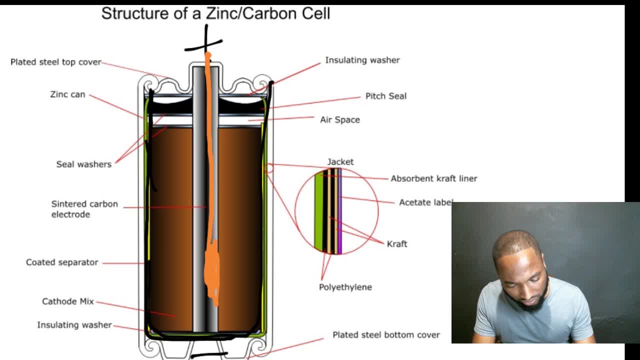 the. I lost my train of thought. this here is the positive pole, although this carbon here represents the cathode, although the carbon represents the cathode and is negative, this here leads to the positive pole. understand what I'm trying to say. oppositely charged, yeah. 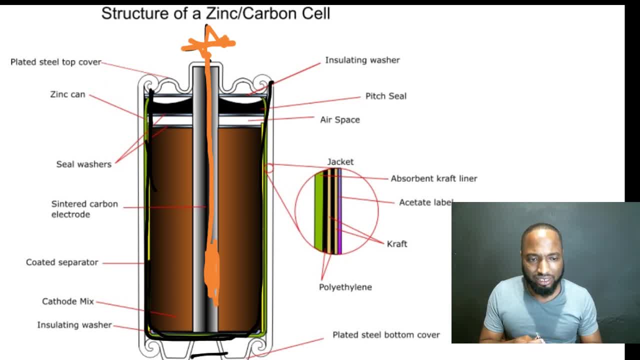 so, so that is that. so run this, go to transformers. alright, let me not waste no more time on this. I'm not too sure this is the syllabus. let me just take a little look. let me just take a little look, just see if I can explain everything on the syllabus. 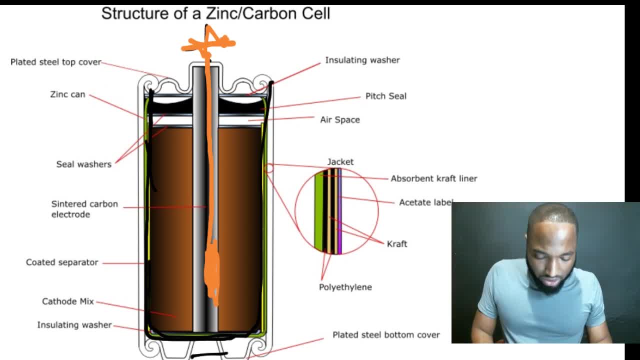 where this is concerned. just checking guys. okay, it looks like an XOD syllabus, right. so I'm scrolling through here looking for this, looking for this, these batteries on the syllabus. I'm not really seeing that I'm and just want me to reach transformers. we come. 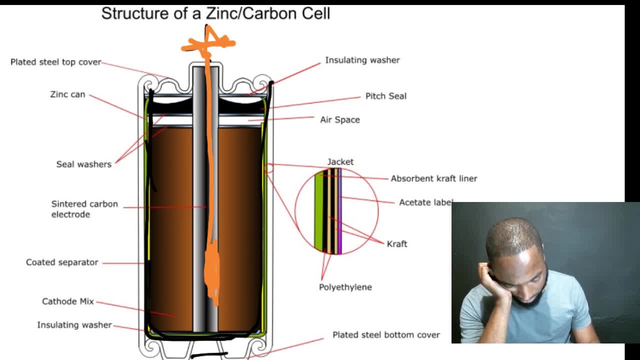 into transformers. we're going to every relationship now, that's the district, the parts of the cell, and mention y'all. it's on your syllabus, it's on the syllabus, but I think we mentioned everything we need to do, the functions of each of the thing. no, we didn't mention the function of the separator, the silly jacket, so I 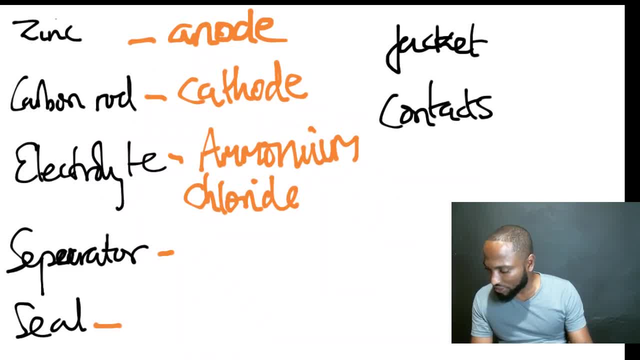 just quickly mention it. so the separator is a gel piece. it's separate the anode from the cathode. yeah, I separate the anode from the cathode and separate the anode from the cathode and separate the anode from the cathode. but it allows ionic conduction for the ions and electrolytes, right. but 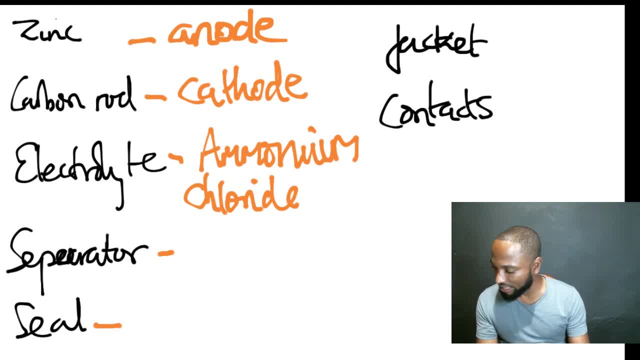 it separates them and the seal stops evaporation from occurring. I'm and say: battery is nice. I seen people falling off the life. the seals stops evaporation from occurring. the separator separates the anode and the cathode but it allows conduction across the. it allows an a conduction to the accrue. the seal stops evaporation. so 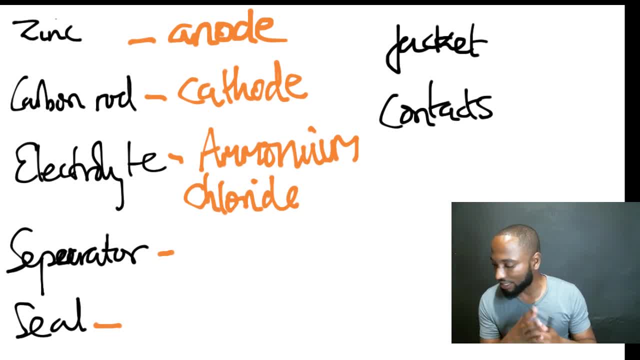 electrolytes to dissipate, because China is a piece and the jacket is just restrained and contacts, there's the terminals, any battery, right. so the key word here: the separator separates step. are we done with this? separates, but it allows an ik conduction it. he would. he has prevent evaporation. prevent evaporation with the jackets. 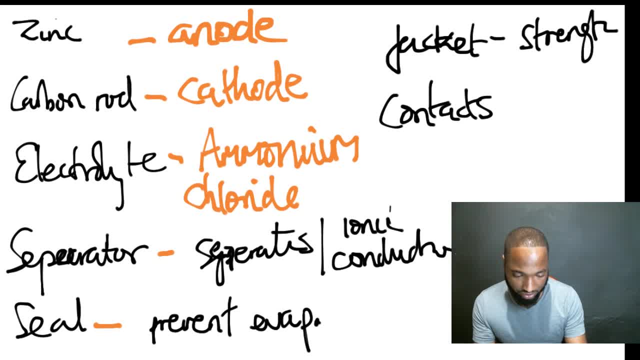 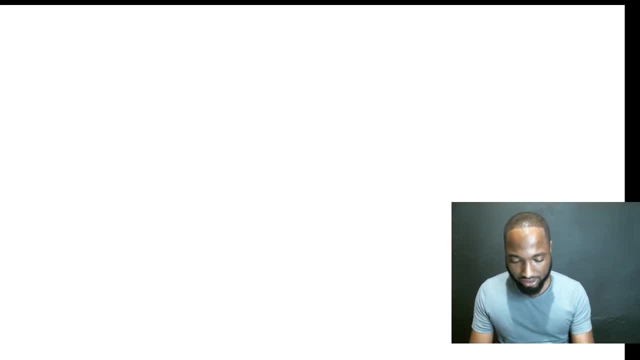 this is for strength and the contacts. these are just two minutes wise in the chat if you ready to move on. there was the difference between primary and secondary cells. you, I've seen some ends- all right for the people who have ends many people love. and just one: check the diagram and I'm practicing text. you batteries, no primary. 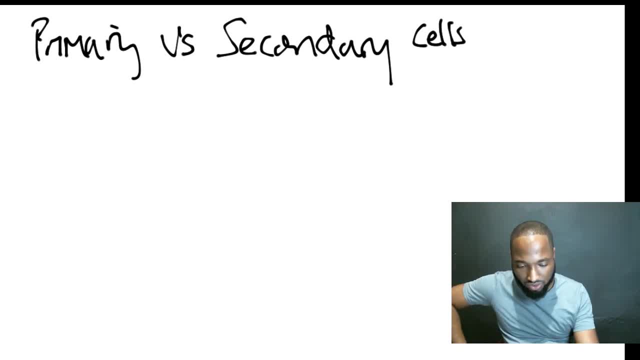 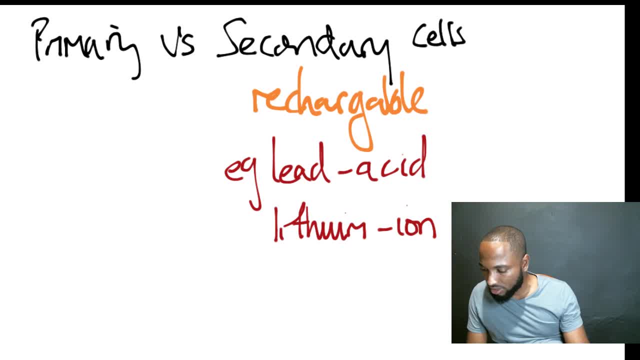 litium, an examples of primary cells, disposable batteries, but you just draw one of just right using cab on. okay, all right, so ready to go there now is these kind of things you don't want to overlook when you're revising and you're trying to get one, and we're trying to. 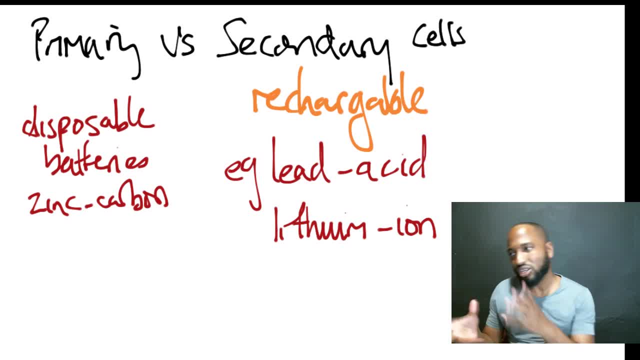 get your merit away, all is so. you revise all your calculations, I think, and you just kind of overlook these things. you want to make sure because it's the little one, mark hunting, I own loss, obviously this: we get the definition of primary and secondary cells. if you just forget your examples, the terminal thing is: 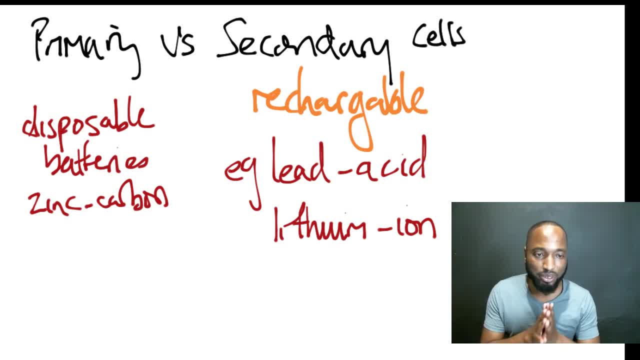 let's take away a little max. I'm making a shine. shine for the people, gonna shine for the people. like mercury oxide, we charging. you can get a question on charging a cell. you just need to know how to use the same formulas from before. all right, let's do a question. we're gonna involve resistance in it by the 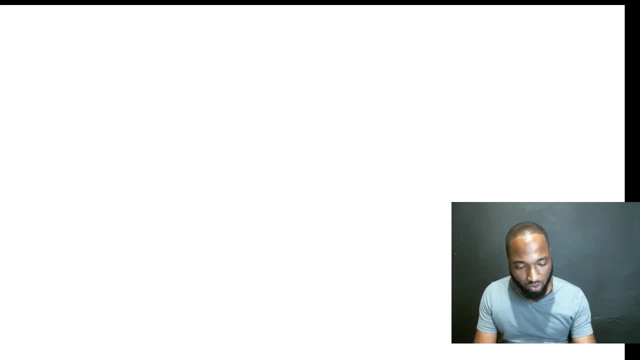 way. what is Ohm's law? let's go on into resistance. Ohm's, not Ohm's law in the chat right now, please, Ohm's law. what is Ohm's law? 920, so we may finish all of this at around 11 o'clock, or 1130 was Ohm's law, Ohm's law. 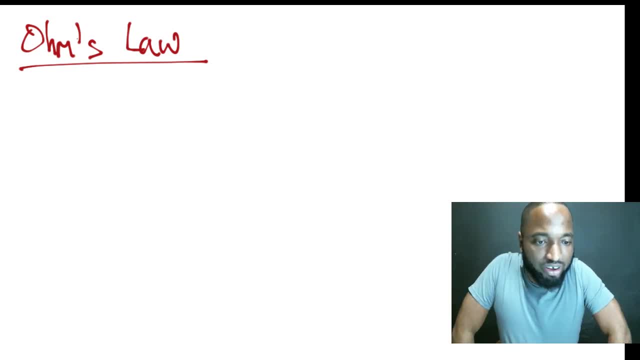 say that the current through a conductor between two points is directly proportional to the voltage across the right. so we Ohm's law know your Ohm's law. people seen it there wasn't to know what is our only conductor. was that only conductor? very straightforward to answer. 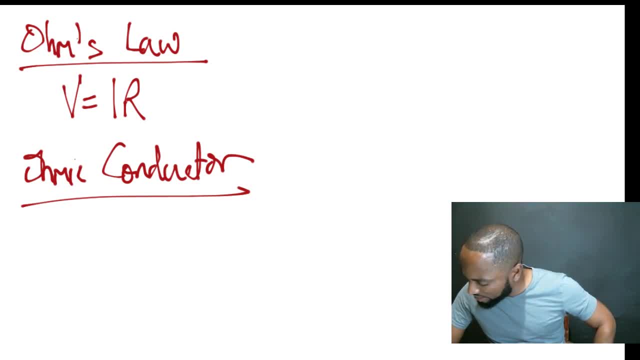 this question. what else? by what else? what else? somebody saying 11, you wanna go all night? oh, that's I sleep and download this video tomorrow. now step and get one time to procrastinate. step and get one time. so if you just put the formula, you will get the correct. no partner. this is. 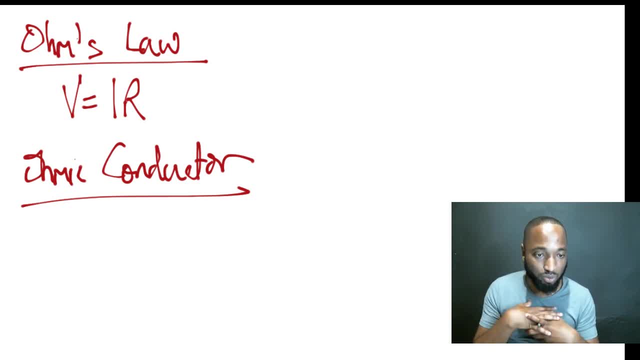 the right definition for Ohm's law. you better write a definition for Ohm's law. sleep is for the weak, your rest is for the dead. explain: community commutator and logic gates. you come into that, all your horses, my brother, money, logic gates part. yeah, we come into that. come into everything we're gonna do, every single. 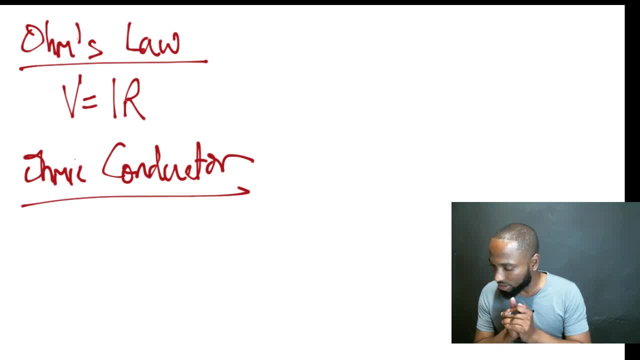 thing in electricity and magnetism, right. so when I've done this video on electricity and magnetism, I've done everything I can tell people just go and check that video when they have physics on Monday, all right. so I think I think I could probably hit a. 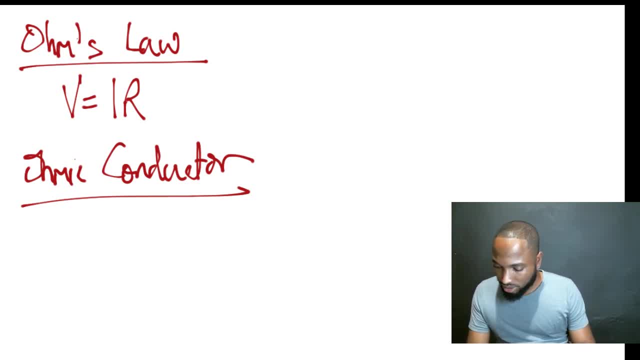 little question. I'll read all the question please now that easy, not easy, not easy, but we'll do some questions when you come across this series and parallel. so you must know a little diagram. you'll see diagrams of filament labs diagram. so, oh my god, oh my. 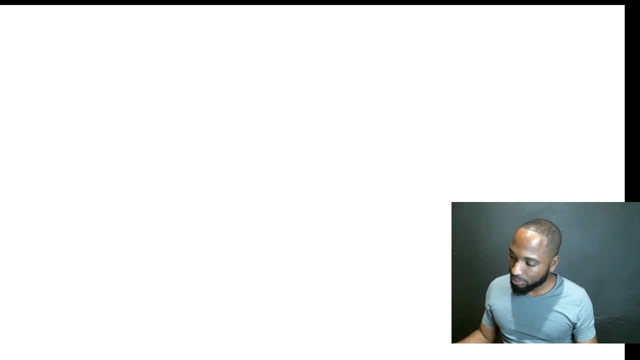 conduct stuff like that copper sulfide solutions facing solution and do this one right of the speed, дети. copper sulfide solution. this is a current. this is their roots, why they are species. when you have your copper sulfate solution, mayhem back. yeah, all right, explain. 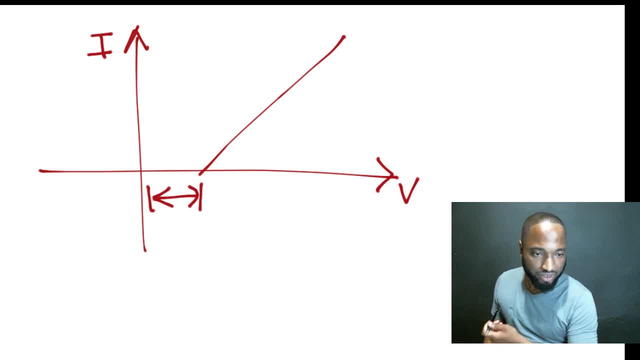 tomorrow is no physics. physics is money. so this is: this is like a cup of salt. this is like a cup of salt solution. you know. only conductor is like this. this is the IV diagram. say what we call the IV diagrams. this need to pass through zero and you know your filament lab. I think. 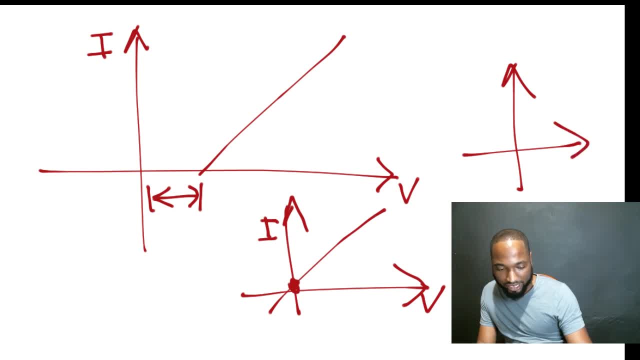 that's what I need to know. the filament lamp will be like this and then cool down like that right filament lamp looks like that and there's also a back in the filament lamp to do this if you use a nervous voltage. we didn't have this little part. here is 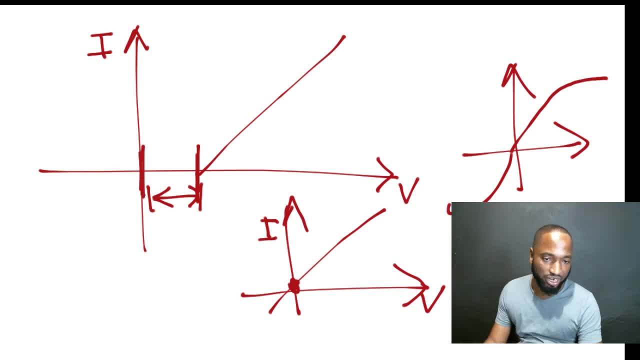 because they need to overcomes. you need to overcome my EMF, it's right, but I don't think you need to explain, I'm sexy. so after your voltage reaches a certain level is only after across a certain threshold level in your circuit. you need to overcome the EMF first. so after your voltage reaches a certain level is only after across a certain threshold level in. 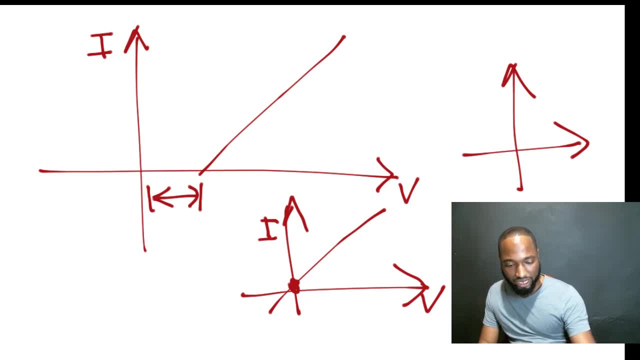 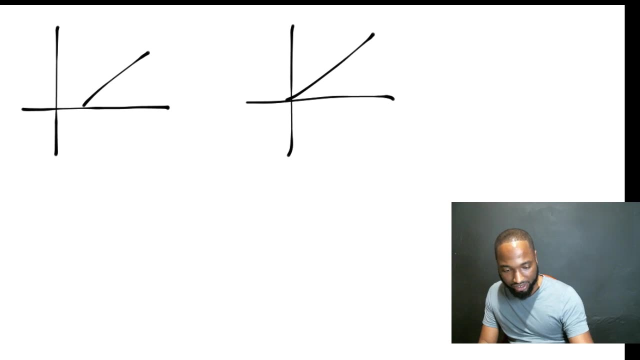 your voltage current. it's that of me. so once again, I'll just draw them very quickly here. I'll write in black now all of them and you will tell me which one is which. there's this kind. there's this kind. there is this kind. there is there's. 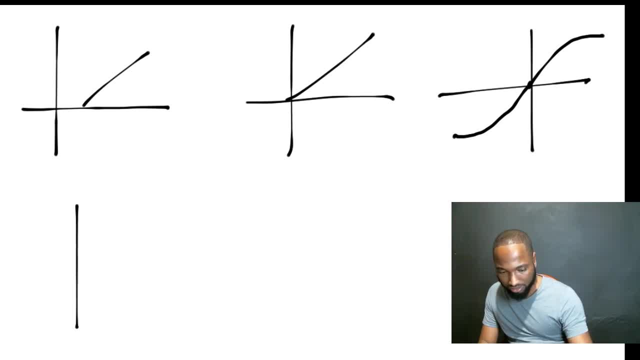 this kind and this one, so that you're at the ready, ready. what there's all of these is IV diagrams. this person, you, this one, goes like that. so one, two, three, four. one, two, three, four. chat answers in the chat label: each of those IV diagrams there- and by IV I mean current, against. 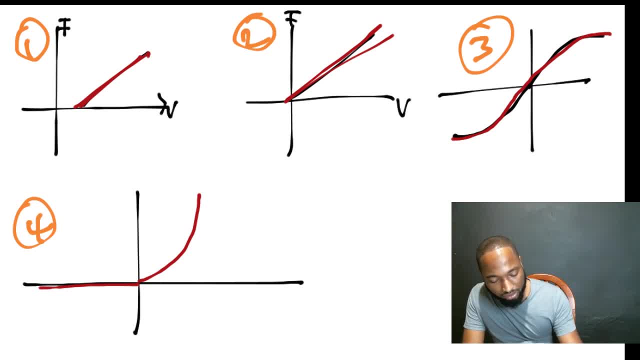 voltage IV diagrams. this goes, this could go down, so to that you know what you write on it and yes, yeah. so for is a diode, one is the annex solution. two is of a metal wire, only conductor, only conduct. so everysi guy are the most powerful hummer혹. yes, so four is a diode, one is 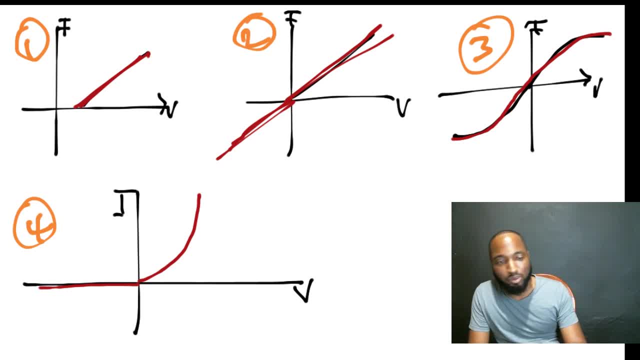 the audit. solution two is a metal wire, oh소 l burden on the condut and treat is now channel. so everybody, you have that, they don't. it's inmy chat. I said oh, I said also don't know it, you don't know it, you lost the math right and you need to study on. 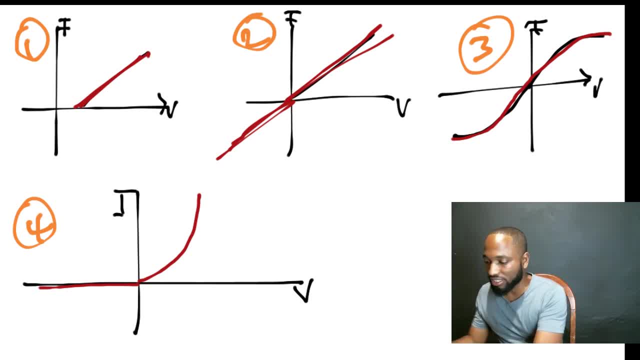 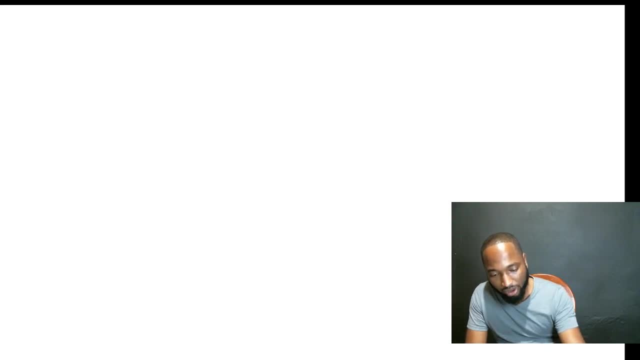 how to do the hard stuff. the calculations make sure you can do easy stuff right. so let's prove, let's um resistance in parallel versus resistance. and look, we reach here, boys, we reach here. so we know resistance in series. give me the formula for resistance in series. 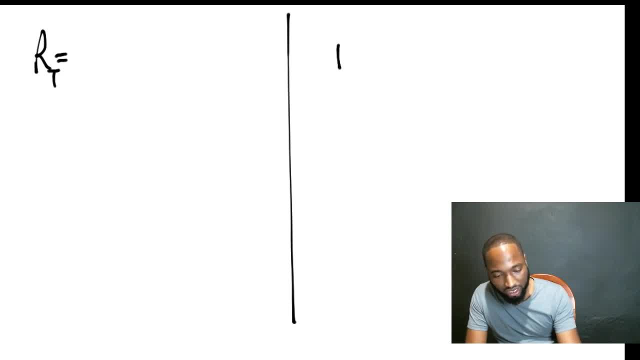 and we normally use t here- and then give me the formula for resistance in parallel, formula for resistance in series, formula for resistance in parallel. can i have them please? all right, hey, hey, somebody's saying something crazy in the chat there. this one is the series, this one is the parallel. 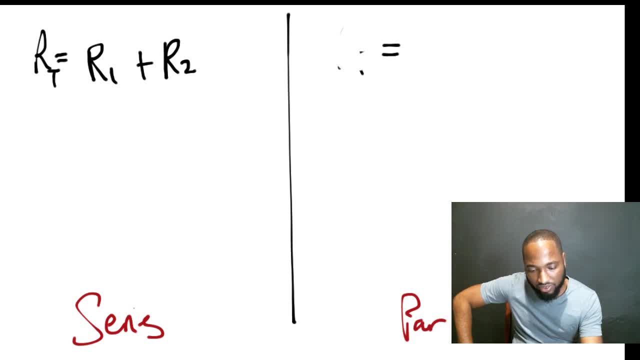 right. so in power, in parallel, you have this situation taking place and then you end up with that and a divide thing, and then you end up with that and a divide thing. i'm adding the multiplying. now sometimes you can have true resistance because that tree. you know what to do. 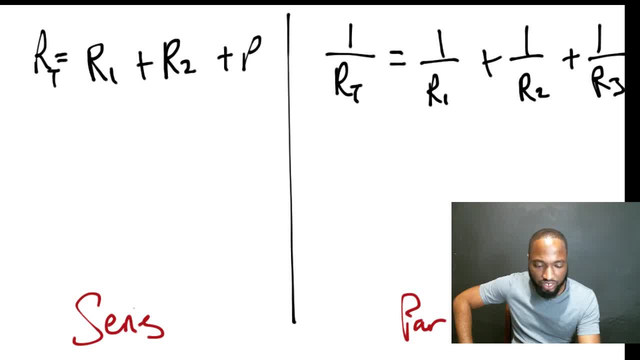 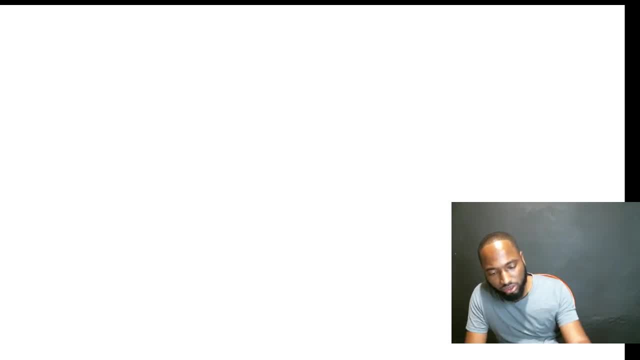 see what, say what. so that's really just add on. yeah, you kinda need to have an idea of how it came about. how it came about. who knows you, maybe acts didn't like a question one. that would be a real nice question one for them to bring, like when they show you it and you can't. 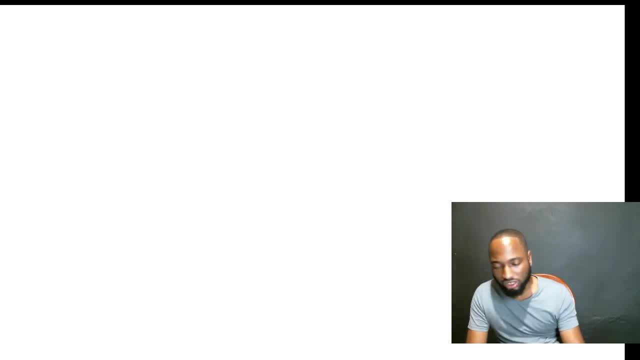 break it down and figure out how it come about. so it comes about because we difficult what adds to what. so, all right, let's start off any series. so in a series of it, let us drop a series of it here and I'll just be the two items, as I said, 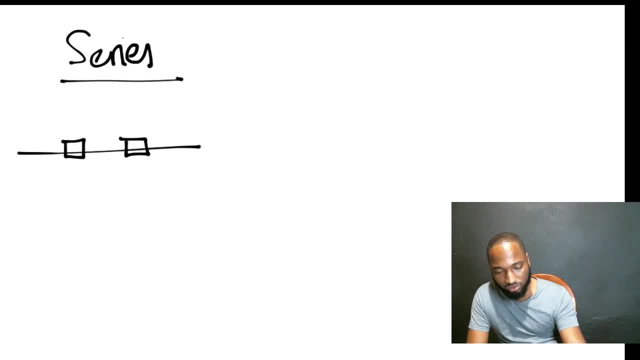 they could have true sisters. all right, you've hold it. here you call that v1 voltage. here we call that v2 and the entire voltage. maybe I should put that in different colors. pay attention, this is very important. v1- all I've seen lots of people going to see. I saw more energy done. all your boy first. well, these who? 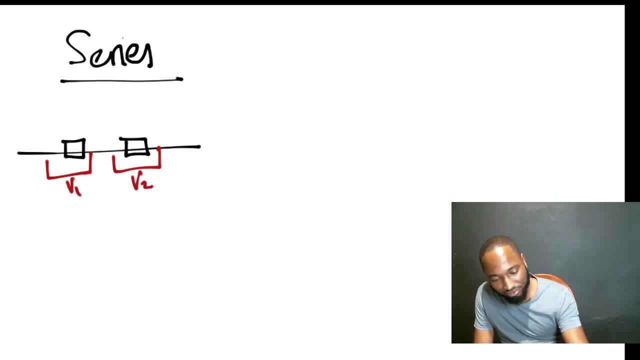 stay in here, but as? how much energy than some of the other, and that shouldn't be because I'm going to sleep. I saw more energy than some of the other, and that shouldn't be. that shouldn't be because I'm going to sleep. I saw more energy than some of the other, and that shouldn't be because I'm 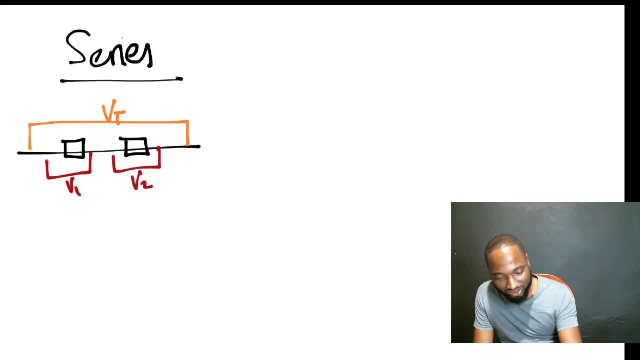 I'm a. I just hit 30 someone here. you're supposed to be able to grind man. so VT is equal to V 1 plus V 2, because in series you add the voltages, because you can think of it like a waterfall: you put on one bump, then you go to the next bump. 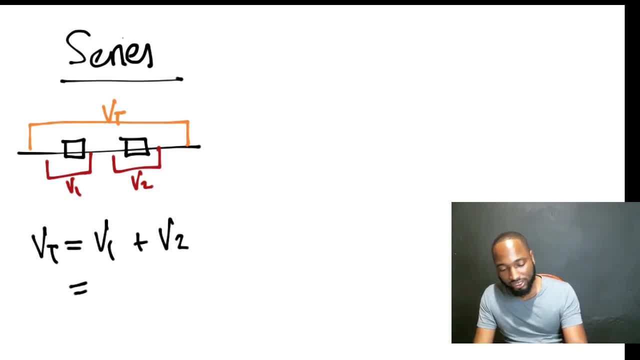 it's losing energy. no idea. substitute with this number. V is equal to IR plus iron plus IR 2. this V here is the same as I are the total resistance. but if you notice, you have I here, I have I here, so you can factorize all the I. why is in? 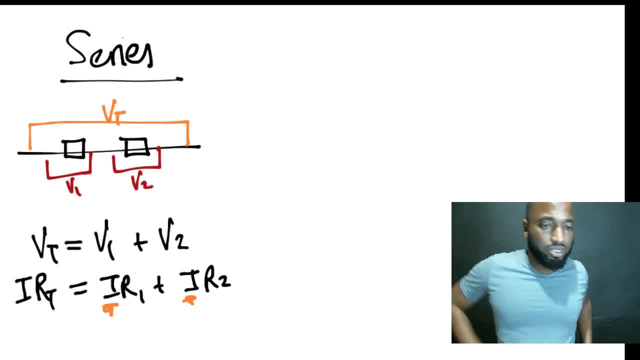 the chat of this making sense for the chemistry exam. I write my name in the school name section. I was so excited all right now. the reason why eyes you know have like I wanna I to here is because the current in series is the same trot. current is the same trolley. 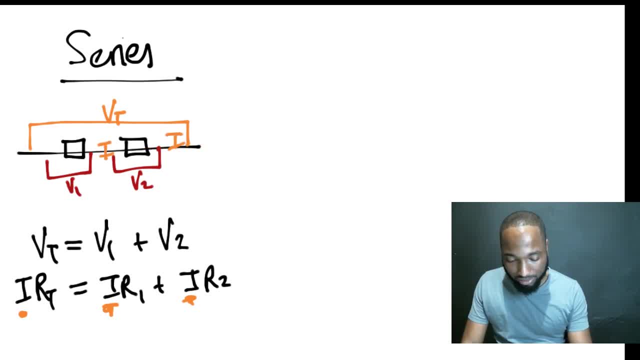 series. it doesn't matter if you take the current here or here, it's the same throughout. so I can just factorize, or the our cancel are from everybody and I'll end up with. I'll end up with a formula: RT is equal to R 1 plus R 2, so 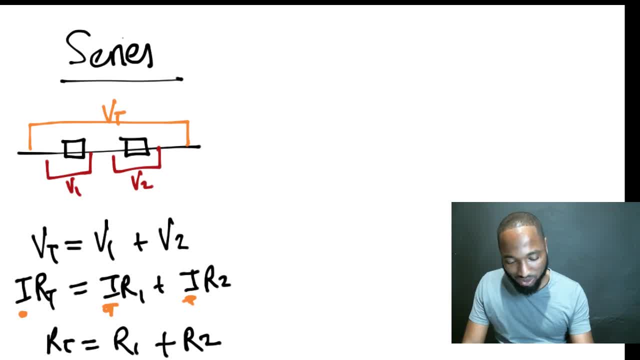 you can set it up in this way and you will get the result of the current in series. so let's draw the series, let's drop the power of the minimum, so you have this one, one item. then we have one item there. let's bring towards the battery, obviously. 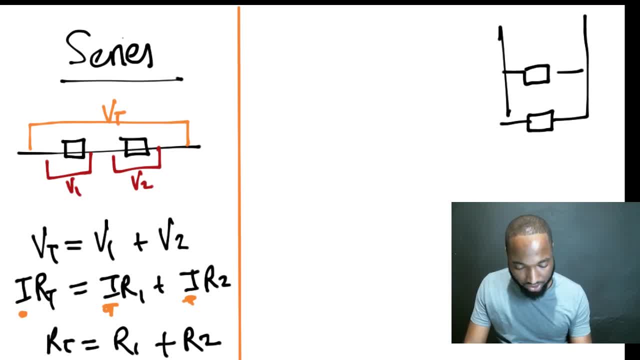 they saw that, come back. I need the battery and I didn't draw the right, but who cares? so now, from here to here, is V T. you can't use V because you have the current and you like to use that. so this one is. this one is half the time we have. to do is analyze this time. Point two: write for another time. so in this, the principle it's less to the left than the right. because we've done so, I say 0.3. we can't use v because this should be equal to S and this in R, and that's what we. 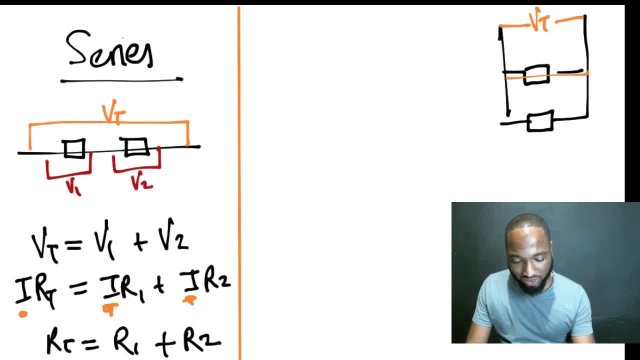 make our total value for the next generation. this V is equal to R and we will, because the voltage is the same here here. so we can't use V to start of the equation. What we need to use is I. The current here is I t. 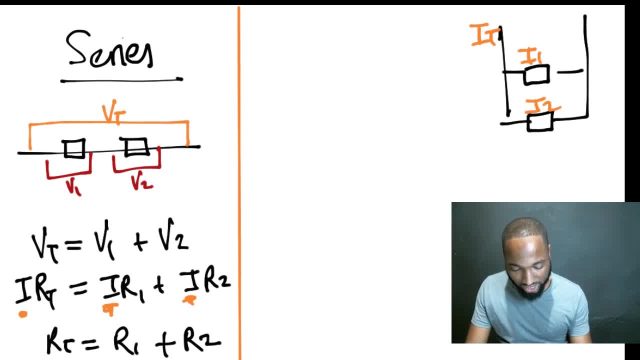 and then the current in this one is I one and the current in this one is I two. so we're using I to start of the flow. So it'd be like I t. you see how we start of it V when we have something in series. 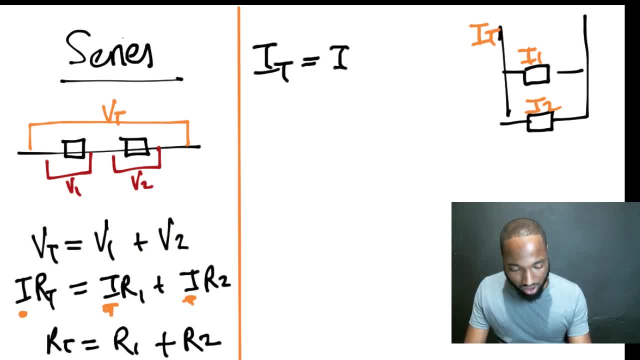 now we need to start of it I, so it'd be like I t is equal to I one plus I two. So if that's we do in the series equation, can we use that? Obviously, this is what you have to use. 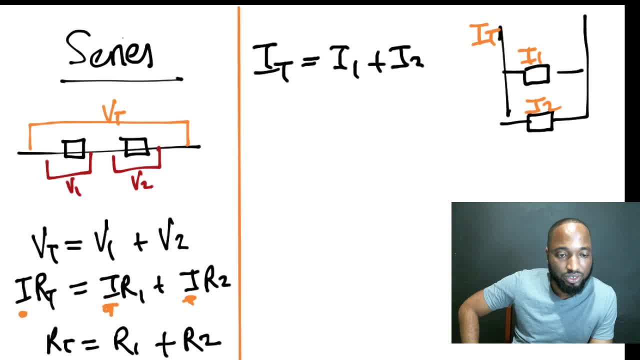 This is exactly what you have to use if you have to derive the series equation: Get co into 30,000,. yes, get co into 30,000 subscribers. No stamina, I have no stamina, So you in, I t. hopefully I have the stamina to do I t. 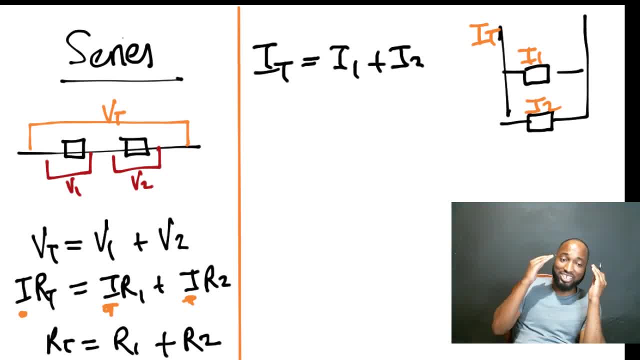 because when I was watching I t I was like whoa, so much things I forgot in I t. I cannot believe I need to memorize all them- acronyms and things. So hopefully I might help all in the I t and in the programming right. 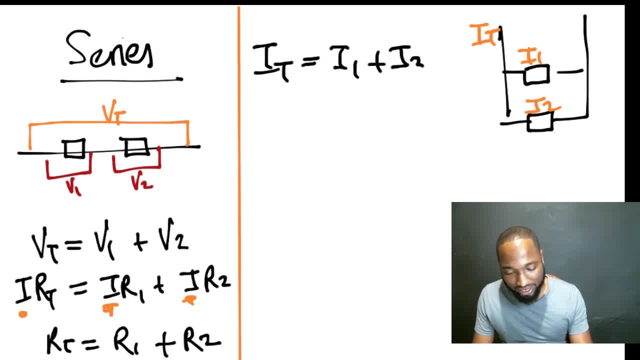 So now remember I- we substitute V is equal to I r here, But I is. since V is equal to I r, I is equal to V over r. So this is why it get upside down like this when we go into parallel. 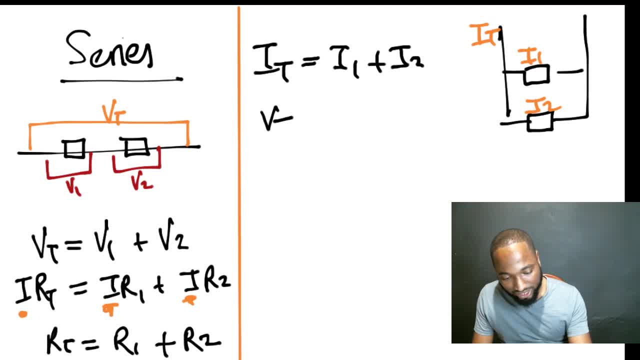 I is actually equal to V and I don't need to put anything. can you see, Because we want to do the same, I t over V r one plus V r two, And when I cancel all the V from everybody, I'm gonna end up with one over r t plus equal one over r one. 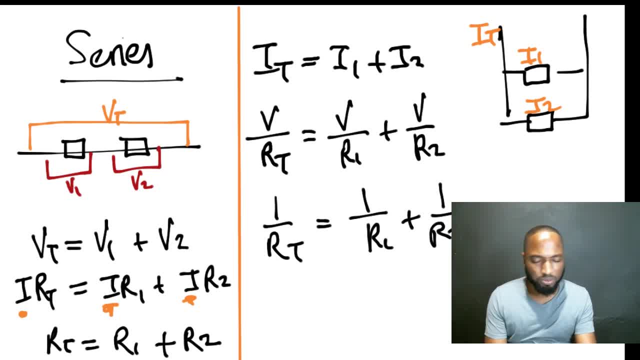 plus one over r two. So it's pretty easy, it easy- yeah, I seen people saying it easy- And that's how we derive those two lovely equations there. You need to know which one to start with, And you just, you just. 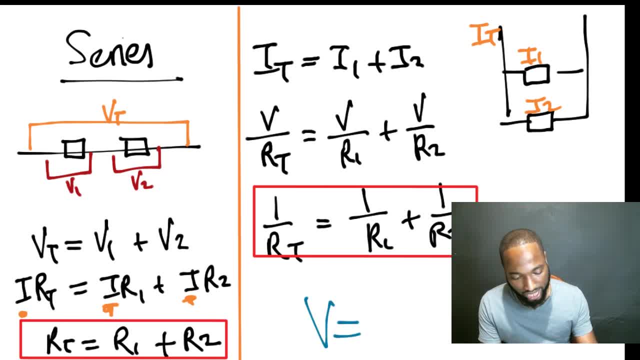 the key is to use this equation: V is equal to I, r In series. you start with the voltage and you add it up, and then you substitute using this equation. In parallel, you start with the equation with I and you substitute using this equation. 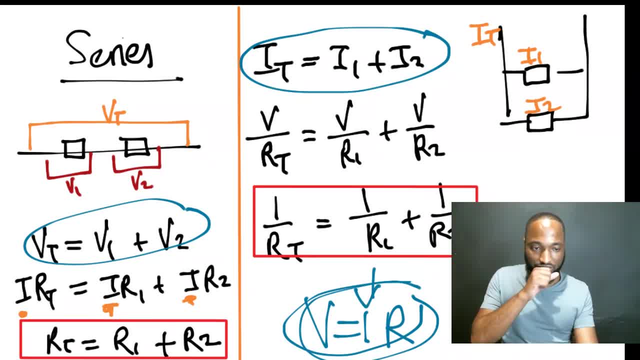 but make I the subject of the formula Y is in the chart next. So then you need to use that information to solve. solve questions, right? Let's draw a little. let's draw this little diagram here. That's your question. 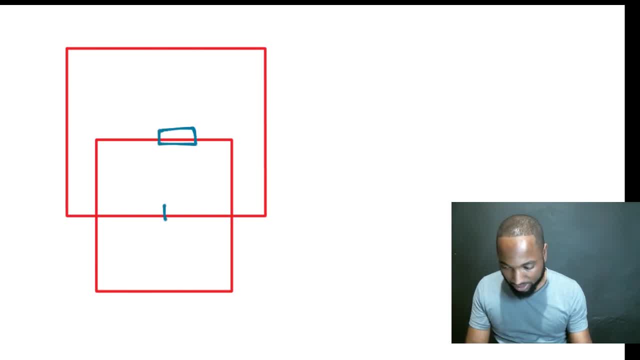 Drop a diagram, ask the people them a question Calling this: one one ohm, two ohm, three ohm, Three ohms, where ohm be in the unit to measure resistance. I one, I two, I three, Cause remember the current splits, right. 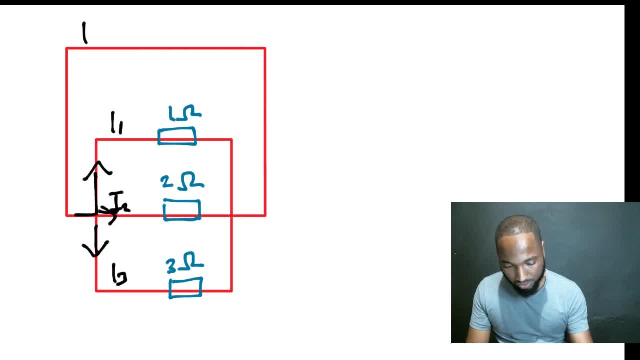 It splits into three. Whoop, whoop, whoop. Current split into three there. So we put: I t here now, Current going this way, coming back up here. Hey, Let's make this the long short. positive, negative. 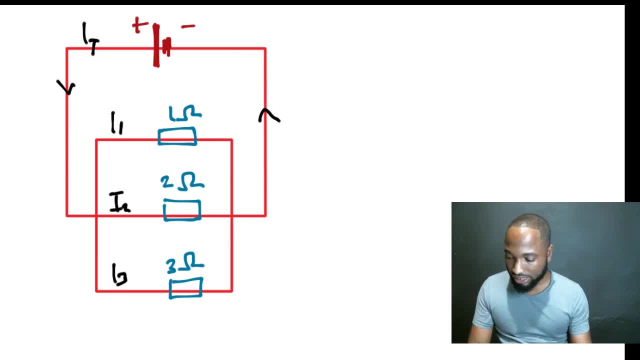 No, but you don't need to have that there, All right, so let's ask some questions. now, Where's the total resistance? Total resistance in the circuit. So I can't put it in. I've got time, Let's look at that. 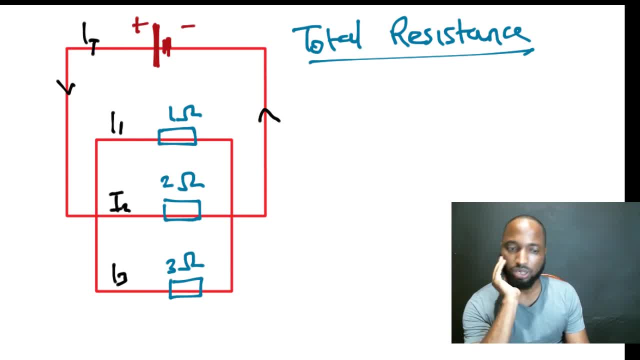 Let's look at that. It needs to bepractice- not me, All right, so let's do it with our hands. All right, I'm just going to do that, Okay, so time to put our hands together. Let's do it with our hands. 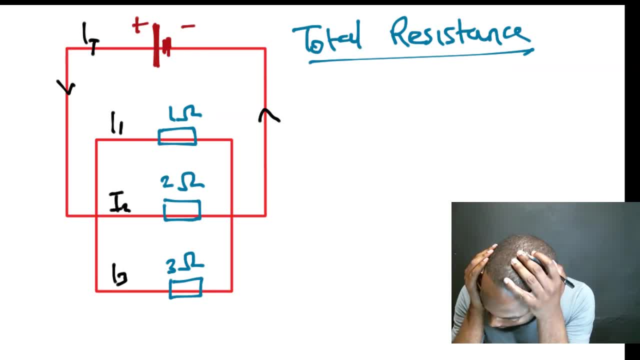 I'm going to stand up, All right. so now I'm standing up. Keep your hands on the ground and I'm going to put my hands up. I'm going to drop this out. I'm going to hit this One, two, three. 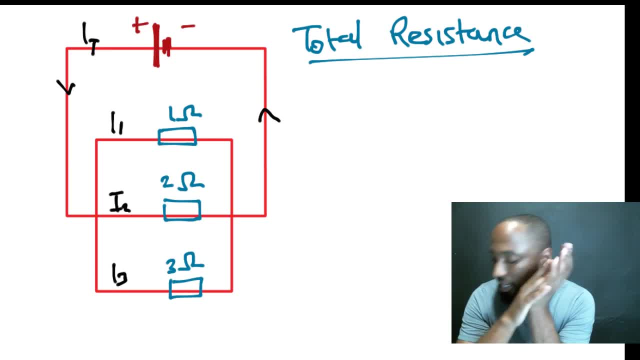 One, two, three, two, three, two, three. All right, so let's look at that next. I'm going to put this down. I'm going to keep the fingers up. i guess you can see the mistakes. i've seen six ohms. i've seen 0.54 ohms, where it really is by. 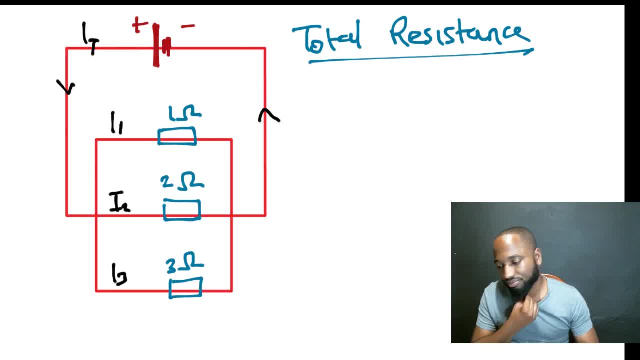 what's the total resistance like, what's the resistance in the whole circuit? then this number here is one. all right, so let's just work it out. one over rt, it's one over r1 plus one over r2 plus one over r3. so one over rt is going to be equal to 1 over 1, so that's 1 plus 1 over 2 plus 1. 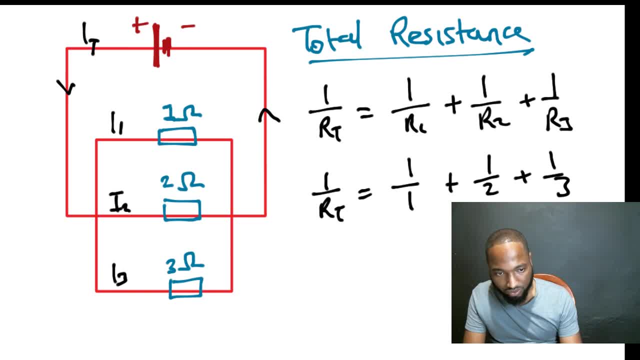 over 3.. what are we getting there? one and five, six. one and five six, so eleven over six, but this is one over rt though, so we need to do a little swapping. swapping here. six over eleven, six over eleven. a lot of people stop at the one and five- six. after we, we just stop what i do. 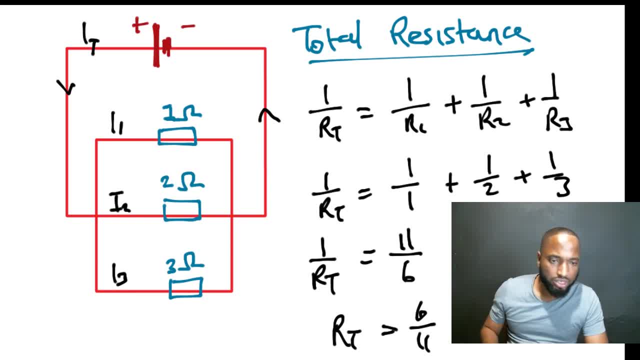 somebody said a loss. maybe we need to re-explain this: i can't do this. somebody say they can't do it. why people saying they lost? why do people don't say how you do this? and you know i have a problem in that senior loss- why are you saying wireless? why are you saying what is that? how you lost? how you lost where? 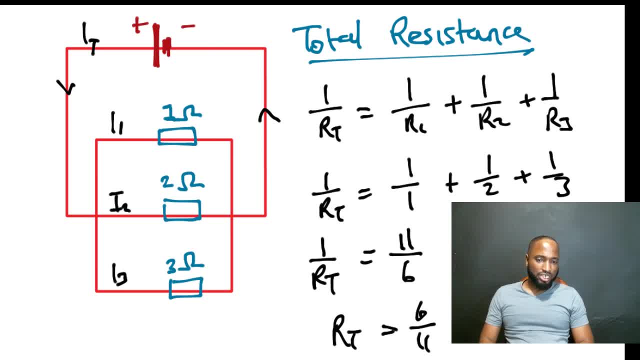 you lost which part? see which part. you don't understand which number, which line. how am i going to pass? that sounds too depressing, man. now this is the real question: why you lost when you lost it. what is infinity? that's easy, some people say it's easy, but some people have problems with it. 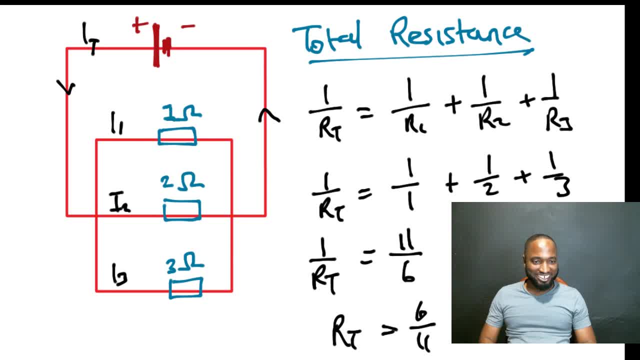 the lc and you're also the lcm and they're going getting heated. they should see main class. i'll be currently students. don't tell me a loss, show me which line, what is the line? and then, when they tell me the line that i explain to them, i'm like: you see, you see. 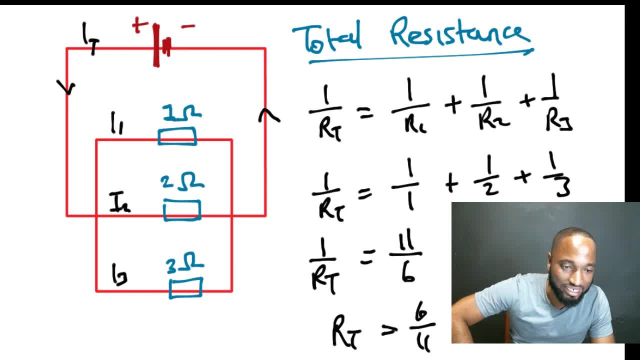 you see, currently defeatist mentality to be more positive, people are so as impedance. impedance is the total opposition to the current for winning on the ACC to in trigger and it's only done so. that's a commentary. so in chin cohen, where did you get the left man? where I get the left man right, plug this in your. 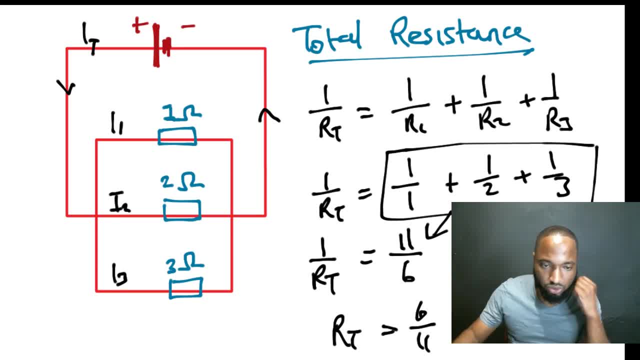 calculator and you see that in purple. so if you are gonna answer questions I can't answer when you see you get lost, all right, let's pull up my calculator here. yes, there's only total any parallel section, but the parallel section is all that. I don't be resistance here, here and here, and that means as resistance in the. 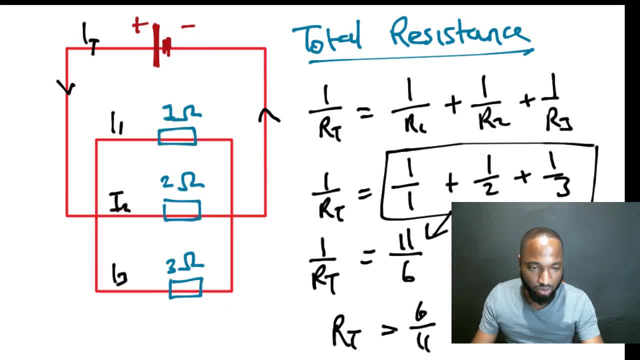 whole series. that's how it works. there's no resistance, there's no resistor here. now, if I had a resistor here, like if they draw resist, I hear that I be some back and out. hey, if I draw resist that day, it means after we bought this and I get. 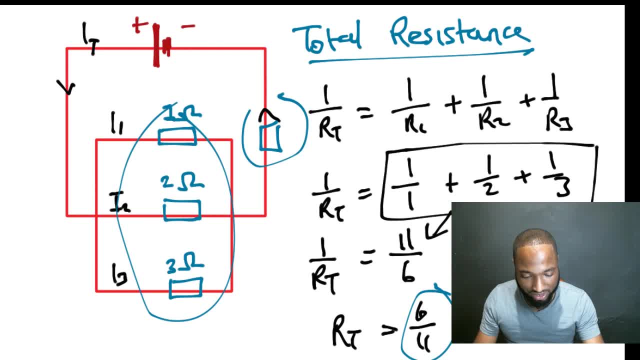 this number. I need to add it to whoever this is, so maybe I'll do that, not personally. so this: this is one and a half and a two and a half three over six, but also ten, two by 656, so one on five six, one on five six. is this correct? 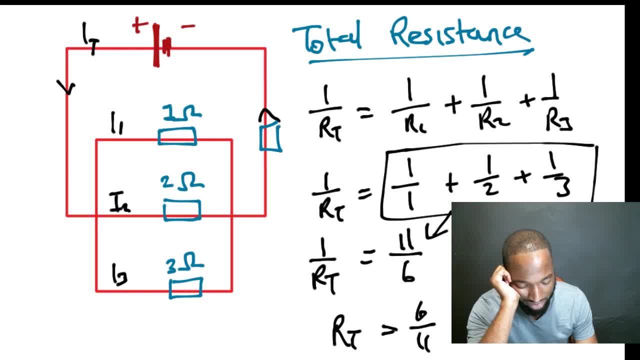 one by six, six plus five, so this is 11 over six right fractions. and then this is one or too tough. well, also, if I pass in tällã a need two people saying invisit, I cool it out. be used that way if I НадHOU Challenge right, so if I'm in您我通話不做啥. 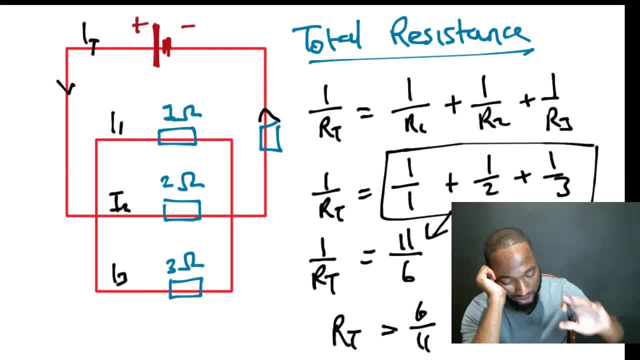 now, if I flip the numerator and the denominator, this side must flip the numerator and the denominator. any more questions, any more questions, any more questions. so I'll give you another next week. if I need to chat about some stuff, take our next circuit now, fellas. 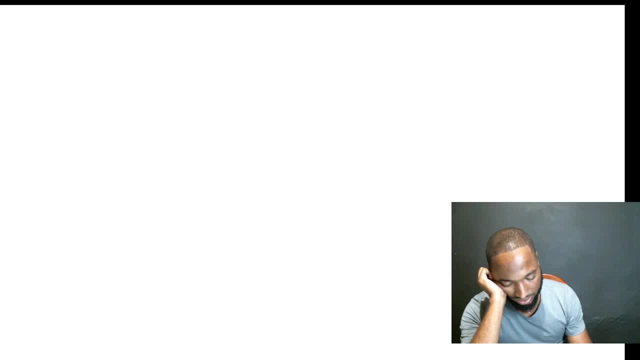 take our next circuit. let's make it similar to the last one, but let's do what I talked about just now and put a resistor here too. let's make this resistor one again. let's make this one two. let's make this one two. let's make this one. 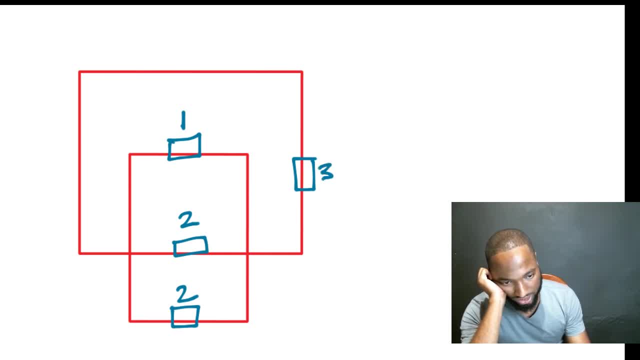 three, what is the total resistance? let me see who finish this. where is the total resistance? here? and after we talk about fuse, we are going to talk about electronics and the logic gates. so after fuse, we're going to talk about logic gates. when I finish with the logic gates, 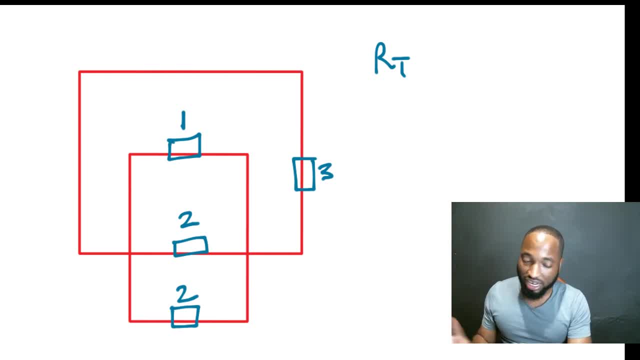 we're going to talk about motors and generators and after we talk about that, you gonna be done. yes, sir, will be done. so again, different actors at 3.5, but you are the first one to pull out a 3.5. Wow, well, you inside you, inside my mind: nobody, somebody see a half homes being. 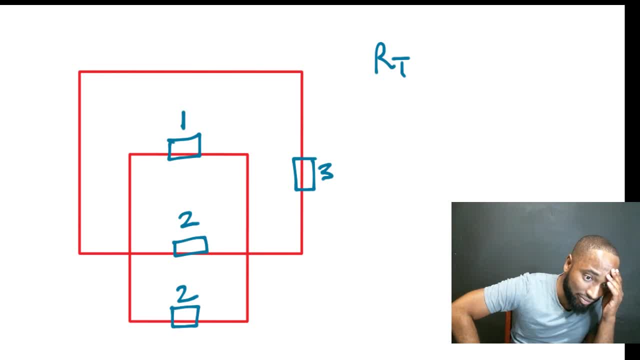 different answers but in five being 3.5, being a half, 2.5 canary in supreme. now it's full of consume. a viewpoint in xtn 408. finally a can relax and I don't tense ol yellow, yellow headed. oh hello, miss me on two hours and a half. 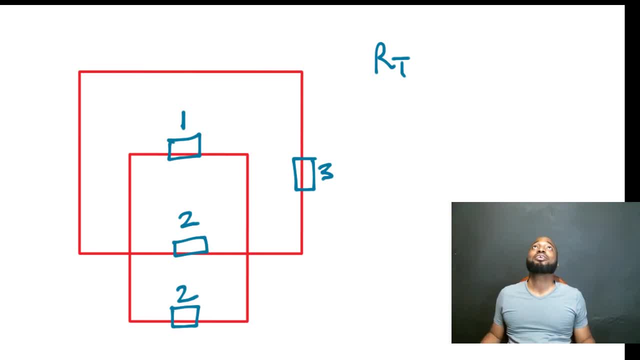 doors and a half. this man is still also. so what passes in fact? yes, lady, and Saturday custom. so what passes you've got? yes, pizza, um, cheap and fine. keep on flying. three zero point eight. when people ask me, so what subjects you teach? yes, 3.6. 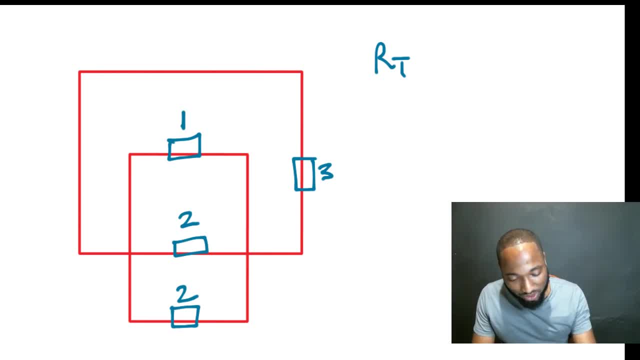 2.5 people getting different answers. they will get up right. so you need to see if you got a question like this for cx, you need to look at one part first, then add on that. so let's look at the parallel pathways, so the parallel part here. so i'll put rp. 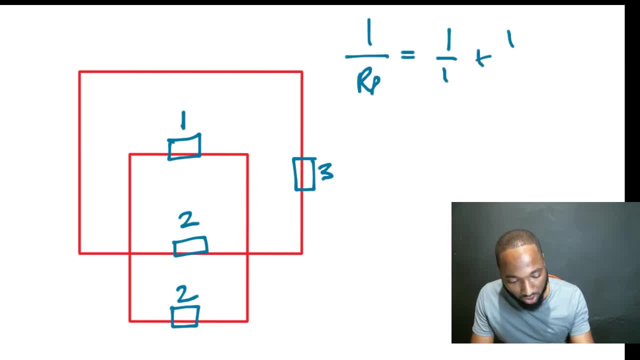 term and term representing parallel part would be one over one plus one over two plus uh, and i just use a new formula. right, i'm gonna put any formula first, so i will be like bluffing my way through. so this is iron plus r2 plus r3- what the hell- plus arch. 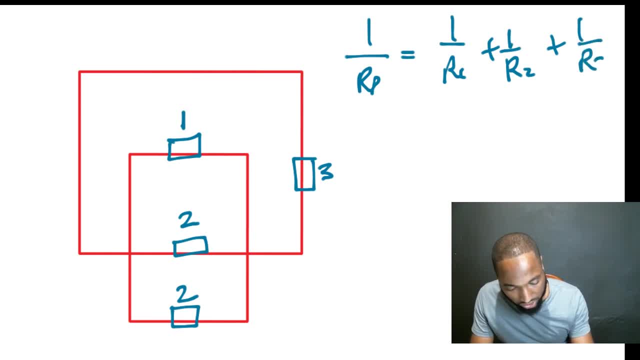 what? one over r3. so this is one over one plus one over. is that a bug of it? well, let me get our passes one over two plus one over two. so this is two. well, one over two. so we got 3.5, one plus a half plus a half. 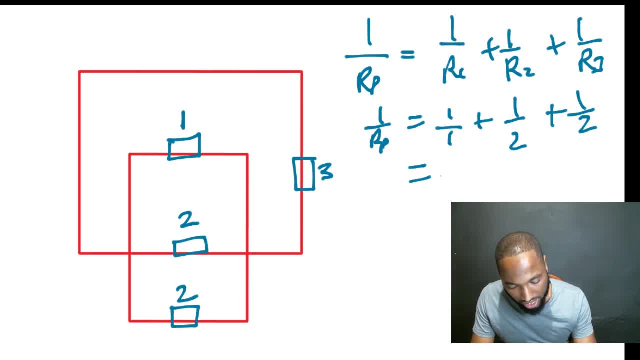 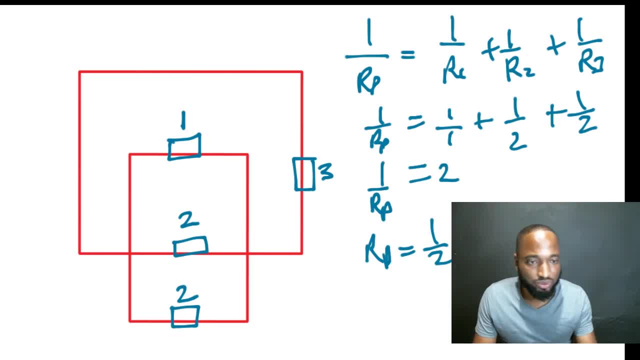 so do i t next piece, but the gates is in it too, so they must currently each resistor question, please. all right, i'll give you another question with a little harder stuff involved. um, can i pull up one from here, and they are one for the people then more so i've got. 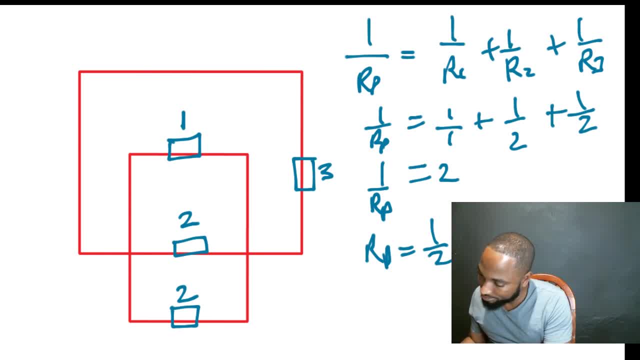 one for the people's them. so i gotta make up that question. all right, um, but yeah, so people pull in back now to 3.5 and therefore the total resistance now would be resistance in the parallel all of this could represent by one resistor, which is: 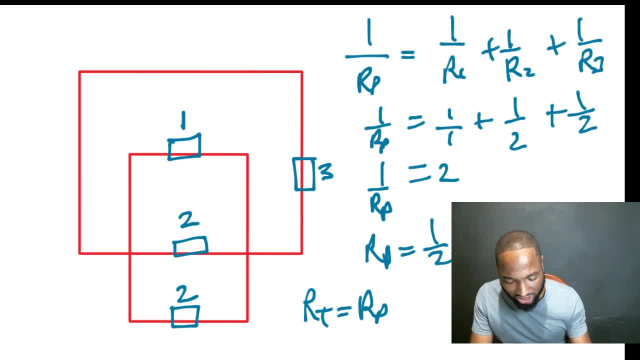 half, and now it's interesting to note that i'll just. i just want to point out something plus that third reason. i put three here, but i will call this resistance j это economies that four or something, resistance. so this is a half plus three, oh so 3.5, right. everybody see how we. 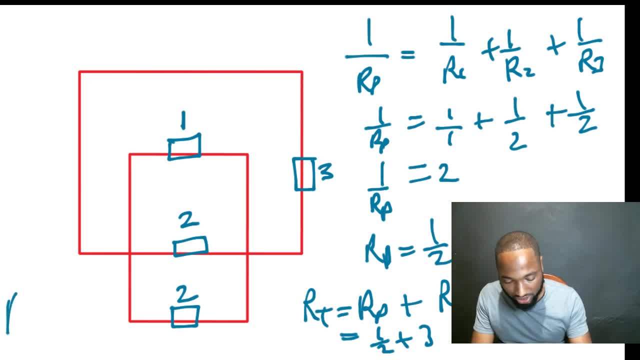 get the 2.5. five y is in the chat, so there's this 2.5. now it's important. i didn't put the battery and the kind of thing but nobody came it's important to. it's kind of interesting to see that this is one ohm. 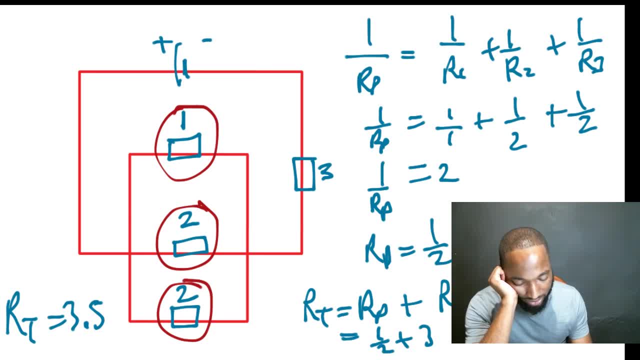 this is two ohms and this is two ohms, but yet when you add up the two ohms to ohms, but yet when you add up the resistance, it come out to be a half less than all of them. it's interesting. it's interesting. so when I started, put things in parallel is make it easier for the 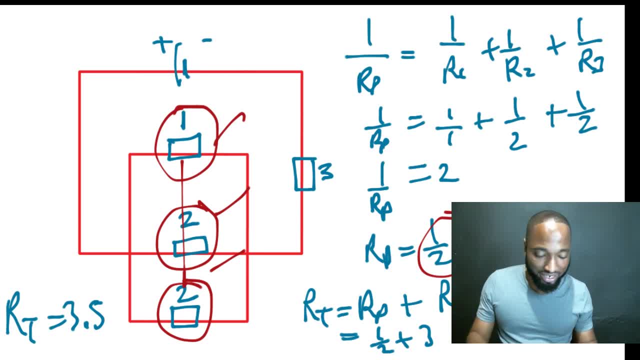 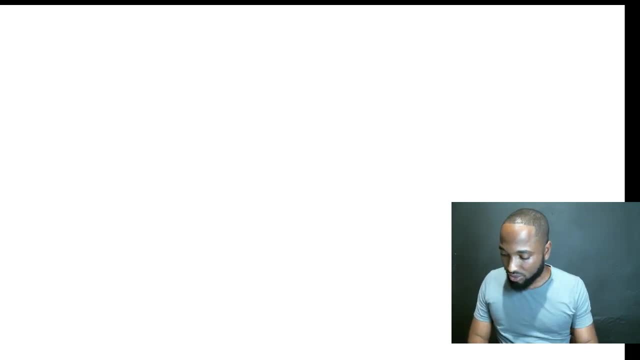 current to pass, even though increase the resistance and if it in parallel, the resistance is dropped but resistance in series is add up that are pretty high. man, all right. so he wanted a question involving like current so he could get some more. some out of it. I remember I don't teach physics right. 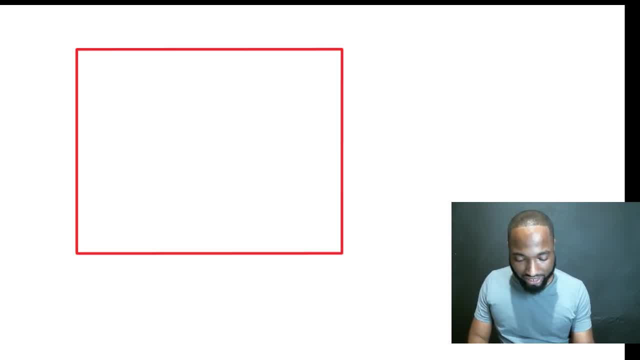 you like, I have a few private students and I just teach yummy hard things as a private students cannot be obtained by the update, so I just teach them like motors and things. I really making up these questions every day. I can maths. let's not do the same city like in a fellow. see, that's it, so let's create. 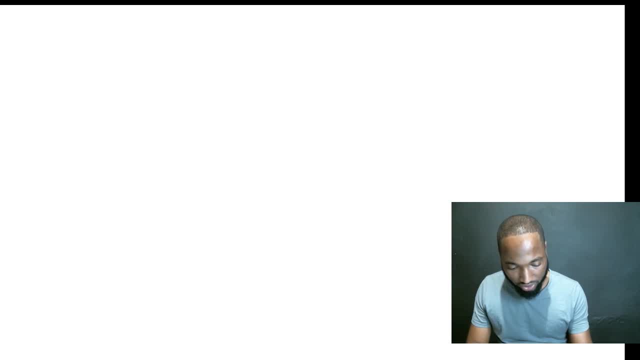 this you let's make you read to my friend. let's draw the secret to look like this: let's just put two. let's erase this, creating the question here. guys, that's not a fuse, it as a resistor register there let's put. let's put a resistor here to know. let's not color the resistor like 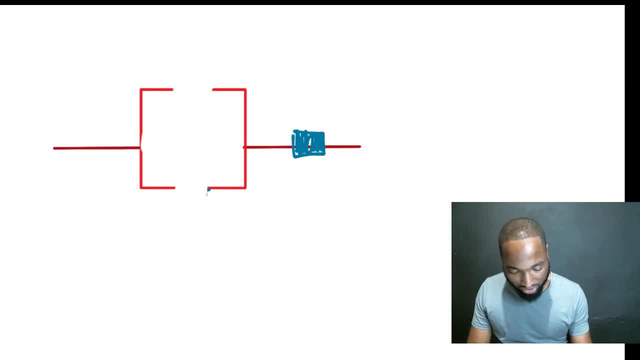 that. so let's be some more time and erase it back off and draw a box. Wow, Cohen really performing here. man, not that, but let's see. this resistor was two rooms. let's seeURL oders so far. let's see that one girls too. city current is. 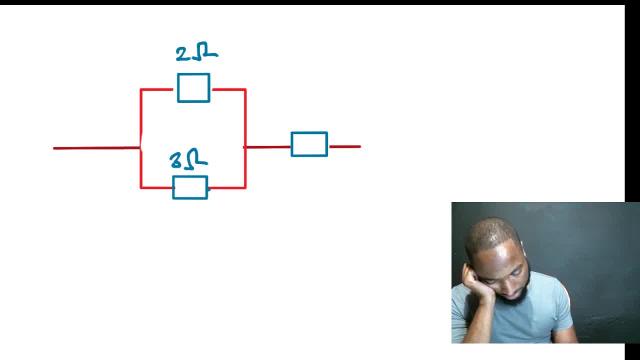 don't you so good here. total current is 5 amps. let's make this. Oh gosh, I've taken so long to make this question. Let's make this. Let's make it 1 ohm. now I will change up the question to suit just now. 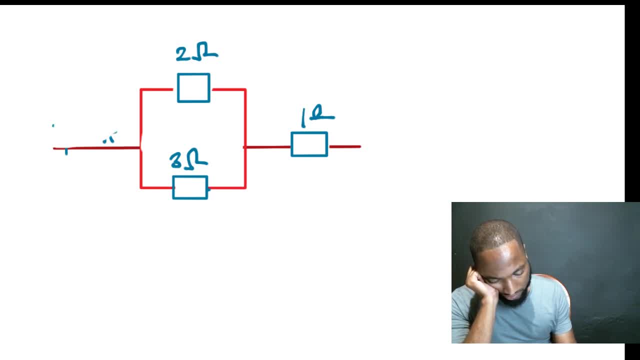 So the current in the circuit is actually 5 amps And They want to know what is the reading on the voltmeter there. What is the reading So? what is V Or what is the total voltage in that circuit? Proceed with caution. 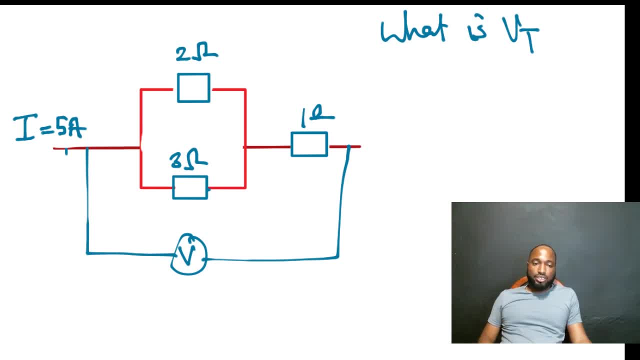 So if you see a question like that on Monday, how would you do it So people don't pull in all that much ohms and things like bosses, like the bosses there. 9 volts, 9 volts. Andrew Black say 9.. 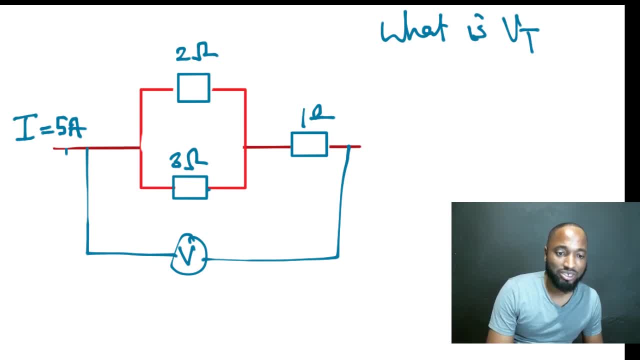 A man say somebody say 2,311 volts, That's an interesting number. A man say: go and sleep on it. A lot of people holding on to Sir, I'm tired. now I feel like going to Yeah, by injustice, hold it down. 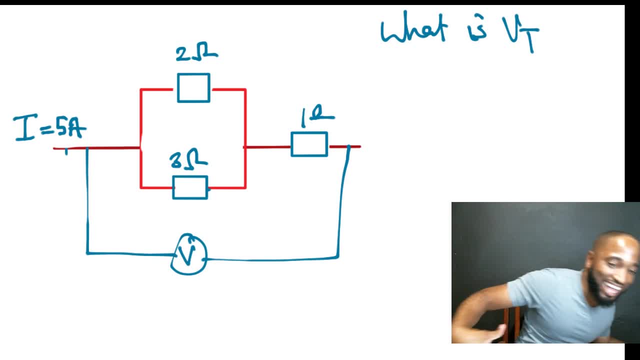 Yeah, You go through all the easy things and are now going into the killers. now the logic gates, the motor and the generator, and you have to go now by. I feel by the time I finish I might have 100 viewers. 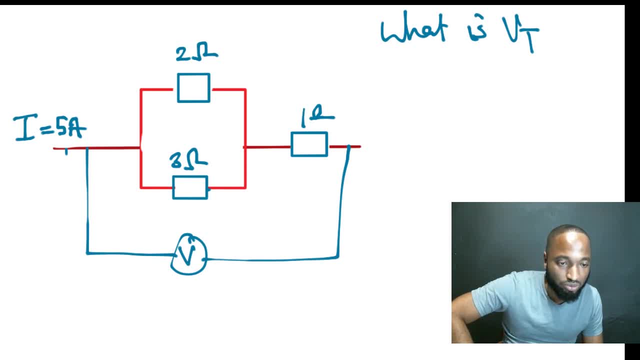 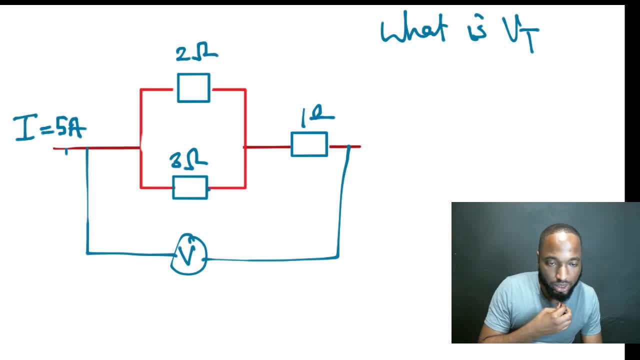 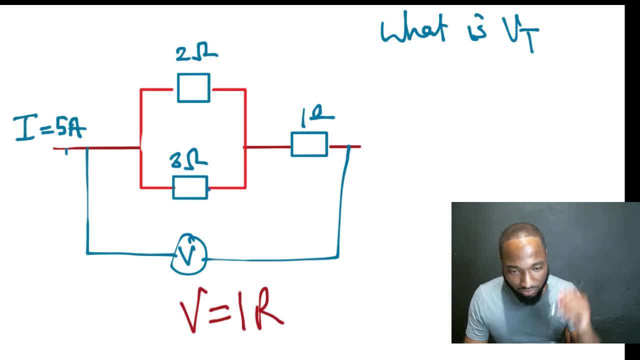 The V to get V, I need V equal IR. So you start off with what you want- I want V- And you check what you have and what you don't have. I have I. I look at here, But I don't have R. 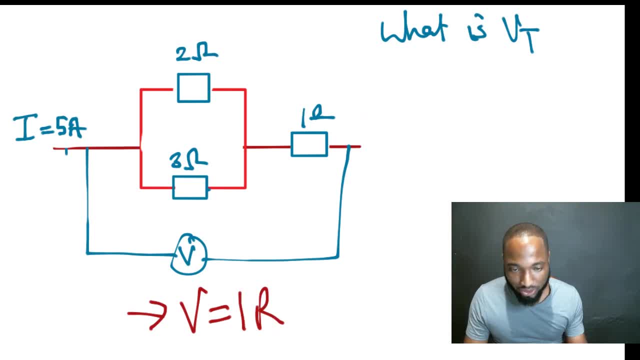 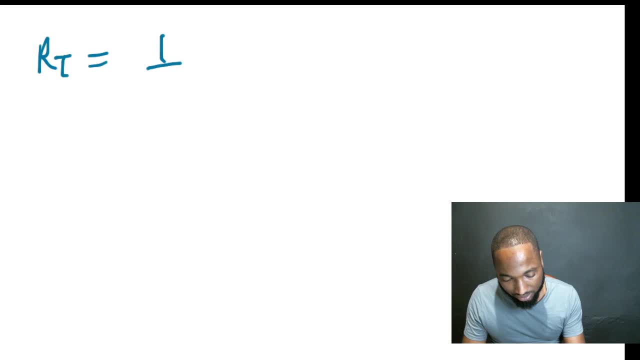 I only have all these things. I need to get the total R, which is what we are doing all the time. So what I'll do is be like: The total will be the sum. You understand The parallel thing, Parallel, And you add 1 over 2.. 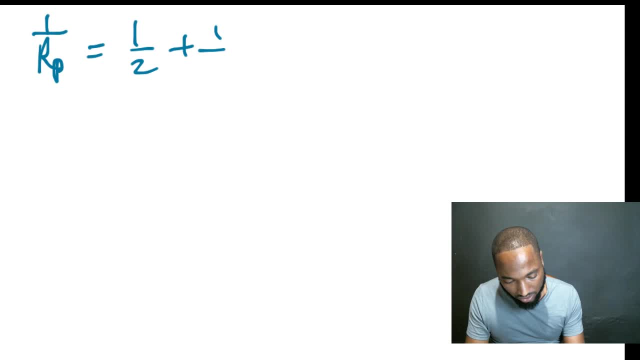 What's going on with you? Lubia? 1 over 2 plus 1 over 3. 5, 6. 6 over 5 is the parallel, So the total is going to be 6 over 5 plus. 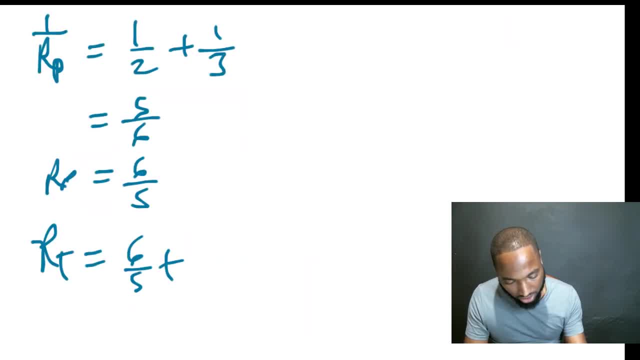 1. You spread up a sum for total resistance. Yeah, you can use that by teaching that from you, Especially how you're mixing the three resistances in parallel and things. I want to talk to people ahead of that, Right, But I see you. 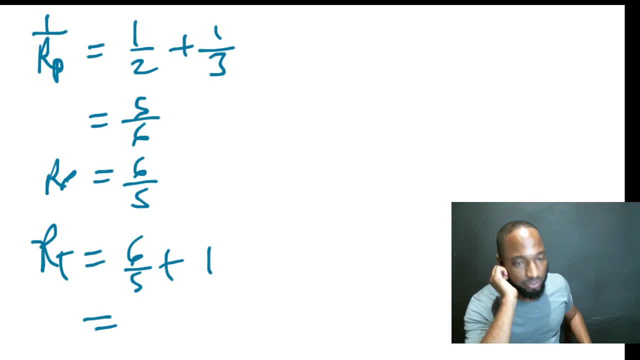 If you're comfortable with that, like some people use, spread up over sum. If you're comfortable with that, free up. Great is the coming and he shall prevail Right. So let's keep going. So this is 2 and 1, fifth. 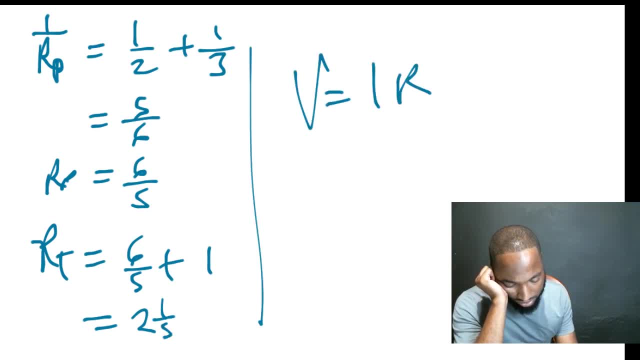 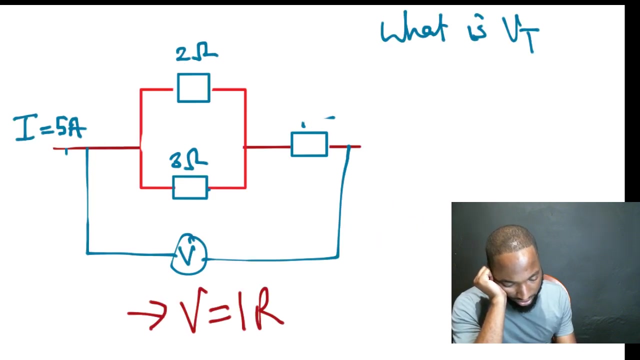 And then now we can go into V equal IR. V is equal to I5 times 2 and 1, fifth 2.2. Excuse me, And everybody get 11 volts, Okay. Change of the question. What if this wasn't given? 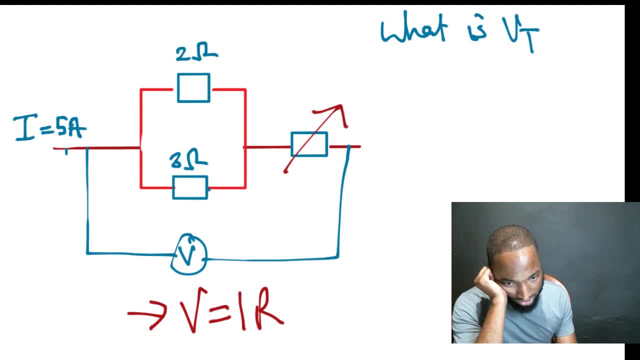 And what if they say that's a variable resistor? Well, this could be as hard as it comes. This is why I say it's better to understand than to memorize of questions in physics, Because physics can come any way. All the ways is easy if you understand. 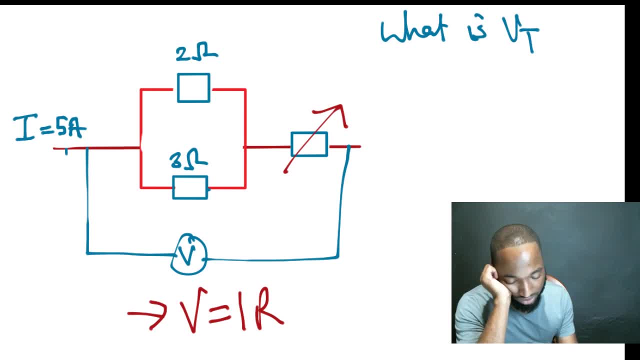 If you don't understand. it can come in millions of different ways. Right? What if they say this is a variable resistor? Right, And they want to figure out Rx. Given that V, the voltage is equal to 20.. It's 20.. 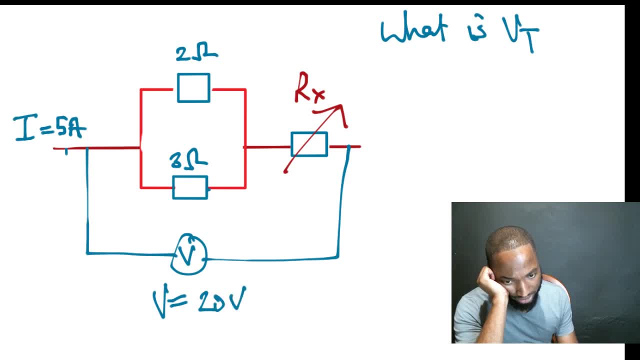 20 is kind of high boy. Okay, Let me make it 20.. 20 volts- I don't know why you're doing a 20.. Okay, Let me make it 9 volts. Sorry to stop those who came. 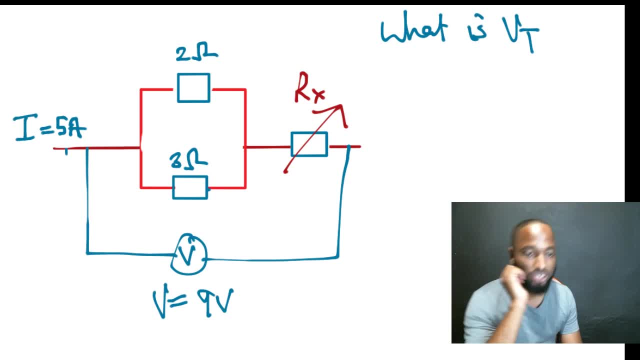 9 volts. So, given that the voltage in the whole circuit is 9 volts, I'm waiting for it to come in here. Do you understand That the whole circuit is 9 volts? what is Rx? What is the resistance there? 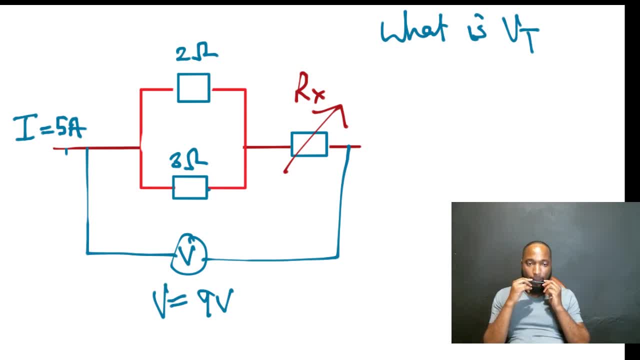 How are you going to do that? How are you going to do that? now, guys, Let's focus, Kick it this close here, This close. We're getting our time out here, brother, But this close, This close. Please don't make me do what I have to do. 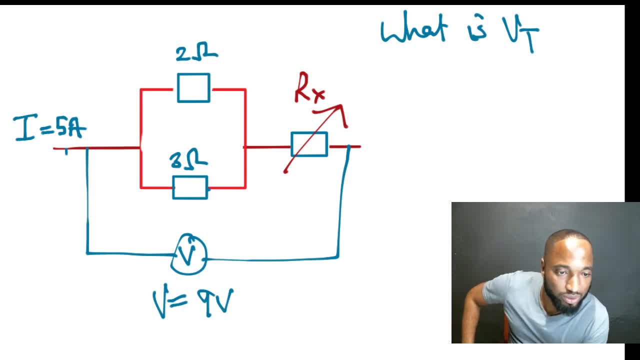 You know I don't like to give people time. Whoa, Ryan says 0.6 already. Joel, pull out 0.6 already. Some killers out here. boy Cool when you're salting on the wing- 0.6.. 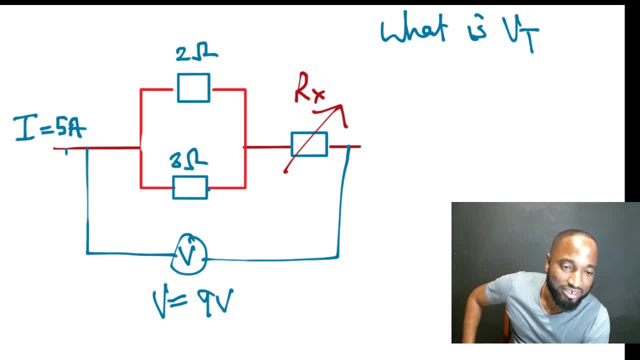 Addie, pull it out already. Yeah, man, Match you 10. 0.6.. I like to put in a little ohms too. Make it big. Thank you, Kicks. Thank you 0.6.. 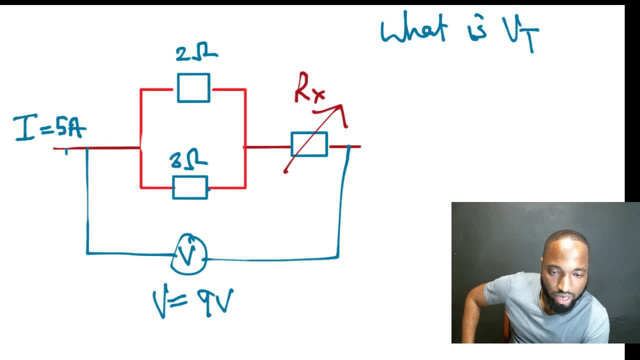 0.6.. All right, So the working fate is like this: right V equal IR, So R will be equal to I over V. You figure out what the resistance is that we need, Like if we don't know nothing before now. 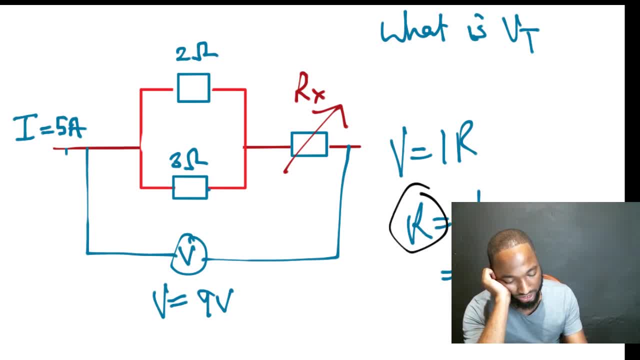 Remember we're looking for the resistance. eh, This will be the total resistance here. So this total resistance for the whole circuit must be equal to 1 over 1 over 1 over Voltage, Not 1 over the voltage. 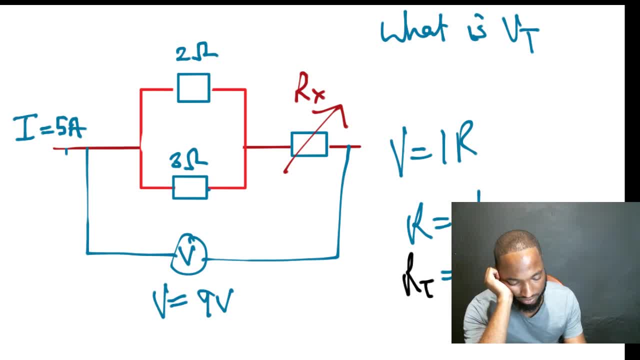 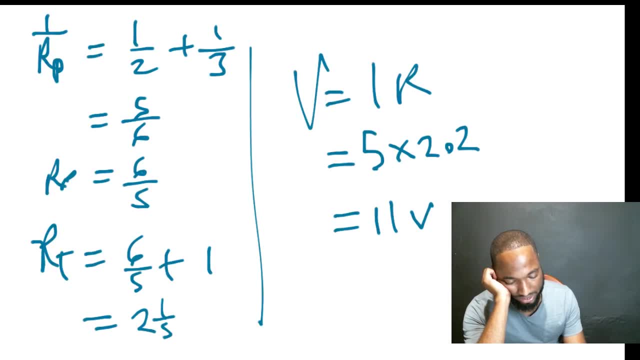 I over the voltage, which is 5. Over 9.. So it's 5.. 9 is what we're looking at. So this means you find the resistance in parallel. It turned out to be 6., 6., 6.. 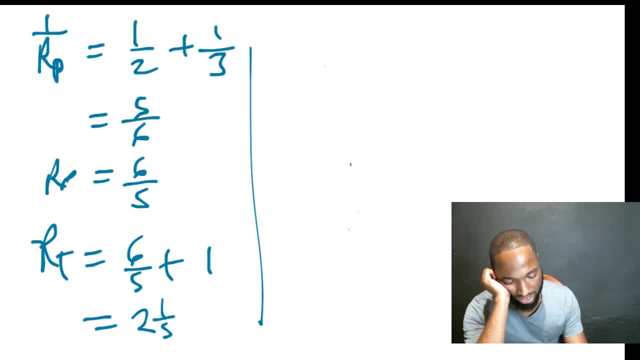 6 over 5.. All the catcher are going. All the catcher are going. You catcher are going, brother Catcher are going. This is the resistance in parallel. That wouldn't change. We didn't change anything there. But R2 must be 5- 9ths. 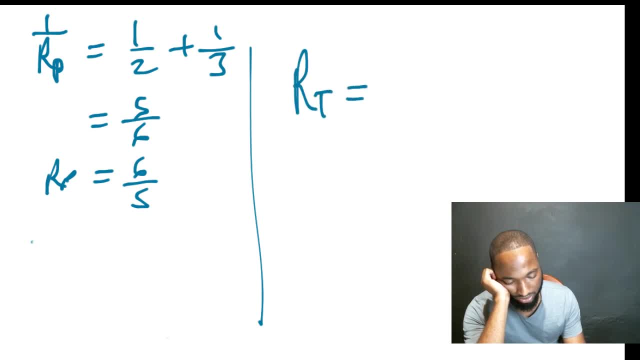 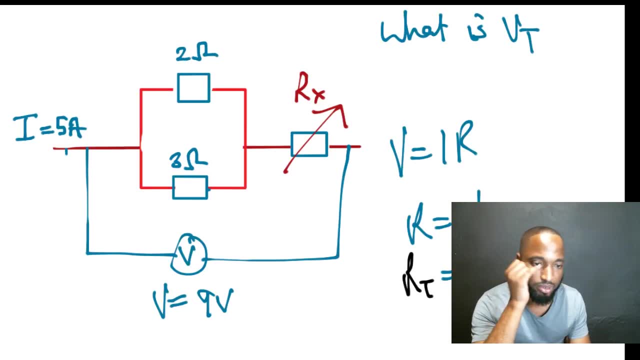 So R2 must be equal. R2 is 5- 9ths, So 5- 9ths must be equal to. Okay, this is impossible. 5. V is equal to IR, R is equal to My bad, R is equal to V and I. 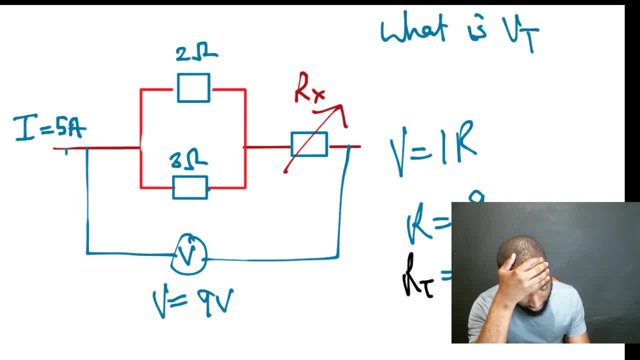 R is equal to V and I 9 over 5.. Anybody correct me, You sample. Nobody correct me. R is equal to V and I 9 over 5.. So 9 over 5 is the total resistance. 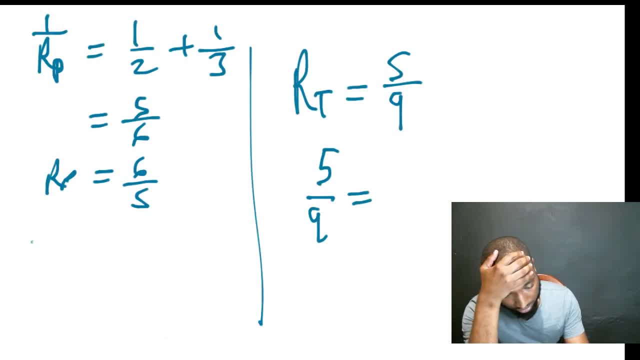 So 9 over 5 is the total resistance, Um 9 over 5.. 9 over 5.. 9 over 5 is the total resistance. This is the resistance in the parallel, plus the resistance which we're trying to find. 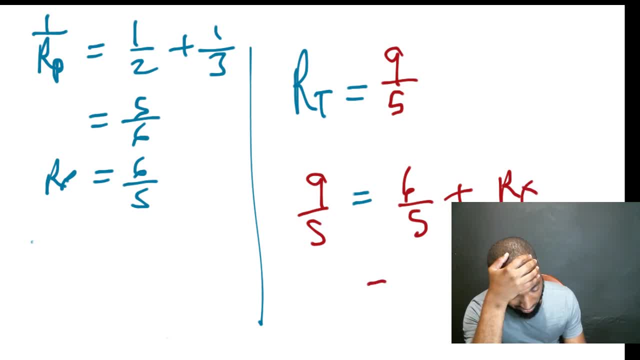 Rx. So from that we could see Rx must be the remaining 3 over 5, 0.6 ohms. Well done to those who got it all very quickly. I can't see you working at the moment So I could have corrected you. 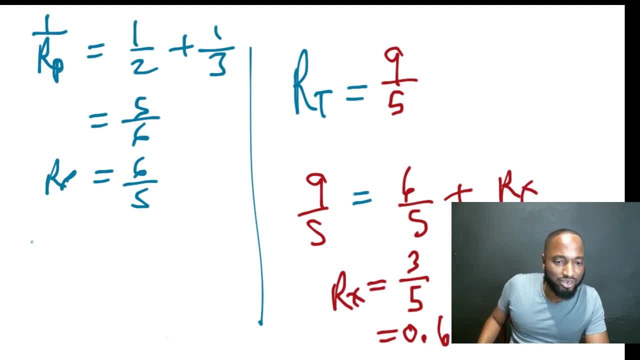 1.8.. Not see and say Not see and say Nobody can see behind your video. 1.8. 1.8.. That sucks, Let's not let the number tune on yet Me. goodbye All. they wasn't seeing this. 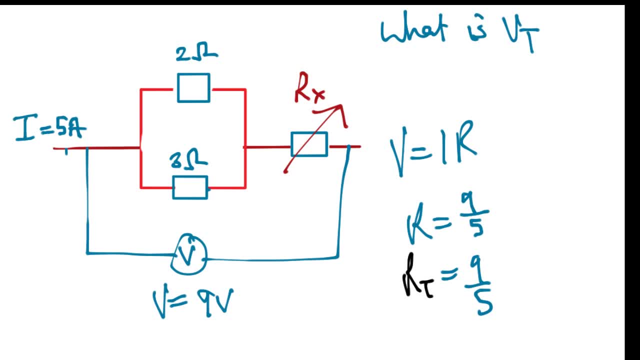 Aight. So that's right. Sorry, I couldn't correct me Pretty good. Do you think, Mr été, you're make mistakes Easy? Alright, yeah, So I made the mistake I make when I was working on R. I guess For some reason I put I over V. It should be V over I, right? 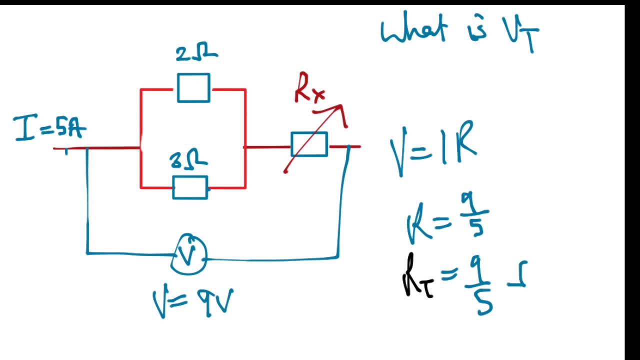 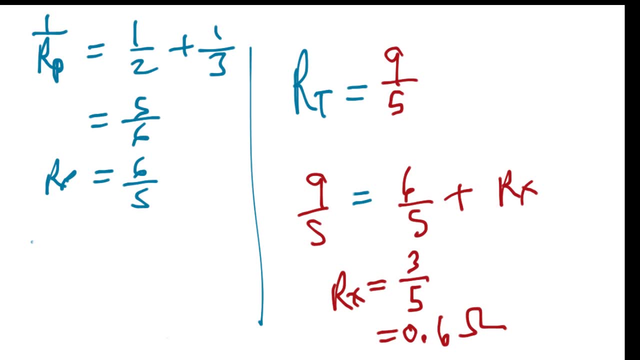 So this is 9.5.. So this is the total resistance: 9 over 5.. resistance. yet once you find the total resistance, that is sick. it needs to just see that, the total resistance. and this is a lovely question for them to bring. 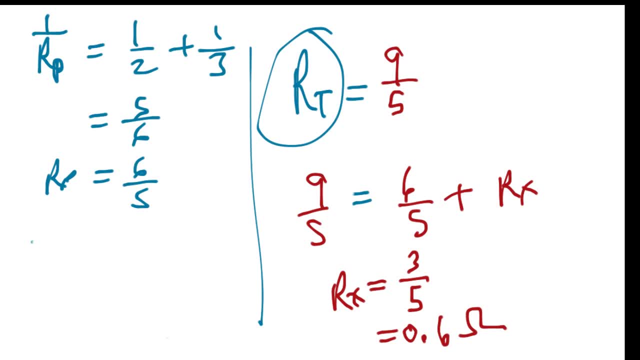 if they bring this a Monday, I'd be laughing. you just see, RT is equal to this is resistance in parallel, plus resistance we trying to find- and you use your algebra called skills wise in the chat. let's move, man. let's move now. come back alive here. can you all tell me the definition of a few things? now there's a. 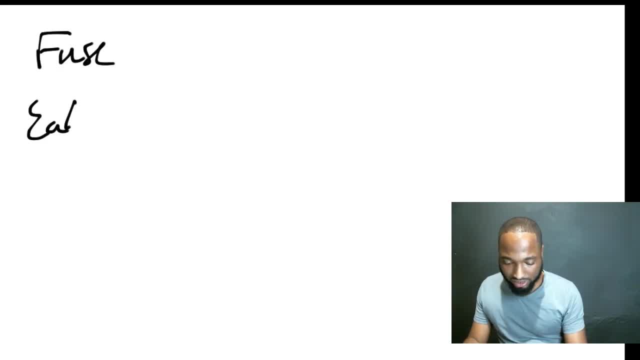 whole fuse and it's question that went along so you have any difficulty. she was an idiot. know the definition of those, know what can I rate infuse? you can choose, for example, if you have, if you have nine, if you have a four amps run in here, this fuse, the couple a. 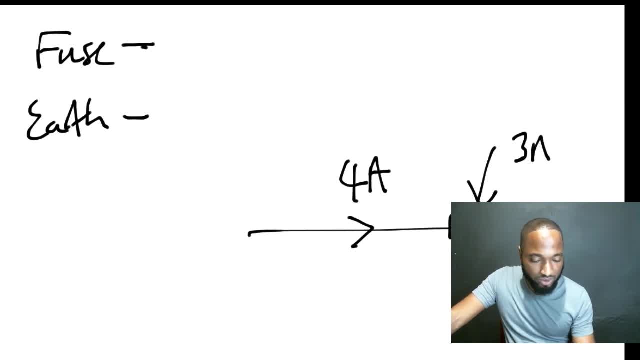 triumph user. I think a blow. you're looking at the five of us, maybe six. fuse prevents thing, but but. but fuse breaks the circuit in case of high voltage back, back, back. I keep drawing behind me. now this question came recently and I do it already. it is flat. 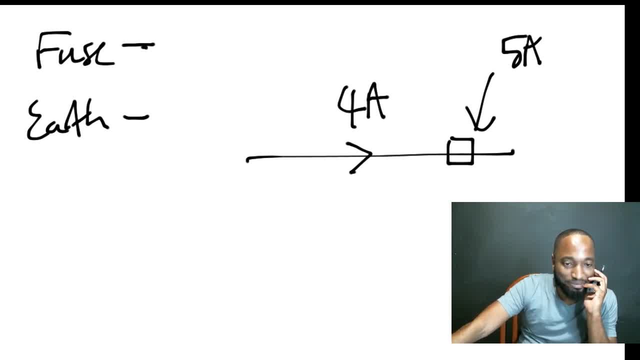 what I need. some conduct, please. and when it is your emission, I don't know, you tell me, but it refuses. I compliment component of just a Princeton. wife says: restrained. yeah, coses, not stupid, brick 만나 boy. I mean, can cards do that? okay, oh yeah, but that's so good. hi, David, where you goin G Gear Button weirdo, William Guillermo. 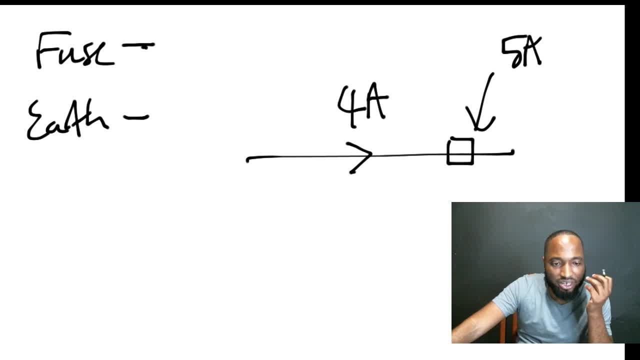 break. I use that mechanical. mechanical so you can. yes, if you can break, and then you can turn back on your breaker, right, but a fuse is actually burn out. you can turn back on your fuse, it burn out. SpaceX about to launch a rocket? that's cool, but teaching the Caribbean better. 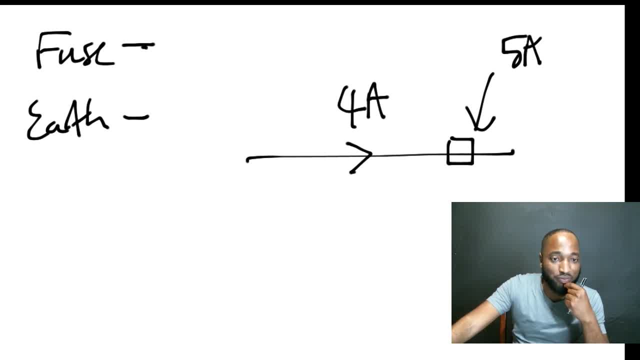 is of more importance to me. so 200 people. hopefully we could keep it to over a hundred by midnight before we finish, right, okay, so we have the definition of a fuse there. the thing for it where protects provides, was the definition of it, so we have this as the definition of it. somebody see Moses? 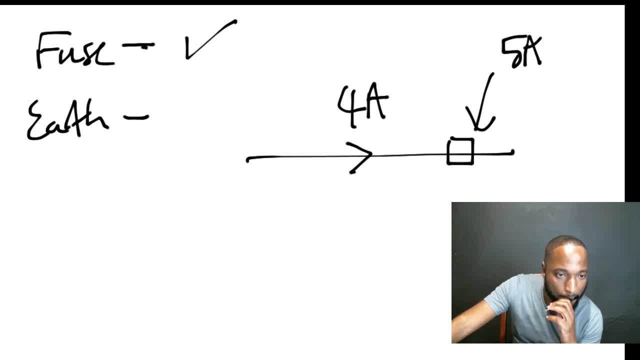 coming up in 1982. you know they need to wake up so you can very time. really I don't find a lot in time. if you this stuff, it's our stuff, about people and they push it where, pushing McInnes right. so when you break us, you know if I break up break it could pay back on is a. 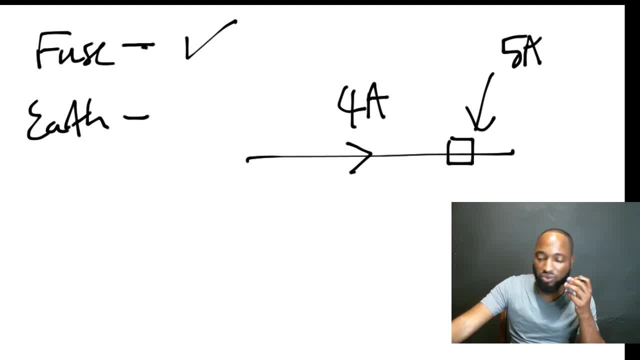 mechanical. it's mechanical, you know, when you fuse below my dizendo that meaning your shoes and as open with a fuse need to know your little problems as electrical hazards. y'all get check back. you get you add when not, I didn't need to talk about talk about it too much. press some lights anymore, your good guys. I believe ago. talk about it too much. press some like email your video, good, safe case by al implied invite. I can update you later and if you have questions it's related to this. you'll be great to me. but see you at the top before going to gonna get a video. we got a video ago. don't forget to talk about. talk about it too much. there's got a record. drinks on yourע. 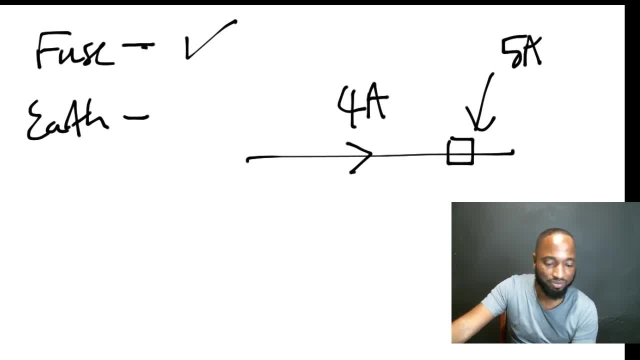 in the video. good reminder, good reminder, Ryan. but you press likes in the video. let's move forward, moving forward. so you have your means. you go to your circuit box, the fuse box, you go to your distribution and you go to your different appliances, house, house wiring. everybody should know your house wiring works. but 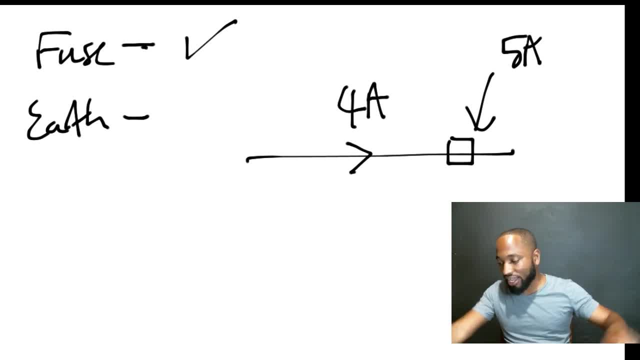 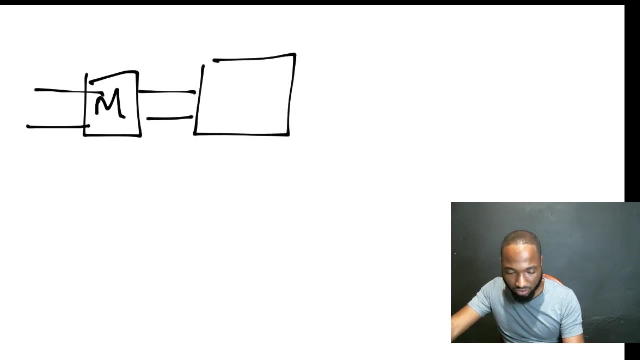 everything is connected to the ground. you have the live wire, you have the neutral wire- maybe I should just do a little heads up on that. so it means m4 means you have your fuse box with now, my power's in charge, you know, thank you, yeah, all right, so you have your mean suppose, and I mean, yeah, this use box, this. 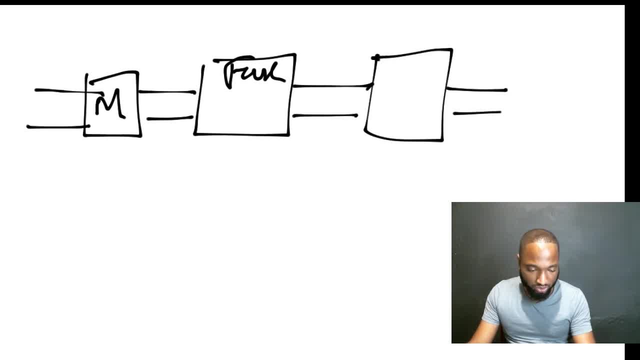 winter. what if I use them to distribute and then it's going to have plants? is this partner? you mess a shoo shoo man. you don't do it if you don't want to do it. if you're gonna do it, then you're not gonna do it. if you're not gonna do it, hey, they have a chance I'm gonna bring. 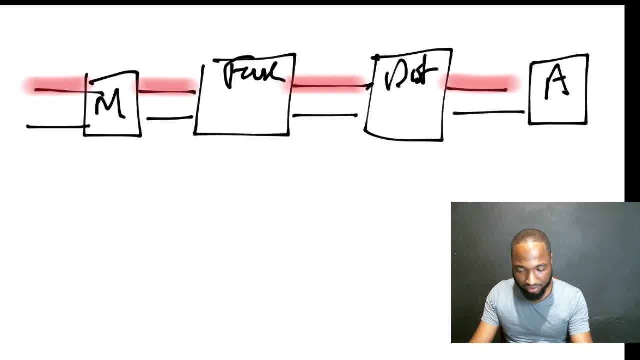 this on my channel here. boys, right, so you have your main. where's? the last of what I'm saying is: this top wire could call a live wire. you should have a neutral wire running. it is pretty grown again. that's okay. when you're going to your distributions you have a ground wire as well. so if they ask about us, 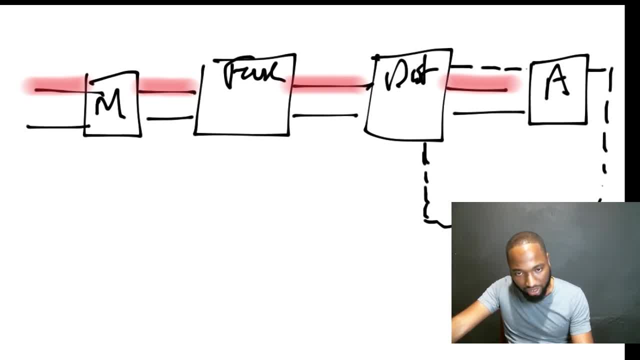 you know to label this. hey, I went, I went behind myself again. so you have your ground. this is a month of ground, that kind of thing, on two strokes, I don't know how for true. so you have a ground. so check your ID. you can check my ID right now. wait time: I think the check that getting my energy. 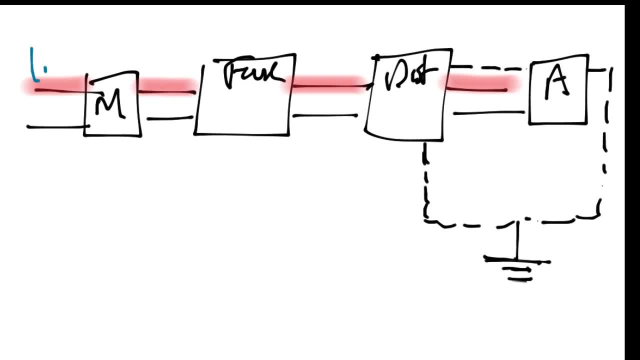 will just drain out and right. so this is your life. this is a neutral, so you feel that they would have to do that, though they're locked in the arm to draw, but you can ask it to leave it. this is your ground. every mean box, a fuse box, a. 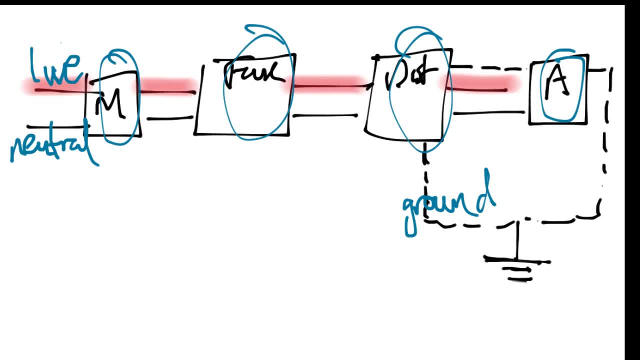 distribution, whatever, and this is like your plants like maybe fridge, fridge, right refrigerator, why's in the直? will take a nap and get back to us tomorrow. um no, no, no, no. it was very tempting. wait a minute. I need to get. I need to get this done now, because we're not gonna happen tomorrow. 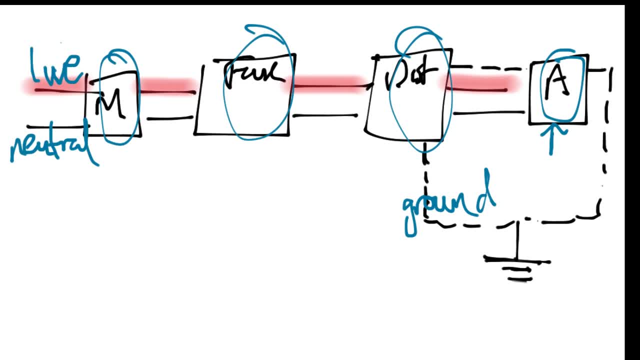 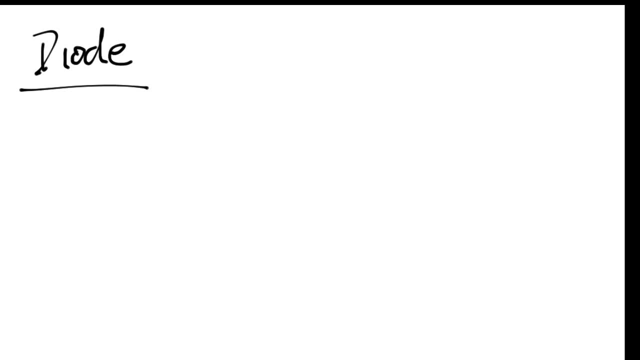 alright. so diode what's a diode? there's a diode, what is a diode I want to have. we wave rectification once again. this custom team. recently- i try my best to write- that day we got president, so we're taking a break. we can't take a break if we take a break. 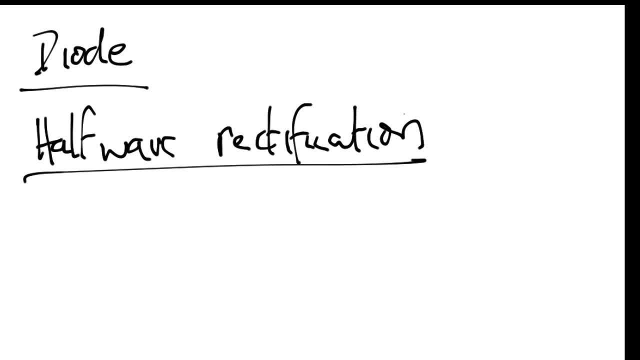 people will knock off going straight. we nearly done earlier. okay, we're not nearly done. we are about an hour and a half. is it time? yeah, i'm finishing 11: 30.. so what book you using? are using real books? is any any physical good? so the 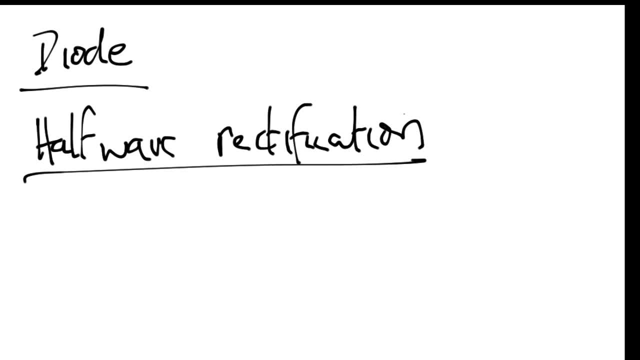 definitions: flowing in diode allows current to flow in one direction only, um. so i'll speed it up a little bit. i'll speed it up a little bit, definitions, and you can just pull it off your book. so the electrical component changes ac to dc, yeah, something which regulates the flow. 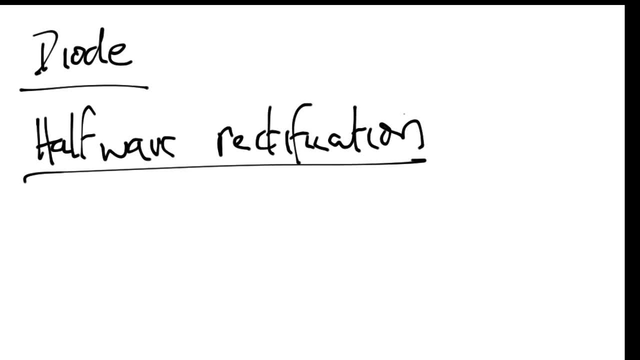 of current. now that two, that two, that two v, that one too big. after recognition it's going to convert it ac to dc using one diode. okay, so let's join in a second. i will. we'll pause halfway rectification so you get your idea what's happening. this is just a load. 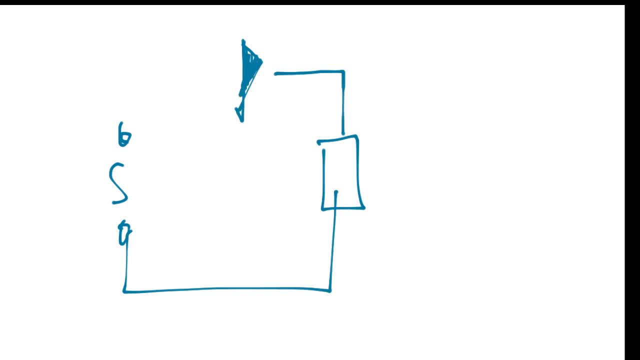 this is a triangle and that's lying like this. so this symbol here means ac, ac supply. the current is going like this and then it's going like this, for over at a hood it's at a frequency, so it's going one way. then it's been one way and it's been one name and it's been. 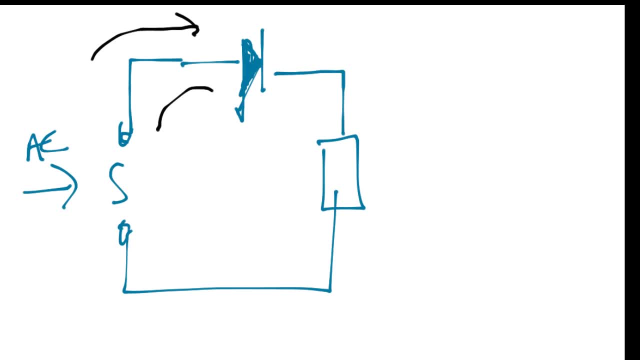 one way. when it go like this, it's accepting. so remember, this is a triangle and that's a line. this is a the supply. the supply would be looking like this right sign. you saw it all, but what we're going to notice here is that only when the current is going through, 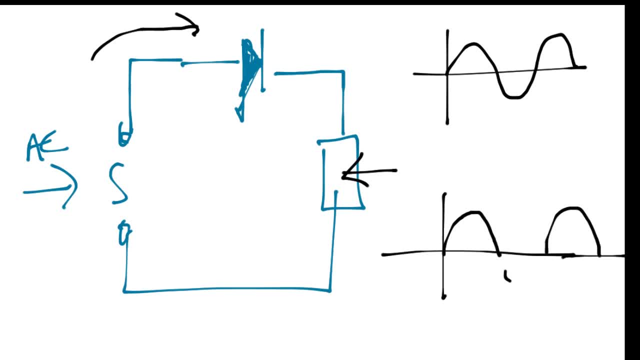 we get in it. when the current is going forward, we get in it. this part here is getting rejected by the diode, because the diode only allows current to flow in one direction and that's basically it. so this here is. it is a half wave rectification, this is half wave rectification and this is AC current. 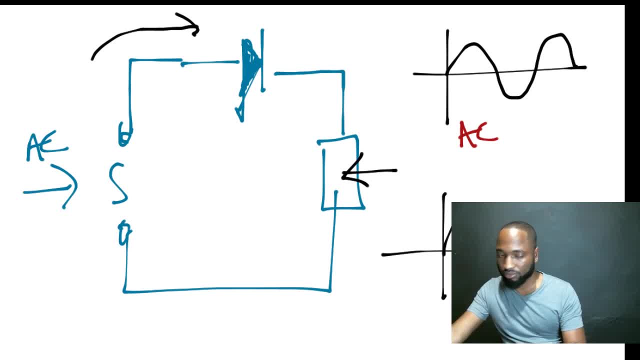 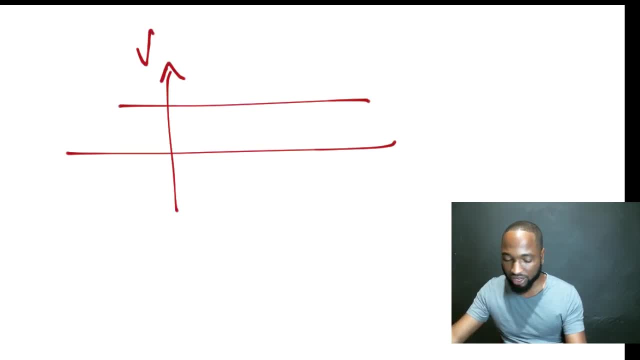 why is in the chat? and an example of direct current would be like that, right, by the way, the unit is voltage and time for current and anything. so we interlogically it's type of logic. it's what type of logic it is this? what does it do about? 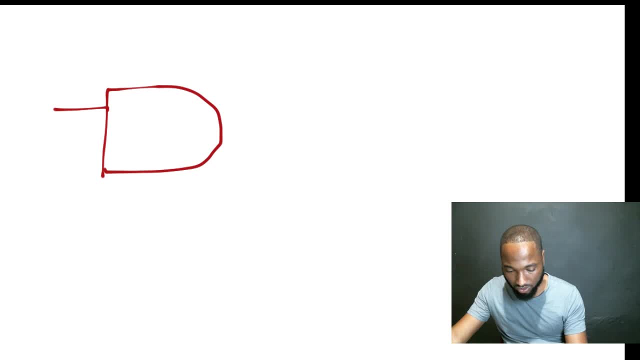 this one, so that's the first one. this one, this one, so that's the T one, and two specialty boys. so everybody seeing them there eating out of Jordan. we can also do need a map and we can trip table them where you really were. let's get these two tables. 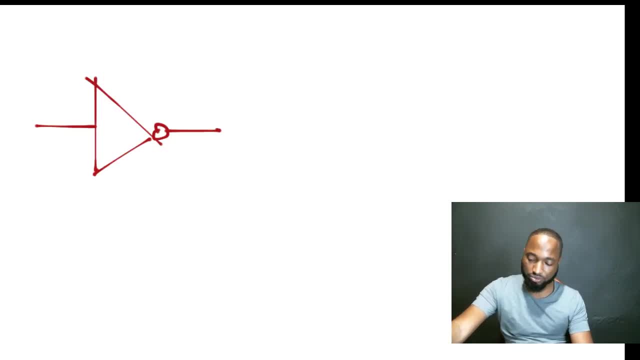 down. so do not get flips the input. normally even each table is set with a code. that's set with a code and then you get a code. you do the input to the input, which I'll put in at the end of the video, but this is all in the table. you 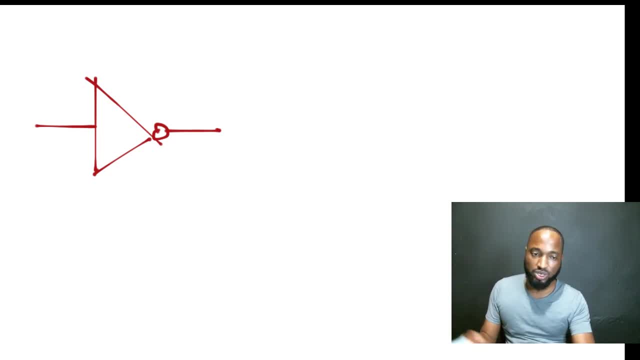 can see in the code. you can see the input is set with a node. so you can see the other tables. you can see the output. alright, so this is the input in. let's see if the thing it does label each thing. now, boy, yeah, so if I put this, if I put this X and Z, my 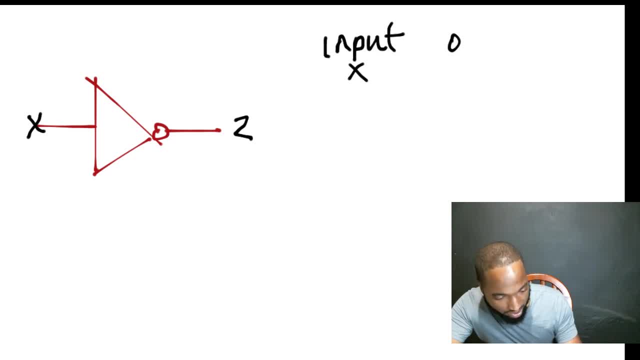 input would be X, my output would be Z, and if I was 1, it goes to 0,. if I'm 0, I go to 1, so the nut gate flips. the flip is a is a. what is it, boy? it inverts, right it. 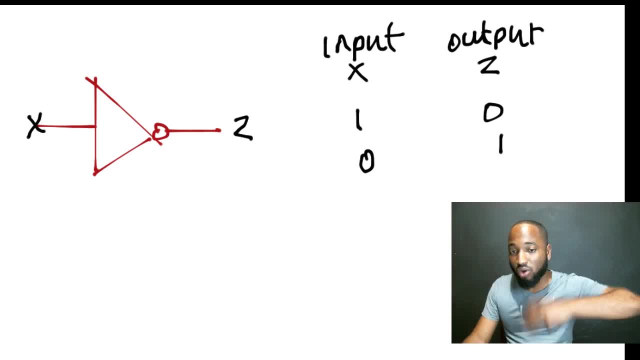 inverts, so the nut gate. if you are 1, then you become 0,, if you are 0,, then you become 1, normally we start off with 0 when you're writing a truth table. let's look at the next. 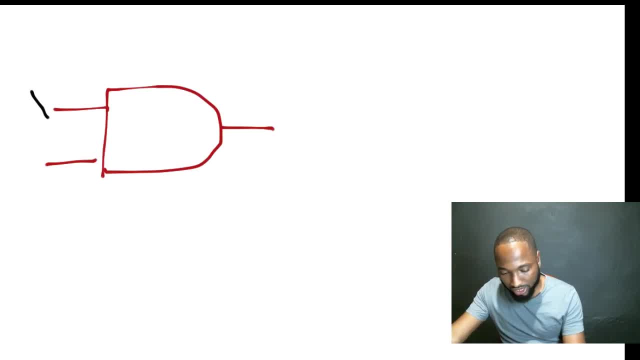 one. let's look at the and gate. so you make this X and Y and then Z. so we have two inputs. now we have X, Y. so this is just the basics. we do some questions just now. Z, so what I do is put 0, 0,, 1, 1, and then 0, 1, 0, 1, like 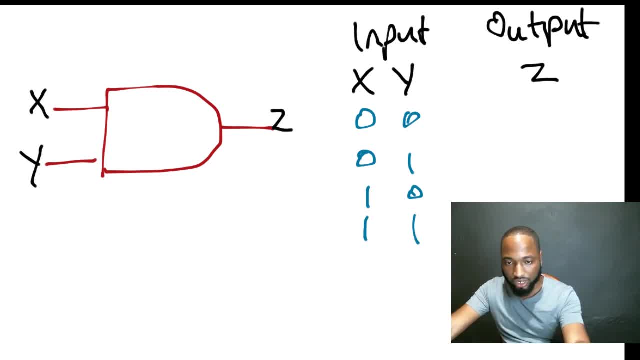 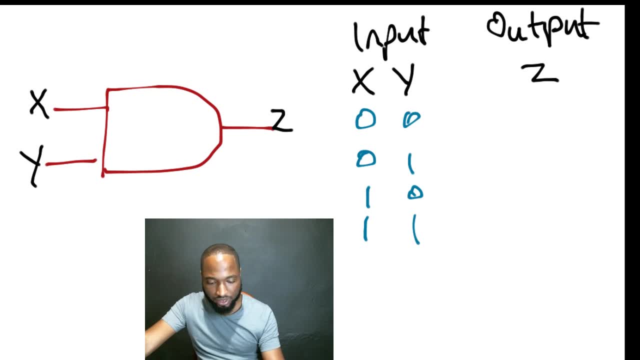 that right, and in this case I could probably come across here. so yeah, so I'm going to look for this part here. so what's the output going to be? Well, this is an and gate. it means both inputs must be positive, both inputs must be there. 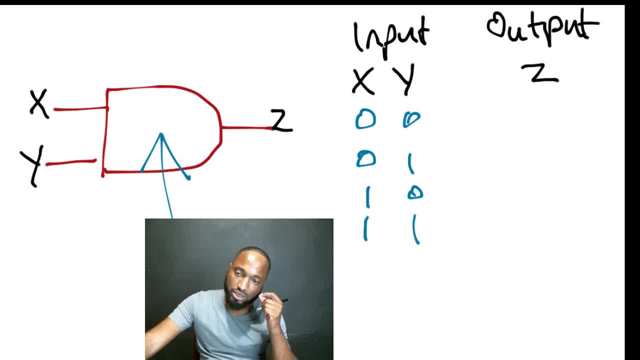 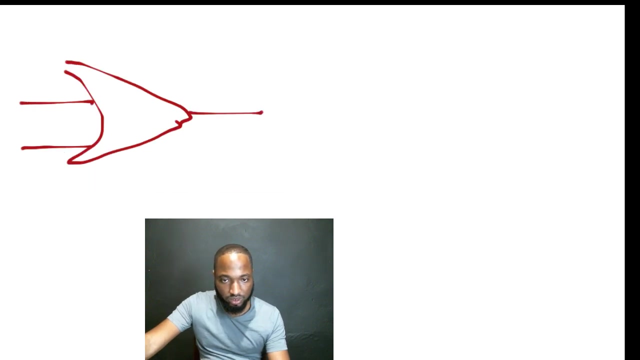 given of current whatever for an output to happen: 1, everything else negative. everything is not there, only this one is accepted. well, how do we see this? okay, and you know it should get back to me with this when I get s whoo people, dying people. that the input versus 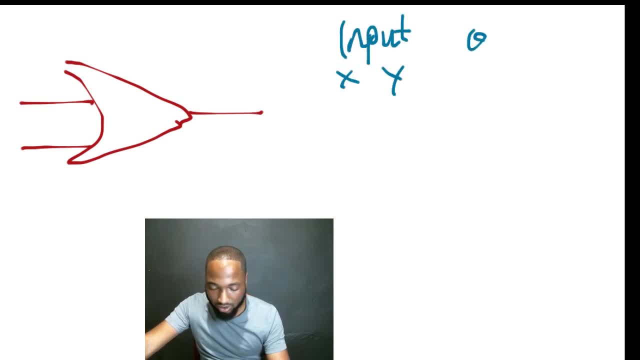 us before example, human Jackson here. why output is in fact is just increase. so zero, zero, one, one, zero, one, zero one. anybody once, once it about one in the dance- you'll get the output right. yeah, if you believe in the Netflix and chill, or just a chill, I feel in the. 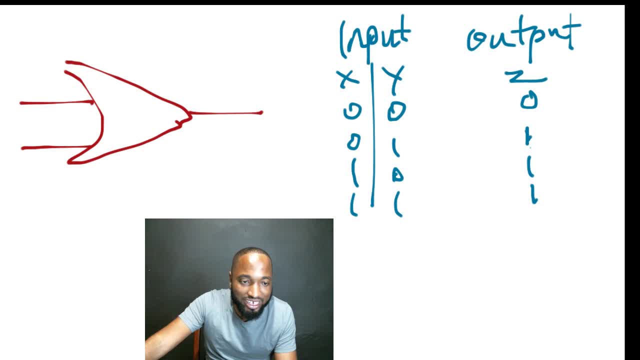 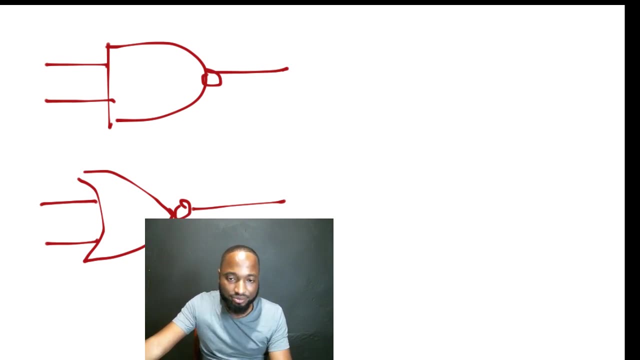 need for sleep creeping up. so when we're- when was, yes, both an ex- about time- when we're die-hard sitting where they had a plan, see, but no things rough, no things rough, no things rough. obviously, if people had a go and sleep, go and sleep. so the Nanda. the Nanda is like if a stick and not eat at the end of and so 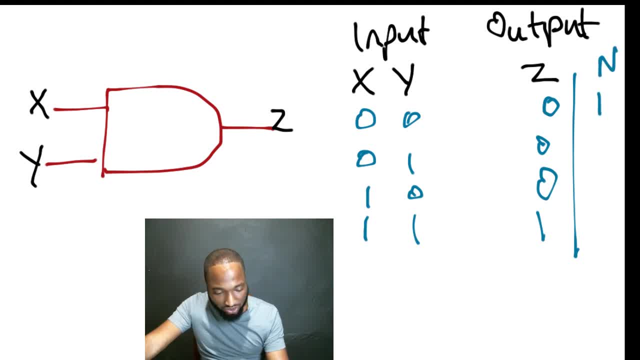 all of a sudden the Nanda. the Nanda is like if a stick and not eat at the end of and so all of a sudden the Nanda will changes. like that and that, like that. there's nothing Nanda's like if a stick and not eat at the end of the and me. so 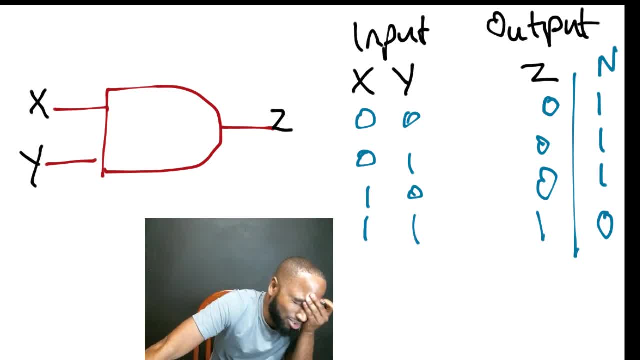 so I have lost. stops me triggered. stop saying your loss, see where. see what is the problem when you see loss was supposedly we need sleep. I sleep when I return from school, like that. all get right. So where are you lost? Where are you lost from What you don't understand, What you don't understand? You need to pinpoint what you don't understand, Otherwise I can't help you. Nand Geet is multiply X and Y and Y and Y. Yeah, wherever floats your boat, Whatever floats your boat. 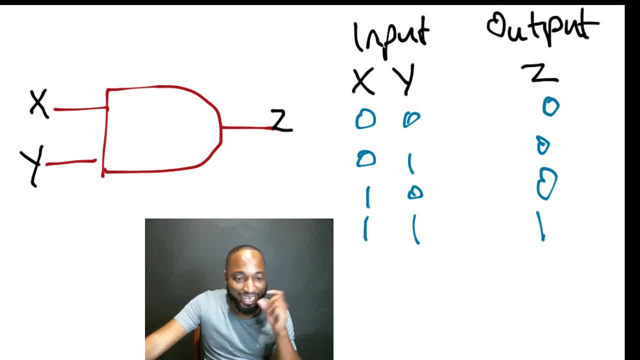 The best way to remember the Nand Geet. Yes, you are damaging your health when you don't get it for first, which is what I'm doing right now, But I will recover. I'll recover. This may be the last time I'm doing this like this. 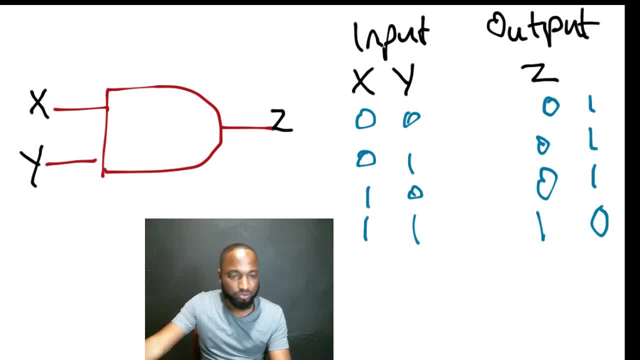 All right. So one one, one, zero, Right. So that's a Nand Geet. I don't like to think of the Nand Geet as not an N, and although Nand it makes sense, I like to think of it as and, and then you put a not, Somebody say everything. I'll help you when you say everything, Okay. So the Nand Geet is like you put a not gate behind the and gate right. 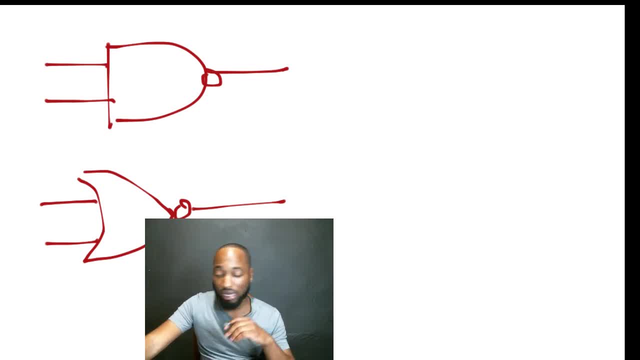 Somebody say you're looking for me energy some. That's way back in quite a while ago I didn't even remember you looking for me energy some. Okay, let's do a question on this. Best way to see it is Zip zap, Zip zap, Zip zap. Now, probably my favorite part of physics in CXC was these, because it kind of kind of fun just to look all these things Right. It's like a cool dog to map all these things to be kind of fun. 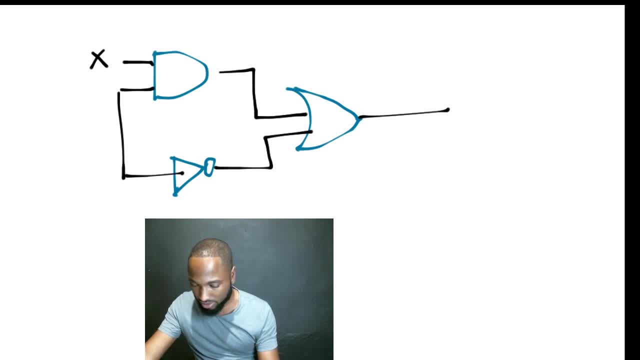 I know it's a way I think to see Why. So what is the question? Draw the two table, But I don't have a whole Right Draw So table. So it'll allow a few truth tables to draw, But in the end the truth table they really want. 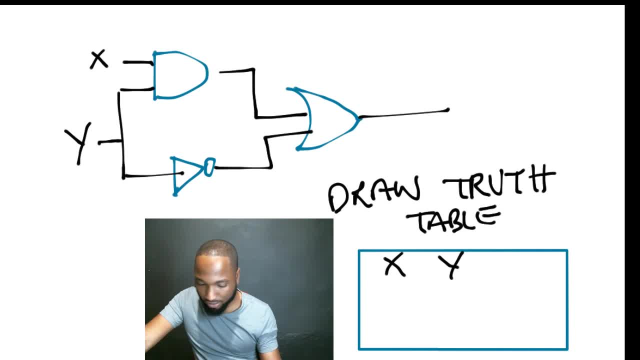 Is basically this X, Y, or is the end Z and the song some letters P with Q. See you don't see you lost. See what is boring. You give us location Y, which you don't listen, So you cannot keep you At. 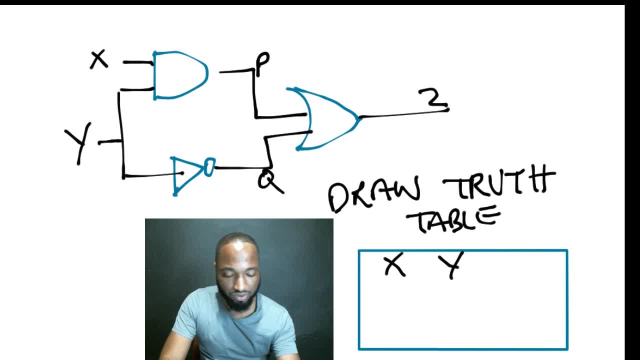 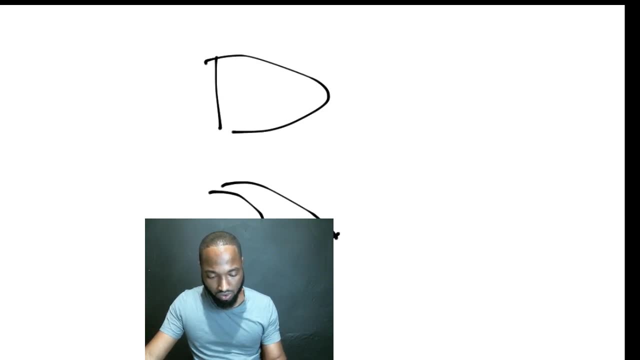 back- yes, that's what we should be doing- says he is missing. thank you, thank you. so see here, i just can't remember the gates by looking at the drawings. what is there not to remember is when he is only three things and or and not. that is it. that's it: three things to remember. 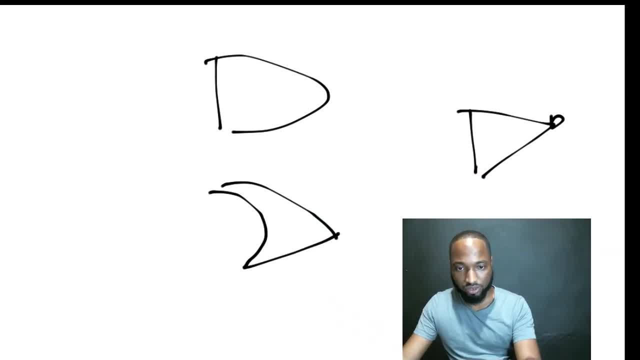 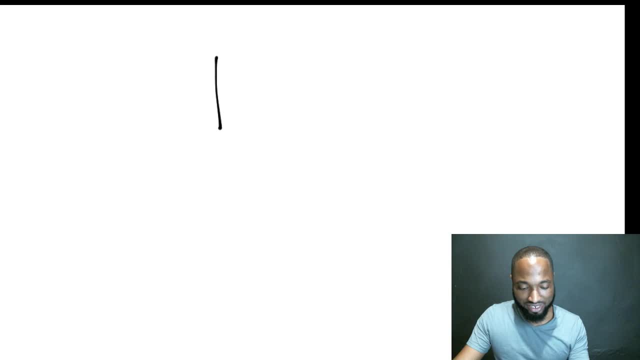 i'm gonna go back in the corner. go back in the corner. i'm so lost i don't even know where i'm lost. um, so, not everyone like you. i understand that. i understand that. i believe all those talking about this easy, this simple, not everyone get it like you. understand that, understand that. 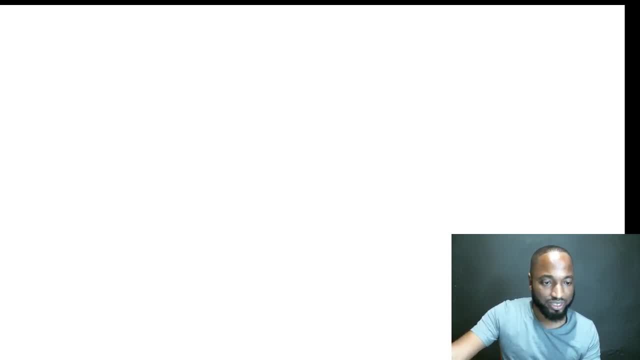 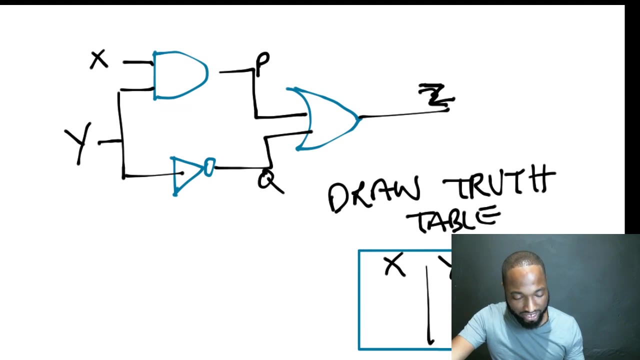 um, but this is common sense. i think ziana is trolling us. trolling a man, say he detecting trolling. last time i thought somebody was trolling, there wasn't trolling um. so yeah, we just got to get out of here here, z. this is what they wanted: the energy. they were able to follow the street cable. so those who 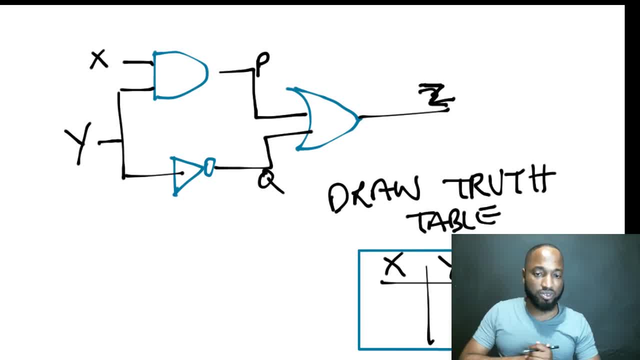 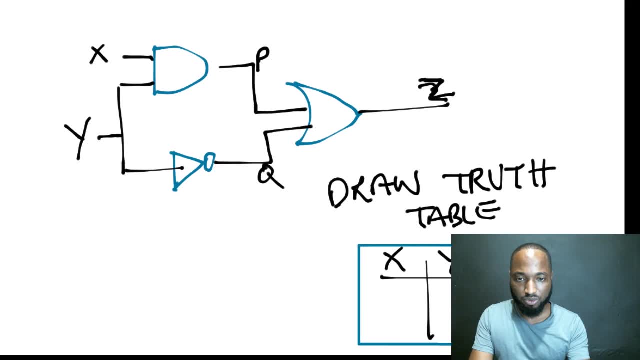 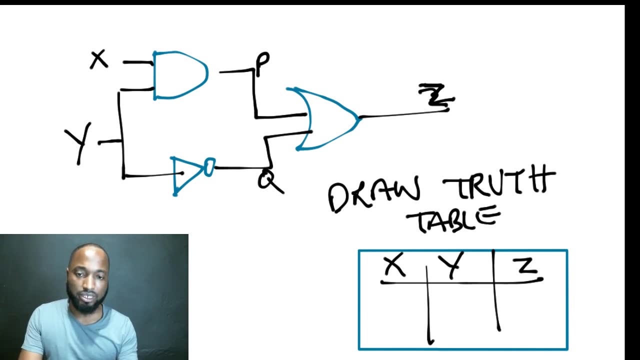 those who understand it kill it off. doing all kinds of things mostly come across here. so nobody. well, apparently that part of the book you're blocking again. so this is what it was. yeah, no one's looking at you, all right. so when we do all this question, hopefully some people who lost will kind of 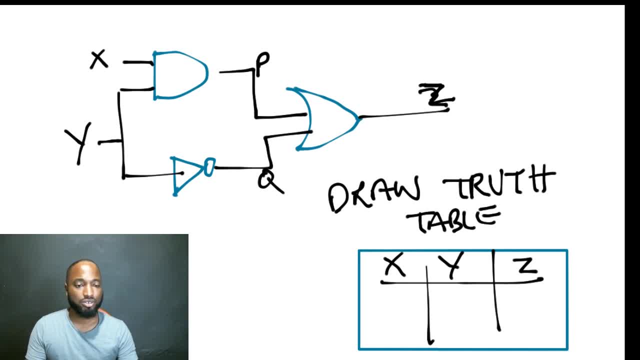 see a little, a little logic taking place here, right, so let's do all the questions. so we need x and y. you don't really need x and y, you make up your own x and y. okay, number 18: zero, zero, zero, one, one, one, zero one. that's how i want the x and y to work. three up on yourself there now. 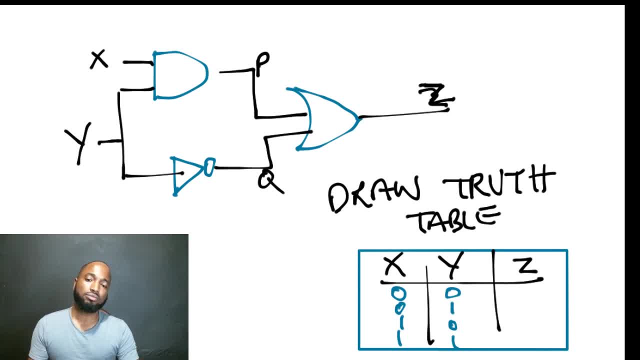 so you need to figure out. so what to do after cxc. the first thing you need to do after cxc is make money. you need to watch yourself in emergency not enough money make him. i seriously i tell my students that one figure out a way to make money. i can give you my whatsapp, my parents. 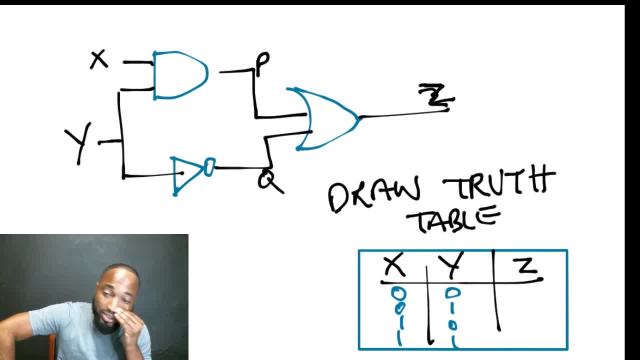 deleted my ig. i know what to say about that. i can't communicate with everybody at the same time. imagine if i come in. that's how much it have in here: 190. that don't have enough time. that's why i do this. good question right there. 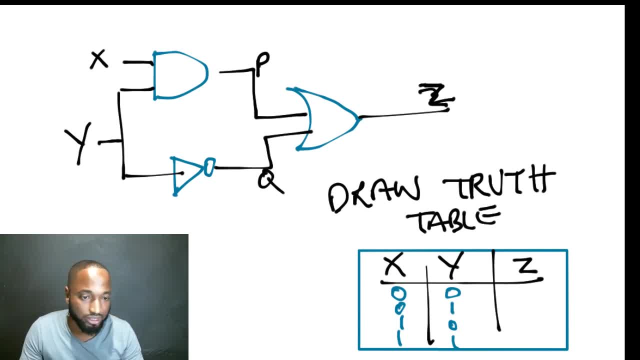 as you, and i see your number, but i may not be able to add you right. i'm very sorry. so you leave all the inputs. no, look the inputs right here: x and y id. anybody plans us? yet this person's thing? us Z is 1 0 1 1, 1 0, 1 1. was that really good ones? your own? yes, that is. 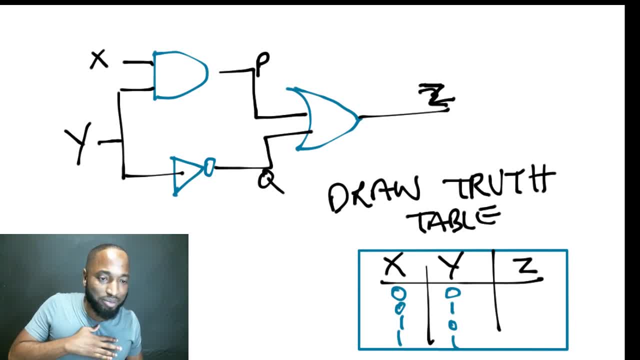 correct chat Chan Chan, whoever. Chana, Chana Chana, I will get shot. a sorry for pronounce the drum, luik, I saw your answers, bro. it's correct. yeah, and I saw your number. I didn't attend to add it right now. you could probably figure out my email crew in spring at ttf, gmailcom, and you can. 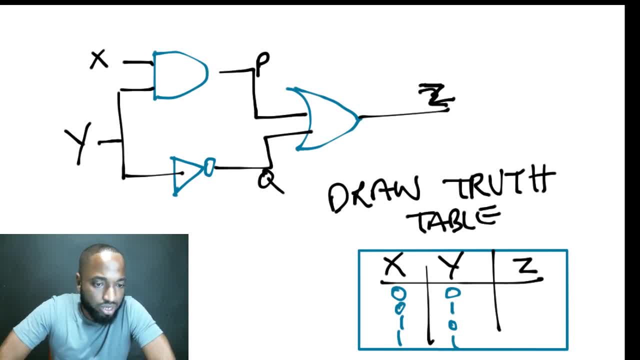 email me right, 1 0, 1, 1. I have. okay, it's Luke's Luke, Luke, Luke. what a spell in my friend. all right, so look others really up to the key. oh, we knew nothing. it's okay, let's go on with some people honestly. that's how you get why, how you. 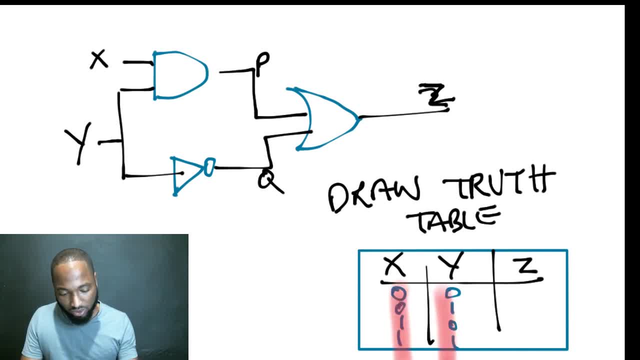 go why. why was given. those are the inputs to the answer. how you get why. how you get why. why was given. those are the inputs to the answer: how you get why. how you get why. how you get why. why was given to the answer. how you get why. how you get why. how you get why. why was given to you X and Y were given. 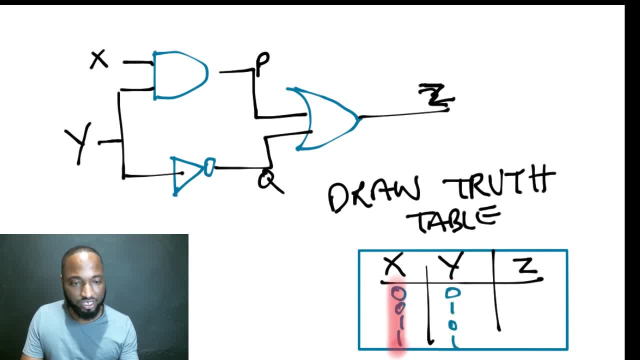 Chana Adi a Shana Daniel. so I seen you and people get on answers. now only you just answers. boss, then at all. the first thing we need to map P and you need to map out Q. you need to get a true table for P and Q, P and Q right, so you can. 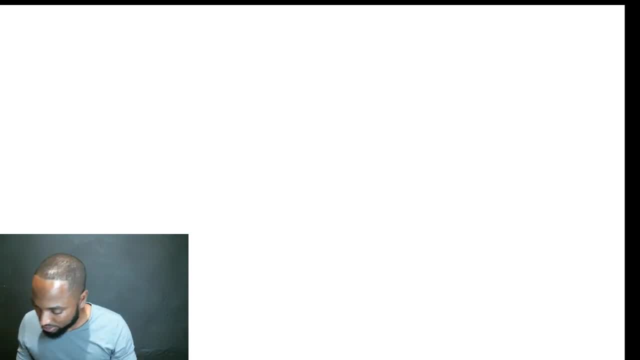 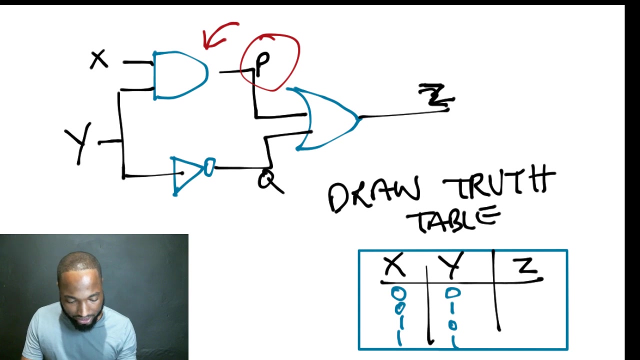 work with us, by the way. so let's draw. the two tables of P need a line, so watch NP. we see NP coming from what Kiper gave. this is: this is a Andy this speaking up here. this is the why, this is really why, and this is X we. 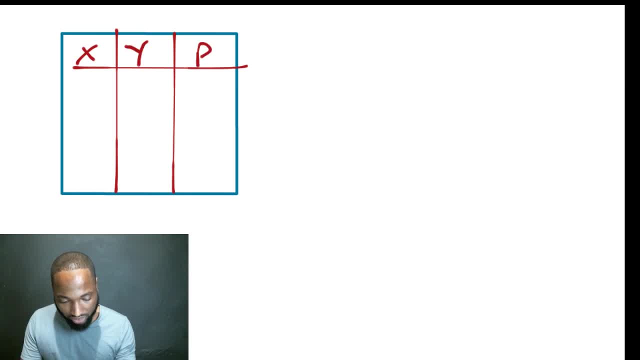 have X and Y as the inputs here. I'm trying to figure out what P is. so you use the inputs given: 0, 0, 1, 1, 0, 1 0, 1, and if it's an hit, that's the angle motor становится a great. so good, we have a quarter key for that in the back pocket. 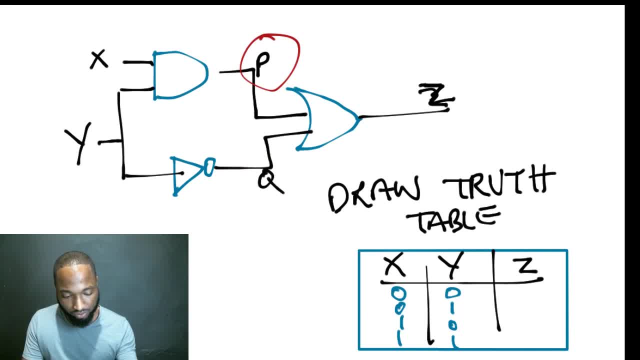 that's good. we have a input for key for that in the back pocket. now we need the input p if you can completely filter fl WiFiffen on any mother instance. back to input for Q. so looking at Q, we'll see that Q just has one input because it's 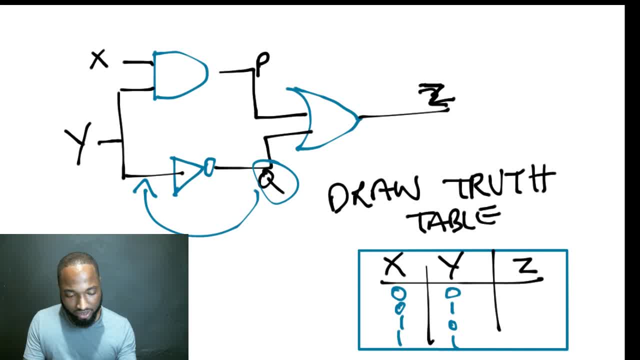 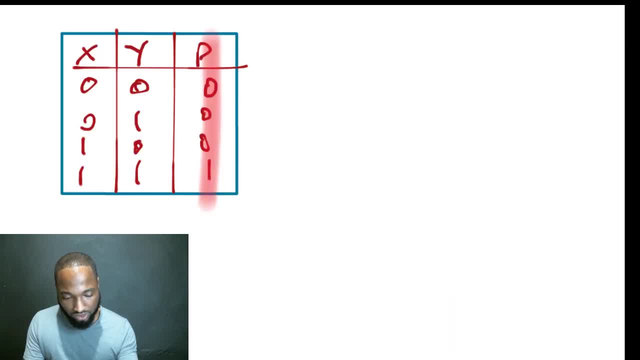 a nut gate and the Y here. well, we just use the Y inputs that that was given here to look at what Q is. so let's draw that once you give up your field and that people's just dropping troop bombs in the chat here by troop bombs. so 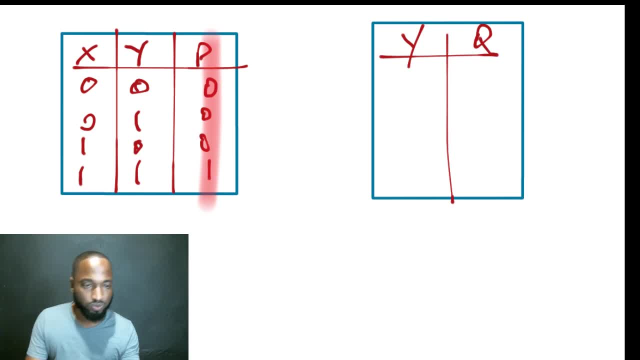 why Q? I don't. one of the things that a teacher is, he's had to understand where a person losing out and then help them. so that's why good teachers is behind to get good teachers. some teachers good at explaining something, just not good at figuring out where you losing yourself. the teachers are real skin and that's. 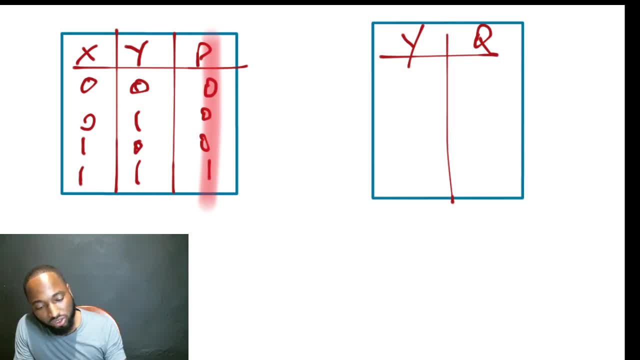 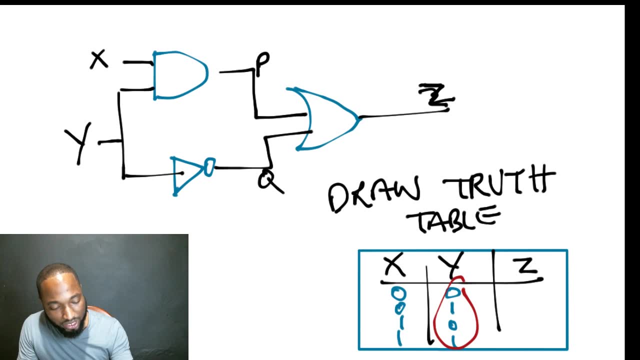 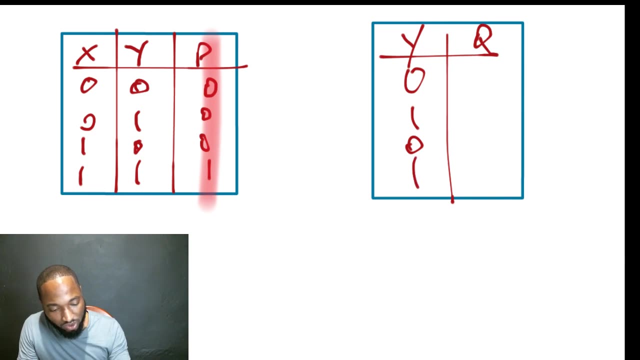 why you need to help them yourself sometimes. so remember the important why was given 0101? we have to put it in that order so that we don't mess up when we're just pulling audience up. zero one, zero one, right. zero one, zero one, and is that not it? so all I was 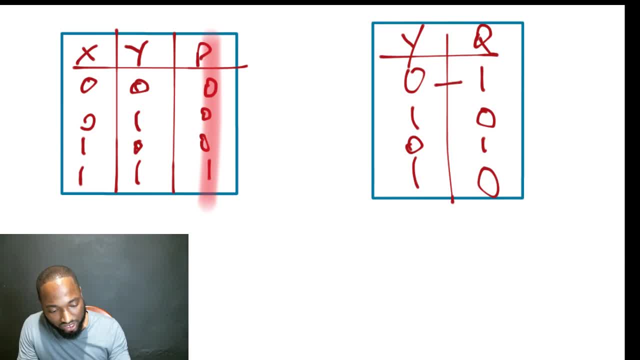 at in q is gonna be one zero 1, 0, one do you not get is flipping it right. so that's the input of thing. this one here was that and this one here was another. I should probably add a little more to this side there, right. 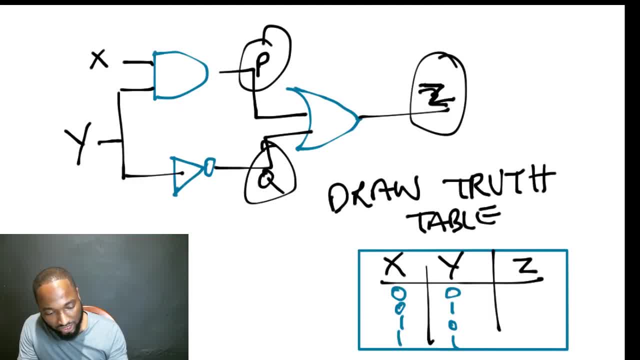 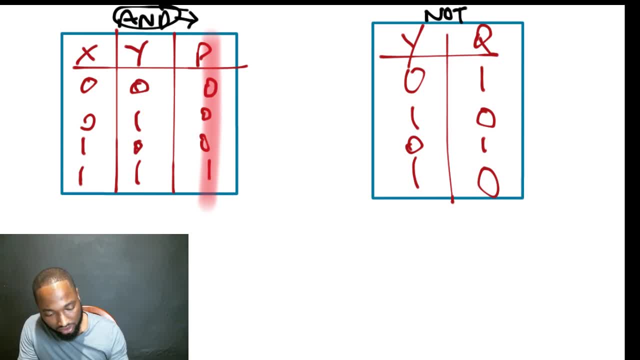 So what do we have? We know P, we know Q. now we just have to find Z, because P and Q going in there to find to make Z. So one more table and we're done. One more table and we're done. 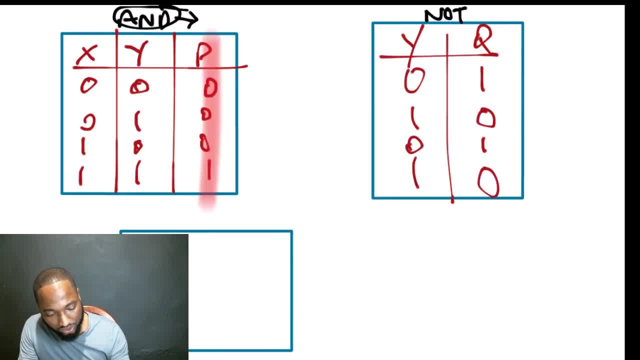 What kind of gate this is, though. OR there's a OR gate, OR gate, So WAP, WAP, WAP. we put P here, we put Q here. You know, P is actually three zeros and a one, and Q is actually, you see, Q over here, Q. 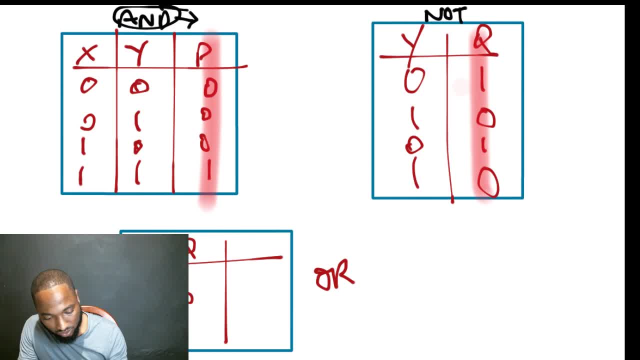 is actually one zero, one zero. So the OR gate, the OR gate, FAC, FAC Forces and thermal physics come in the Huckelau graph. Also reactivity, with Einstein equation coming. Alright, Luke, if you say so, Hey, I'm lucking. 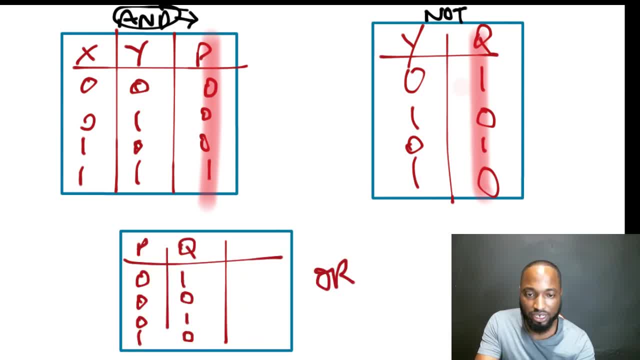 Thanks for writing that there. I saw a custom bean in the next corner. I draw that there. Sorry about that, people. I'm going to replace it. I'm going to rewrite it, So P. I got the input for P. I got the input for Q. 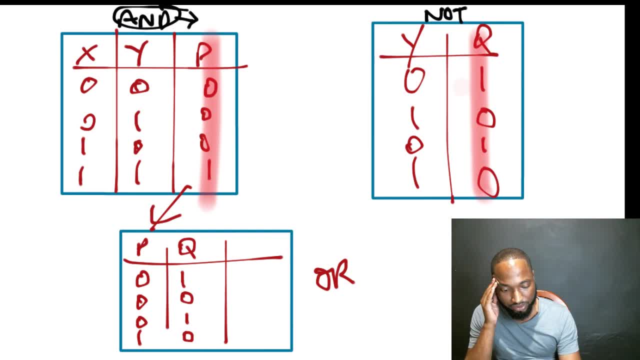 Oops, it went out. I put it here in my troop table and the answer now has to be dictated by an OR gate. So OR means: once I've seen 1,, put 1.. This other is 0, so I have to put 0,, 1,, 1, right. 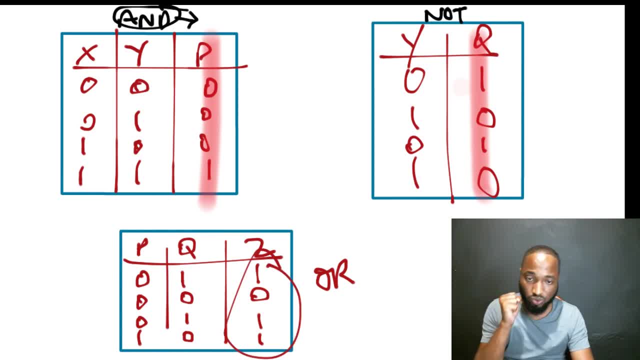 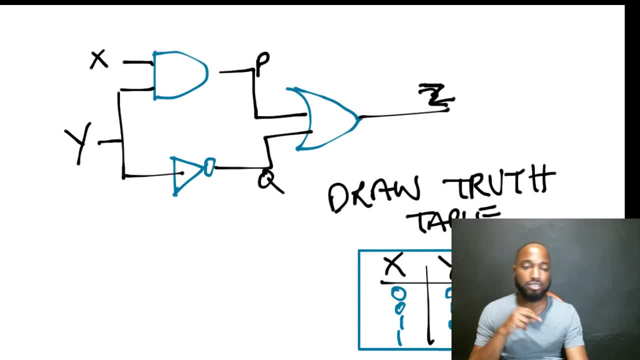 And this is the answer for Z. I can safely take this answer just so whole as it is and put it here now, because I kept everything in order: 1, 0, 1, 1, that's the answer. 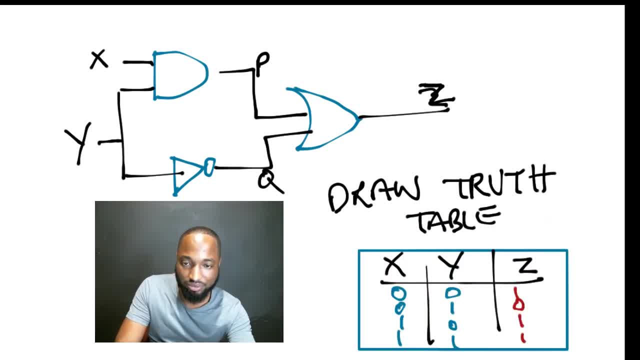 Why is it in the chat? I need the green screen. I can't do it again. Yeah, I had the green screen before but my lighting. I had another light and a green screen board from somebody and I gave it back to them, so you know that pressure. 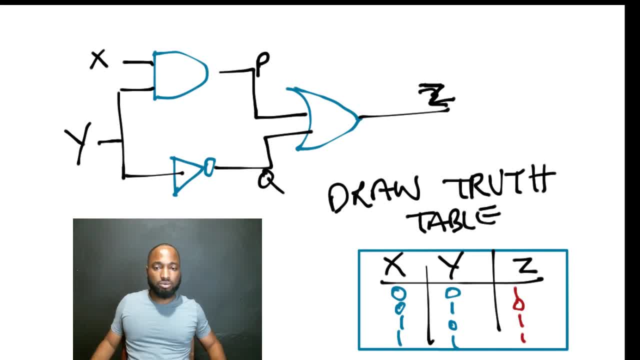 Why is it in the chat? You need proper lighting for your green screen. right now you have my ring light, so pressure. Okay, Can we move on? yeah, let's move on. you all want another one. I'm not doing Newton's. 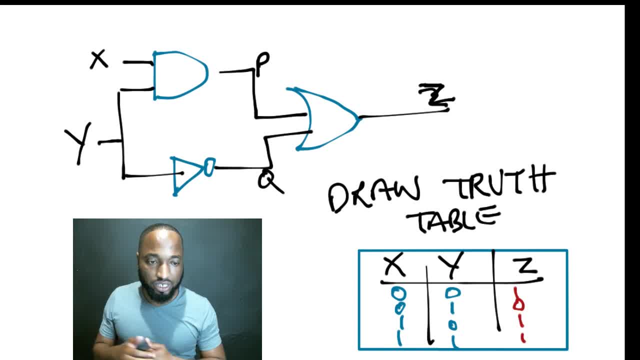 Laws today, definitely not doing Newton's Laws today. coming from someone who came out of depression only October last year where I was even hospitalized, right now I'm putting 10 mental states where I am now. it says a lot in there. do not give up, no matter what. 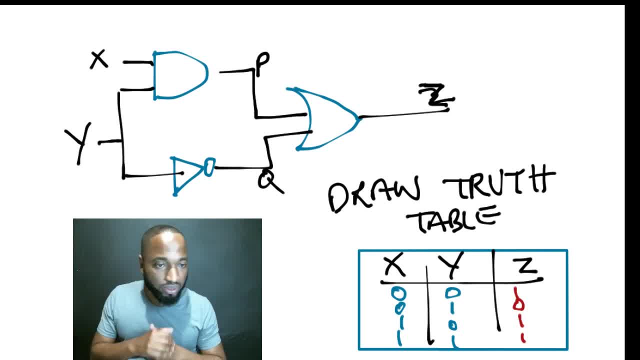 I think that's a good table for you all. then your book has concise revision, of course. it's really helpful, right? can you do kinematics? hmm? so all them Newton, business and things. another day you have to try some more logic gate questions. I'll do a live tomorrow, but 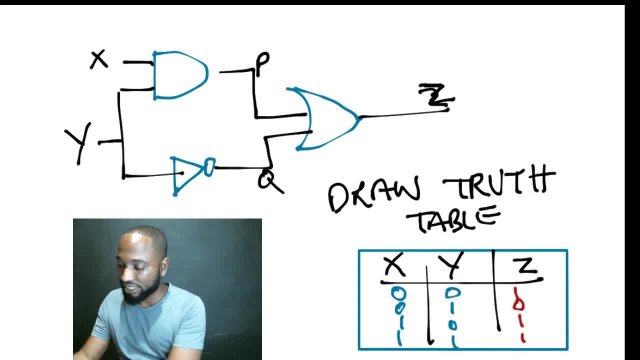 I'll do a live tomorrow. Okay, Okay, Okay, Okay, Okay, Okay. So I still have the old magnetism to do, but it's kind of like a render juice there. That would take me like about one or two hours to do, between one and two hours to do. 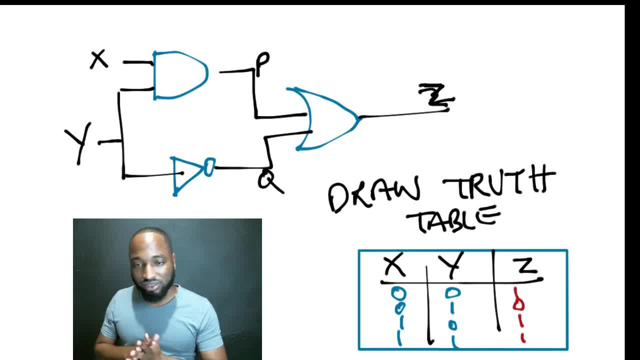 We did all of electricity. that's all of electricity and logic gates there. Alright, Let me see some one more. One more in the chat, if you can go on. let me see some ends in the chat, if you're ready to call it at night. 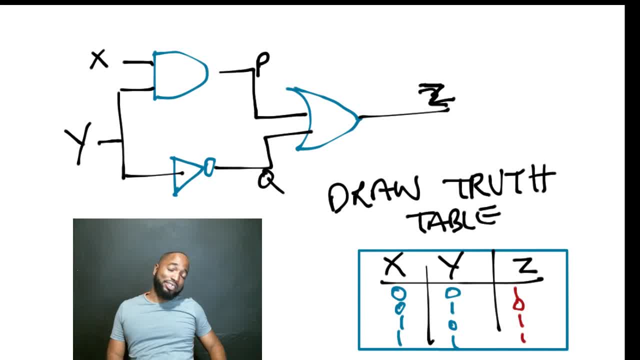 if you can do that, magnetism tomorrow, before i do so, before i do it. or integrated science, why isn't the chat for, if we going on or like we're going on, people out here, people are people ready out here. so definitely ready, i'm ready. so let's talk about magnets. i'm going to skip out the whole of magnets. 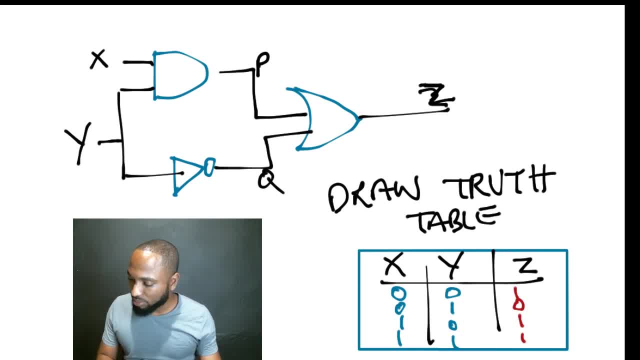 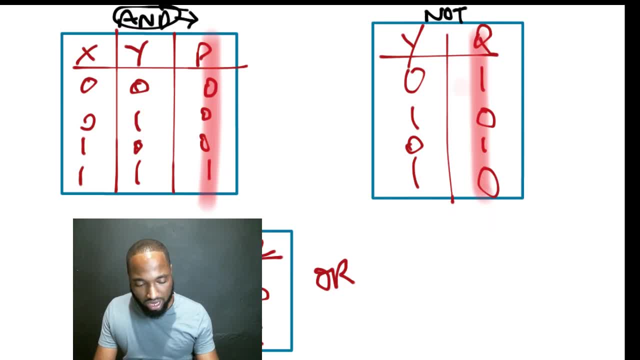 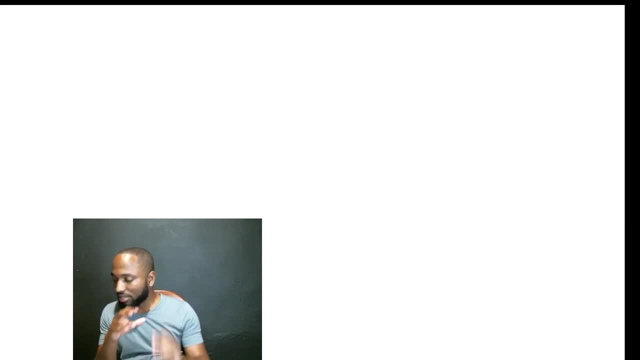 because i honestly find i read- i'll just mention some key points, and i'm skipping out magnetism- i just keep learning little basic pattern magnets here. so some key points. magnets exist, either attraction or reports of force. like forces attract, sorry, like forces repel. like this happy hour, happy hour. things are starting to happen. 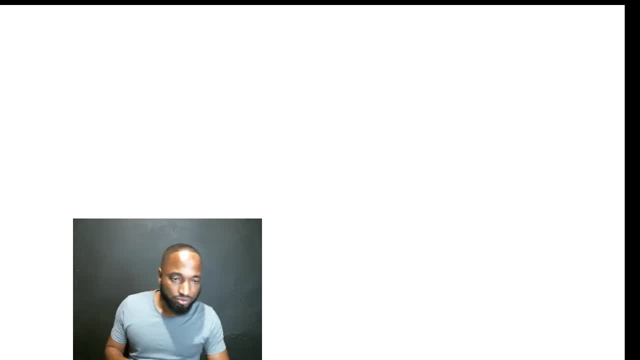 different forces attract. i don't drink coffee. different forces are trapped right- a free lease. if you hang a magnet like this and it's suspended freely, it will align itself: geometrical north and south, geometrical north and south right. so the two ends of the magnet is like north pole and south pole. 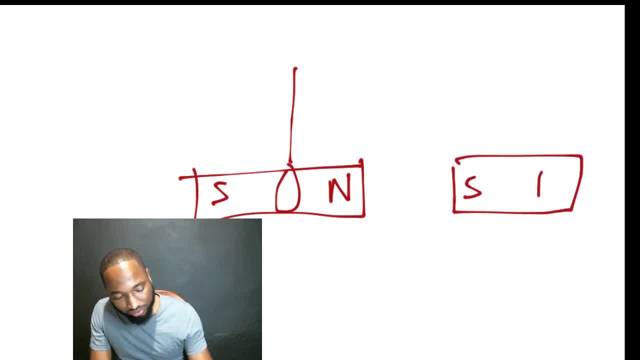 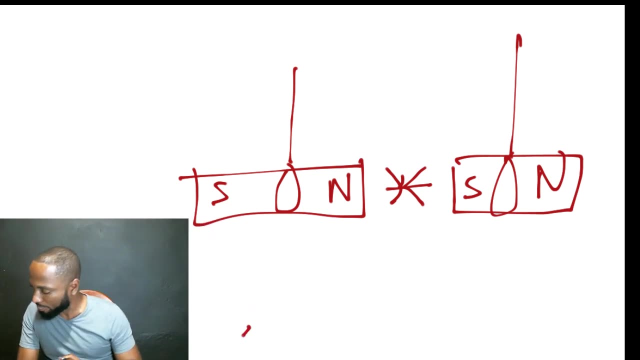 the closer magnets get to each other, the stronger the forces of attraction will be. closer magnets get to each other, the stronger the forces of attraction is gonna be. um non-magnetic materials can get. obviously there are different degrees of magnets. it's permanent magnets and temporary magnets. what is a temporary definition of a temporary magnet? 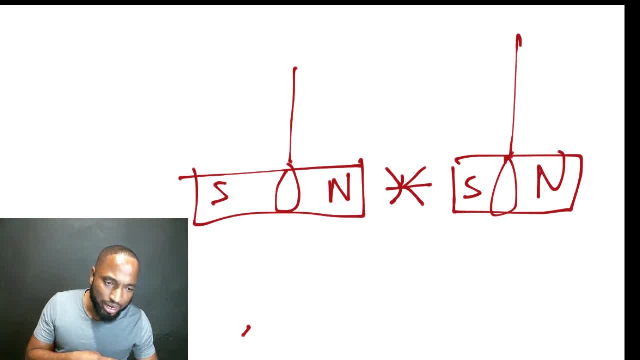 definition for permanent mind already do circuits. why is she asking me to do circuits, though, but already do circuits? i did circuits with the circuits when you have this phone. that's making my nose ting. the circuits is when we have new the resistors and thing magnetics. magnets get attracted to magnets. 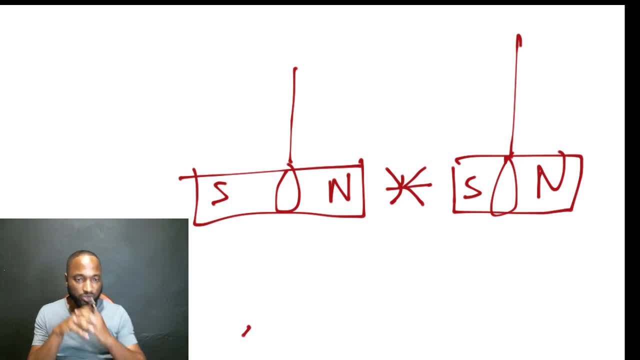 each other by magnetic induction. so we see any definition of a temporary, any definition but women, and by kicks, permanent magnets. when mm-hmm takes, I've any definition, vision, King of the definition, as the definition of a temporary. oh, well done, kicks. well done, kicks. all right, what else way, what else? oh, how can you plot the magnetic field? 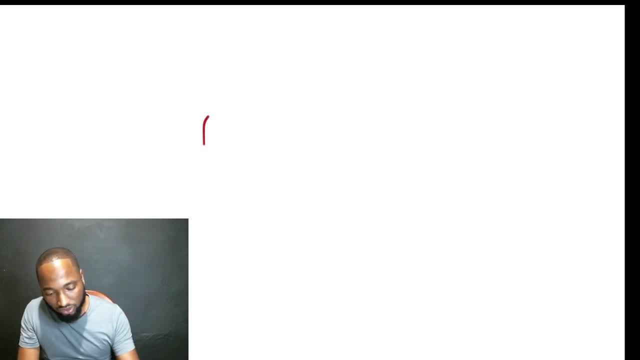 around a magnet. how will you put the magnetic field around a magnet? so, like, see, have not. and so what can we use? the plot, the magnetic field around a magnet? yes, it's going to move out, you know that- into the song. we know that, but what do? 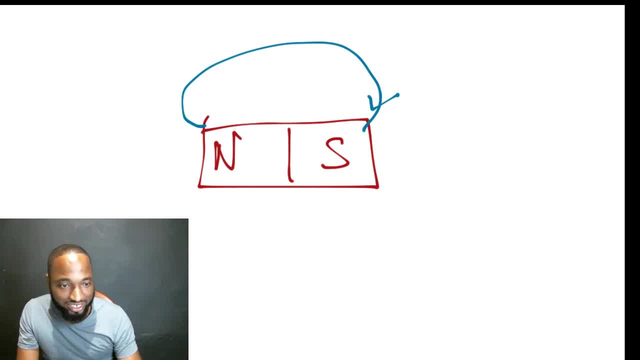 we use. you can use the compass method. very good, you said: yes, that's not. it has some people who just jump out and see the correcting and just go back in to hide. in fact, I pull out right, so you can use the compass method when you understand. 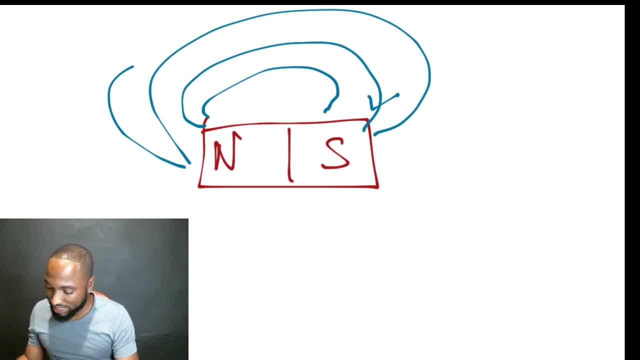 I really not in tools to draw this any better than this actually, so I just draw it shortcut. I just got two lines like that. so you're going out, we not. that's very important to remember, especially when you start to go into solenoids and generator. Fleming's left and right. 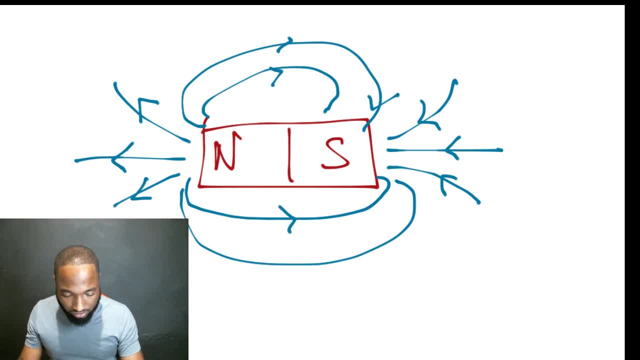 right and repent of anything. how do you not into the salt? one more thing: what is our neutral points become post method is very a compass and put down everything. she's taking small compasses and please the never nil go along the magnetic field and it has drawn away nobody proper. so point to what is the magnetic field and 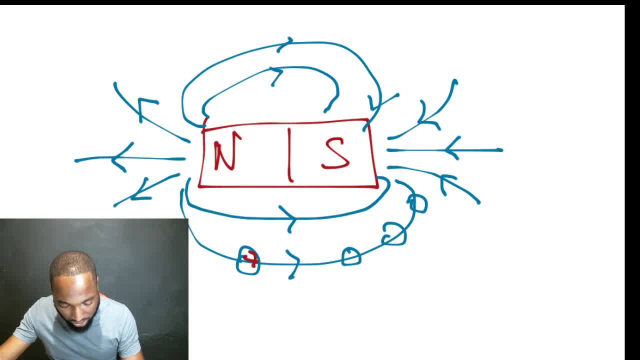 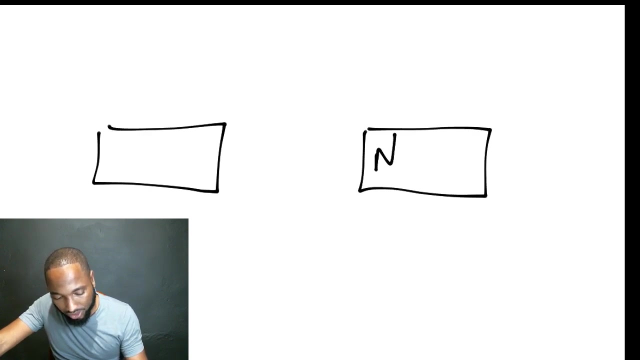 it has drawn out this song. so Luke's Luke said what the new definition of a neutral point is: appointment have no matter the field, a point where no matter if he is acting. and that happens when you have two bar magnets like this and they are the same. 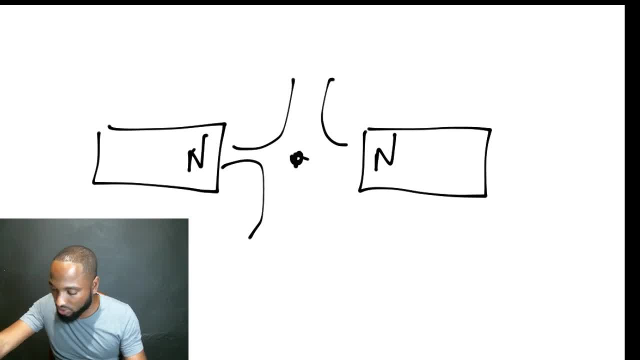 and boom in the middle. they call a neutral point in the Sun was he might be winning. so if you play anything head when move neutral point, it's like what was like a cancel out each other, right. so that's the basics. they know we could winter thing that actually. 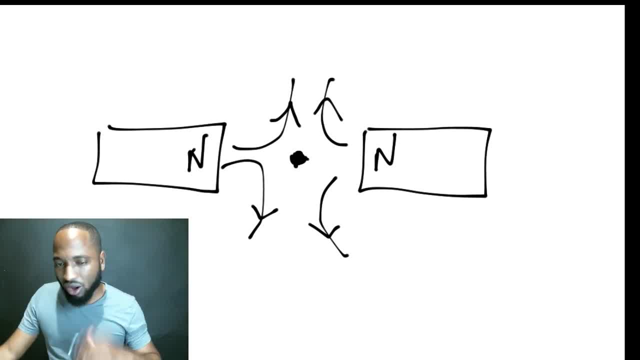 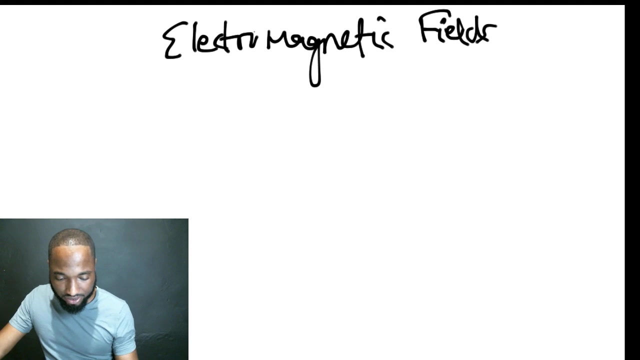 must notice, catch a magnetic field, remember all the north into the south. once you know that, you see right. so he's catching electro magnetic fields, now natural magnetic. so what are the electromagnetic fields? electromagnetic fields: you need to know to chat, don't need to know to sketch. 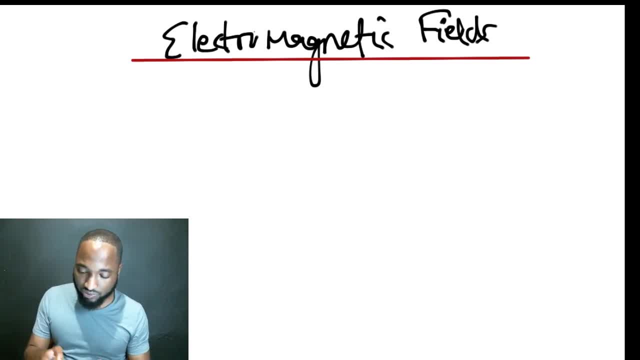 never appear Irish, but that electric fields. we need to know the sketch. people see it's dirty to mention you in their story. all right, see it's a dirty you, you. I don't see no answers. you need to know the sketch. see people that instant, the solenoid. 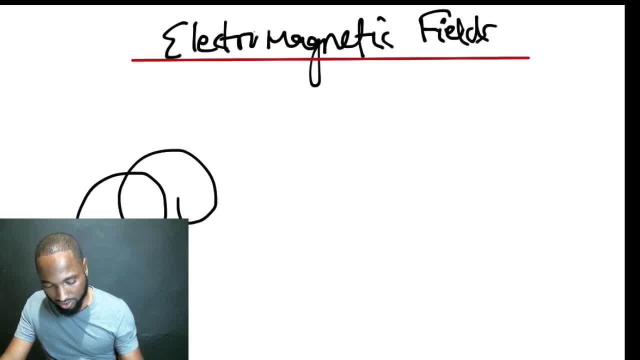 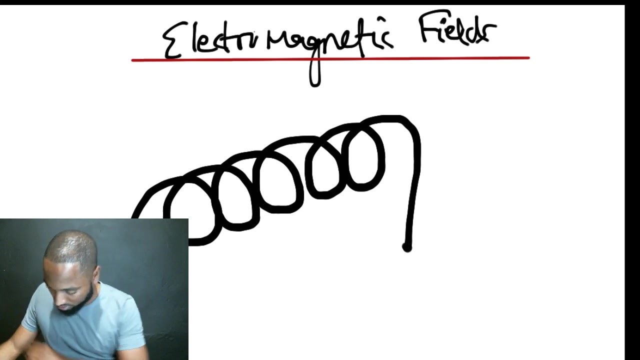 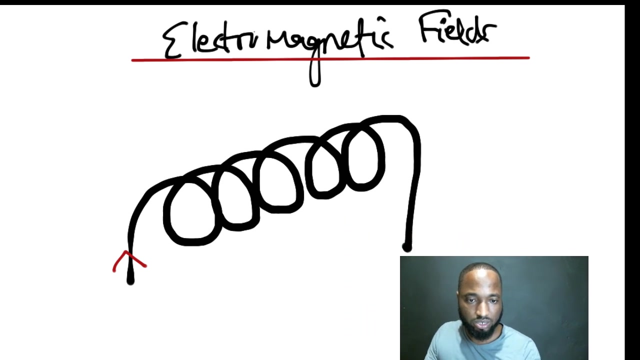 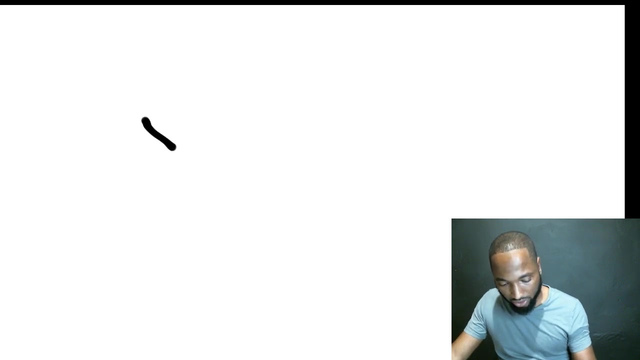 you. I'll just talk about the solenoid. that's kind of lucky, maybe anything to use a bigger right. so that's the solenoid. number of current is through in here. you, you, you, you. you need to take out of the paper. what else thing is it straight conductor, so like it's kind of going up? here was he field. 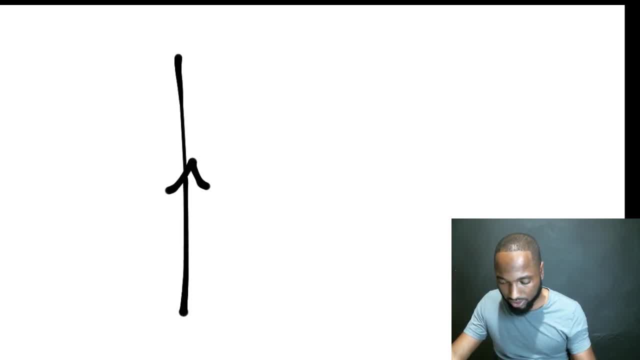 straight conductor. so you're gonna do all of these. you're gonna do all of these. we're going to do all of these. in our potty, George women sat a fee or not eating because he feel shut up. so you're gonna do all of these. you're gonna do all of. 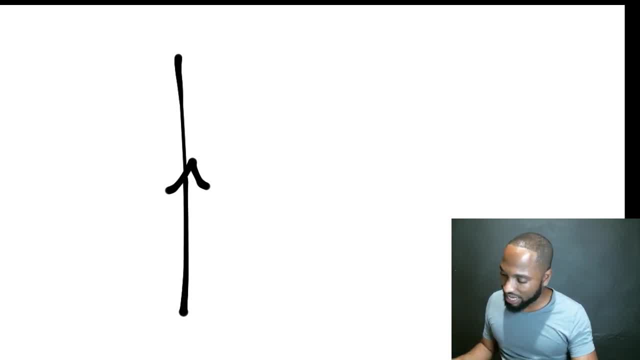 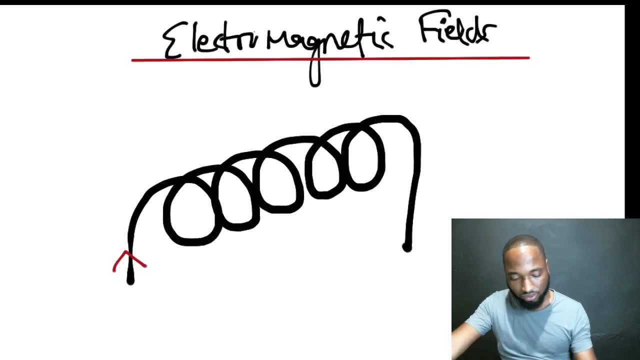 these, you're gonna do all of these and I fill our apology, or chairman, I feel not, I'm not feeling much assembly like. I get useless. it great. you off my ass. see you Like again useless, All right, so let's do this. So what I remember with this solenoid from ever since back, whenever. 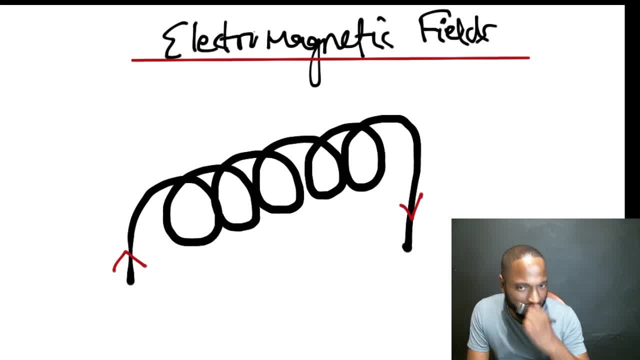 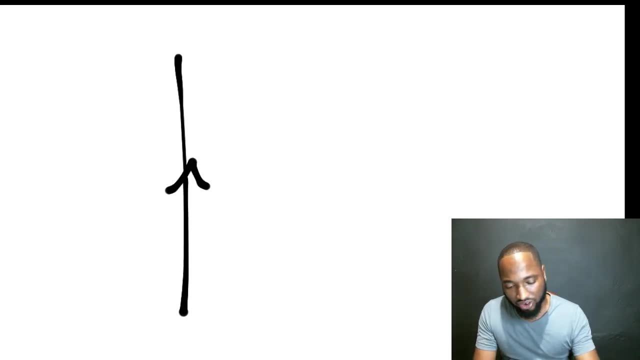 You need to watch which direction the current is going now with these electromagnetic fields. What happened in is that current passing through some wire and creating a magnetic field around the current carrying conductor- A Roller current carrying conductor to here. So that's what happened: current carrying conductor. This is a feel, a tingling up. 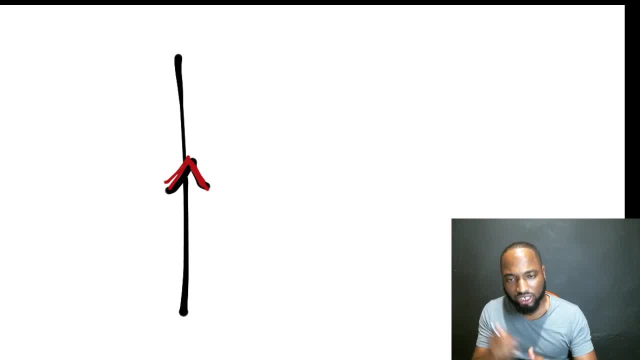 So like this one is the easiest one to do, Because it is one- is your right hand grip, Right hand grip, right. So there's the right hand grip, There's the left hand rule, and then there's the right hand, Fleming's right, the left. So, moto, you write this for generation. 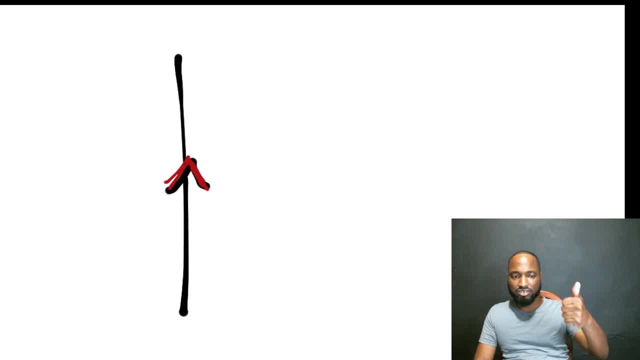 You write and grip is for just fields, So you need to get that down. you write under the first one. You're seeing about the first one. You'll come across right and grip. I know left and get ready. Do you write anger? And The left hand rule with Fleming's is the one. the second one, you'll see. that's when you started. you like motors most book. 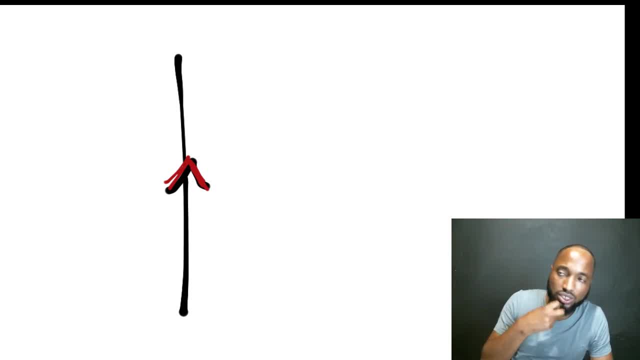 This will be second one. You'll see that's an idiot. motors right-hand rule is for generation. that is When it's again. that's an enemy opposite. in a create any current We left hand rule is an attic in the current to make motion. This one is when you take in motion of a magnet to make current. Okay, so let's go back. 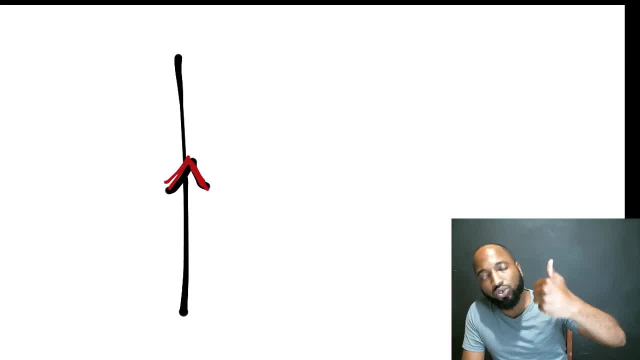 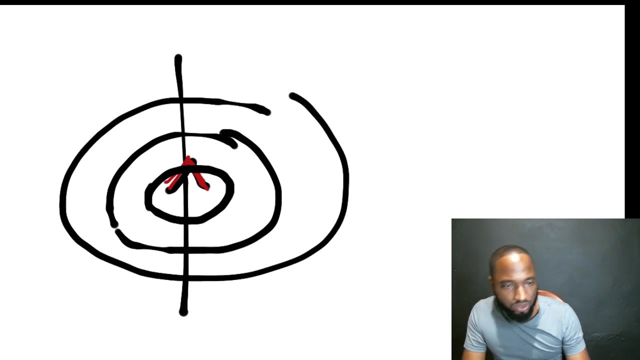 Let's come back into joining electric fields. so right, and grip means of your whole onto that, Latting over the, and then you'll easily see that your fields are going like this. See the next thing in the book, but I don't care. So which direction should it go? should I put it? 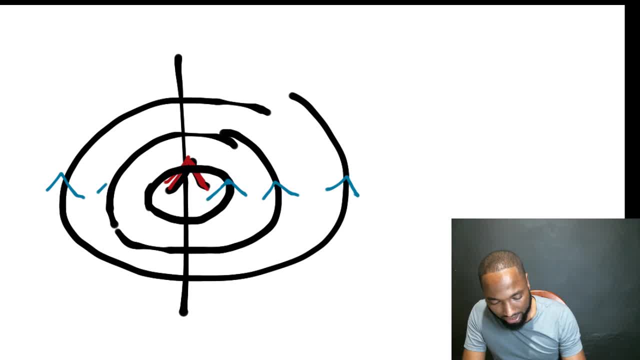 this way? Or should I put it on this side, This right or left? Yeah, Max Maxwell's crew, You just confused me. Somebody seen left, somebody seen right. So our next person said that. my next is a serious already going on here. Which arrows are correct and these arrows correct or these arrows right arrows on the left arms. 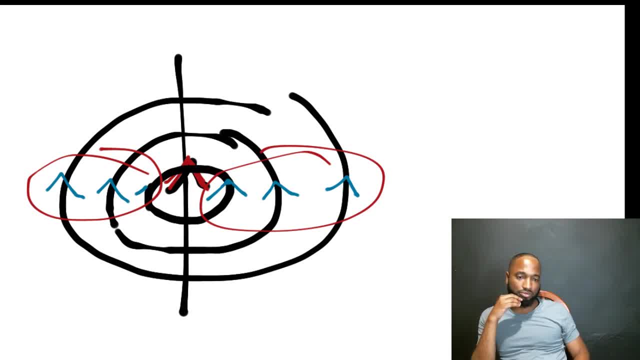 I, I, I. the right, the right arrows, Right hand grip where my fingers cooling in at this in this kind of way. So these arrows following that like this. So the right hand get a watch which way your finger feeling on your thumb running along the way the current is going. 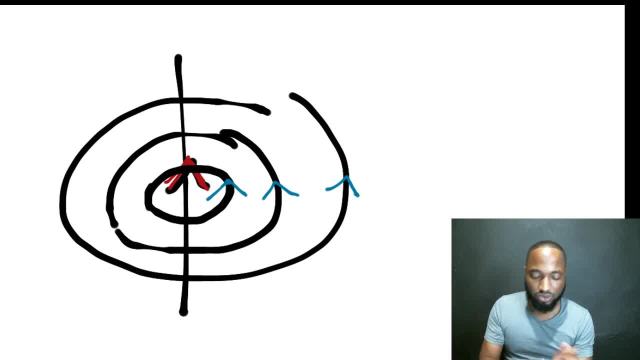 This is conventional current, by the way. So, in other words, I can't put ours like that. They have to power doing this way too. so, Like that, does your right hand grip Right, so flip your screen. No, I don't need to put my screen. I think I could be. 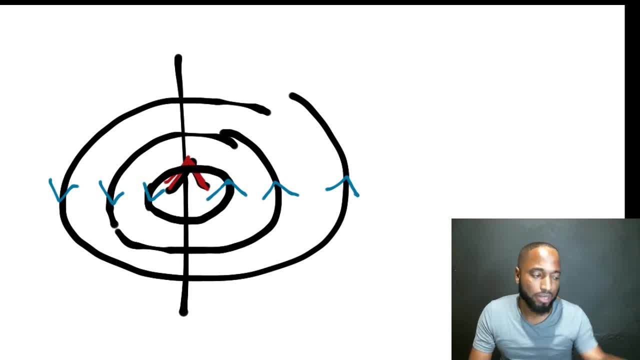 All the video camera. Let me check on. let me check and see if I Have a little more make sense. So I would not be like video here, But like you don't alone right, My camera reverse, Oh crap. Well, that sucks. I can flip my screen, yeah, I can flip this screen. my car and you flip this screen. 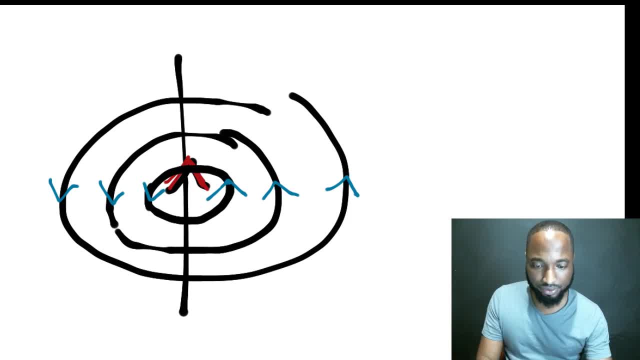 Hmm, Let's flip. it. Clips the screen. now Tell me if this makes sense. I mean I'm flip the screen, Not important when I teach in, a real important when I teach in generators and thing, but Always flip this. I can't represent, But everybody gets it do. 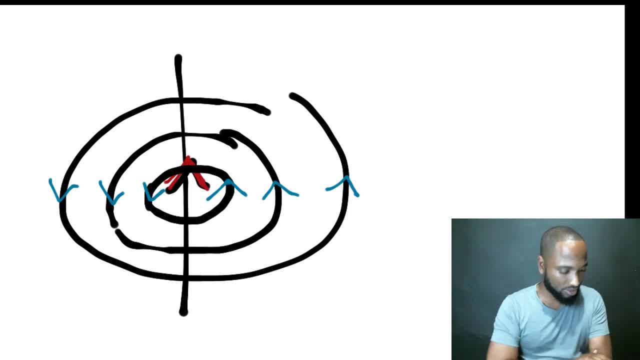 Alright, we get it. I see now Right hand grip. You can see right and grip. now Come on, catch back up with me there. That's the right hand grip. All right, it looks now. It ended with me. Yeah, I can look in me. So right and grip. 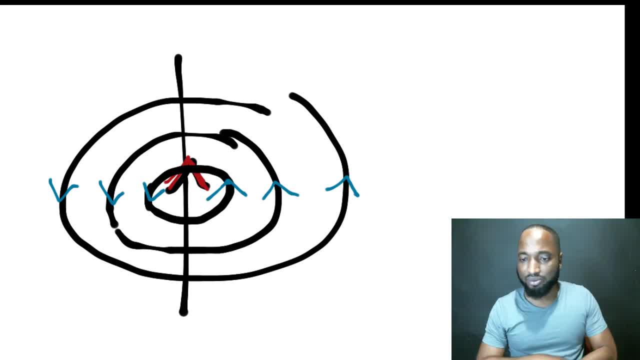 So green, wrong like this: Yeah, we get it, We get it, So that's good. So the right hand grip To the value of what you like, what the heck See right, and your foot side is so we are a finger spoil and tells the direction of the team. 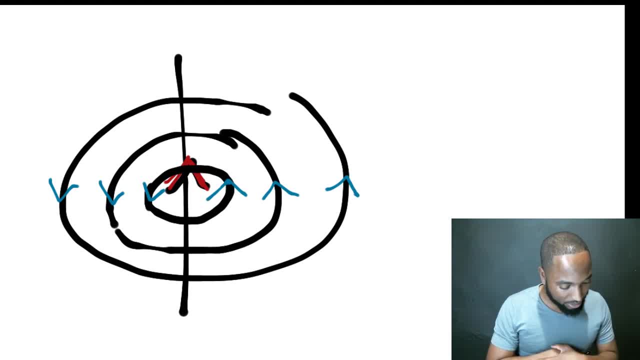 I still get a computer group aligns to the people Already grip aligns. Yeah, I don't watch your finger. so It's like my hand is the wire, My hand is the wire going up soon And I, using your right hand, grip where my thumb. 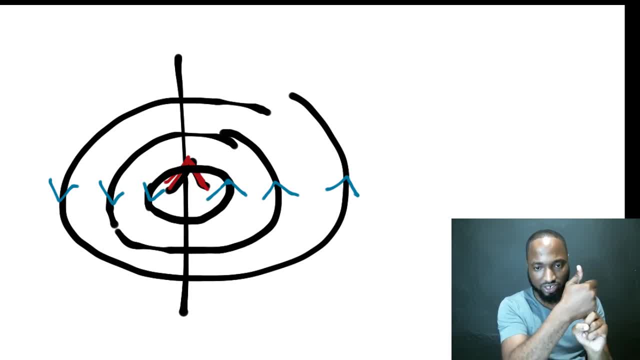 my thumb, Tom, Going in the direction, and we were fingers cool telling you which direction to draw. if you're watching the diagram, That's the direction to draw. imagine gripping the wire with your hand Right. Okay, I, I use my thumb right here to drag the line, And now I'm going to drag the line. 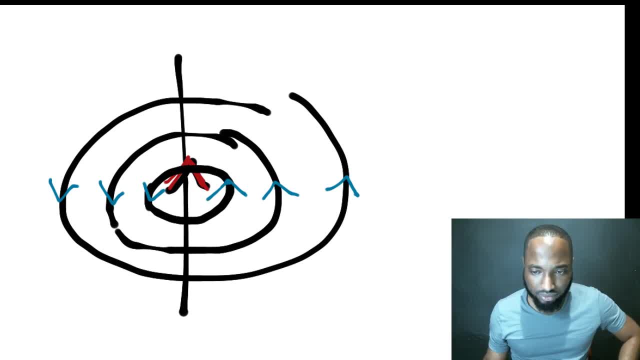 I'm going to drag it to the right side. Okay, I'm going to drag it to the right side. So I'm going to drag it to the left side And I'm going to drag the line to the left side. so I'm going to drag it to the left side. 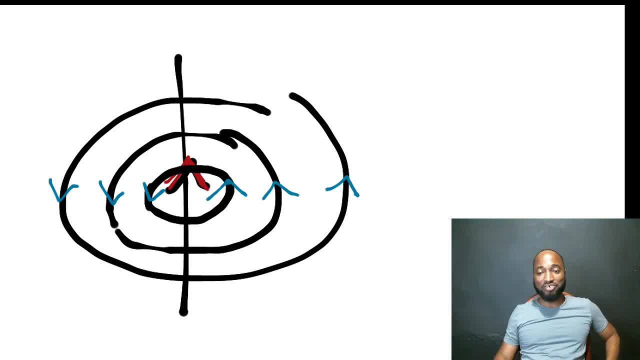 Okay, look, you have a look. message me in my inbox. I finally have some nice predictions. a few people is I like a fool? I see a man at the old wall Who, big um years and things like that, what they could go into some kind of statistical analysis job. 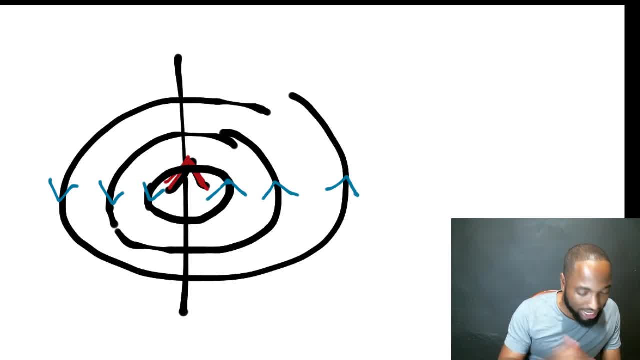 anyhow. so that's that. that's the right hand grip. you spend enough time on that. so this is how the field looks. this is how the field looks in current carrying conductor. by the way, if the current carrying conductor was going down like this, then obviously you draw the same circles, but the 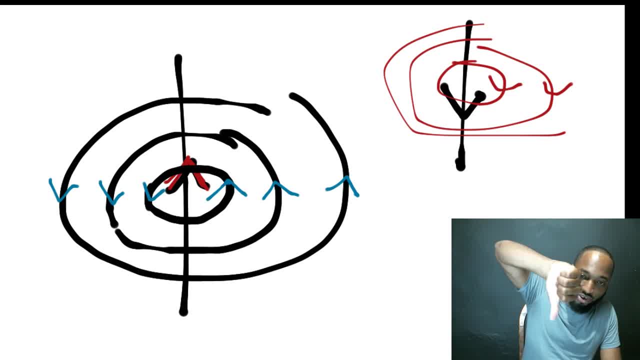 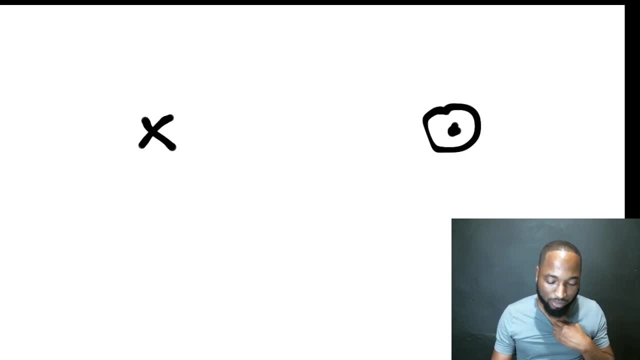 direction would be the next way right, because then you grip it going down. now it will curl this way right. I'm predicting hook slow for the all right. what about in the paper and out the paper, using the same thing for the second? which one of these symbols means in and which one of these symbols? 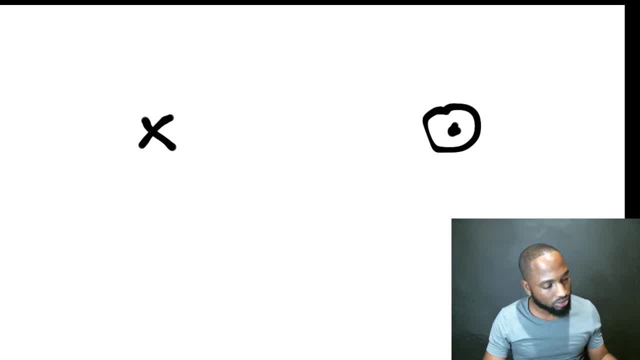 mean out, which one of these symbols mean in and which one of these symbols mean out. so somebody say, shoot in an arrow, the X is in nice and this circle, that thing is out. so X is in, X is in, right. so just going in the paper, hit them the right hand, grip like grip, like this. so we're going in the paper, you're. 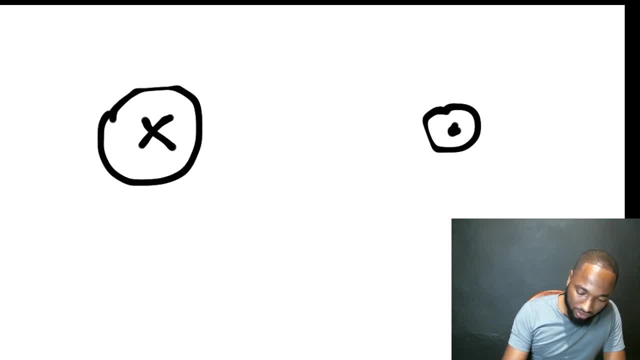 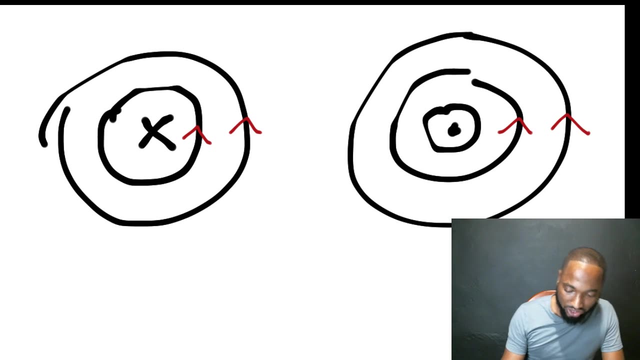 expecting to see. well, I wouldn't say now the answer. so is this correct? I'm gonna put both of them in the same direction. which one correct, which one wrong, which one is correctly left or the right, which one is correct and which one is wrong. nice, what, which one is correct and which one is wrong? I see the top, the top people getting them getting. 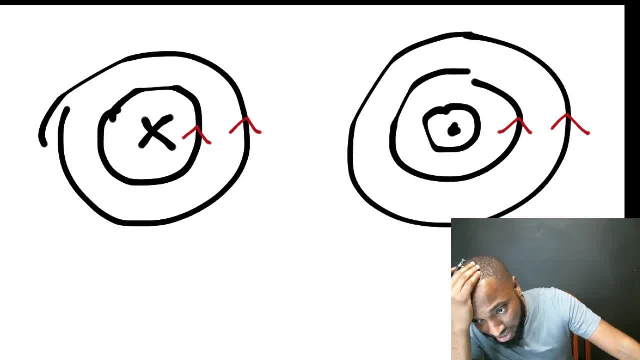 different answers each. let's get some consensus here. grinders- this is the 188 left, the last of the Mohicans, the killers, the people who could go down. you could really grind. let's pull out some consensus here. so some people saying the X is wrong and some people saying the always wrong. 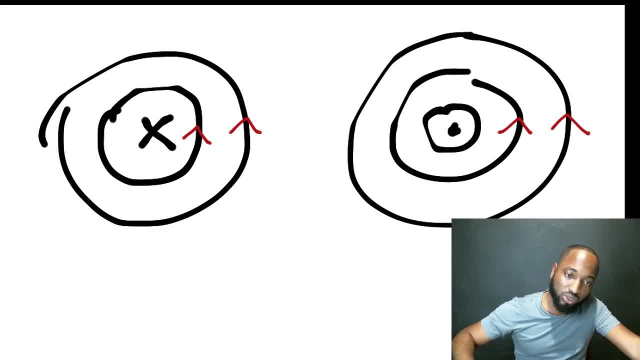 well, let's check it out. X is going into the people, into the people, into the people. right, I'm actually playing my top on it. see my thumb making that squiggle thing. there's my thumb doing that right. and now this is gonna turn like this: 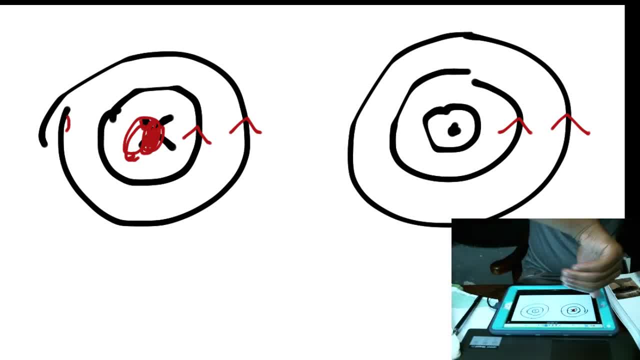 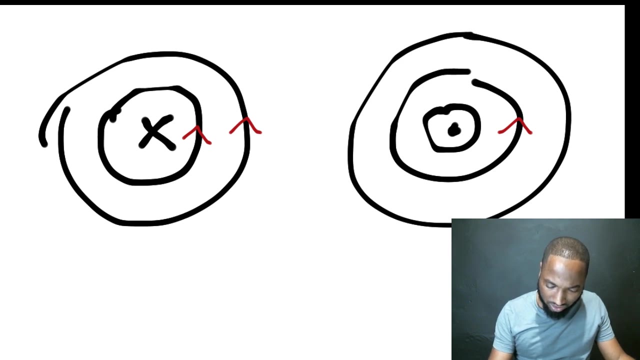 like this, right to do so, because it's in it like that that one is actually wrong. I'm going like this. it's standing like this: I just need to follow the direction of my fingers. bam, bam, right, so everybody good. and now the O is going out of the people, so this: 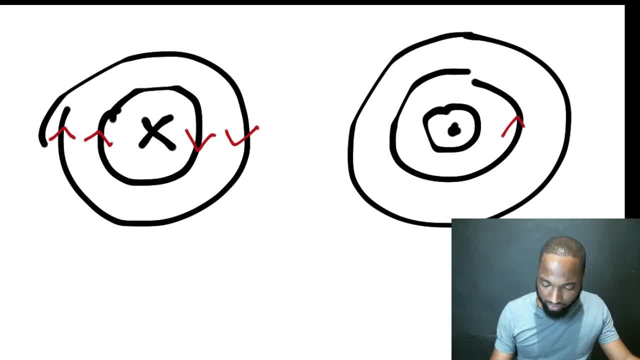 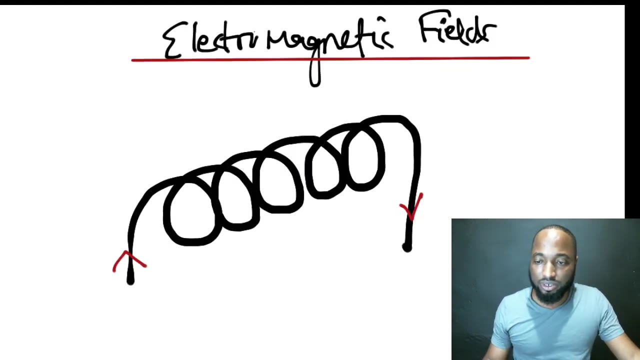 feeling like this, so I just need to follow the directions of the killer of my hand. why is in the chat wise, in the chat curry goat and what's up? chat next right. so I notice helping others, just helping a good few people out at this hundred again, hopefully getting some good work done here. 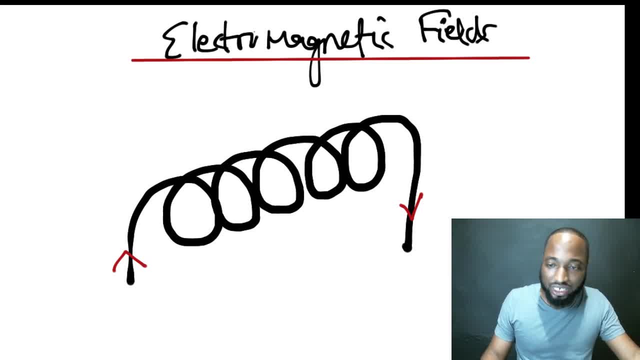 team. will we cut this here? normally I don't go for three hours at a time. it's kinda running up zero to four of us here. it's a pull. it's a pull. now how are we gonna? are we gonna do this one? are we gonna do this one? now people say to me from our faces: 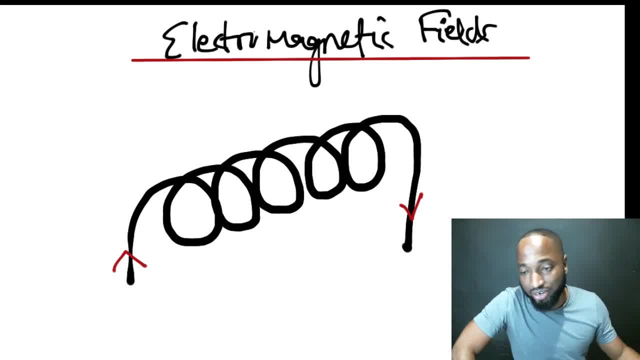 Now people say to me from our faces: can use your right hand grip for this too. there's a way to use your right hand grip for this, but it's fine, it kind of tie up now. so the best thing, I'm gonna tell you the method that is used for this. see what I do here. I'm going to tell you the method that I. 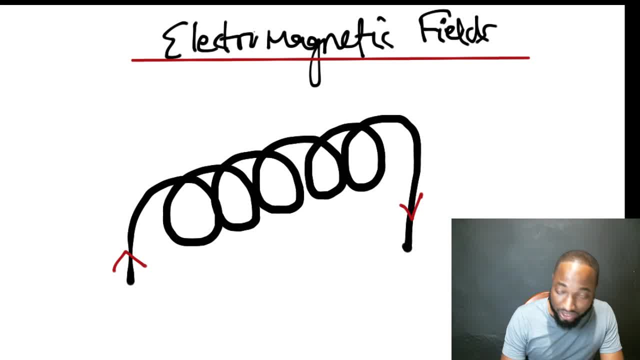 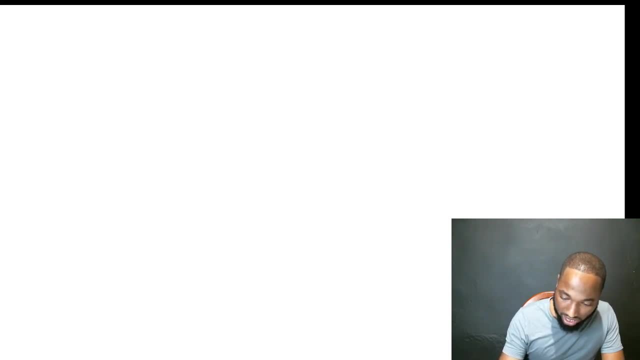 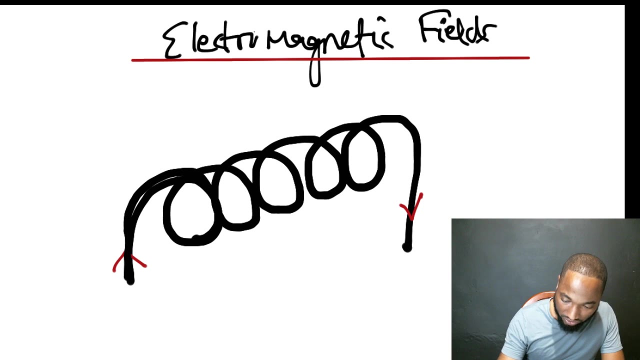 use for this and hopefully it helps somebody out here. hopefully I think of this where doesn't sit in a new slide. you see this part here. think of this part here. like the attention it like that. that difference ring right, how's this that says ring current is going up in. 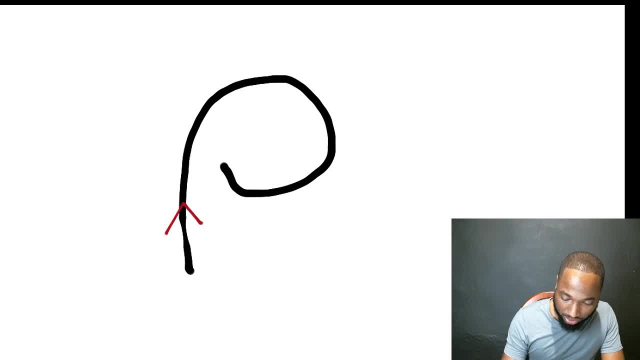 this example. it can be going down up getting it right. it's been up. there's two things I, Colleen, I learned me. note anybody else. leave your post a comment and i shall continue with the next video. it like this and then in the salt. this is how I lean it. anybody has linked it. 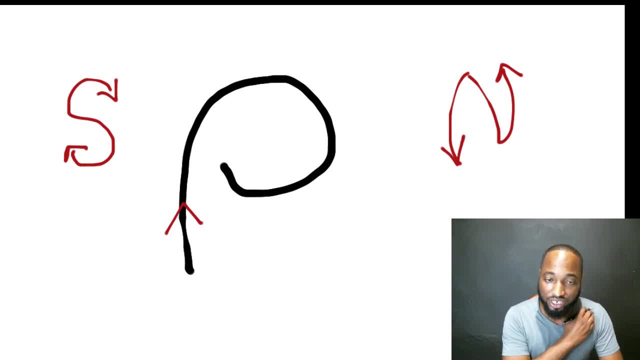 like that. so I'm going to learn the North Pole and the South Pole and then I'm gonna show you why. and to me this is this is like- because sometimes in this Illinois they suddenly believe in the North Pole and the South Pole. so I might as 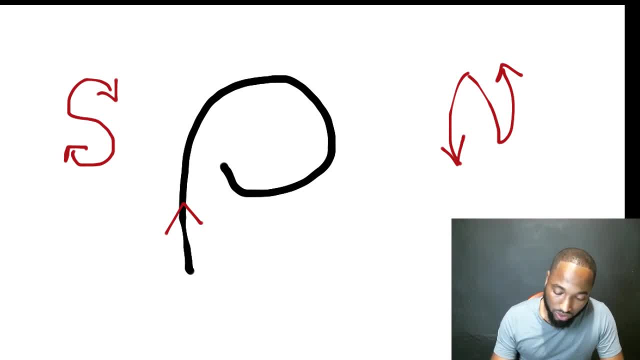 well, just lean it like this, you understand. so, since the current going up, the only ones fit not in here because Norths not fit in here. this telling me that the current going 스 it in here. when Republicans not saying that current adequate, kind of one thing, what by the current actually going? 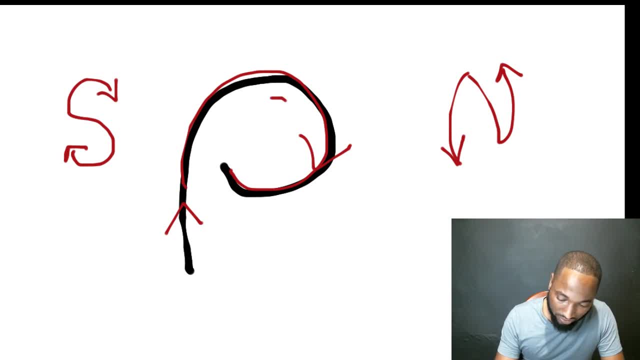 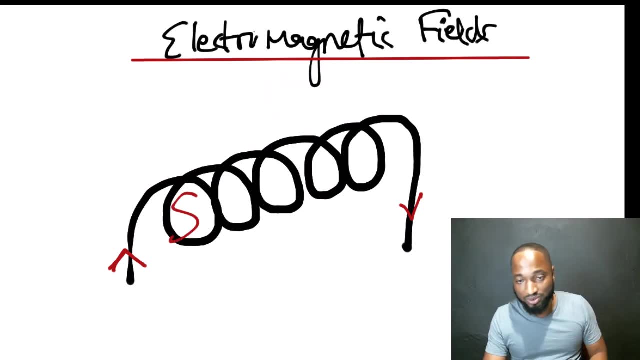 clockwise, and so you current going. so why are you foot in you South Pole? so just mean this is the salt, that's it saw Poole, and if I watch it from there at this South Pole, That means this has to be the North Pole. Now, what do you know about South Pole? 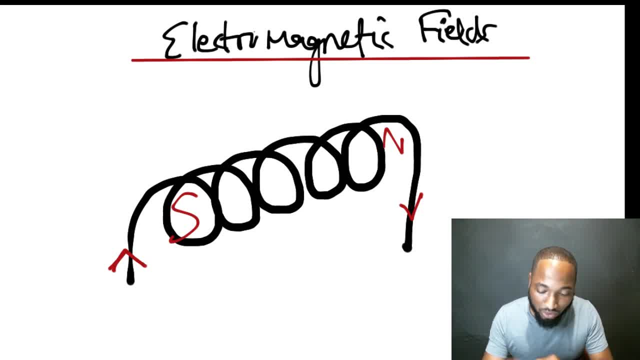 and North Pole. What do you know about South Pole and North Pole? The current is leaving. which side, Which pole will the current leave? Which pole will the current leave? Current always leaves, or the field, or the magnetic field will always leave the North. 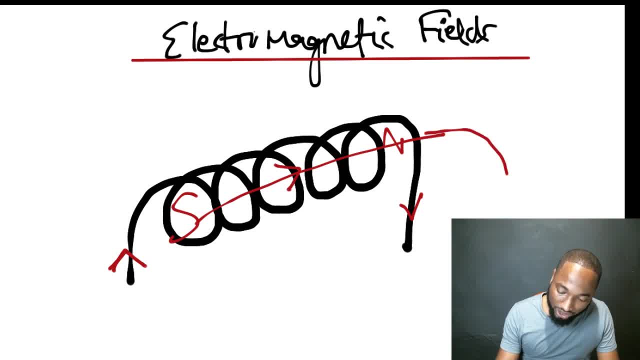 So it will be going through like this, busting out the North and coming back like this. So let me get a diagram from the internet: Solenoid, Solenoid. Let me see some wise, if you kind of understand that. 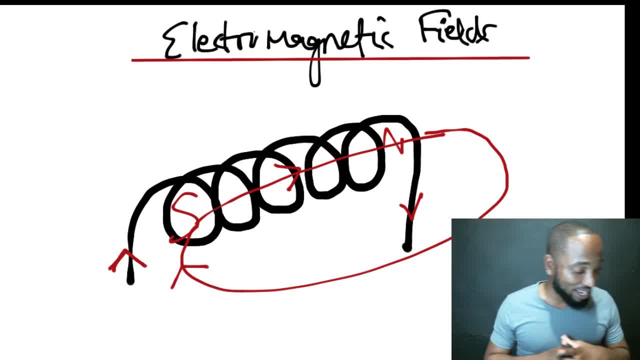 Hi, She was at 41 minutes past. Alright, I'm looking for what I'm looking for: a solenoid. You see when, when I get this later, I start to get a teaching holiday in school. Went and fixed some program. 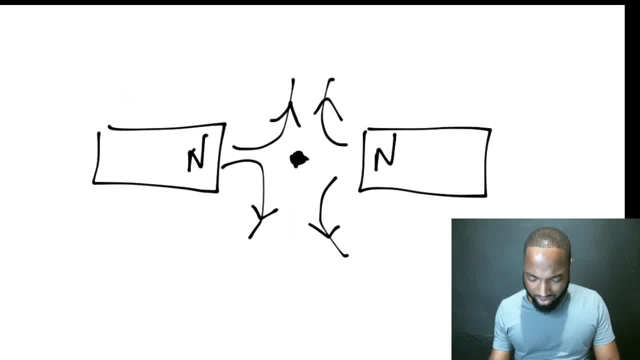 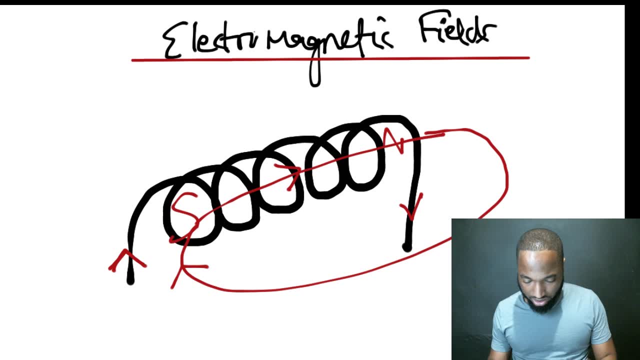 So not program, just fix up something. What I'm looking for- a solenoid electromagnetic field diagram So I can explain again. once again I can explain some nice explanation. Some of these diagrams are real extra boy. It's a bit too extra for me. 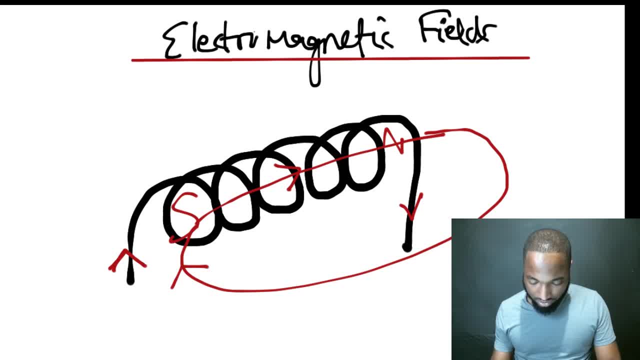 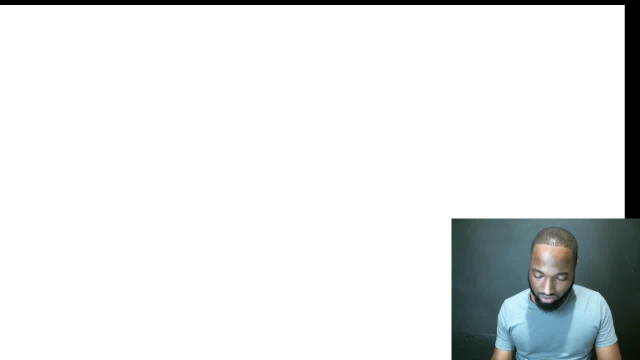 So I think this is like the last thing we did for the night. So just hang on, just hang on, I will do. I'll save the generator for next Next class generator and Motu. So here we have a solenoid. 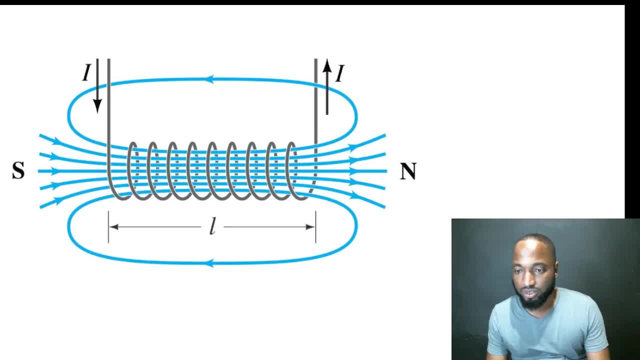 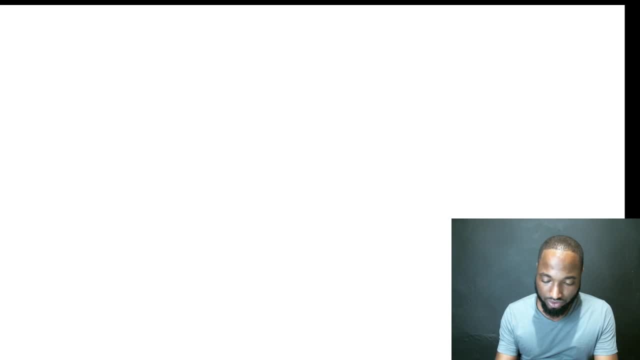 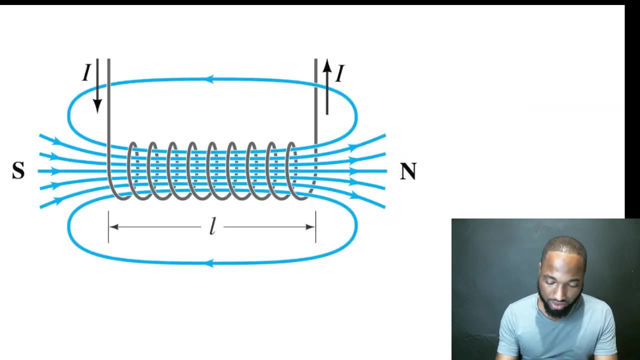 It's a little different. It's a little different. I don't know how to press. I don't know how to press, I'd call off. I don't know how to press right. So once you figure out that method to me, you're safe. 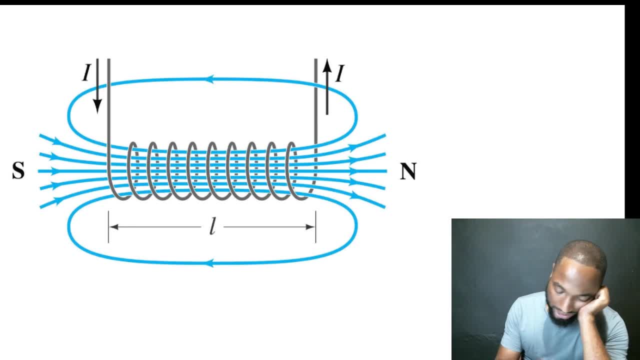 You're safe, You are going live tomorrow for sure. Okay, let's see how we'll use it in this. Now your spatial understanding need to be good. You need to be able to see things and people and kind of visualize it three-dimensional. 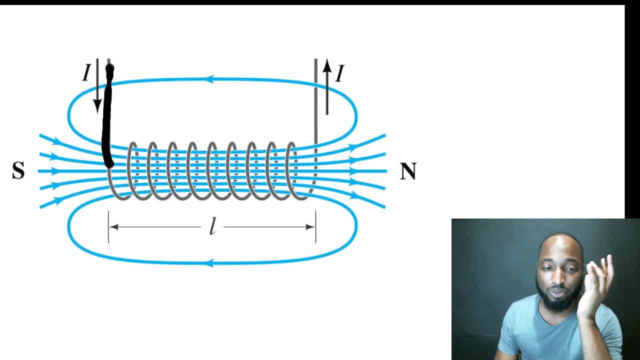 And I understand that there's a percentage of people that that's just very hard to do. It's basically how you grew up, what you was exposed to when you was growing up- Leg moves and them kind of thing, and how much of that you get exposed to, right. 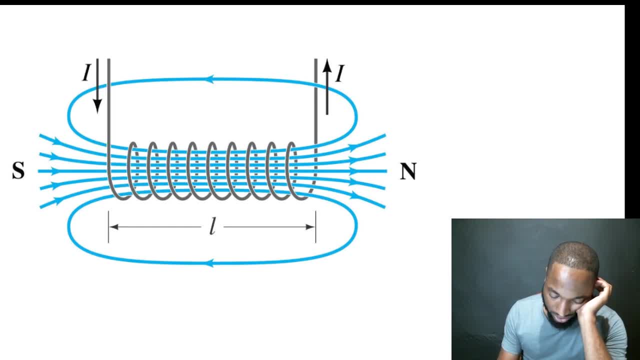 So there's this going like that. Now you're seeing it going down and going across like this. So if I was watching from this side, this is what I would see. If I'm watching from this side, right, This is what I would see. 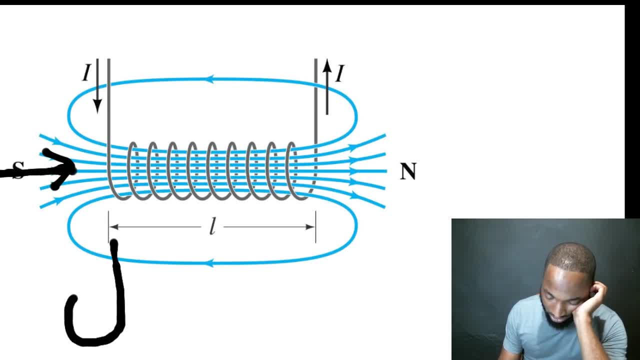 I would see something coming down like this and turning like this and going back into the people. So now I can use my North or South pole test because the current is just going down like that. Remember, the North says that the current has to go. 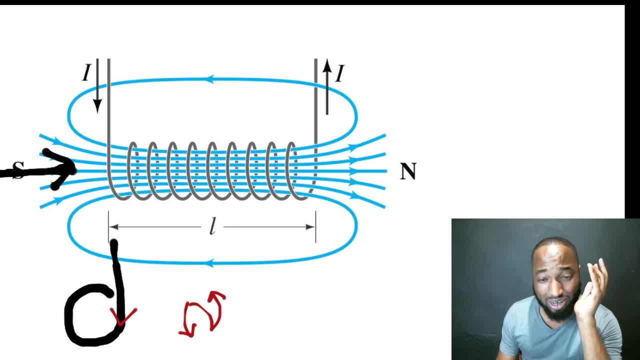 Clockwise, Sorry, anti-clockwise. The North pole says that the current has to go anti-clockwise, But this current is actually going clockwise. It means that this is North, This is actually South, And when I put my arrows on the edge of the South, bam, it's working man. 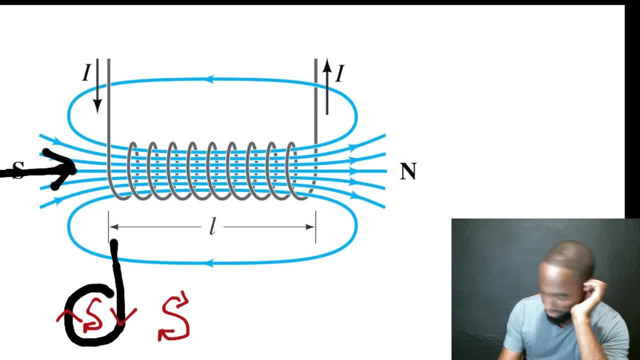 It's working. It's following the pattern, right. So this means that this here is the South pole- And if you watch, they label it as the South pole as well- And this here is the North pole. Obviously, if you're finding South pole, you're finding North pole. 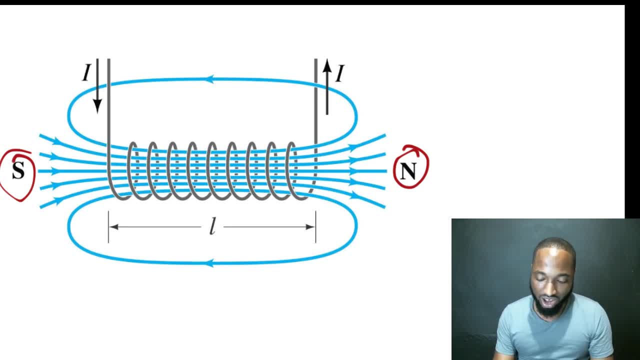 And the electromagnetic field will. To draw the field now is easy. It will leave the North and enter the South. It leaves the positive, enters the negative. It leaves the North, enters the South. Why isn't the chat That's solenoid for you there? 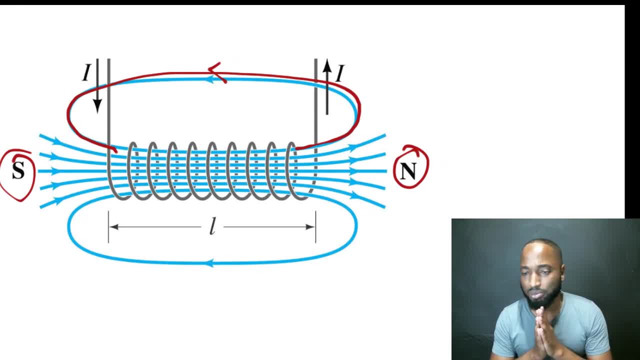 Now there's a way to do this with the right hand grip too. I'm not going. I'm not going to that. But if that will float you Right hand grip, Okay, Let me explain using the right hand grip then. 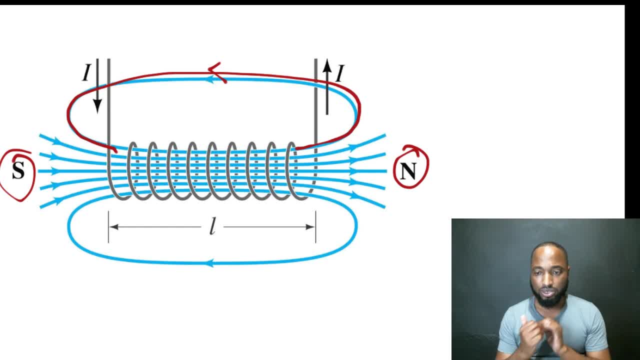 With the right hand grip, you're following the You're following. But keep in mind, even if you have the right hand grip, you still need to know how to label the North pole and the South pole. Let me explain the right hand grip. 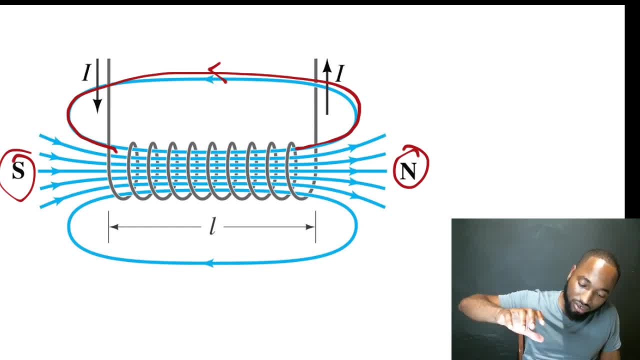 With the right hand grip, you're following the curl and the solenoid, So the solenoid curled in like this: You're following the curl and the solenoid And your thumb will point in the direction of the current. That's it. 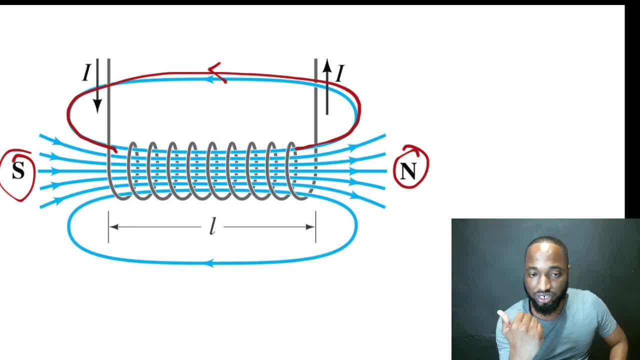 So your hand needs to follow the curl of the solenoid, The curl that points in the direction of how the current is going, And your thumb will point in the direction of the electromagnetic field. Right So the right hand grip. If that floats in your boat, free up yourself. 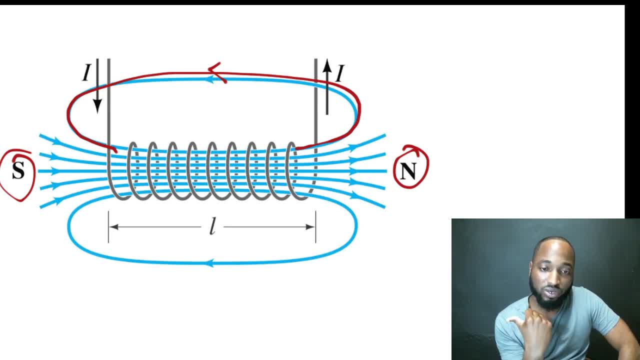 And if you want to use the right hand grip to try and figure out which pole, now Remember, after you figure out the electromagnetic field, which direction it's going in Curl in the wrong way. No, I'm not. I don't know if you're seeing something wrong. 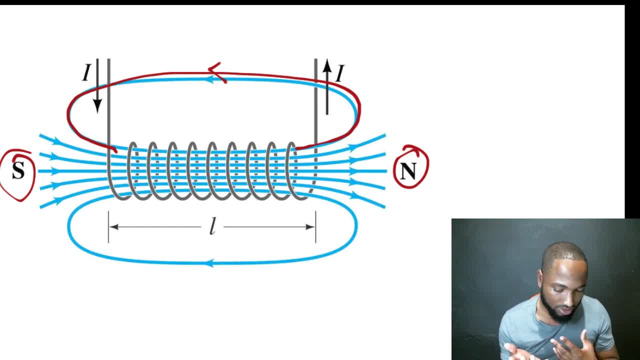 But I curl in the wrong way. I am not curling in the wrong way And I curl like under. so Because it comes down and goes forward like this, right, So it comes down and goes forward like this. It comes down and goes forward like this. 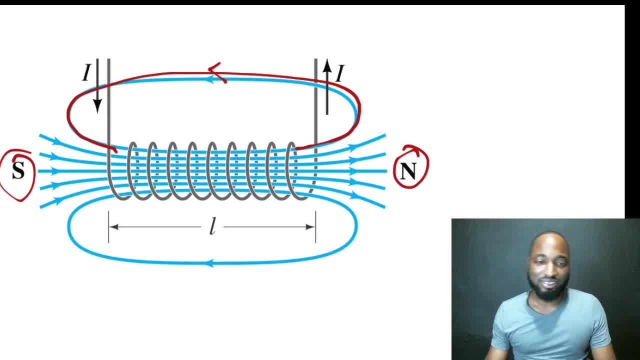 And it's going so All right. Yeah, So we feel going so. Well, I actually pointing in the direction, that thing pointing in here, But when I do so now it's pointing so in the arm. You understand what I mean. 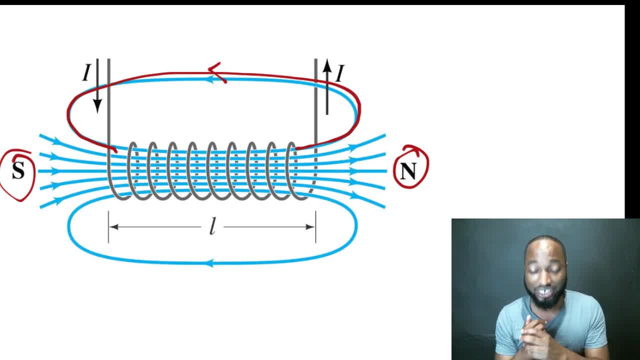 How the camera flips. That's what's happening. It's pointing in the correct way. Trust me, How to show this boy. This inversion thing is real messy up. when you have to do this kind of thing, Face the wall. Thanks, Luke. 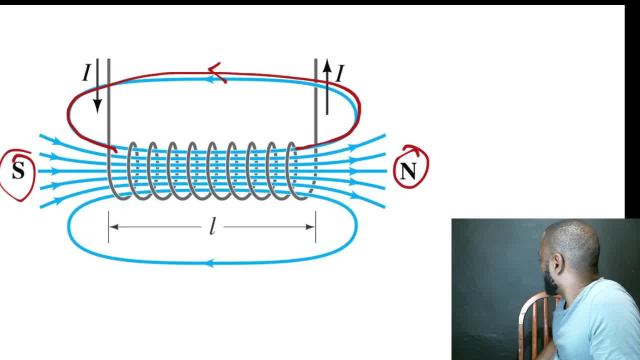 Thanks my brother, Thanks my brother. So curl underneath. I just repeat that. This is what I'm saying, Little like this: No, They're not helping me, They're not helping me, Forget it, Forget it, Forget it. 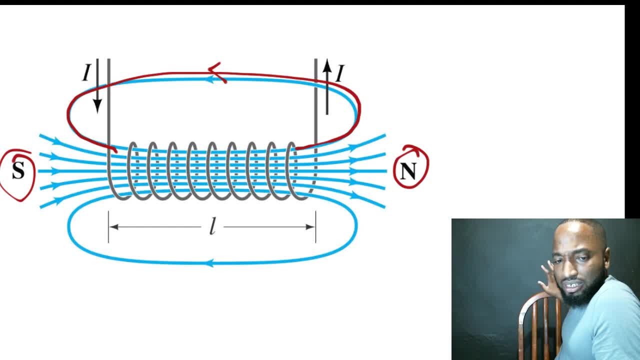 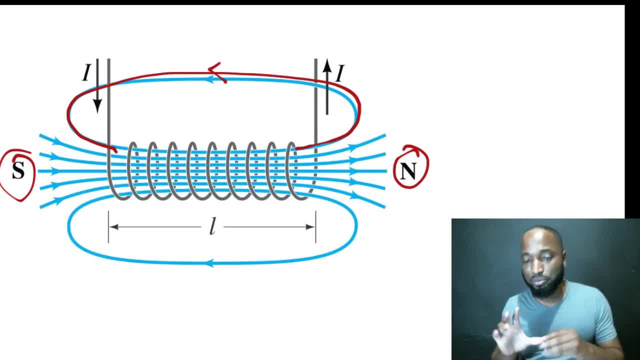 Where the How, the solid noise is curling And the tongue represents the direction of the feel. It was a good night. It was a good night. I wanted to. I couldn't finish where I wanted to finish. I have, like about what? 10 more pages to go. 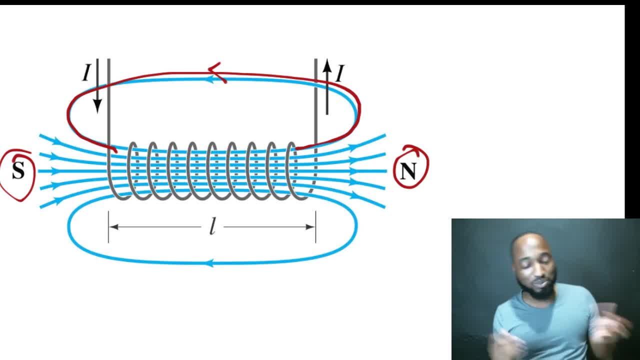 Or less Five. Five to 10 more pages to go, Which is basically motorcycle and generators, So that'll be a separate video by itself. That might take me an hour-and-a-half-hour. That'll be a separate video by itself tomorrow. 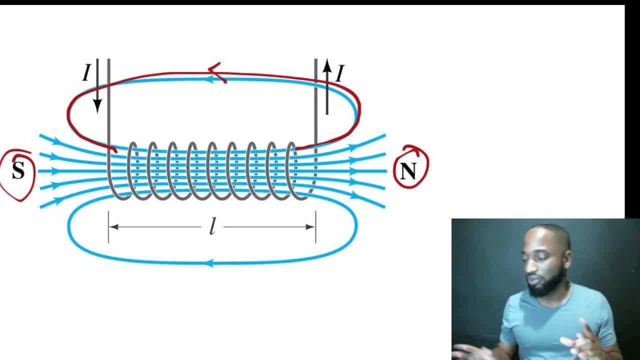 I'll start the video with that. We wait, You're welcome. from about 350 people to 200, which is not bad. normally it's dropped down to hundreds and in the hundred and thing. all right, so i'll do that magnetic thing tomorrow, then i'll do waves optics. 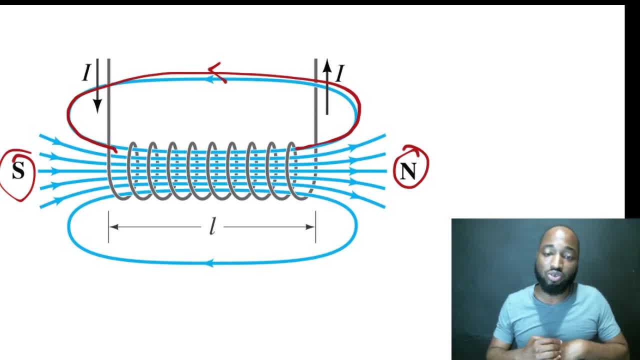 then i don't know if i have time to do anything else. i may have time to do the first part of chemistry maybe. maybe i can do heat and gas laws and things. maybe i can do those kind of things. that would be the night before the exam, that would be the diet, that would be the 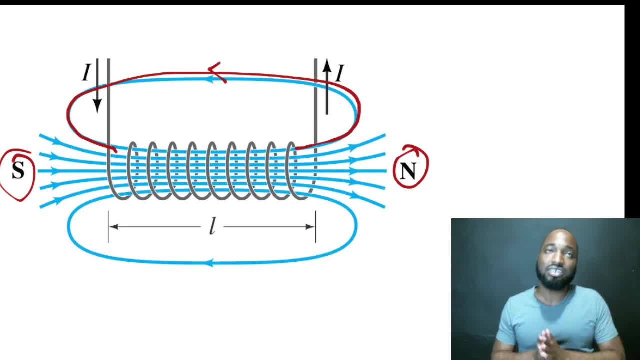 killer session. everybody's being signed and in between all of that i need to get time to do some it. hopefully i can do some programming and i need to get a man say i think the hair going back, of course. of course i need to get time to do some integrated sense. so some infotainment and some. 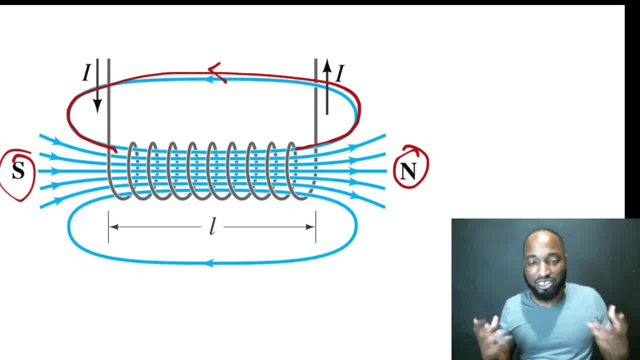 integrated sense. hopefully i get time to do that, some of that, while you see what going on right at the balance. but the balance work at the balance. time with my kids i had to do my son's help, my son do his homework. that's something plus: i'm a helped. 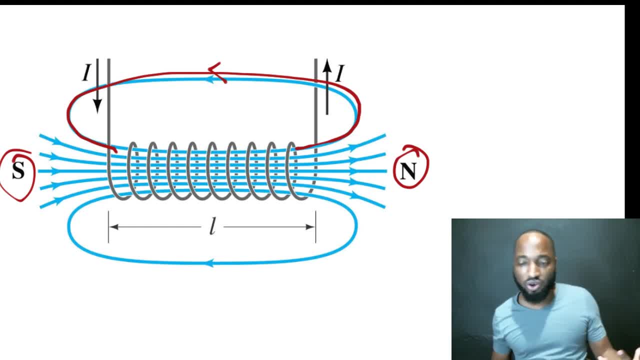 and as young as i used to be, so i can't be going without sleep for too long periods because i can damage my organs anyway. lessons we'll be doing multiple choice: geo, chem, physics, bio and maths. multiple choice. pull it up. can the thumb show you not? yes, thumb points to the 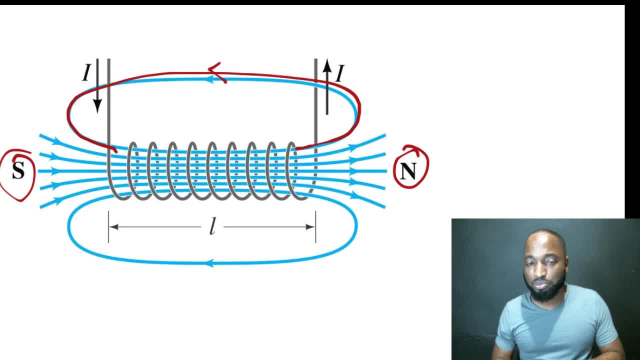 note: the thermal point to the note. you're using the thumb to point to the note, so the thermal should electromagnet the field. so it's going to point to the note and out. right, i always make appointments with my barber, doc, but i was in a hurry, like i was always calling you. 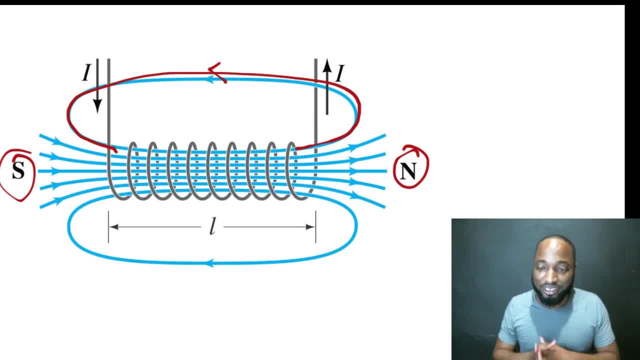 and he said, yeah, come through this time. and thing i- i have a barber set up, it just has just, it's just a pure bad day that caused this, this here like thing to happen. pull it down. you welcome. you welcome to all the people who say thanks. and thing this was a nice cheer was then 15 minutes. 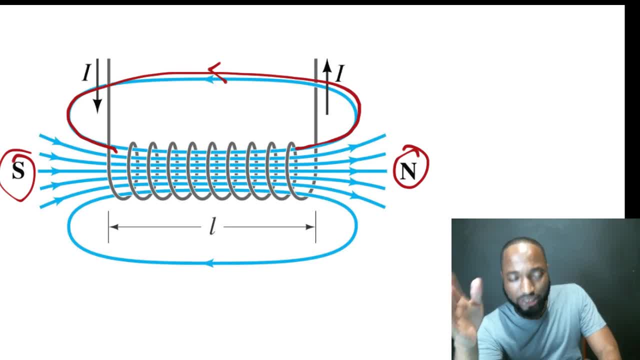 if you haven't followed me on instagram yet, follow me on instagram. my instagram look wet and also i do surveys on instagram. i figure out what people want to want to do and i post encouraging stuff. if you're off of instagram now for exam time, it's okay, it's? 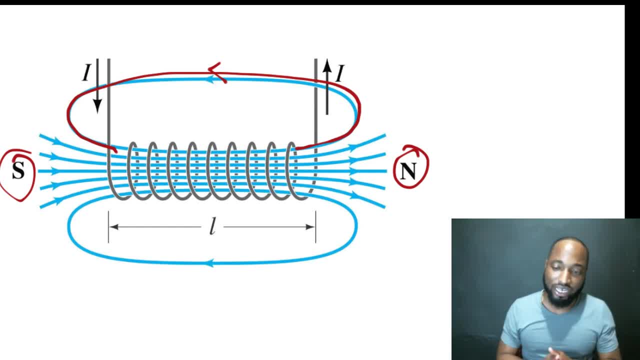 okay, you'll go on instagram just to follow me when, when i, when you have, instagram could be extremely distracting to students. when you come back on, we can link up lessons. i'm real good ideas and things more coming, what i'm going to do after exam season. for those of you all who don't know, 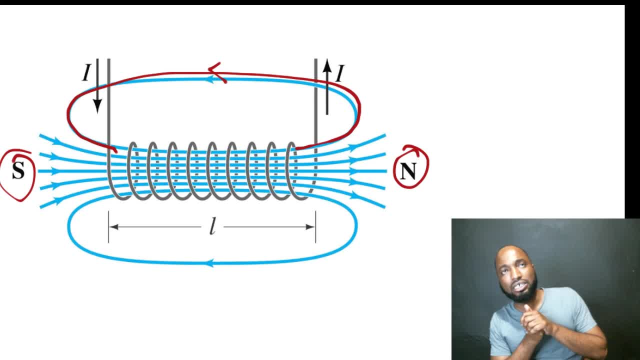 who- a lot of you all who do physics here- will probably do pure maths. in about six i am going to have an online pure course. it's going to be 200 a month, 280 a month, if you're interested in that. your registration for that will start in two weeks. there are already people registering for the maths course, which is 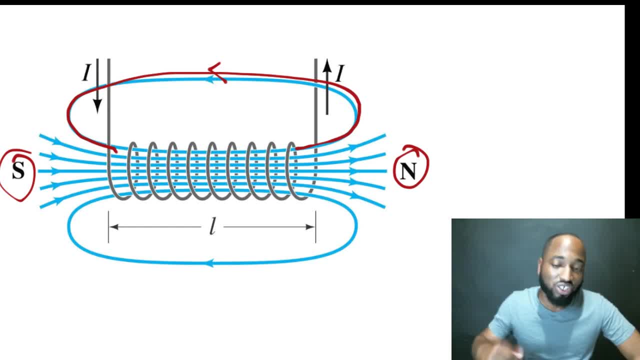 going to start in about a week or two, but the registration for the yo if your maths class starts in july, so we have time for that. if you're going to do your maths and you want to work along with me in like a class like this: every week, every week for two hours, um, every week for two hours and then. 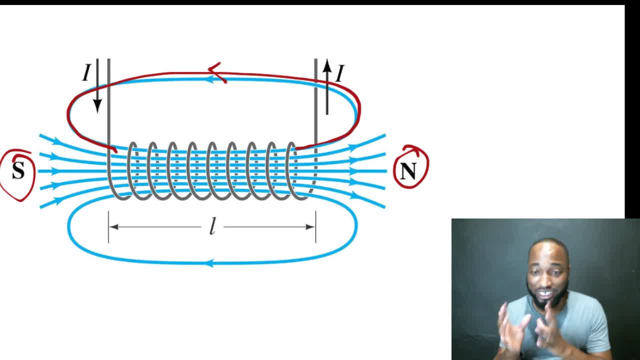 you'll be in a whatsapp group that does does. i feel like that's me almost as important as the life, because right now i'm a whatsapp group with- and i'm sure some of them may be here- a whatsapp group that i did for the advanced crash course and i didn't. i didn't delete the group, i left. 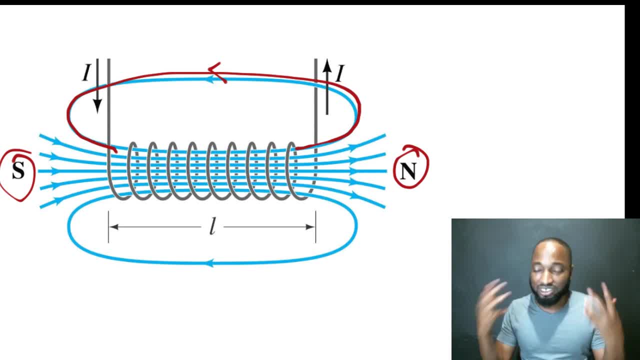 wow, that group was very, very helpful for the students there to get past people's notes, pass along this, send information, ask questions, get help from each other, so that'll be really nice for pure start to get a little harder and you have to figure out stuff if you're working along with. 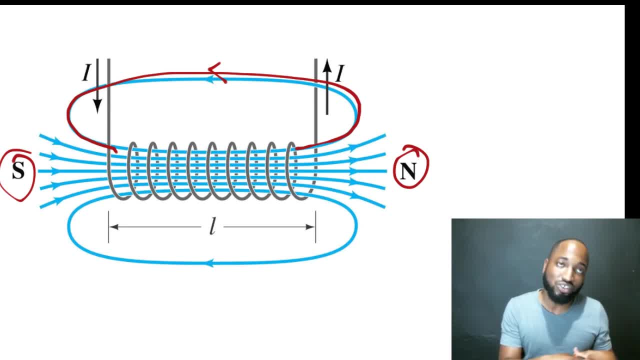 me in that you will be exposed to that group. you'll be able to converse with each other there, so it's a good idea. so look out for when it's when the registration starts. when the registration starts in two weeks or so, i just need to make sure i have everything organized. 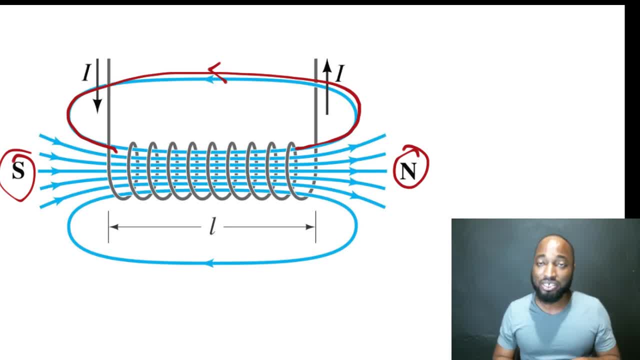 i also need to fully polish up on my pure maths because i haven't thought i i didn't teach pure maths this year. i just need one kind of way right and i used to teach pure maths privately all the time. so i just need to polish up on the syllabus and make sure everything runs smooth and make 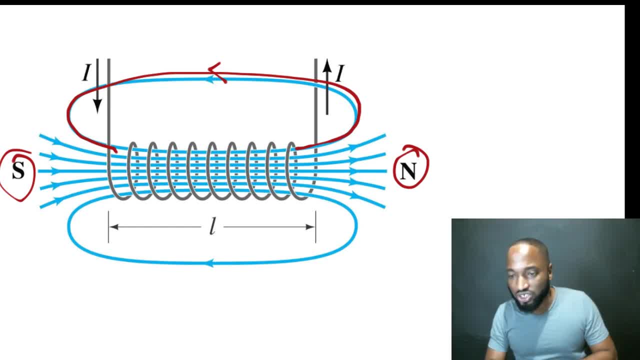 sure everything is well prepared. i see people going so goodbye. so you teaching, keep, i teaching it longer, fully polish up the forehead and excess gaming. you know you're gonna just come out, so how you find advanced examples, i find it was really nice. there's only one tough question: the stationary. 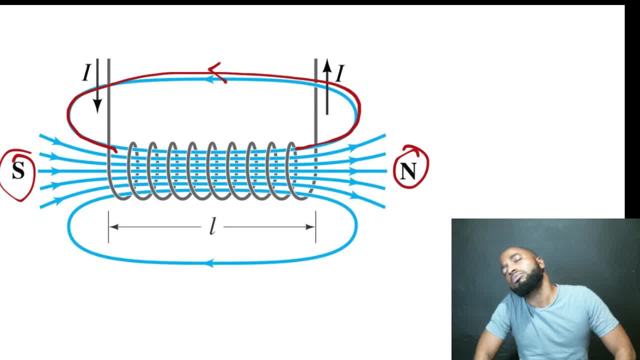 points question: what time tomorrow? so about six o'clock five six um. economics is a science, science and i don't teach economics for business. i don't drink red bull. yeah, yeah, yeah, all those things coming, i'll, i'll have a nice station. yeah, that's the point question. but i already have some people on instagram already. 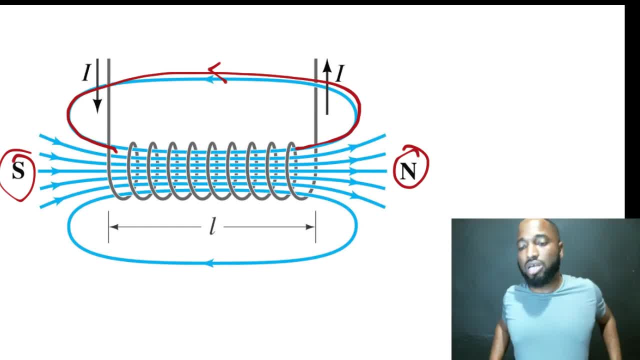 all night and i don't know all night, just so, just so. i need to, i need to live, i need to live. people, living is. living is nice too. you know. living is good too. um, so where is the class? what class is that online class? so the classes in your bedroom? 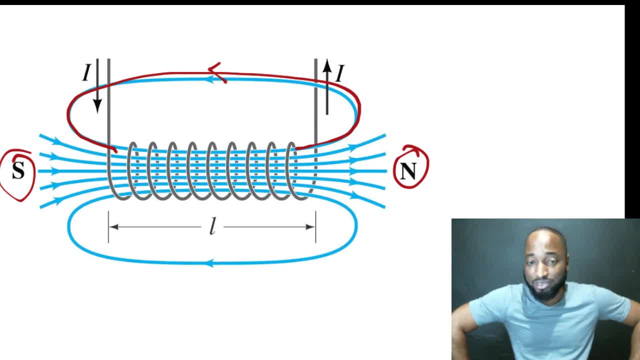 the classes in your study room, the classes at your table, the classes wherever you want it to be. the class can be in starbucks, um, wherever you want it to be, the class will be, because the class will be running from your phone, from your ipad, from your laptop. you'll be getting a private invitation to 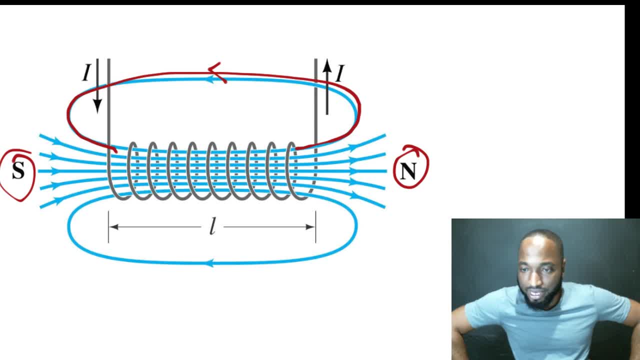 the class i say thanks so much, bye. business will be thing bap. uh, thank you for typing on star madness for physics- maybe out, maybe about six o'clock. online classes for in january max. if you're interested in your online classes for january max, this is the number to call for january. okay, just. 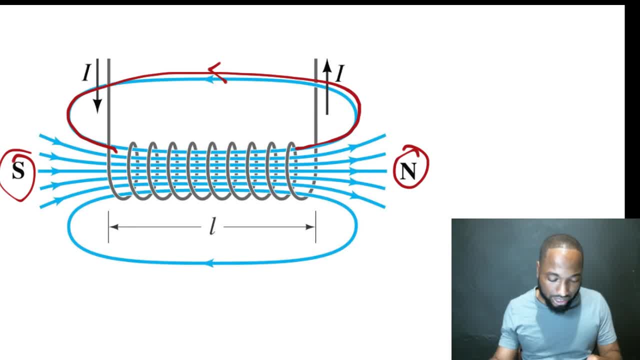 for matzah, for mads. let's give this number very quickly: um 7, 90, 8, 8, 1, 3.. this would be the number to register for the pure maths as well, so you could probably take it down, but don't call it yet for the pure maths, because the pure maths hasn't opened up. 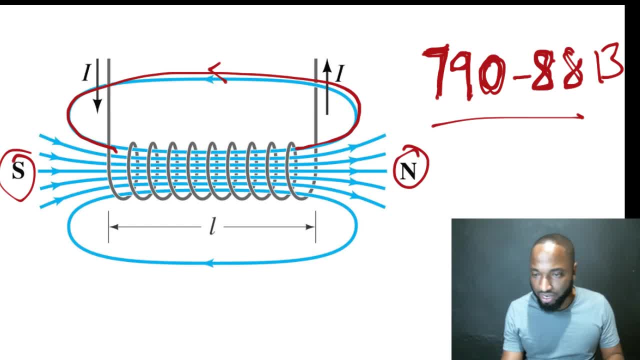 registration right. any other questions? i never went to starbucks. multiple choice for real, though. yeah, the multiple choice pump coming right after them physics- and i'm saying so when it's in- protect. i don't know if you do a prediction for the topics in season, um, i don't know. tomorrow 6 pm, they pass in venus and making a people. much love, much love. 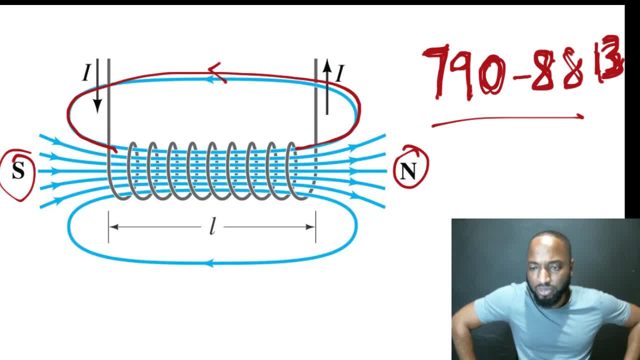 my brother. so you're not tired, i am tired. do we have to reset maths? unsure about that. unconfirmed. i find cx notoriously quiet with this point. yes, why? why? senator in senator update down again rumors that this one see that, this one see this. people inside cx is saying this, this one. 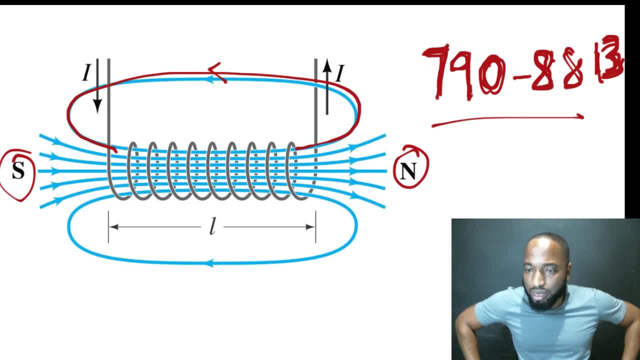 send out our update. um, so follow me back on ig. okay, send me a message and tell me to follow you back. if your profile is edifying to me, i'll follow you back, like if you assume substance now because i don't have profile, like it didn't struck me to.